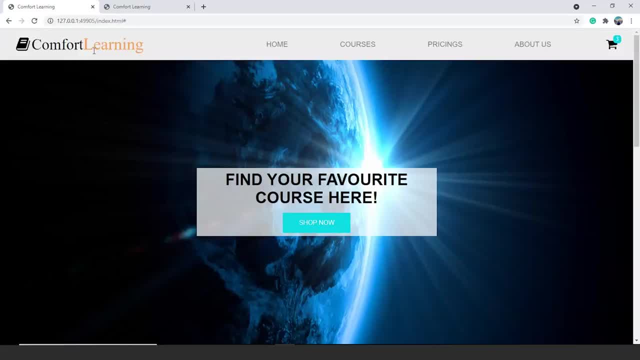 the book to let the user know that this website is for them. So we'll see further in this video how we can use these logos and all. Then we have links for several other web pages of our website that are not working because we haven't added these web pages till now. The reason for this is we don't want to make 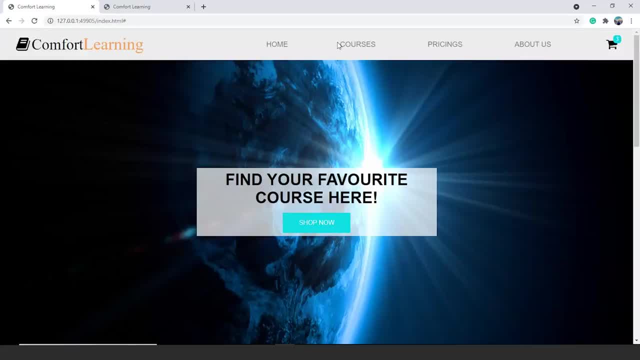 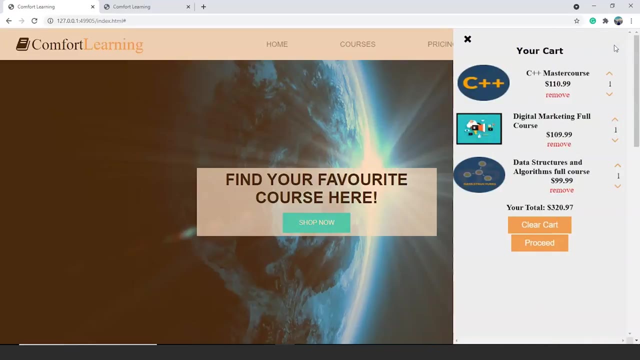 this project a long one. We want to finish it quickly and we want to give you guys a basic idea of how to use JavaScript and other technologies to create a fully functional website. Next up, we have a cart button over here. On clicking it opens the cart with items. 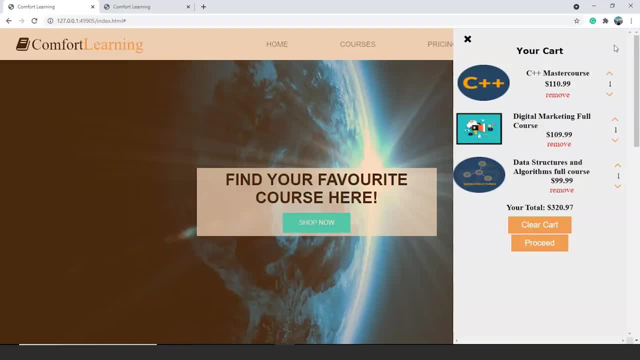 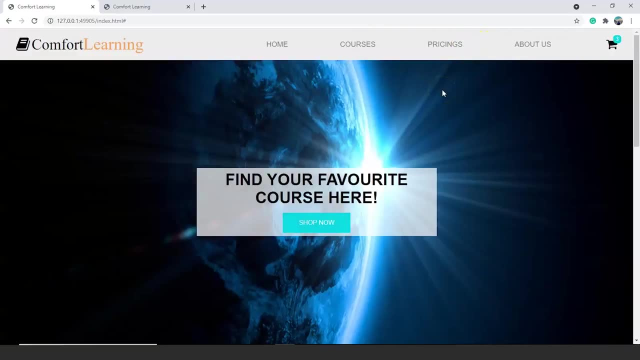 present inside it and the user can either clear the whole cart or proceed further to buy all the things they need Right following this cart button. we have a background image over here with a cart present over the image. The cart says: find your favorite course here. 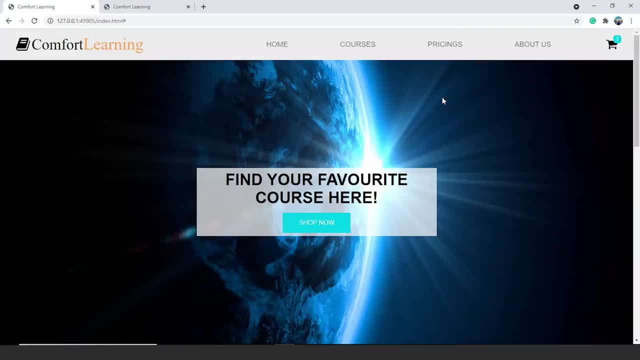 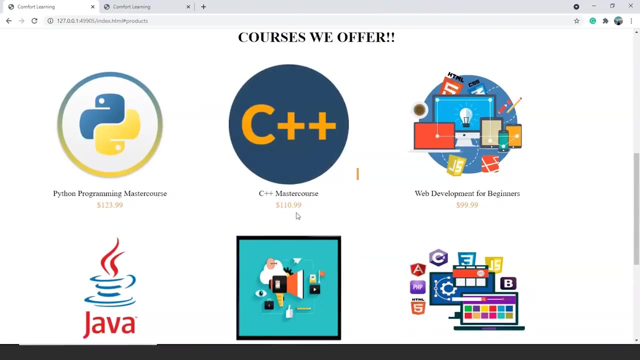 Now you guys might have guessed that this website is for buying courses and the user can buy some courses here which they want to study. This shop now button is completely working and if we click on it it will take us to the courses catalog, where we have several courses present to choose from. We have 8. 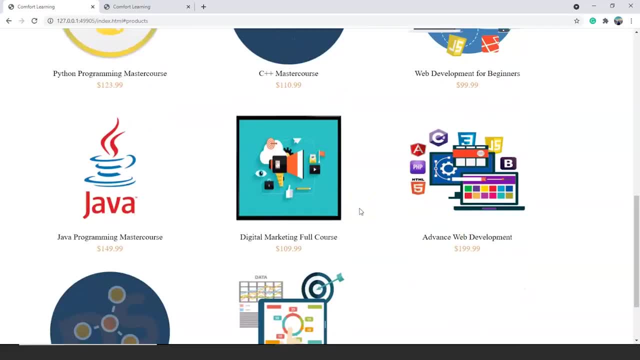 different courses present here. You can add as many courses as you want or as many products as you want, So we can add any of them to the cart. On taking the mouse cursor over any image, You can see it gives us an option to add that particular product to the cart Right. 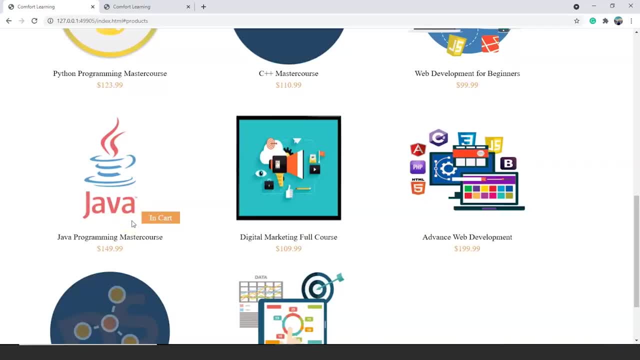 If we click on this add to cart button you can see it says in cart. It means that we can't add any specific course to the cart more than once. We can later change the number of items in the cart, but we can add a course only once. 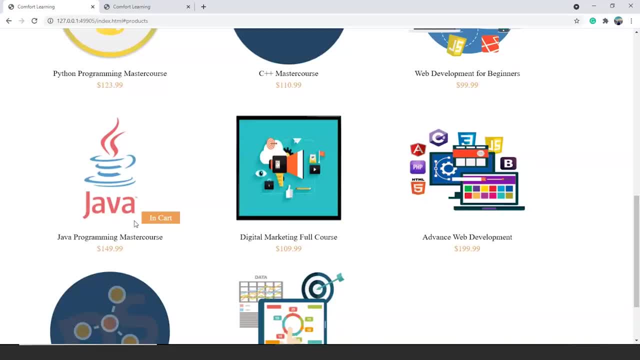 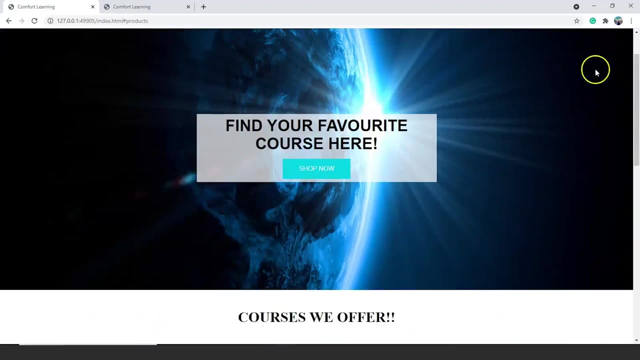 from here. Let's add some courses to the cart and then we'll see if it's working or not. So we'll add few courses. We'll add this one, So it says this course is already present in cart. Similarly, this course is also present and we can add this course. Now we'll move to the cart. We will. 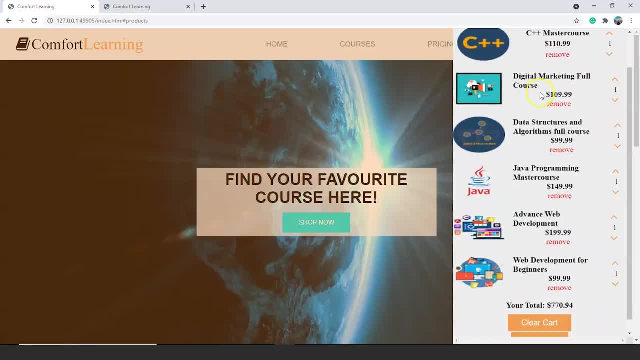 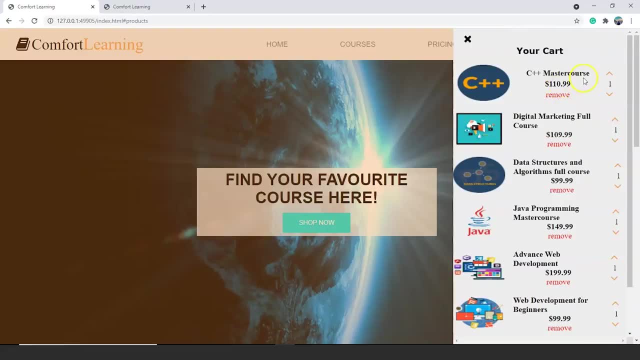 click on this cart button and you can see we have all the courses present over here. Now, if you notice, here we have these small arrows present right. We can click on these arrows to change the number of items. We can either increase the number of items or we. 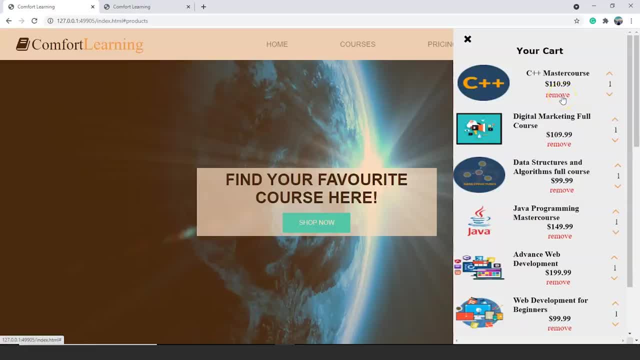 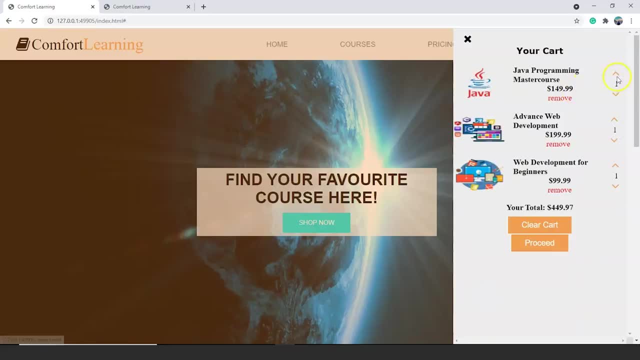 can decrease number of items as well. then we have a remove button over here, and if we click on this remove button, you can see the course is removed. now we can remove any number of courses we want and we can also increase the number of products in our cart following it. we have two options over here. 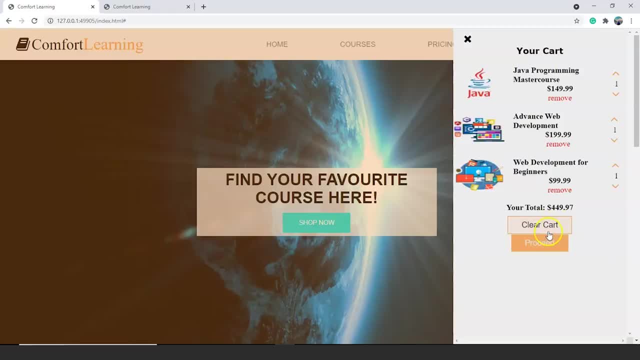 either we can clear the whole cart or we can proceed. if we click on this clear cart button, there will be no course present in the cart and the total price will change to zero in that case, fine. so i hope you guys must have known the task by now. it's clear and seems effortless, right? but 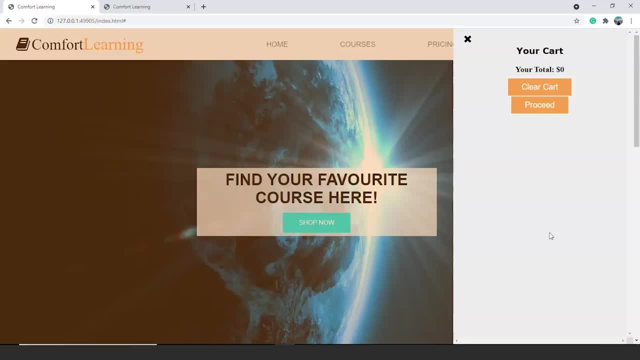 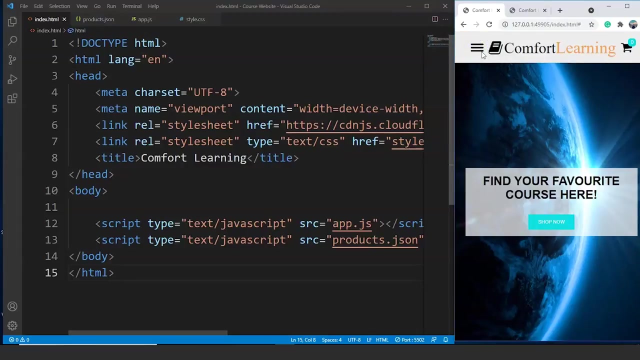 these small things take a lot of precise coding and attention to work smoothly. so let me show you guys one more thing before we move on to the coding part. if we reduce the size of a web page, or we can say, if we remove the size of a browser, you can see the size of website also changes. 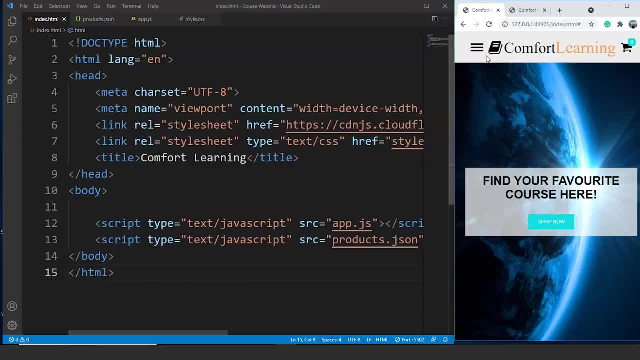 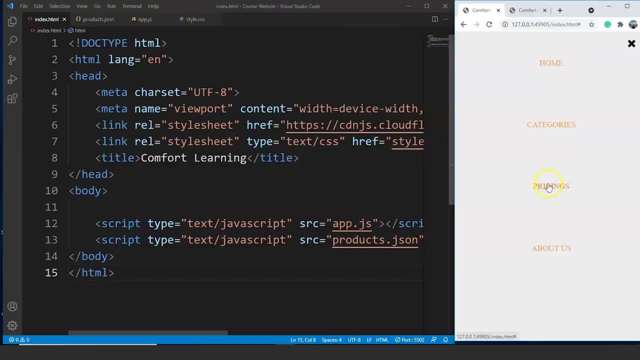 if we make the browser similar to a phone, you can see we have got a menu type of thing over here and if we click on this we are getting the options here. we have home categories, pricing and about us, right. so these were the options present in the navigation bar. we 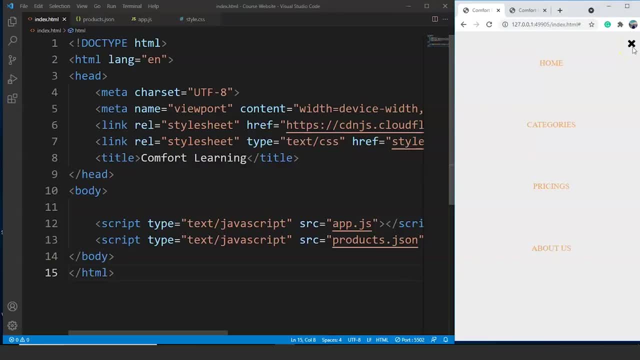 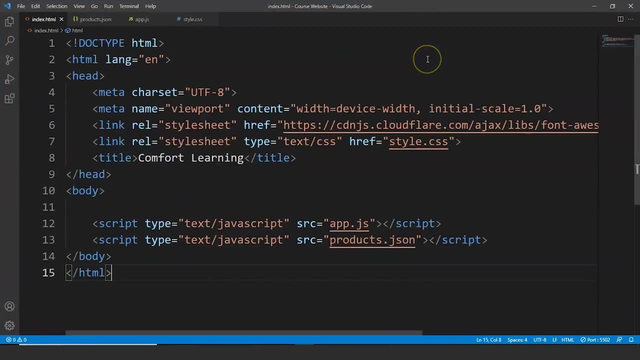 can get them inside a particular menu using css. we'll see how it actually works. so a website is responsive, right, we'll do it with the help of css. so let's move on to the programming part now. so here we are. in the vst code, we have all the images already present inside the images folder in our system. 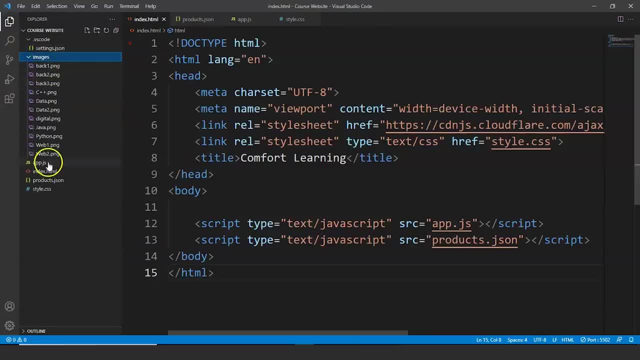 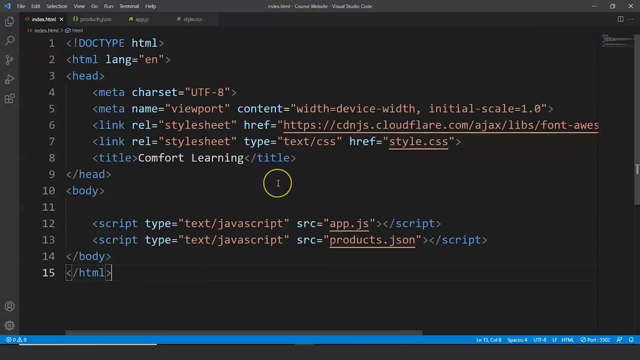 so if you want to see, you can see here. we have all the images present over here and we have four different files. we have appjs, we have indexhtml productsjson to add products and we have stylecss to style all the elements. fine, here we are in the html file. some of you guys 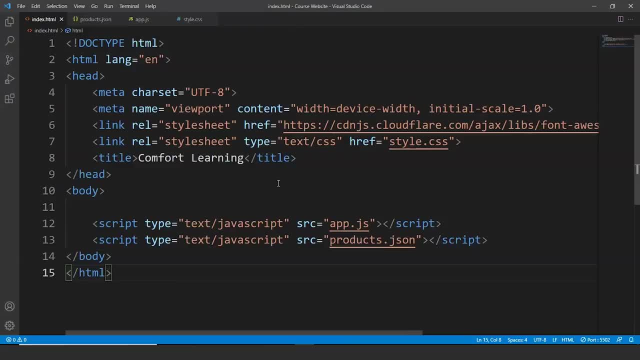 may think that html, css and javascript were fine, but what's up with the json thing? we haven't heard of it in the previous videos. so let me tell you guys. json stands for javascript object notation. just like we create objects in javascript, json is also used to create. 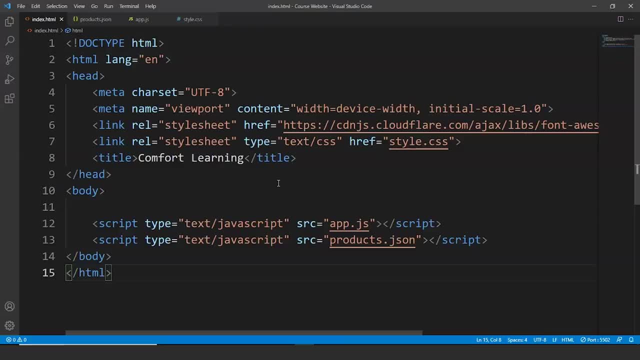 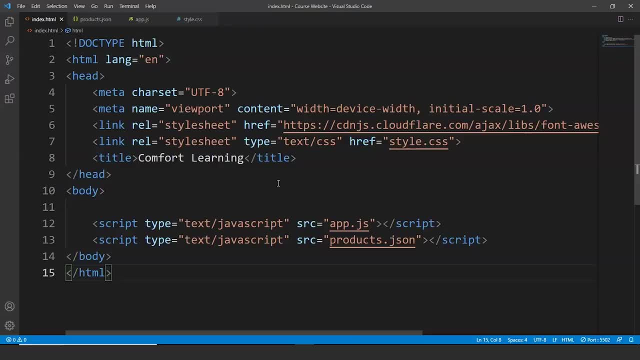 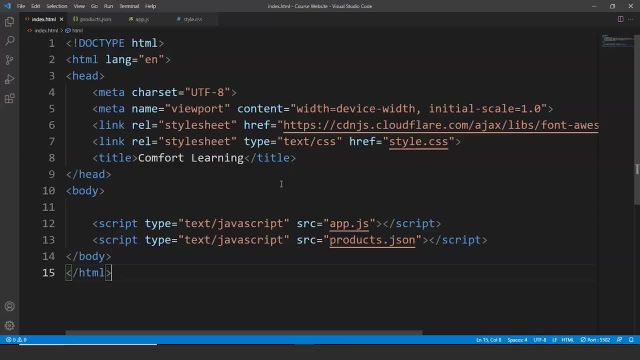 use them when added to cart. so you will get to know more about it while working on it. basically, so for now, if you know enough about javascript objects, then json will be easy for you guys, because the syntax remains almost similar in both the cases, that is, in javascript. 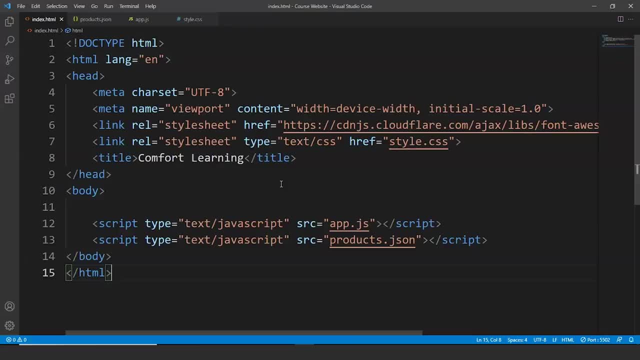 and in json. so let's start writing the code now. here we are in our html file and we have already linked all the files over here. you can see here we have used font awesome library for icons we'll use on our website. you have seen that book icon we have used in our logo. 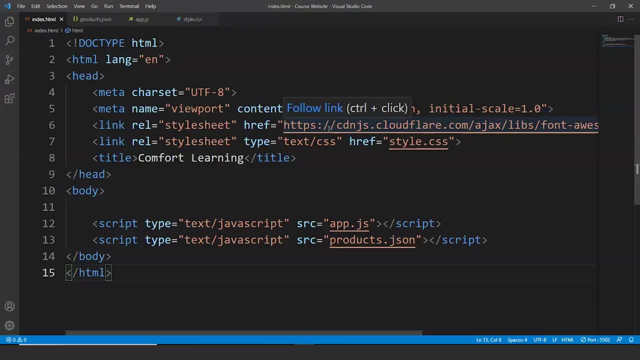 part, and several other icons like the cart icon, etc. so we'll include those predefined icons in our html file using this particular library. to include this specific library, you don't have to do much of a task: go to google, search: cdnjscom, slash libraries slash. 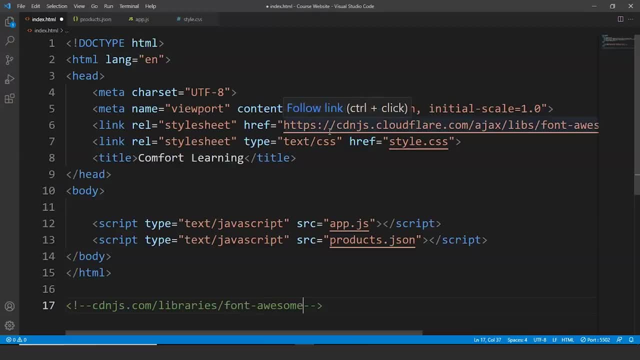 font awesome. go to google and search for this and then select version 4.7.0 under the version option, copy the third url with mincss as extension and paste it into your html file. as simple as that. i'll let you know about the classes we'll use while working on the. 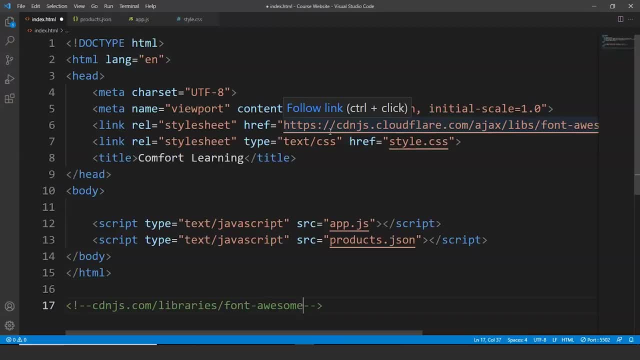 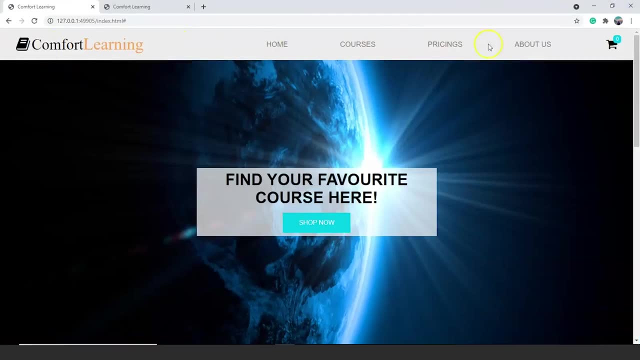 website. we'll get back to the tutorial as soon as possible. so now let's get back to the website. now let's start with the programming part. the first thing we have on our website is the navigation bar. right, let me show it to you again. so here you can see we have a navigation bar. will first work on this one, only so. 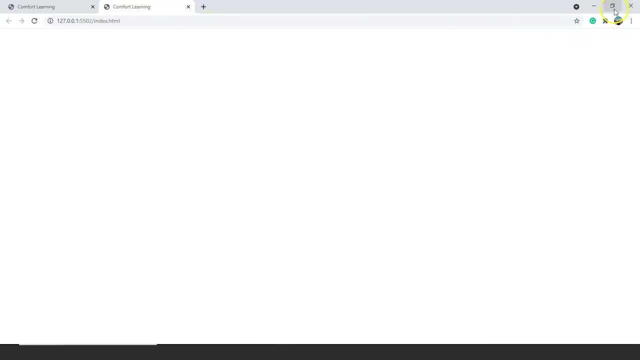 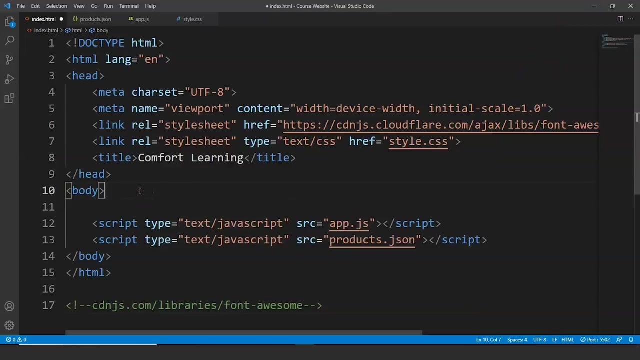 let's start writing the code. so this is the output of a current website. so what we'll do is we'll minimize the browser and we'll start writing the code here only. so what will do is will write here: nav class is equals to nav bar. then 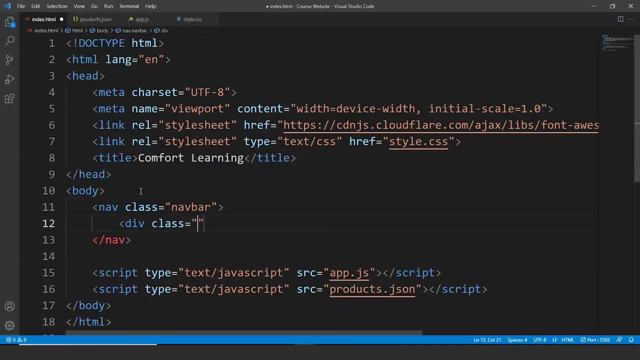 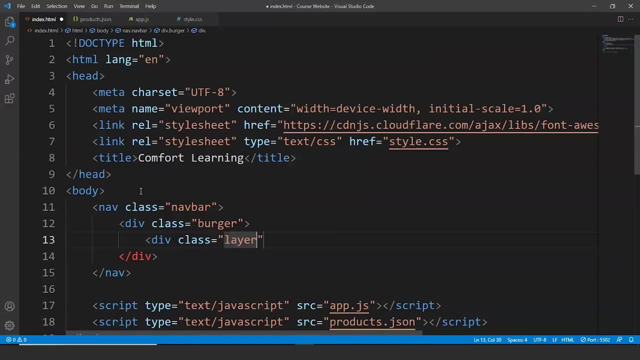 inside this will write div class is equals to burger and inside this will write three div tags will write a div class is equal to layer one. We'll close this div, we'll copy it from here and we'll paste it again three times. Fine, We'll write here: layer two and layer three is class. then, after this particular, 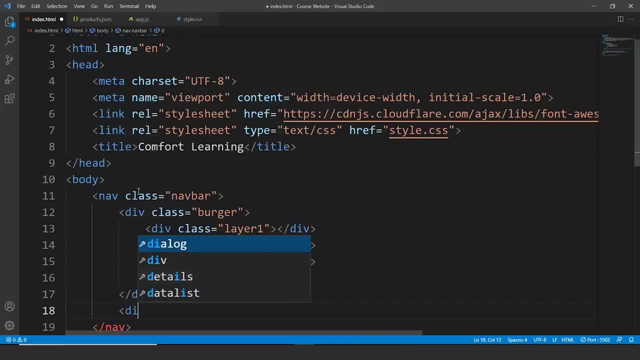 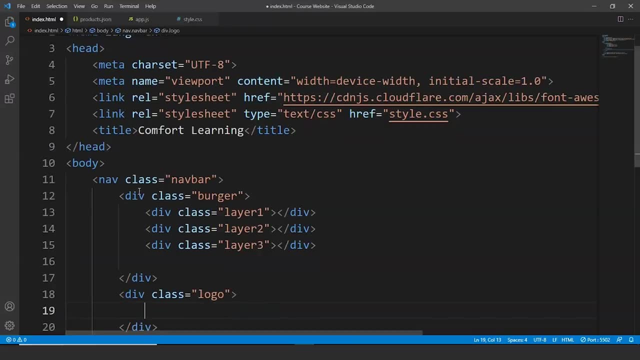 div tag. we'll add another div tag with class as logo. Then inside this we'll use the span tag. we'll write here: span class is equals to logo- logo text. and then we'll write here: I will use the I tag to make it a little bit italic, So we'll use the class as far far. 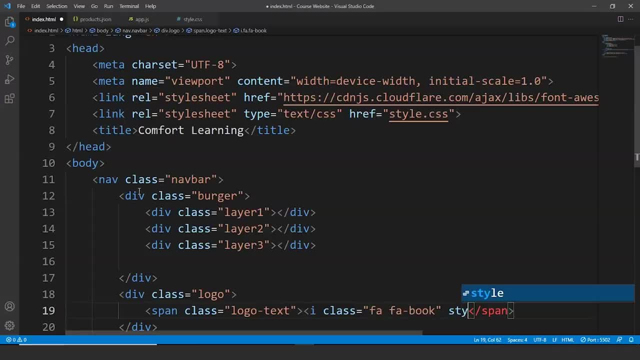 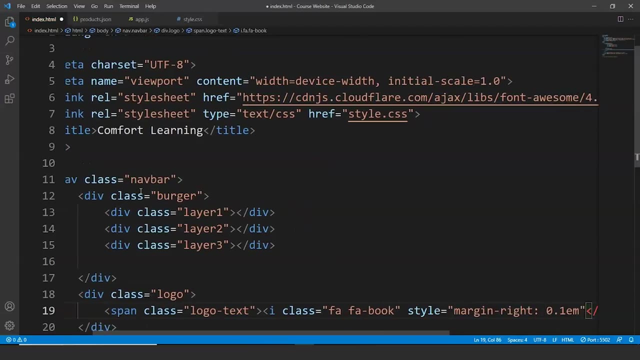 book: Fine, We'll write here: style Is equals to margin Margin right. We'll write here: margin right as 0.1 m. Then we'll write here: Similarly: we can close this. Fine, Now we have added the book icon to our website. 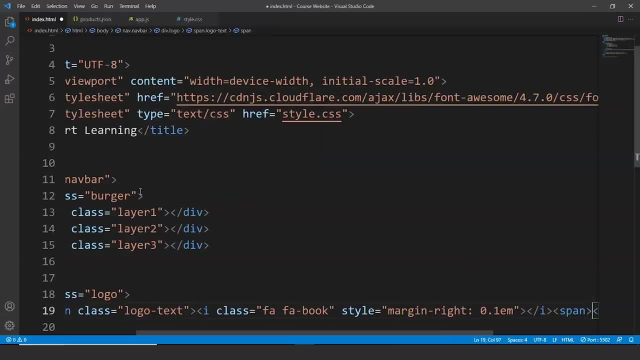 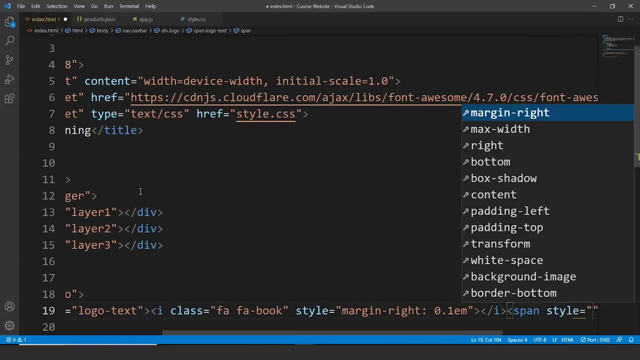 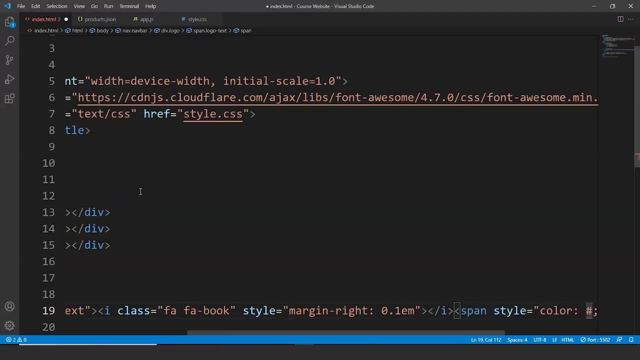 Then what we'll do is we'll write here again span, We'll use the span tag. within this span tag, We'll write here: Style is equals to color and the color code is hash. F zero, nine, five, D, one. So these are the color codes for this particular website. We'll use them. We have written here: F zero. 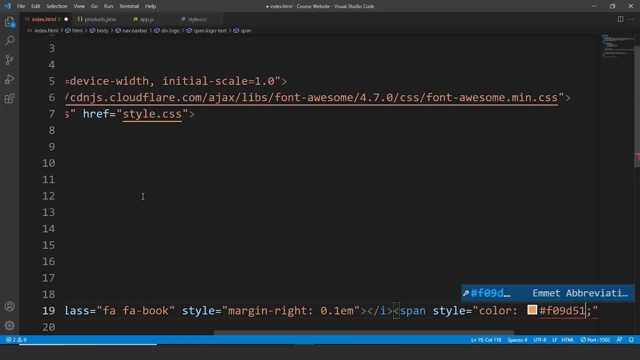 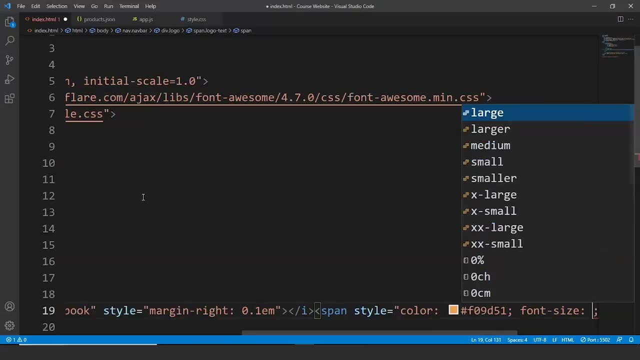 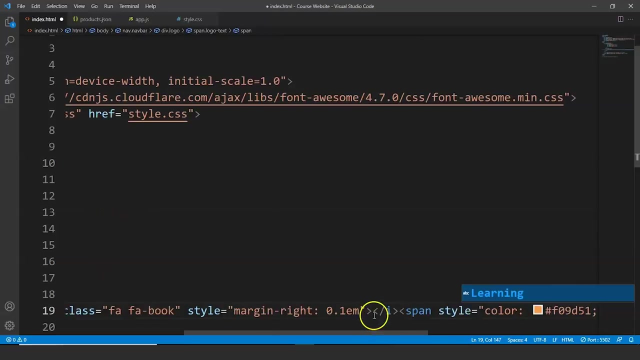 nine D, five, one. Fine, Then what we'll do is we'll write here: Font size is 1.1 m and what we'll do next is we'll write here: Before the span tag closes. we'll write here: Learning, Fine. So what we did wrong here is: we forgot to mention comfort here. 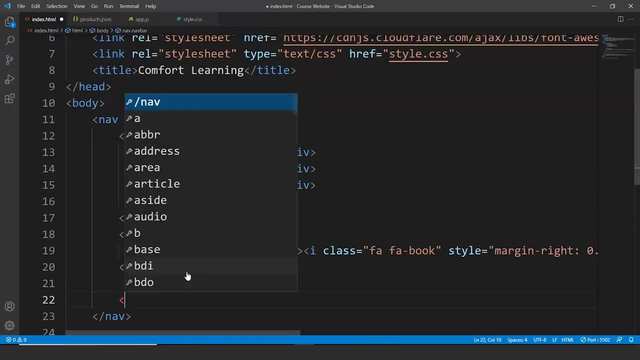 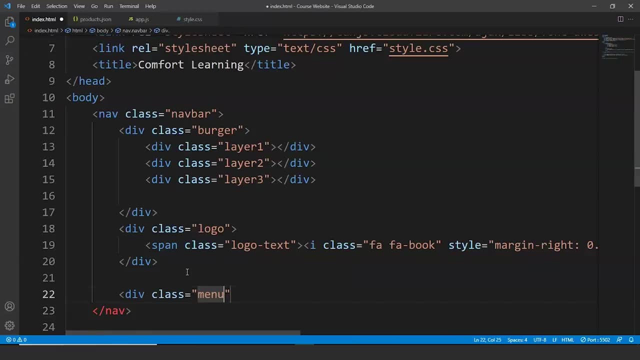 Now we are done with the logo part. Next up, what we'll do is we'll write here: div. class is equals to logo. class is equals to menu bar. we are working on the menu bar for the hamburger menu, so what we'll do is we'll write here ul, so ul stand for unordered list. we'll write here: class is list and inside. 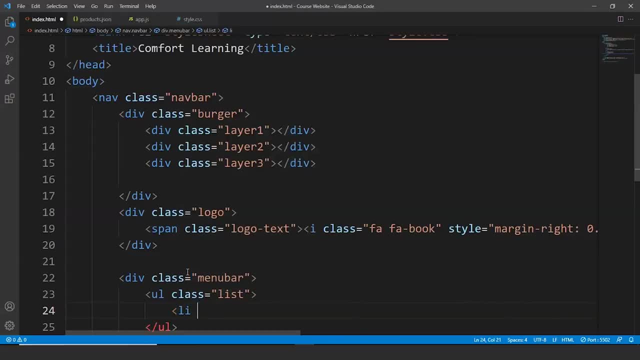 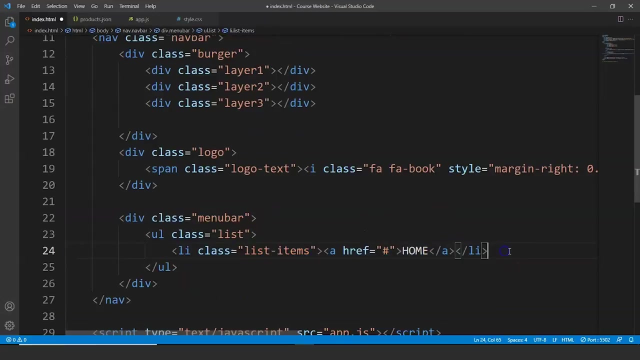 this. we'll use li tag, so we'll write here class as, let's say, list items. we'll write here: a href is equals to hash and here what we'll do is we'll write here home. fine, we'll copy this piece of code. we'll paste it again three or four times. we have 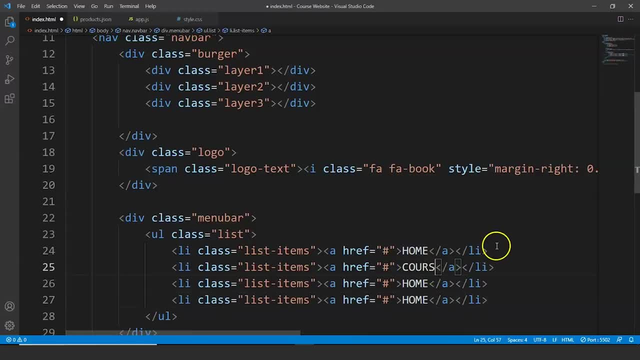 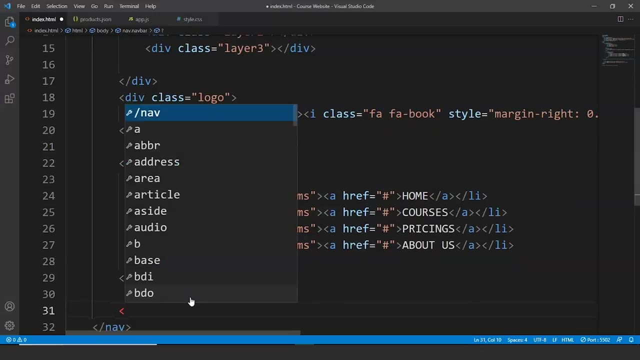 four different options. we have home, we have courses, and then we have pricings and finally we have about us. fine, so we are done with menu as well. next up, what we'll do is we'll write the code for cart now. so we'll write here: div class is equals to cart and inside. 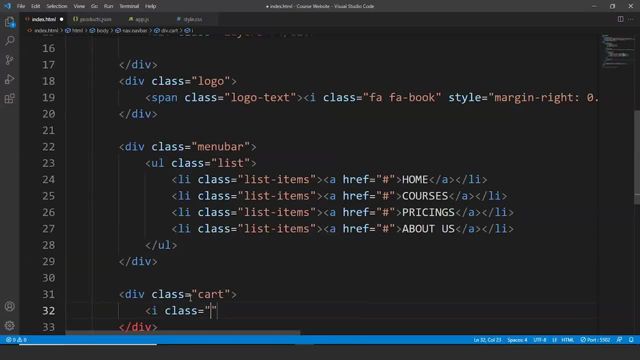 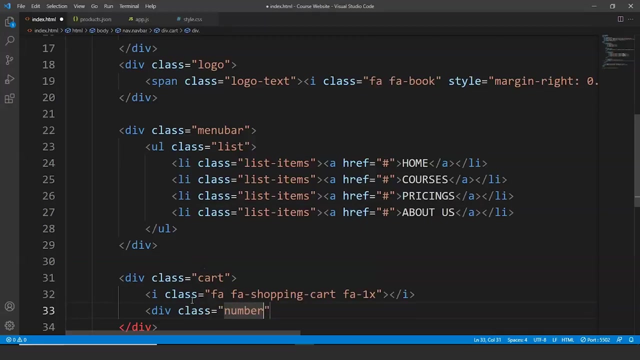 this we'll write: i class is equals to cart. we'll write div class is equals to cart, and inside this we'll write: div class is equals to shop cart for 1x. so here we have used this special class to include the cart icon to a webpage. now next up, what we'll do is we'll write here: div class is equals to number of. 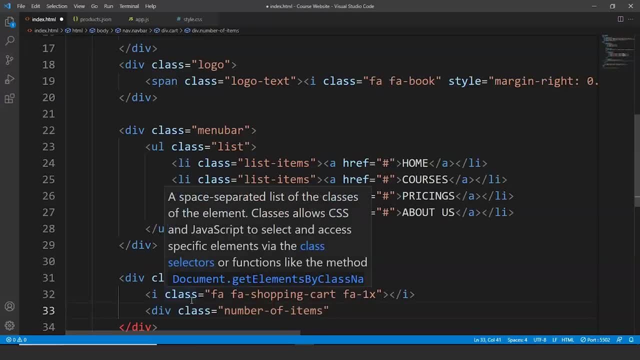 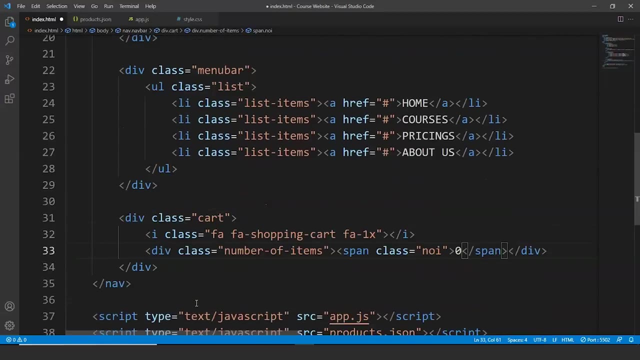 items, and then we'll write here: span class is equals to, lets say, or whatever you want to, let's say, noe. Now what we'll do is we'll write here: zero inside this. Fine, I hope you guys understood what we did till now. We are working on the navigation bar only. 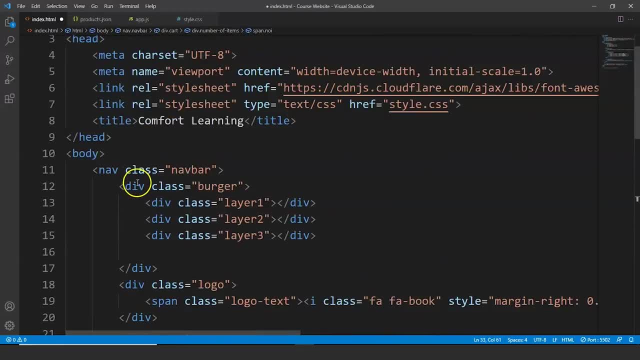 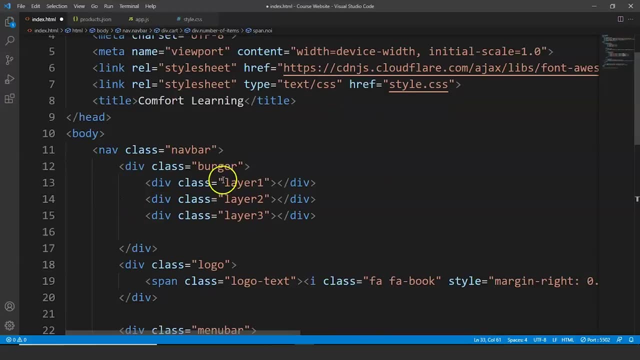 We have created the navigation bar. So this is the code: Firstly, we have used a class navbar for this particular navigation bar. Then we have used the div tag for burger menu. We have three different layers: layer one, layer two and layer three. So this is actually. 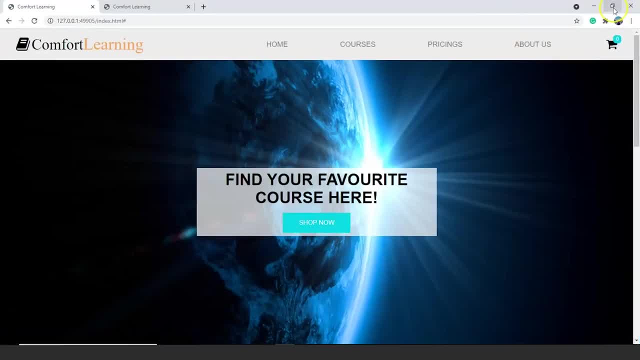 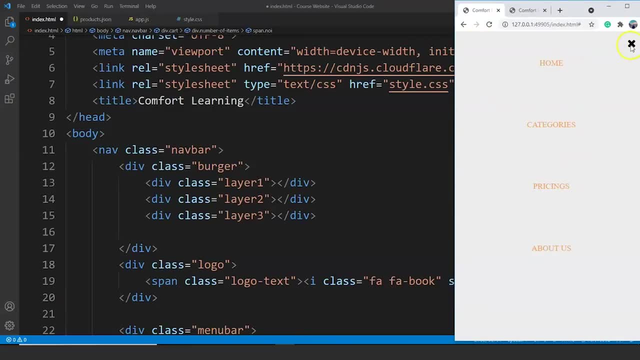 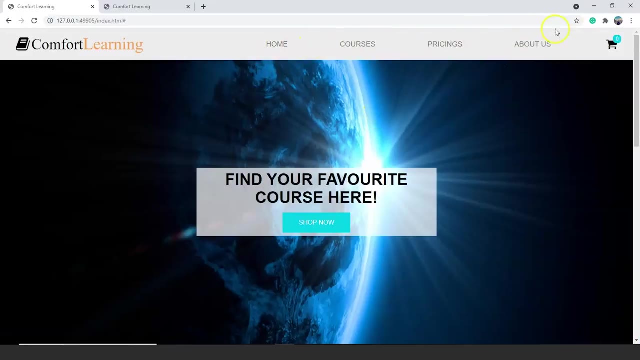 the icon of burger menu You can see here if we reduce the size of our website. So we have defined this burger menu and inside this we have four other options which we defined later here inside the menu bar. And we have four options. We have home courses pricings. 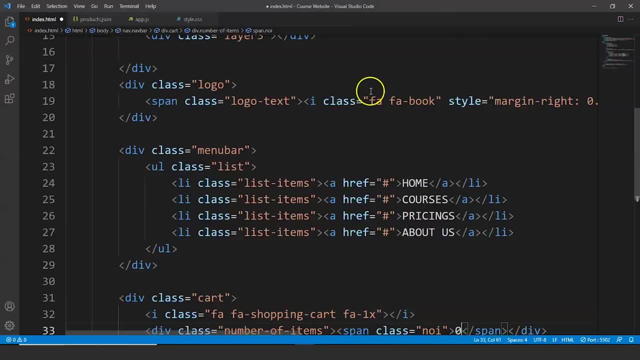 and about us. So we are doing totally right. So till now, we did some basic tasks here. We have added all the navigation bar elements and the next thing we have to do is to style our navigation bar. And we will be adding all the navigation bar elements and the next thing we have to 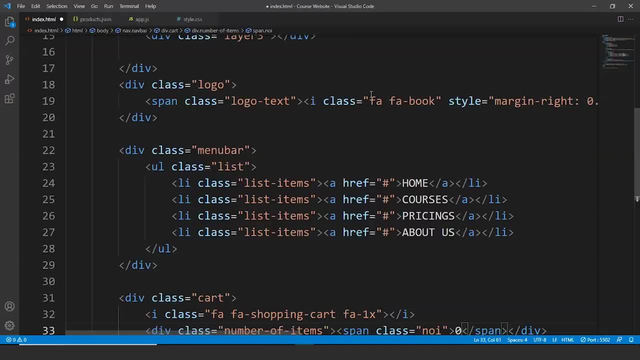 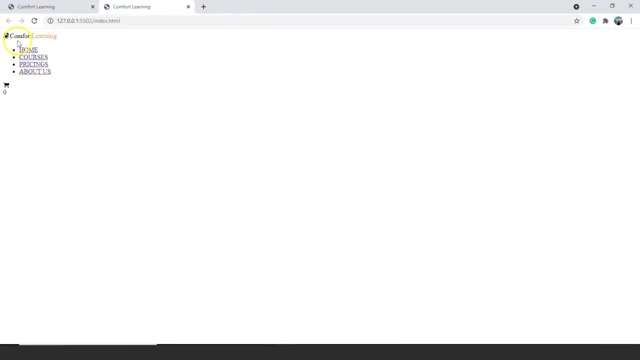 bar. according to the final website, it's pretty simple. let's do one thing, let's save it once and check the output now let's see if it's working. so it's totally working. we have a book icon over here, we have comfort learning written over here, we have cart icon over here and we have zero written over here. fine, 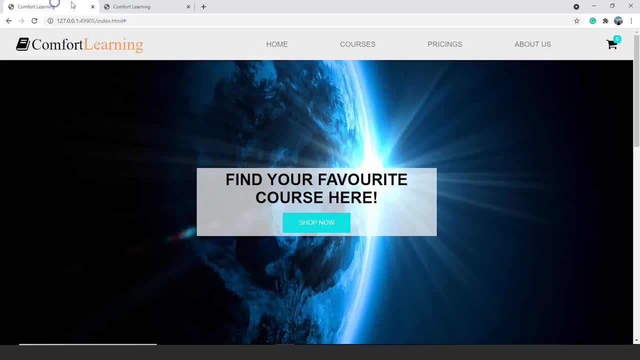 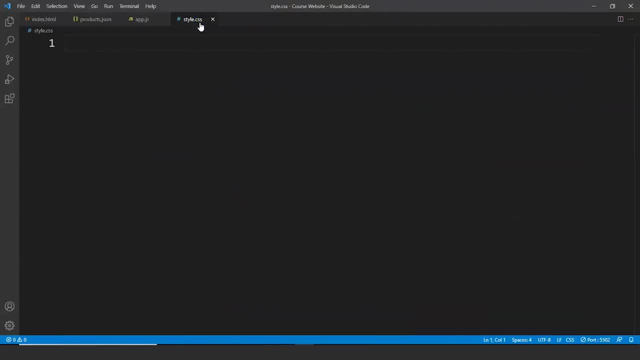 now we have to style those elements accordingly to make it look like this. so we are making this navigation bar. so what we'll do is we'll move to our CSS file and we'll start styling by doing some default style changes to the entire HTML document. we'll write here: star. 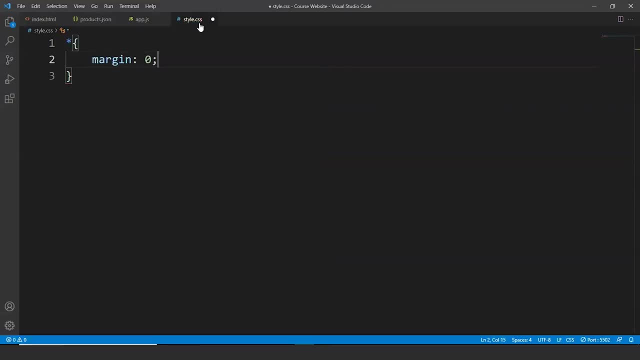 margin will be zero. the default margin will be zero. padding will be zero. then we have box sizing. we'll write here: border box and font size will be twenty pixels for default. fine. next up, we'll write here: HTML will now style. HTML document will write here: scroll behavior is smooth and will write here: 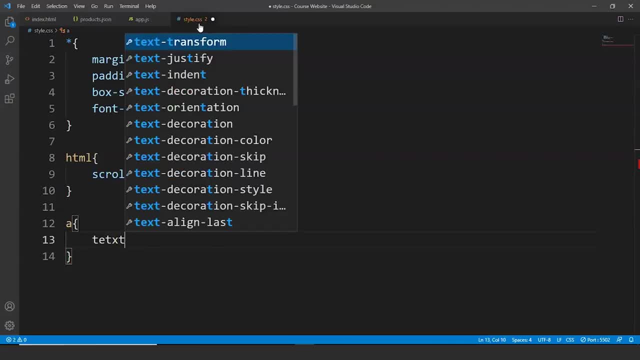 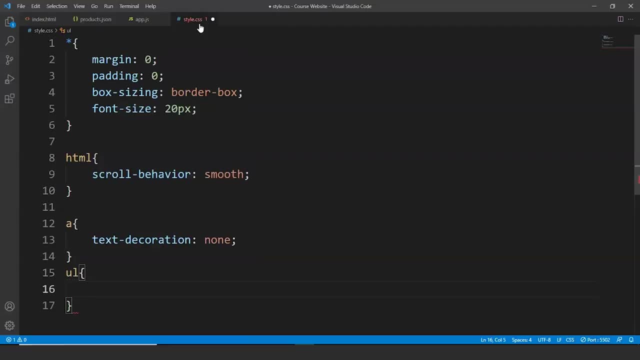 anchor tag will write here text decoration and will write your text decoration is none. and then we'll style the unordered list. we'll write a ul. we'll write here list style as none. fine basic styling is done. let's do some more for the navigation bar as well. 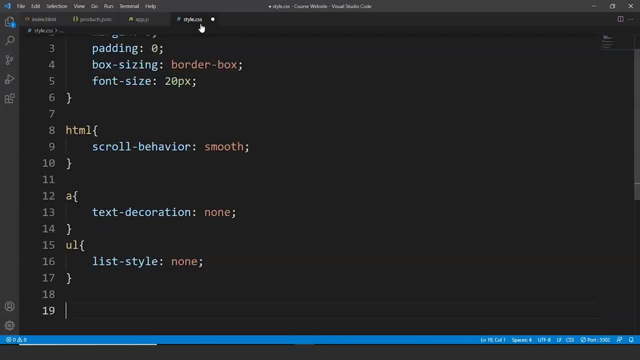 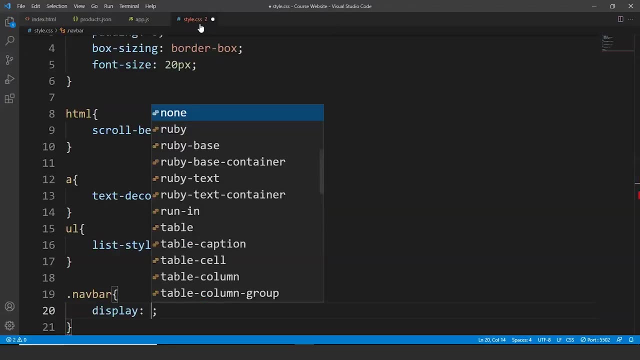 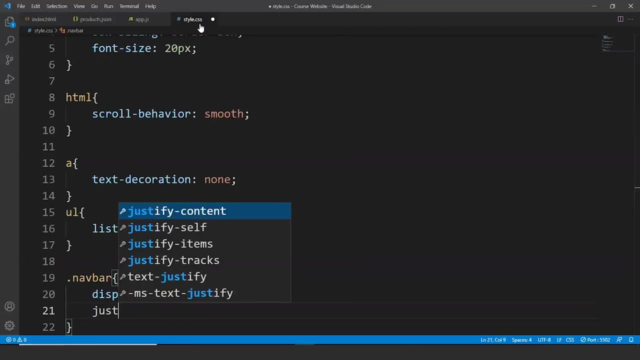 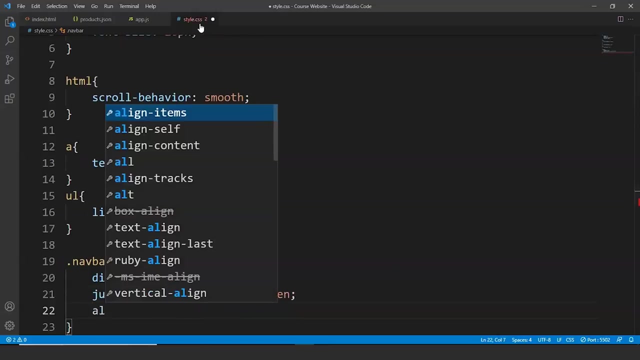 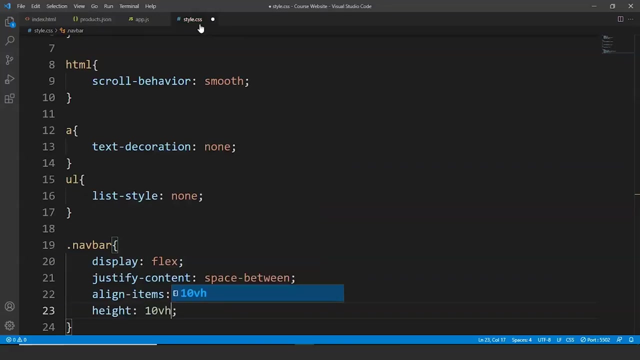 what we'll do is we'll write here: dot nav bar. this is the first class we have used in a html page. we'll write here: display as flex. then we'll write here: justify content as space between. align items as center height as 10 vh. so 10 vh refers to the viewport height. 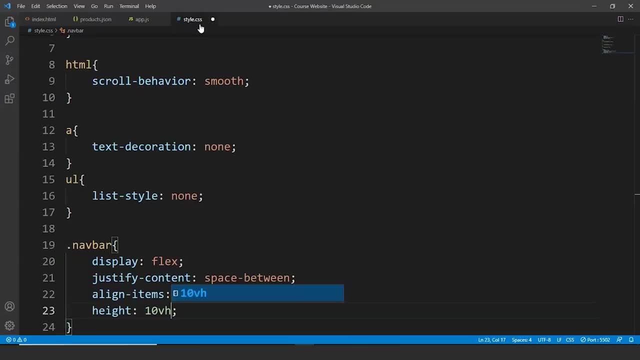 it will take 10 percent of the total height of the screen. then we have background color as hash, ec, ec, ec. so a little bit of gray, grayish, white, we can say. then next thing we'll do is we'll style a logo, we'll write here logo and inside this we'll write 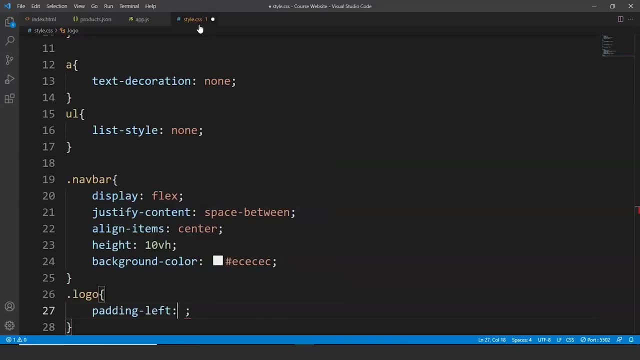 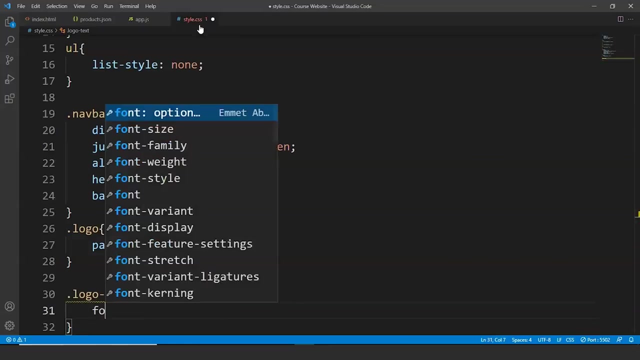 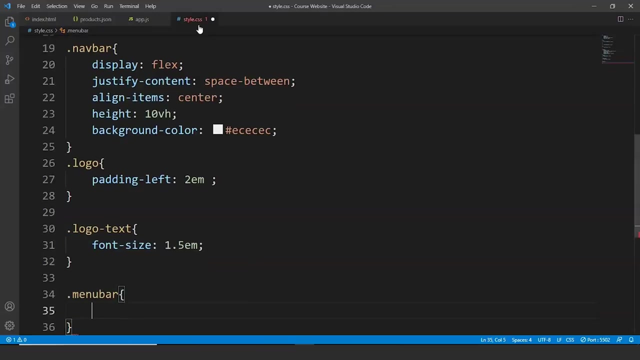 padding. sorry, we'll write here padding left and the padding left will be 2m. next up, we'll write here logo and text. so this is the next class. we'll write here font size as 1.5 m. now the next class we have to use is the menu bar class, so we'll write here width as 45 percent. 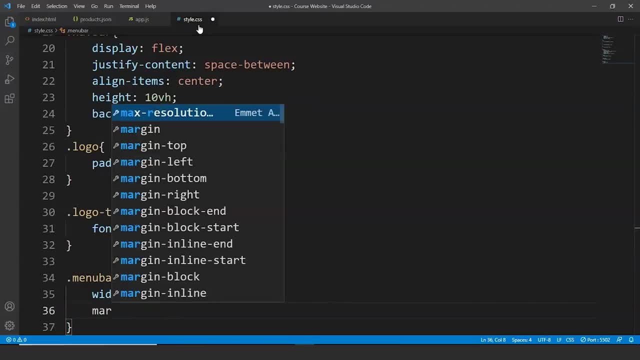 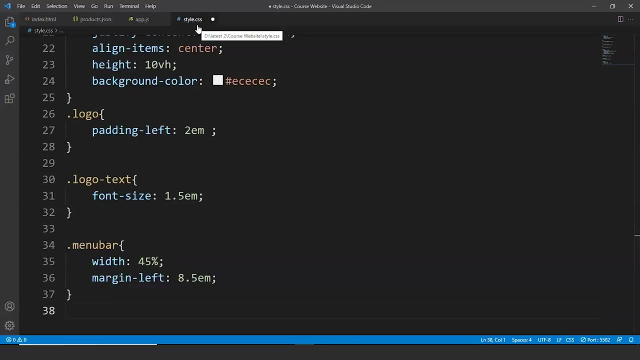 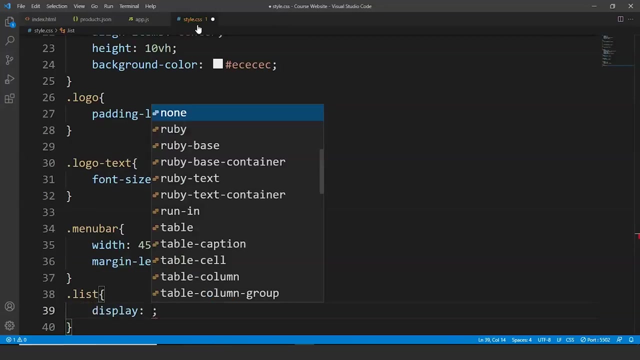 and margin left as 8.5 m. fine, i'll let you know what this m means in a moment. so first we'll do this styling and all next up we'll write here: dot list will access the list and we'll write here inside this display as flex. 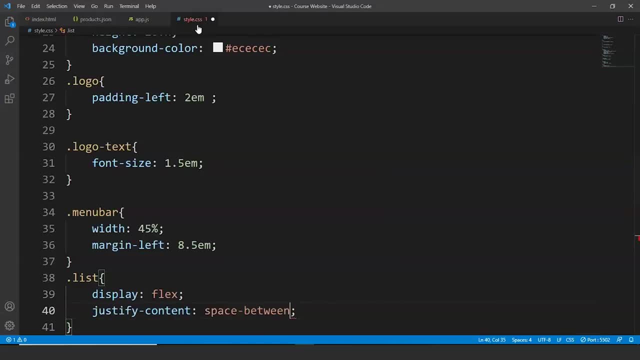 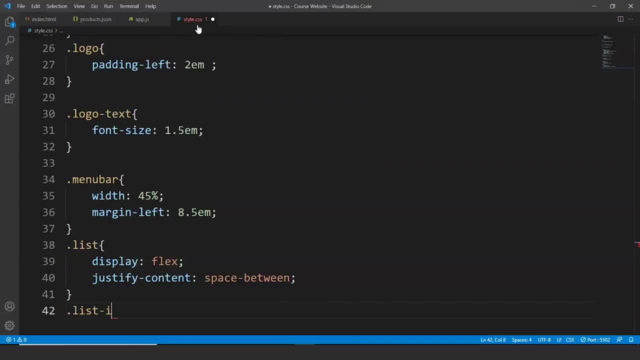 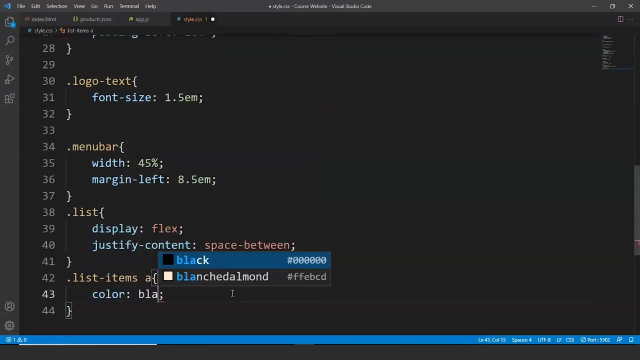 and justify content as space between fine next up. Next up, we have the list items, So we'll write here list items And we'll of course write here A as well. We'll write here color, and the color will be, let's say, black. Next up. 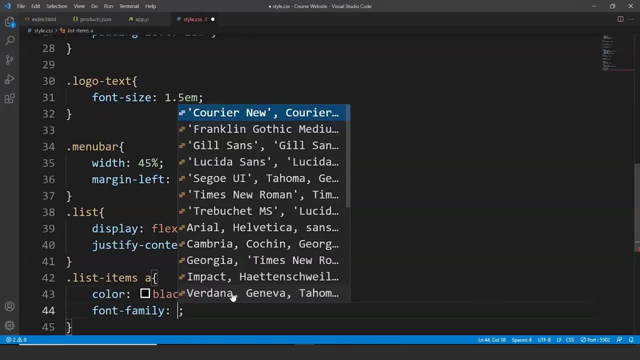 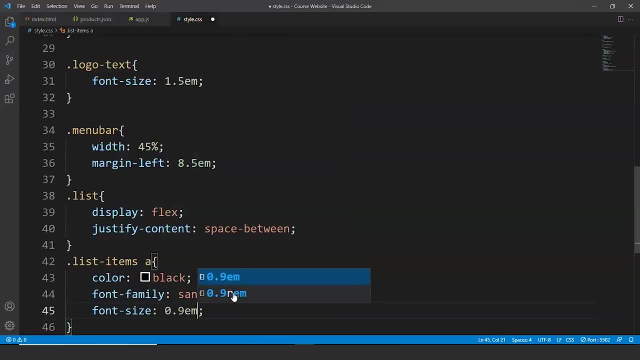 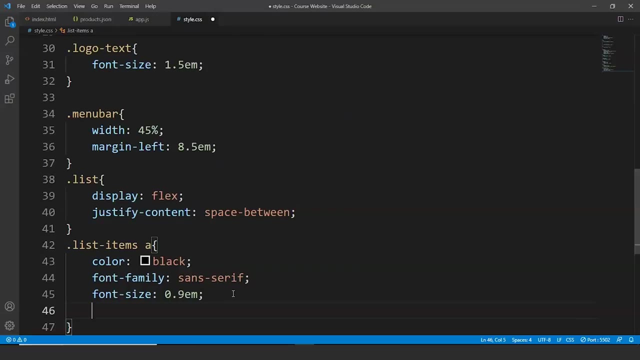 what we'll do is we'll write here: font family is sans serif. font size is 0.9 m, So you must have noticed earlier that the default font size was 20 pixels, So keep that in mind. I'll let you know the use of m in a moment. Next up, we'll write here: transition: 0.4 seconds. 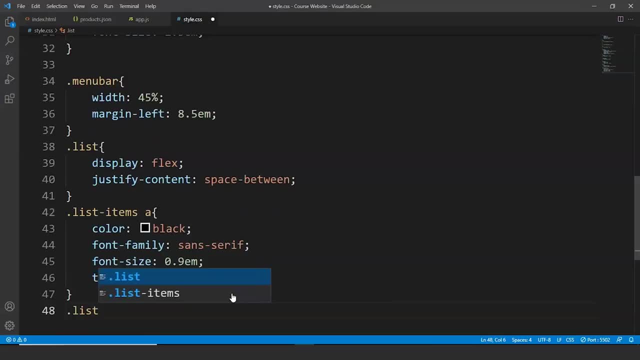 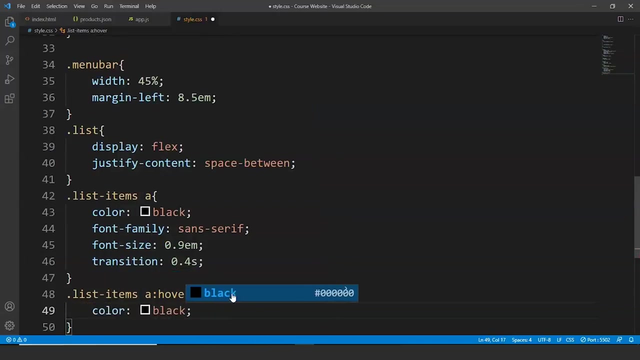 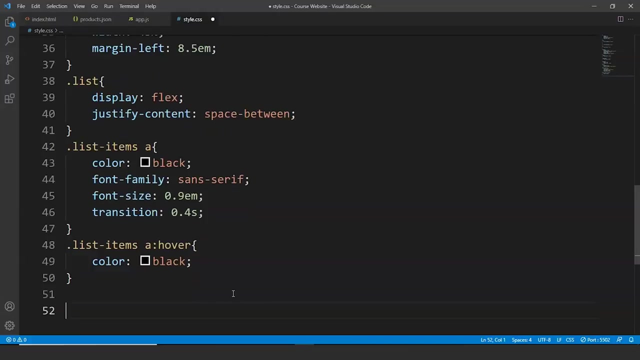 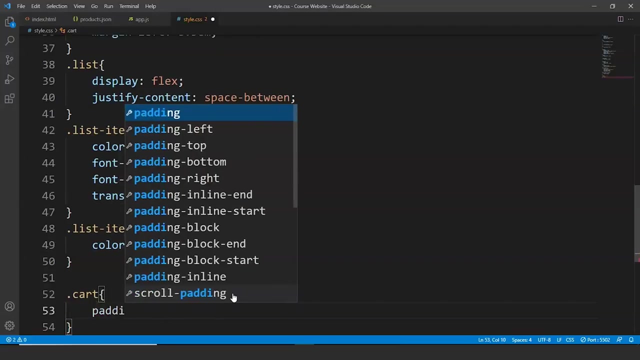 And we are good to go with it. Next up, we'll write here list items And we'll write here: hover Fine. Then we'll write here: color is black. On hovering, the color of the list items will change to black. Now the next thing we'll do is we'll write here: cart Padding right will be 2 m. 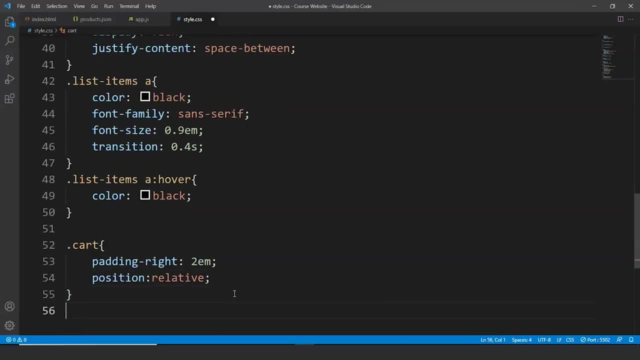 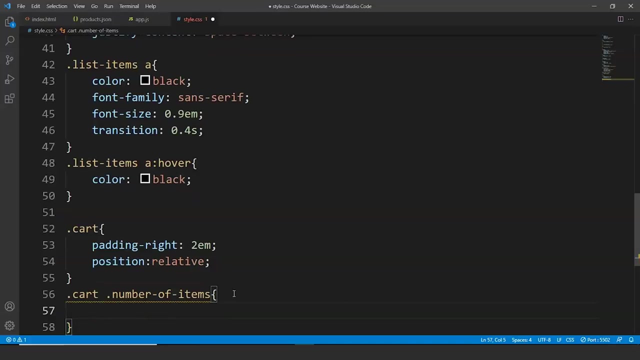 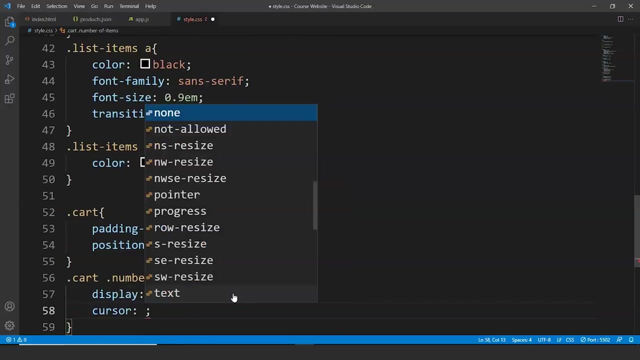 And position will be relative. Fine, We are done with the cart Next up. We'll write here cart number of items. Fine, We'll write here: display is flex, Cursor is pointer. We are using- repeat, We are styling- two different classes here. We are styling. 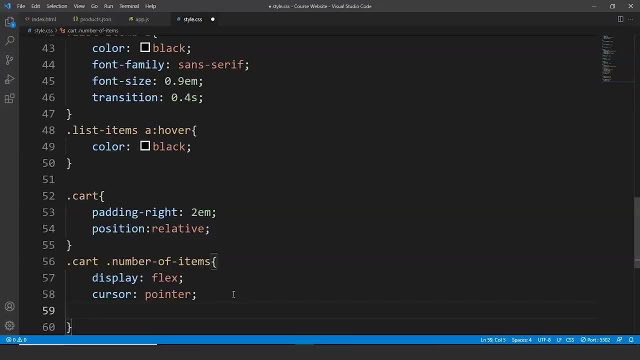 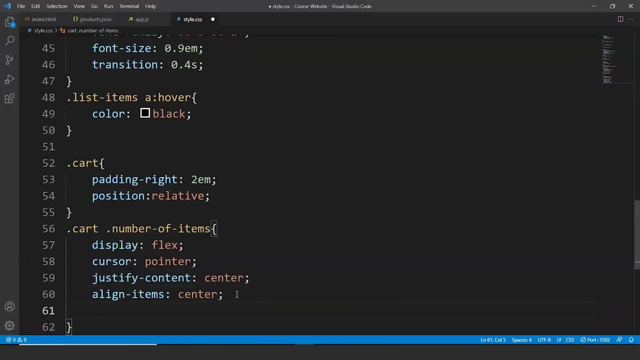 the element with class as cart and the element with class as number of items. So we are done with the Himalayan Fine. We'll write here: justify contents to center, Align items to center. We'll write here: color is white, Position will be absolute. And then we'll write here: left is 18 pixels And we have. 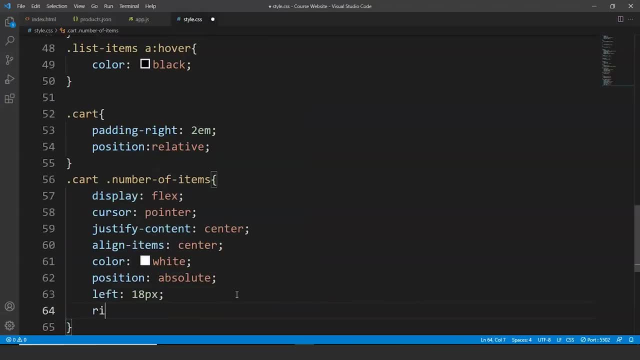 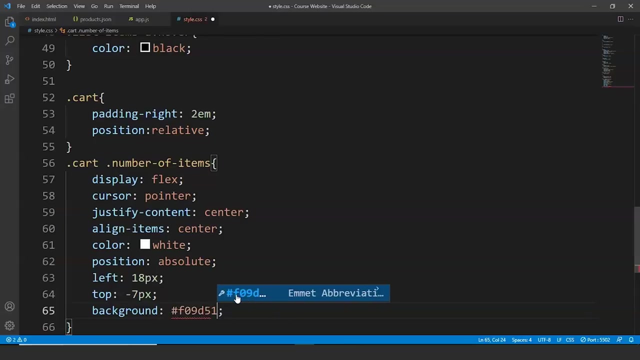 1 месте here: Ok602.. and right as okay. sorry, we'll write here left as 18 pixels and top as minus 7 pixels. next up we'll write background, so the background color will be hash: F, 0, 9, D, 5, 1. so this will be a. the background color will define the height and width. 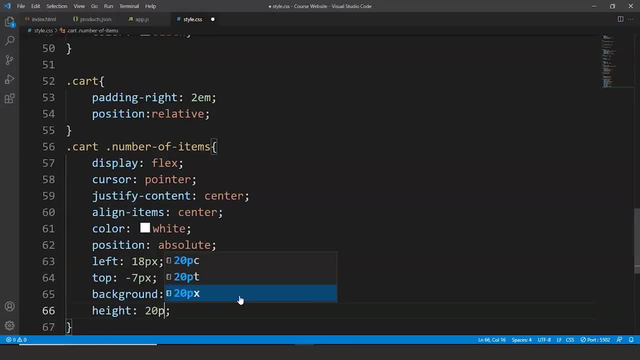 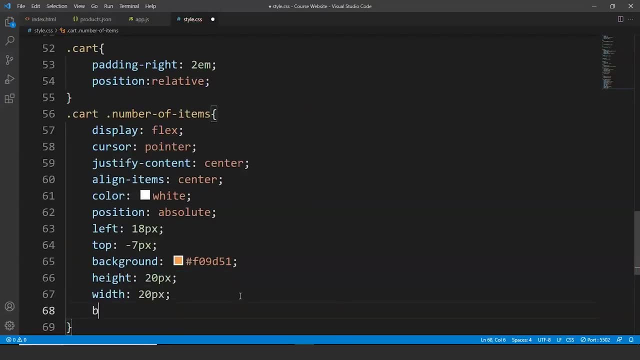 as well. so height will be 20 pixels and the width will also be 20 pixels. fine, the last thing we have to write here is the border radius. so keep one thing in mind, guys, while you are styling all these elements: do check the weapon site after every styling event, because this will let you know what this 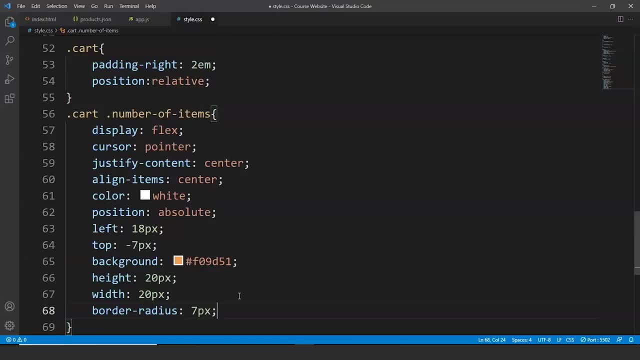 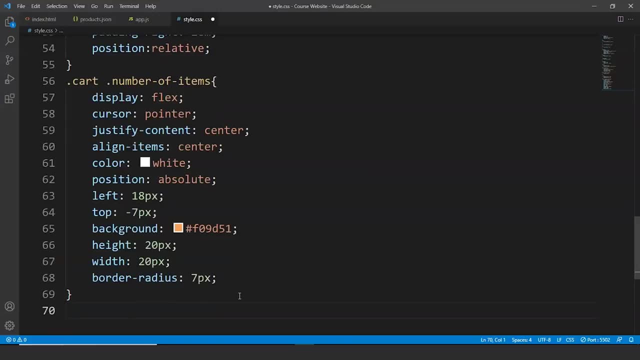 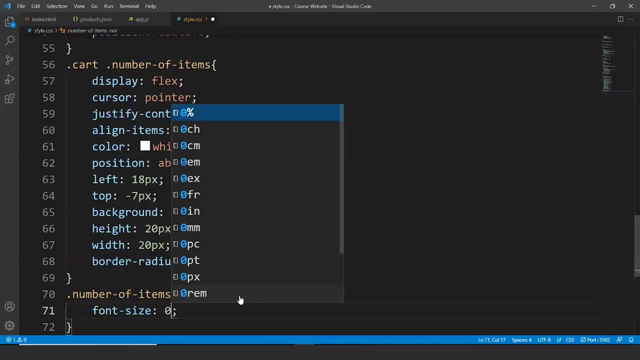 particular event does, or what this particular styling property does to that particular element. so do it when you are writing this code next up. we'll write here: dot. number of items, space dot. knowing so now it was the class we have already declared, we will write here: font size is zero point seven M. 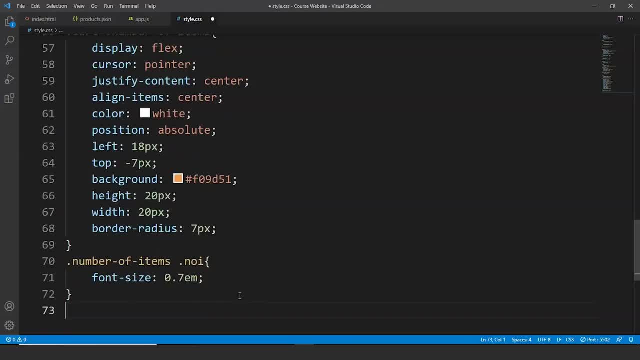 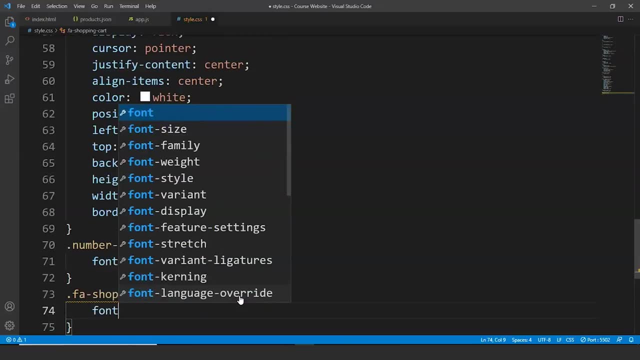 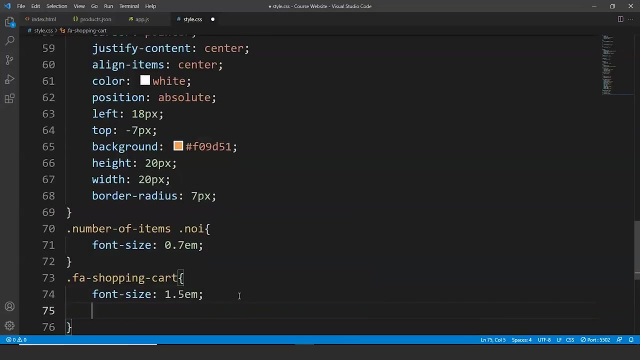 the next class will be styling is the shopping cart, so we'll style this icon as well. we'll write here: font size is one point five M, the font size will be equal to around 30 pixels. then we'll write here: cursor is pointer. then we'll. 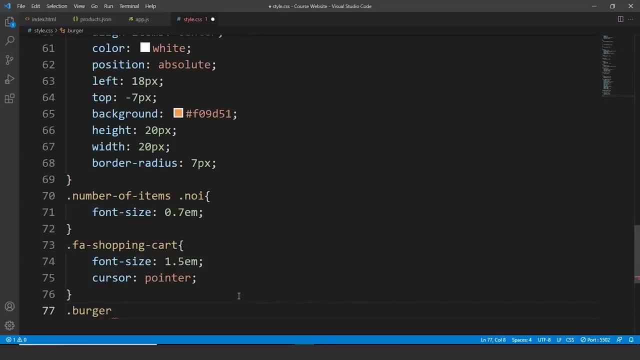 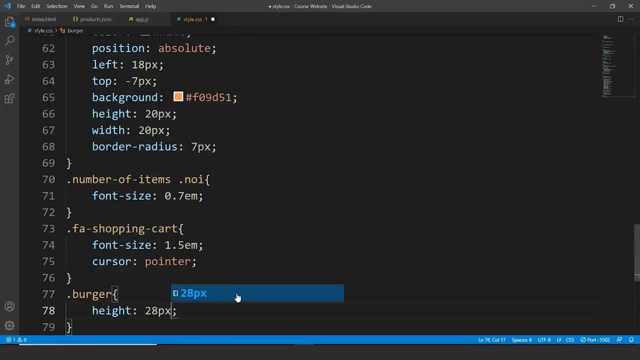 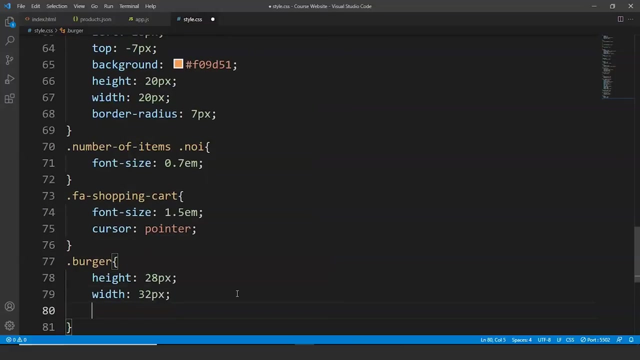 write here: burger will tell the menu as well. we'll write here: height, height will be 28 pixels, width will be 32 pixels. and then we'll write here: display is none. then we'll style the layers as well. we'll write here: dot, layer 1, dot layer 2 and dot. 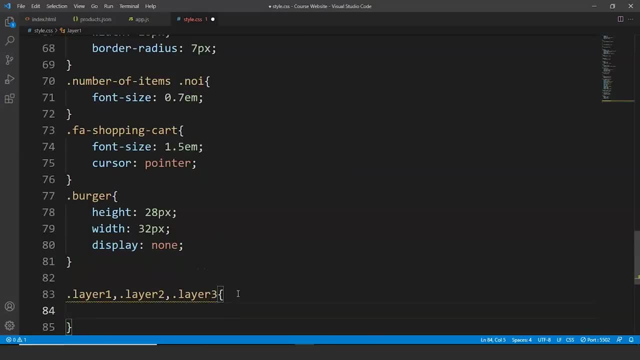 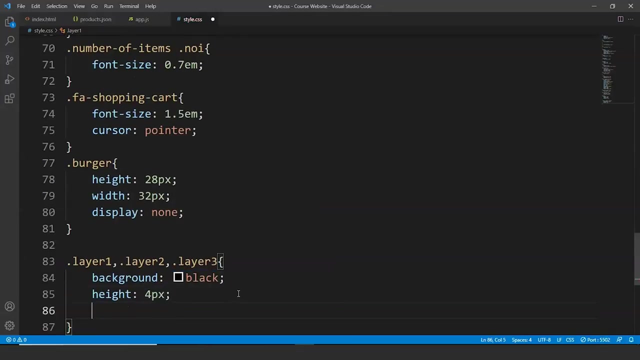 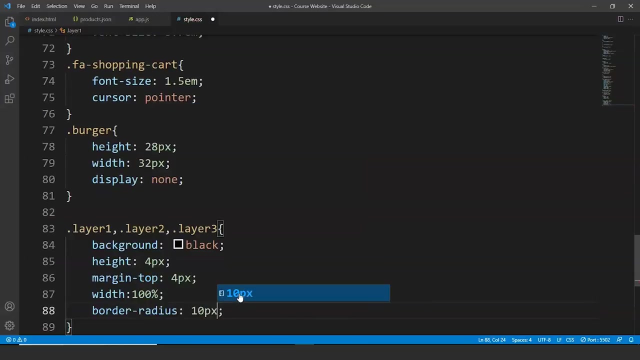 layer 3: now, inside this, we'll write background as black, height as 4 pixel, margin, top is 4 pixel width as 100% and will write here border radius as 10 pixels. fine, you have seen that hamburger menu. you have seen that icon. we were styling that till now. now you. 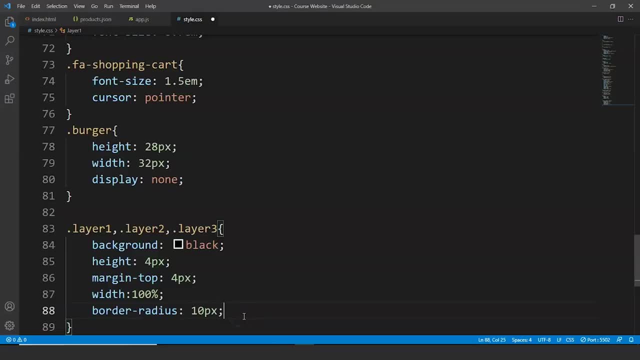 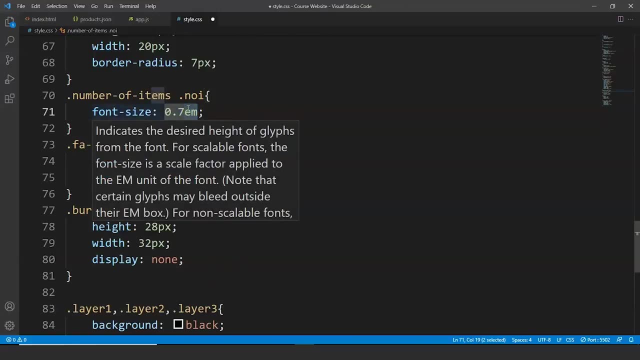 might have noticed here that we have used M here in the CSS file, so I'm talking about this particular M, or we can say E M as well. until now we were using rem or pixel to define the size of the file. I hope I was able to help you out with this video. If you like this video, please subscribe to my channel and give it a big thumbs up. Thank You for watching. 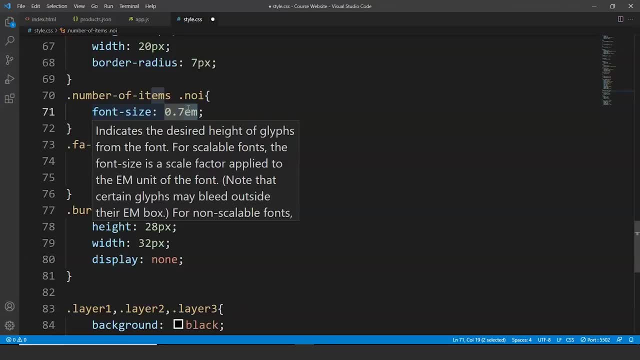 anything while studying, but today we are using M because M uses the font size. for example, if the font size is 30 for the parent class, in this case the font size is 20, the default font size is 20 and the padding is defined as 2M, then the 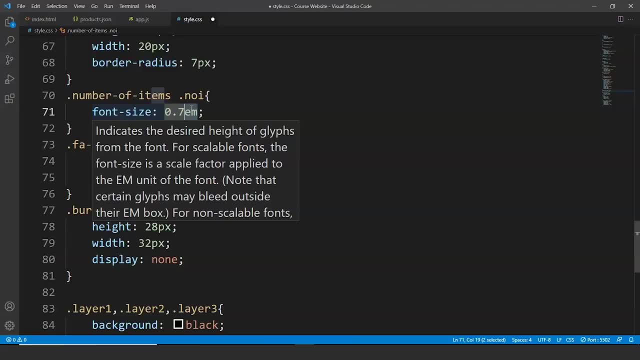 padding will be 40. in that case it uses the font size to determine the size of the property. that's why we are using M, and if you try it yourself you will get to know better. so just try using M. and you can also use RAM or pixel in this. 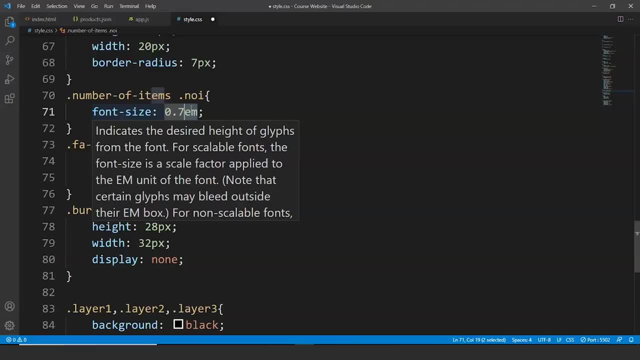 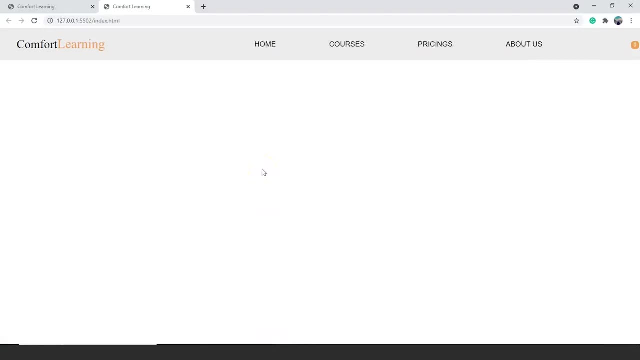 case, but for now we'll use M, so this might be a little bit new for you guys, but try it and you will understand it much better. now save the CSS file, move back to the browser and you can see here that we have a navigation bar ready. 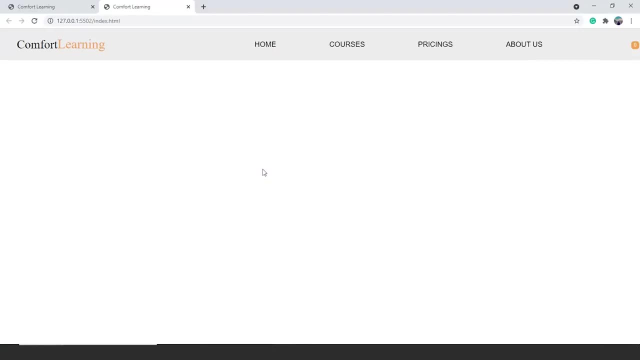 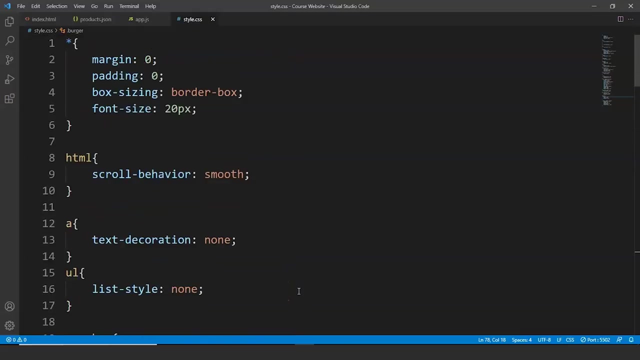 right, it's looking fine, although the icons are not visible. the book icon and the cart icon is not visible, so you can see that the navigation bar is not visible. so let's go back and see what's wrong in this CSS file. what we'll do is: 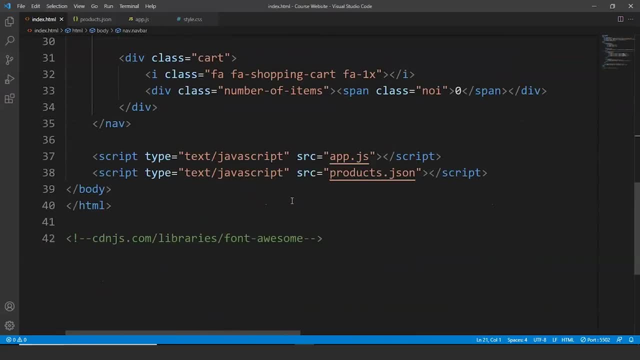 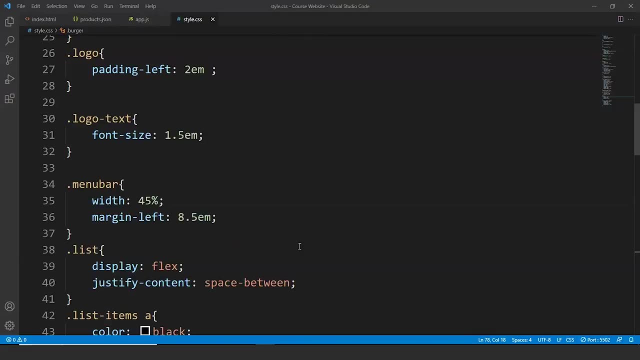 we'll move to HTML file and we'll see if something is wrong here or not. so nothing is wrong in this case. the error is because we are not connected to internet. so if this error continues, just try to connect your laptop or your PC to the internet and the icons thing will work fine. so you can see, here we have our 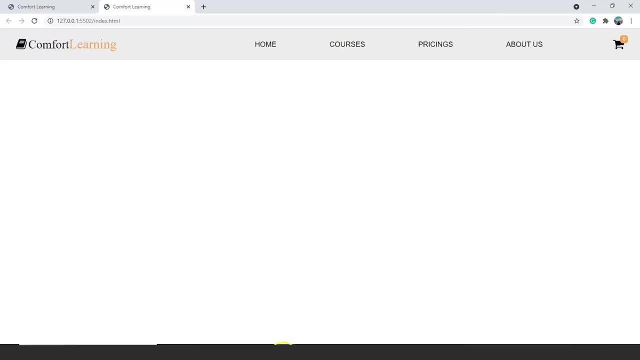 icons. over here, we have our icons. over here, we have our icons. over here. we have the book icon, we have the cart icon, and what we have to do is we have to increase the size of this logo and text a little bit right. so here you can see. 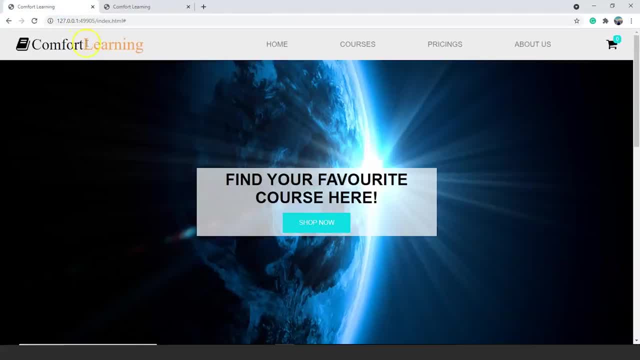 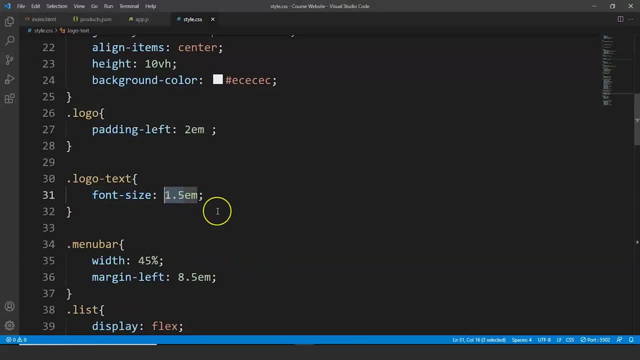 the comfort learning is a little bit small when compared to this particular website. so what we'll do is we'll move to a CSS file and we'll write here: instead of 1.5 RAM, we'll write here 2M, fine, save it and here you can see it's. 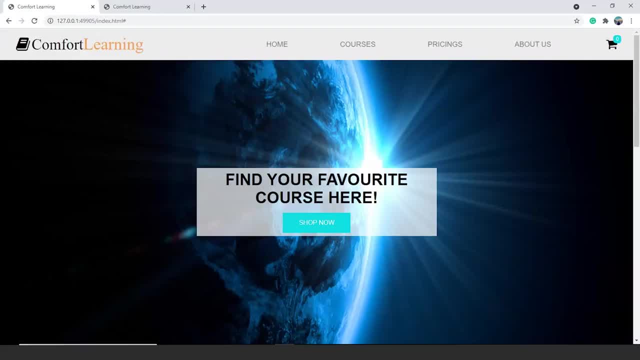 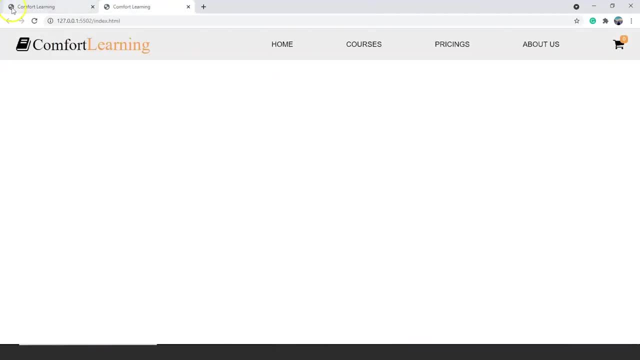 looking fine. now, The difference is because of this scroll bar. we don't have this scroll bar in our website until now, So this is why it looks a little bit different to you guys. It's working totally fine other than that, So let's move on to the next part. 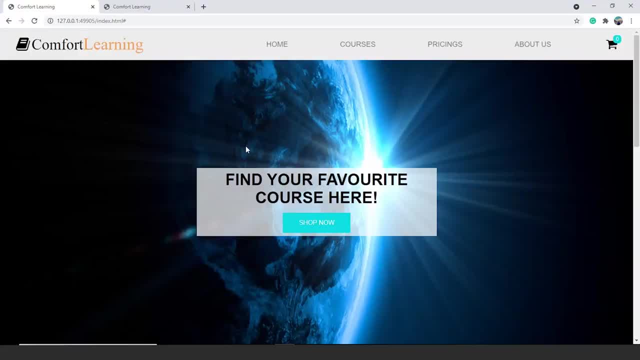 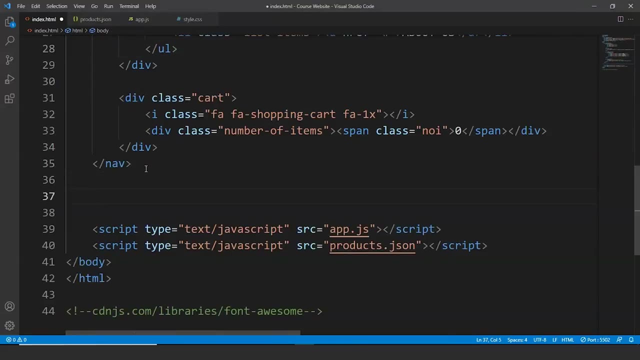 And the next part of our website is the background image with the card present on it, right, So let's write the code for this section as well. What we'll do is we'll move to our HTML file And right here we'll write: section class is equals to section one. 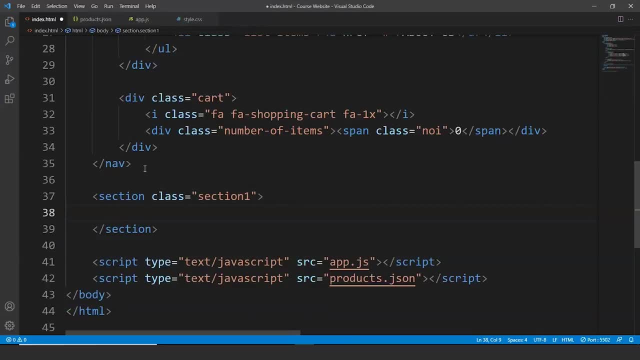 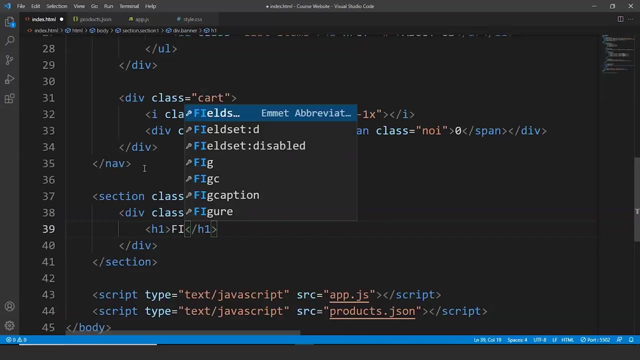 So we are using the section tag to define a particular section in the web page. Now we'll write here: div class is equals to banner. And here we'll write inside h1 tag: find your favorite courses or course here. Then inside this, what we'll do is we'll write here: 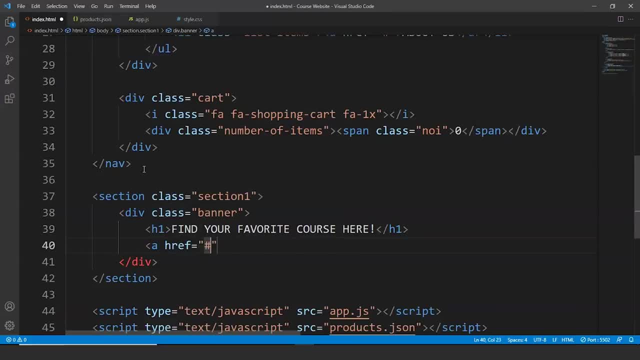 href is equals- Okay, It's equals to products, So the product file will be using JSON for this, So leave it for now. We'll write here: shop now. So shop now is actually not a button. What we'll do is we'll use a link and we'll define it later. 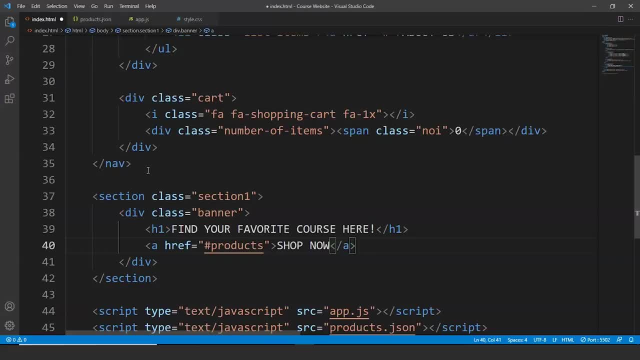 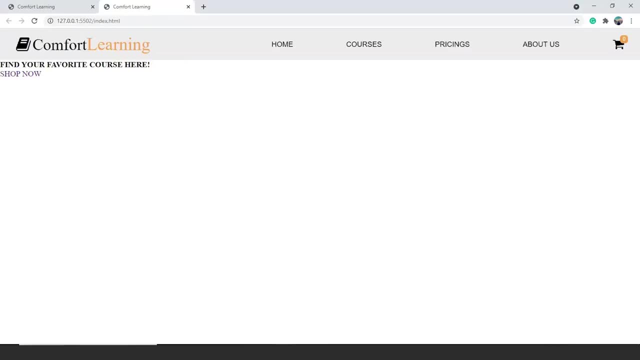 So let's save it and move to the browser. Open this website and you can see here. it says find your favorite course here and it says shop now. It's not inside the banner Because we need to style this particular section to make it look like a website. 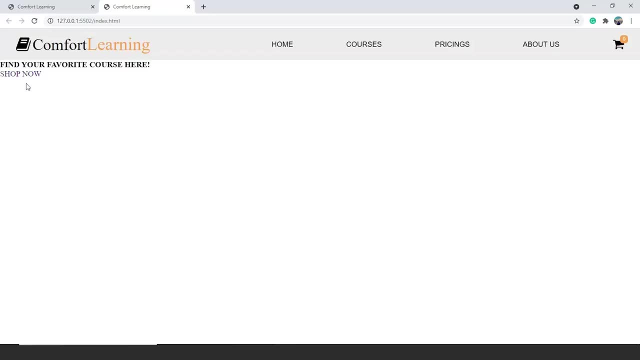 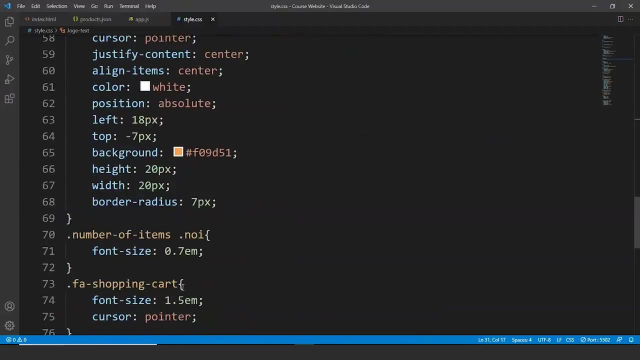 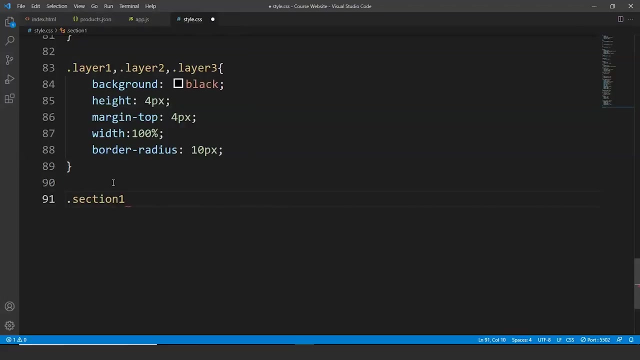 So let's do the styling part as well, And then we'll talk about it. So we'll move to the CSS file now, And here what we'll do. we'll write here: dot, section one, height. We'll use the calculator. We'll use the calculator. 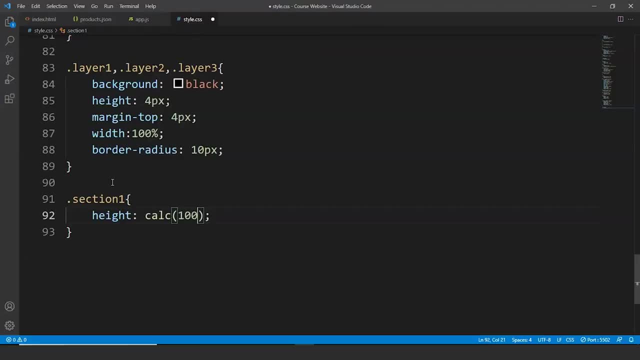 We'll use the calculator, We'll use the calc function and we'll write here 100VH minus 10VH. So what we are doing is we are reducing the navigation bar's height. We are reducing 10 viewport height from 100 viewport height. 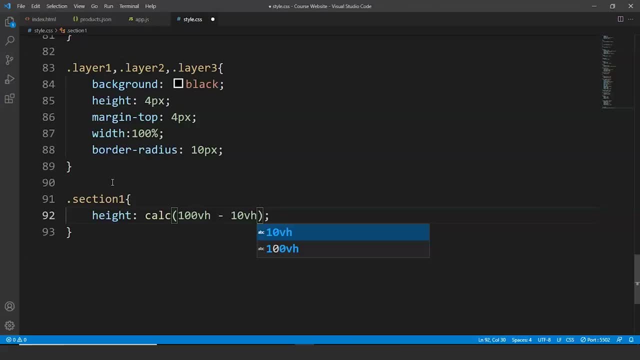 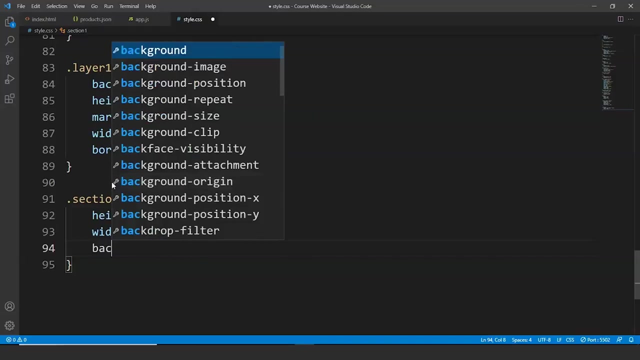 It means that from the whole screen area it will reduce 10VH and give it to that particular image. Fine, So next up we'll write here Width as 100%. We wanted to cover the whole home page, So that's why we are using width as 100% background. 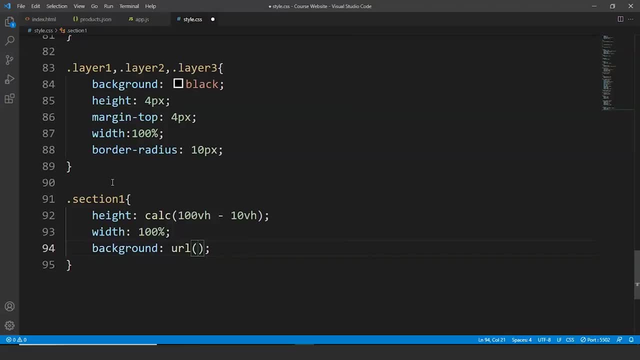 So we'll add the background image, We'll write here URL and inside this we'll give the path of our image. We'll write here images back one dot PNG And we'll write here: center, Center, cover, Fine, Let's do some more things. 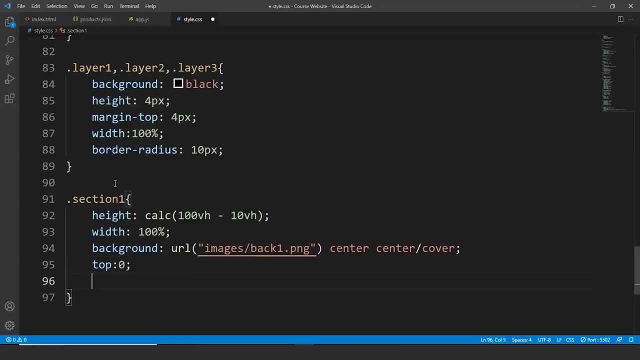 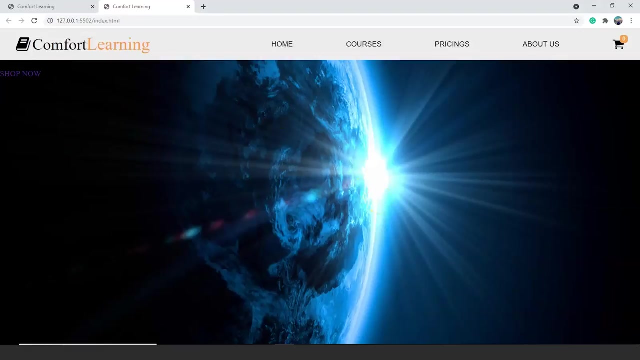 We'll write here top as zero. Left is zero, Z index is minus one. Fine, Save it. now Move to the browser and see if it's working. So here we are. We have our image over here, but this banner is not here till now. 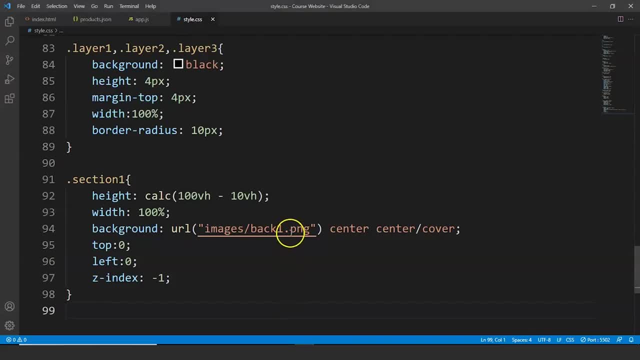 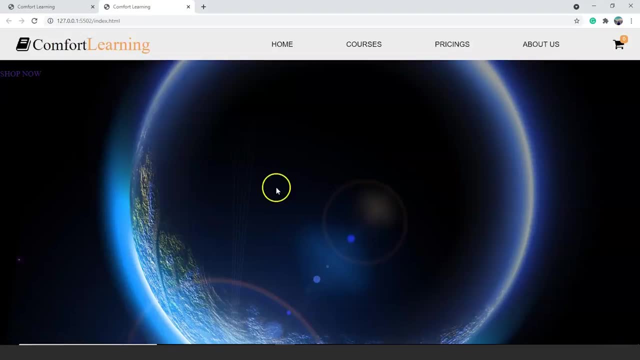 We'll style it So you can see the images over here. And one more thing, guys: we have two, three images over here inside a images folder. I'll let you see all of them. So here are the images, and this is the third one. 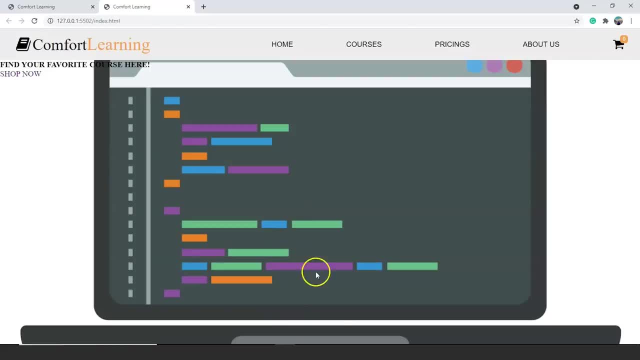 Okay, So this is the third one, So I was not sure which one to use. But If you guys liked any of these images, do let us know in the comments below and we'll use that particular image. for now we'll use my personal favorite image. 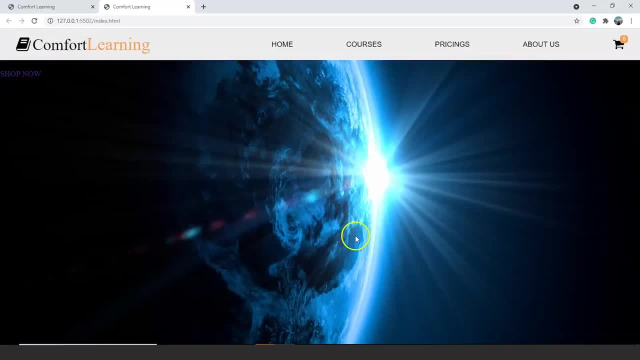 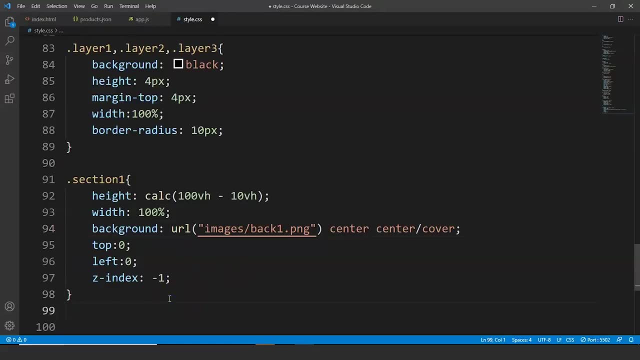 We'll use back one dot PNG. save it now And this is the image we are going to use in this particular video. So let me know if you have any other preference or if you know any other image, we'll use that as well. 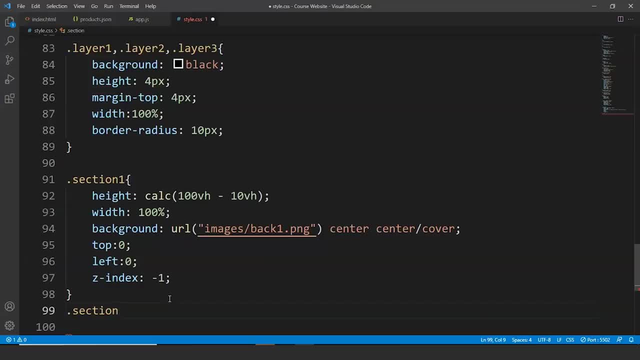 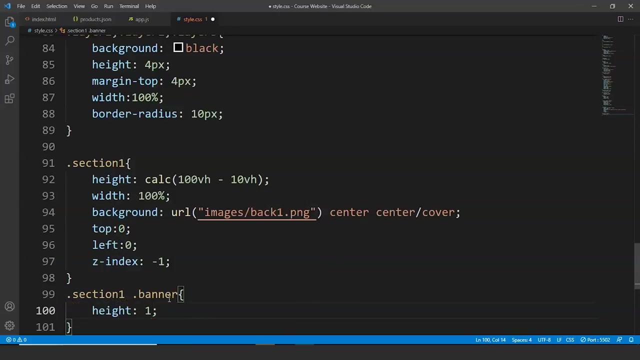 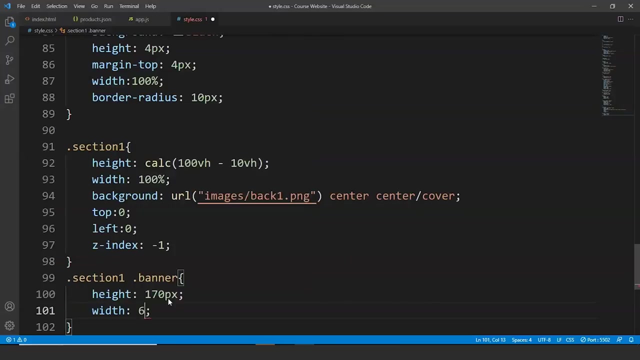 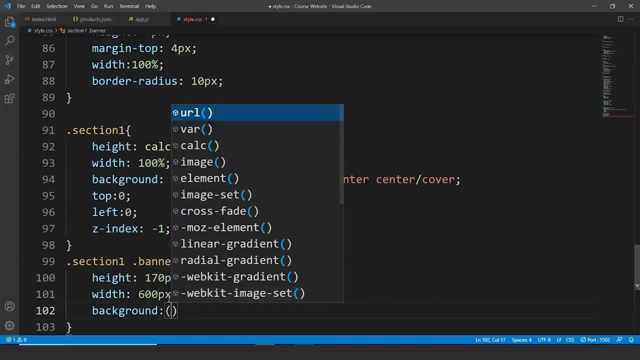 Then we'll write here section one And we'll style the banner as well. For that we'll write here: banner height is going to be 170 pixels. width is going to be 600 pixels. background is going to be a little bit grayish. 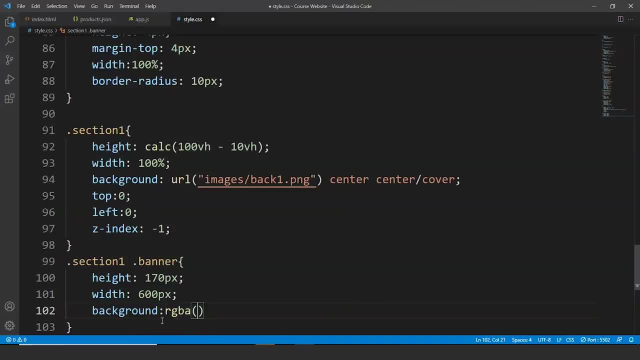 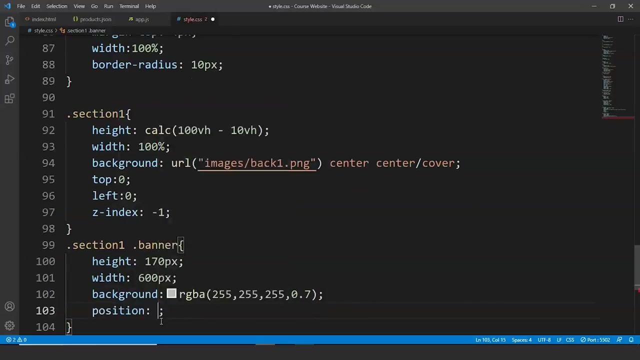 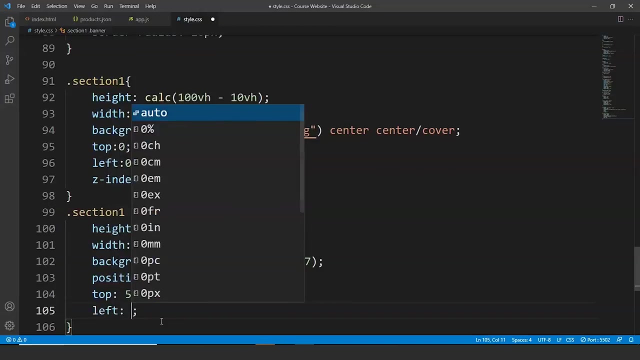 So we'll write here: RGBA- 255 comma, 255 comma, 255 comma 0.7.. So this is the particular RGBA value And next up we'll write here: position as relative. top is 50%. left as 50% of the image. 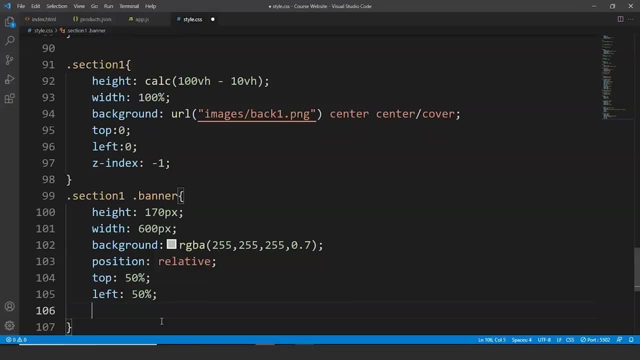 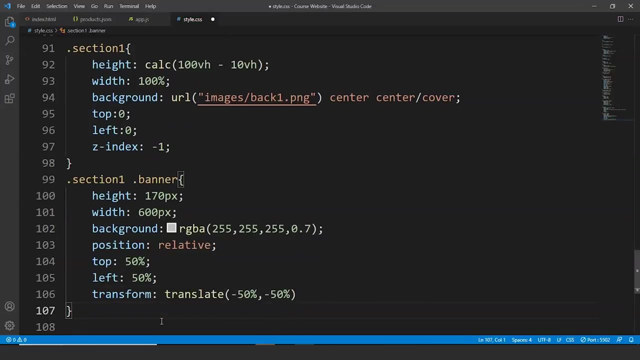 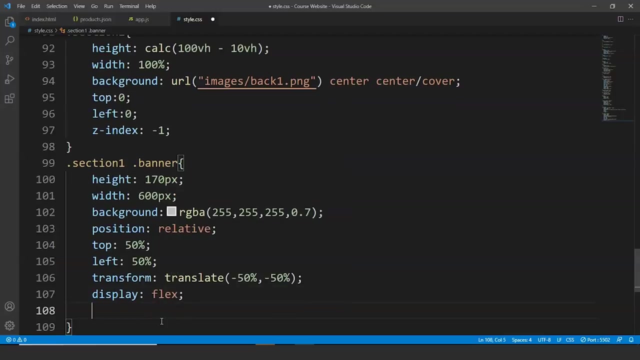 We want the banner to be present at the center of the image, right. So next up, We'll write here: transform translate and inside it will write minus 50% to minus 50%. Next up, we'll write here: display is flex, Justify content. 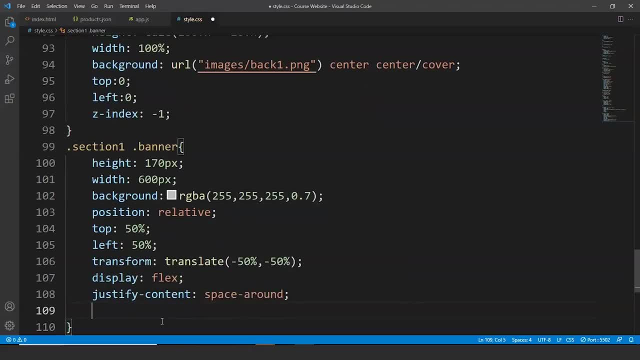 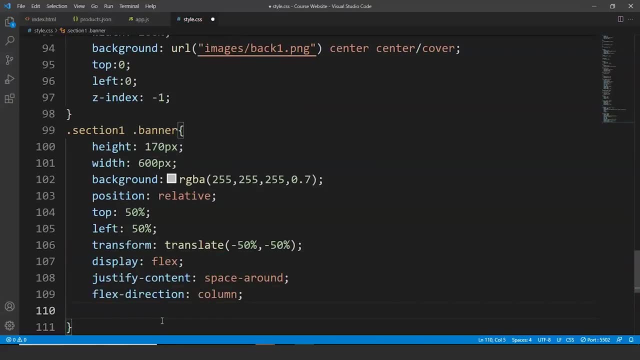 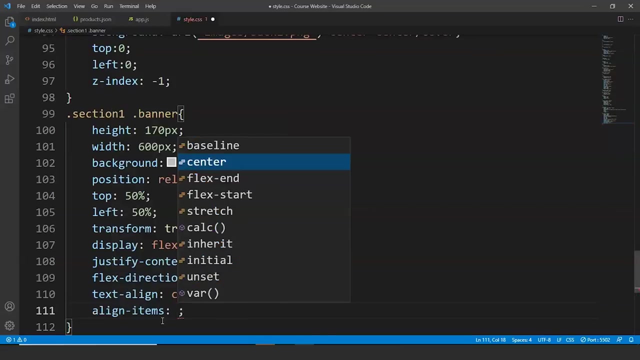 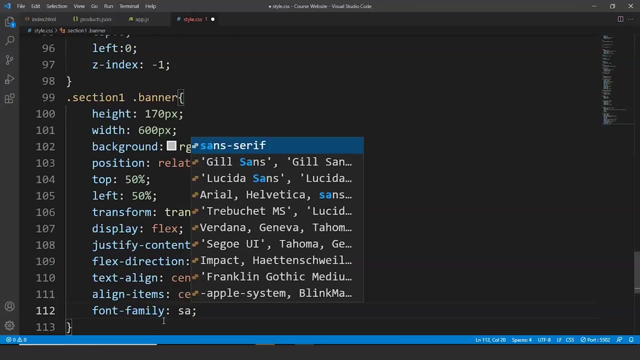 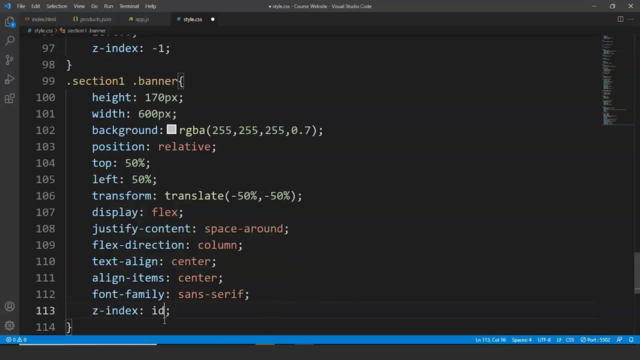 Justify content is space around and flex direction is column Text align is center And then we have align items is center. Font family is going to be sans-serif again, and we'll define the z-index as well, So the z-index is going to be eight in this case. fine, 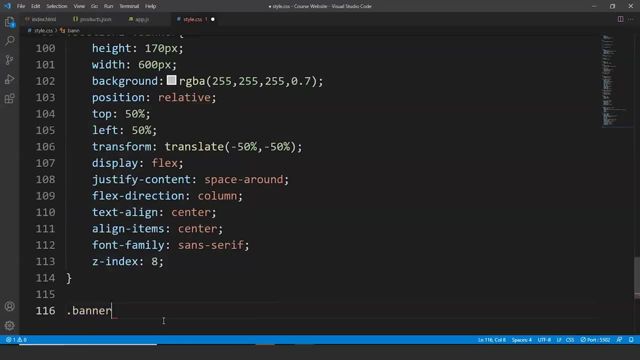 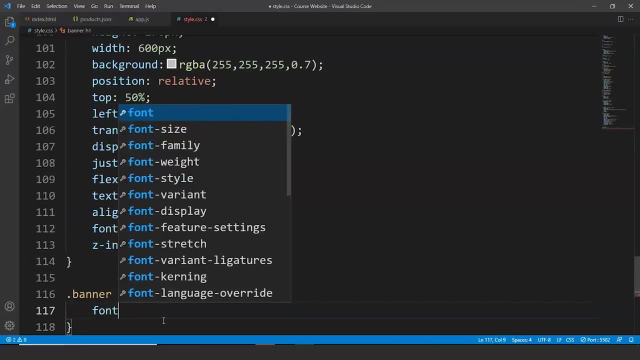 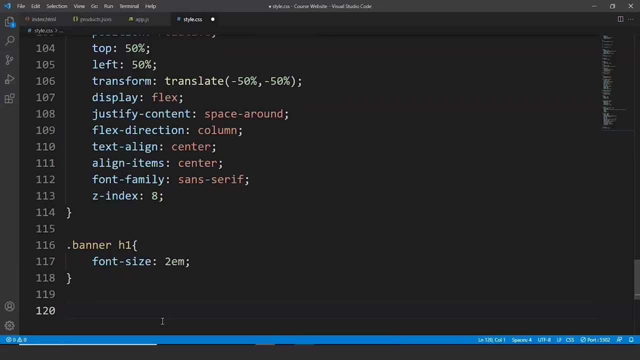 Next up, we'll inside the h1 tag inside the banner. So we'll write here: banner h1.. And inside this we'll define: the font size is 8. 2 m. Now we need to define the link for shop now. 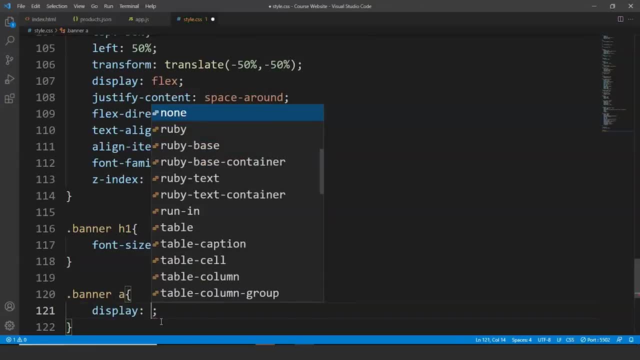 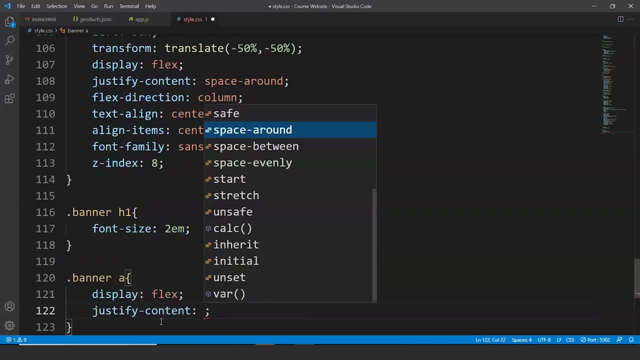 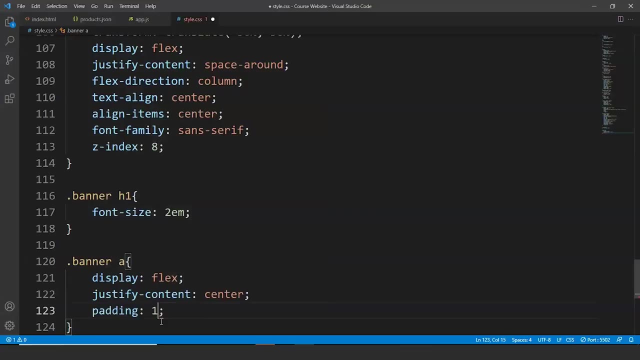 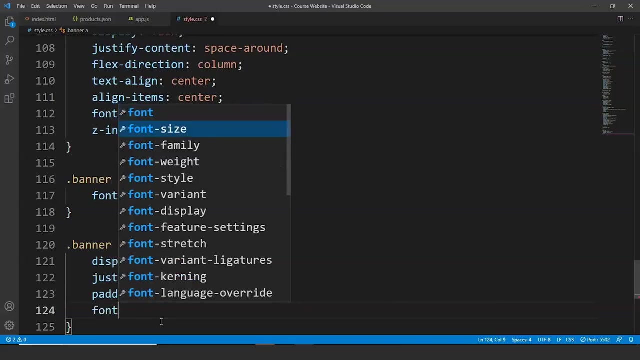 So for that we'll write here: Display as flex. Justify content is center. Padding is going to be 1m. Type text: Text change Type text change Type text change Text change space: 2.5 m. next up we'll write here font size as 0.8 m. so this is the font. 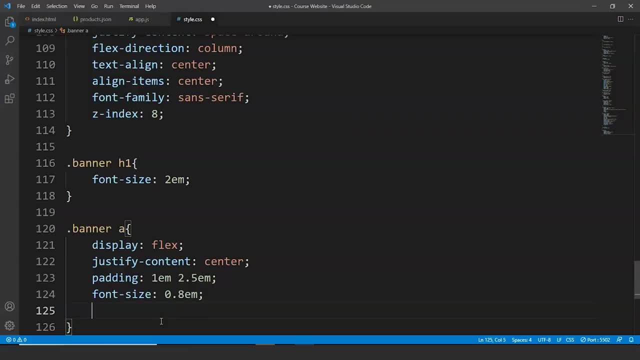 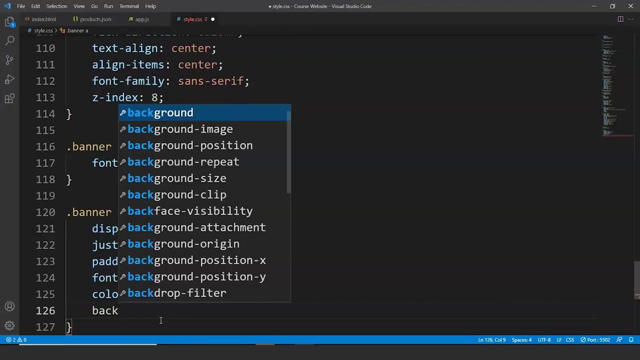 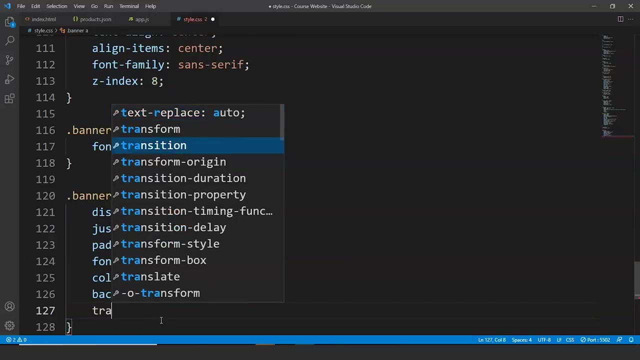 size for the shop now. button which looks like a button, but it is actually a link. so what we'll do is we'll define: the color of this button is white and here the background color is going to be ash: F, 9, 0, d, 5, 1. let's use this color and we'll write here: transition. 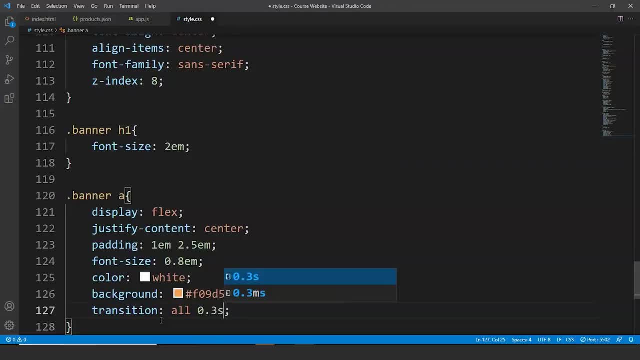 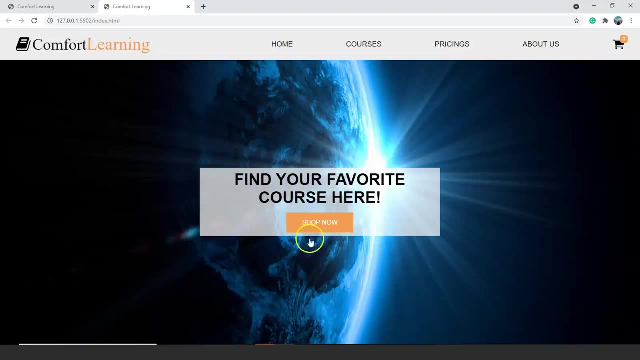 all at 0.3 second. now save it once, move to the browser and you can see. it looks fine, though. the only thing that is different here in this website is the color of this link, right, or is the color of the shop now button, so we can change? 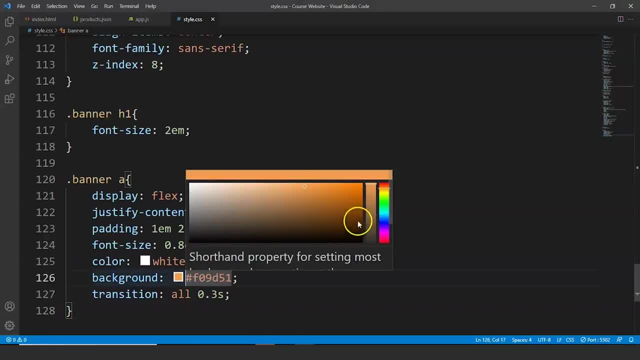 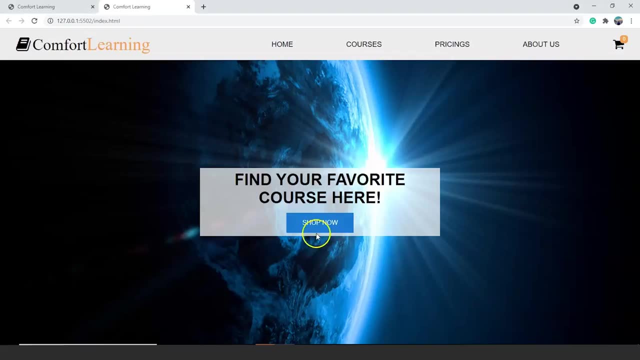 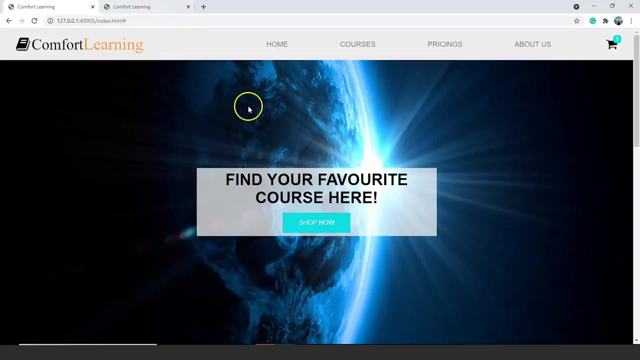 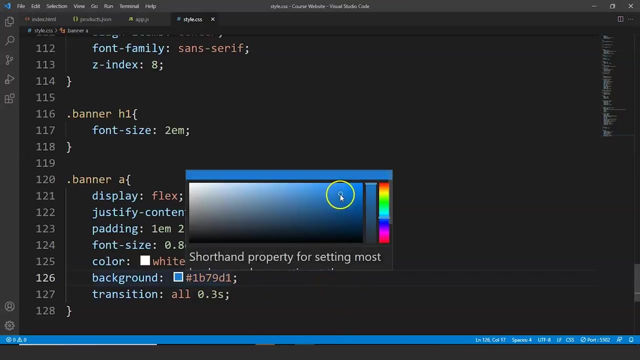 the color here. the color is sky blue. let's try to do it so. here you can see, the color seems a little bit different. now I don't know the actual value of this color. that's why I'm not sure about it. so what we'll do is we'll make it a little more bright, but save it now and 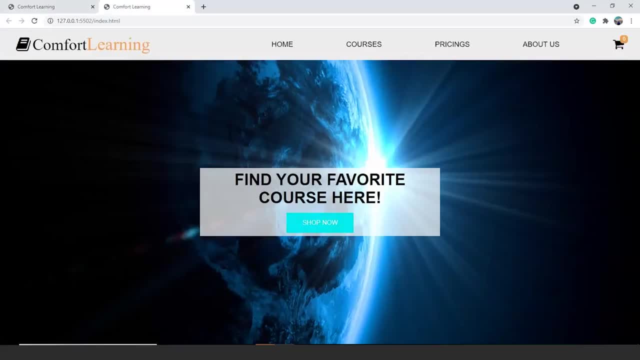 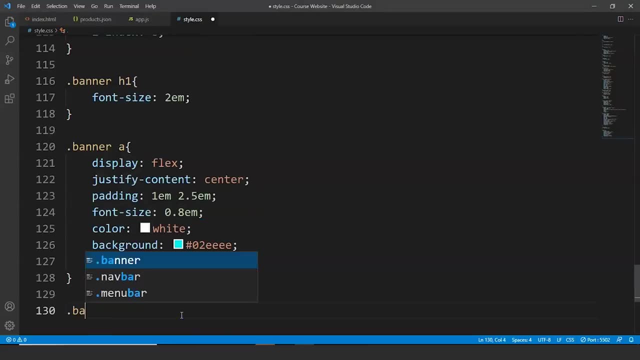 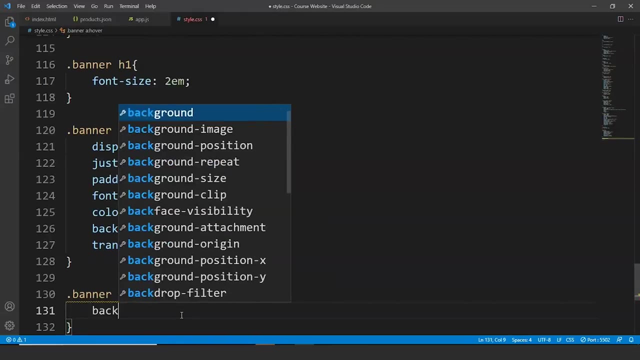 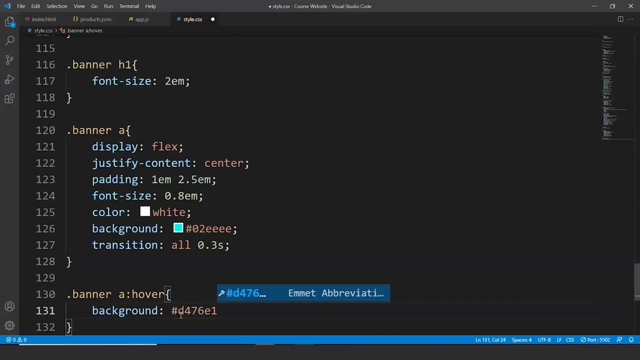 you can see it looks same now. so this was the color. we found that now we have to change the color of this button on hovering over it. so what we'll do is we will write here: dot banner a over, so the background we are going to change. we'll write here: hash d 4, 7, 6, e, 1. okay. 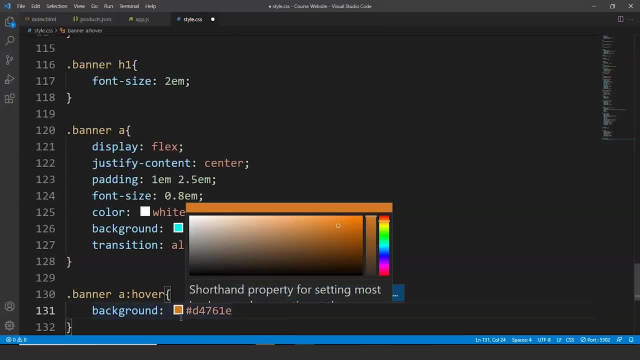 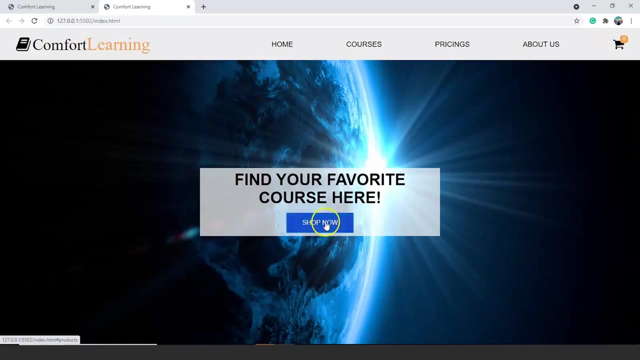 1e. the color codes are pretty hard to remember so we are not using this particular color, so we'll change it to a little bit blue. save it now. move to the browser and you can see it looks nice right. and the actual website it's a little bit dull, but in our website it looks nice right. 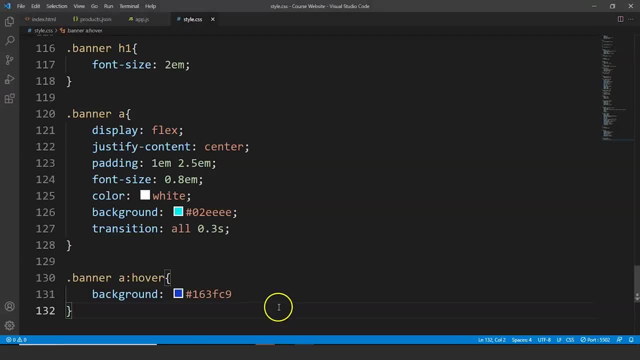 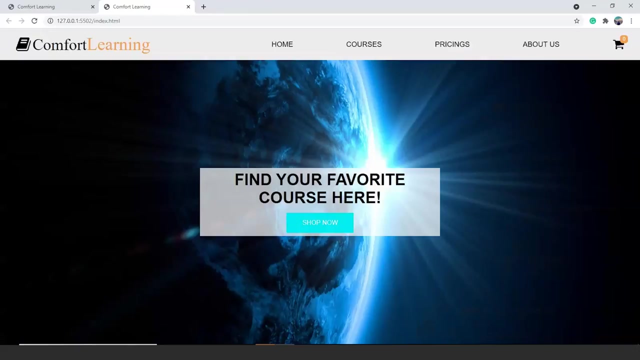 it's a little bit dark than the original color, so that's fine. you can change the color according to you. so you have seen that this part is also done. it looks. it just looks nice. right till now, the task we did was quite easy. the next thing we have to do is to add products to our website, which are the courses will. 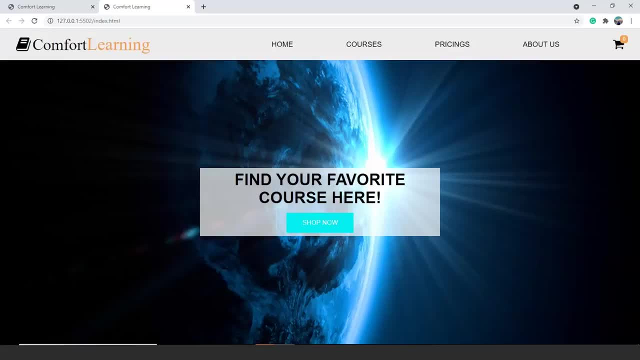 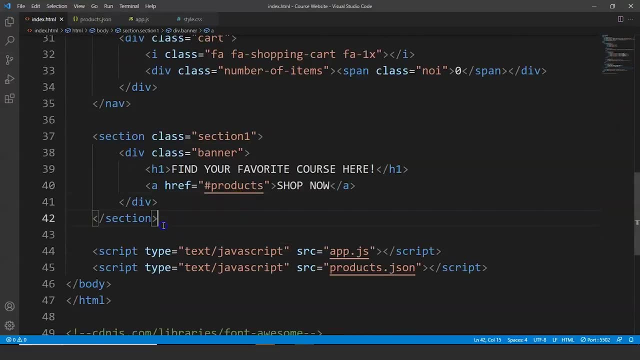 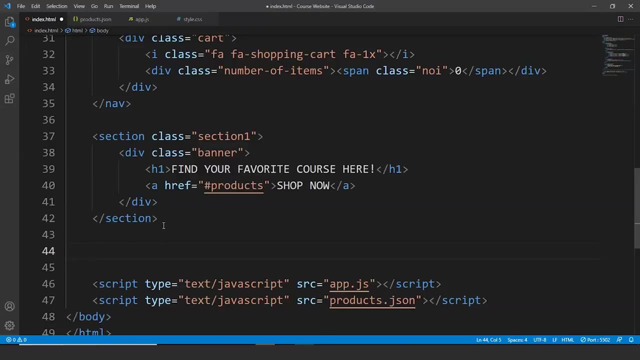 add those images to a website using Jason. we will add those images to our website using JSON only. so let's do the HTML part first, let's finish up that HTML file again and inside this now what we'll do is we'll define the section for products, so we'll 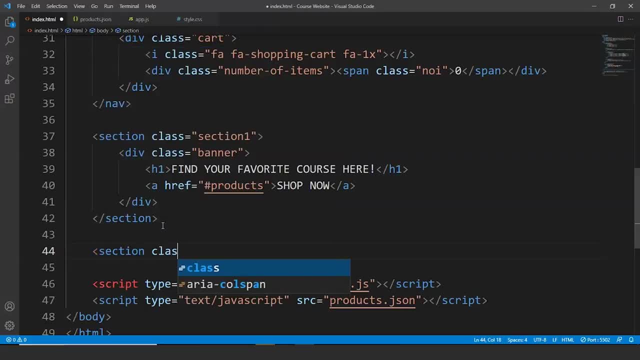 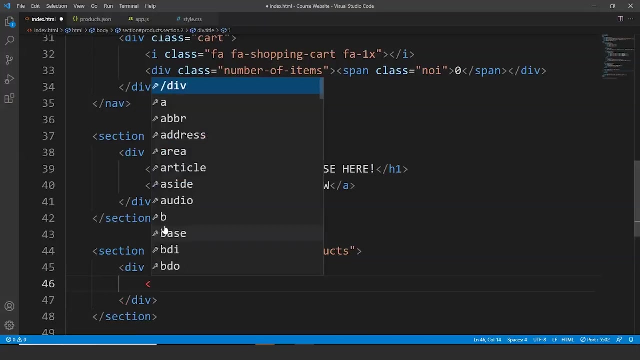 write here: section class is equals to section 2 and id is equals to products. fine, we'll use both the class and the id attribute for this particular section. we'll write here: div class is equals to title and here what we'll do is we'll write here h1 and inside this we'll write courses we offer. 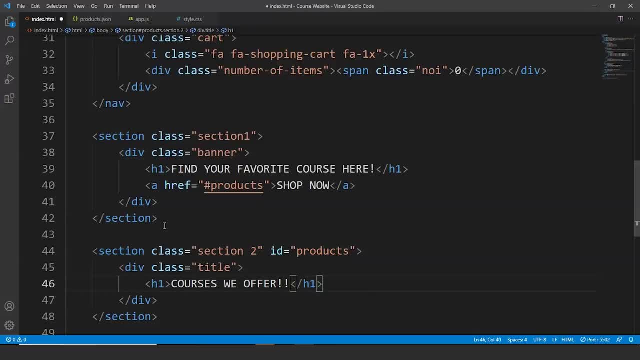 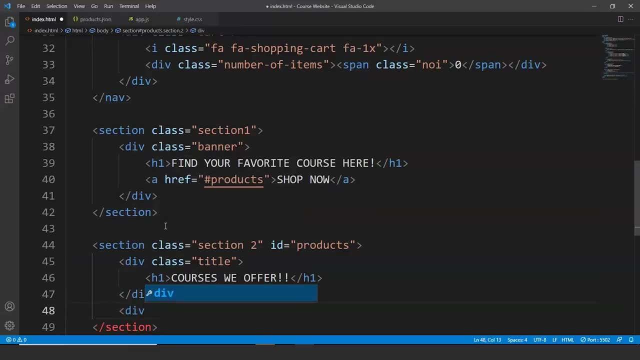 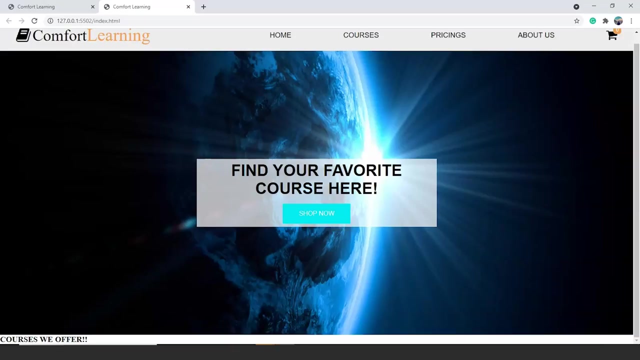 here we'll again add another div and inside this we'll write: class is product. close this div tag, save it, and there will be no difference. on the web page you can see here we have some text present at the bottom which says courses. we offer nothing else. let's add those. 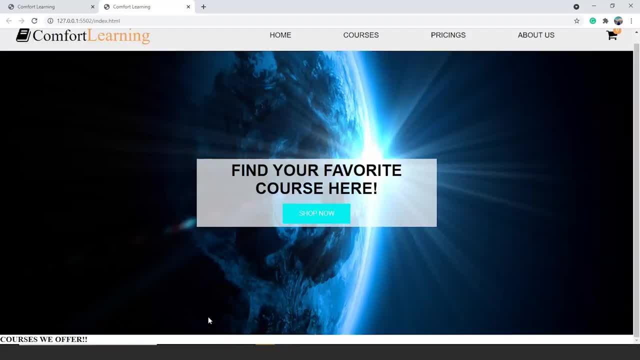 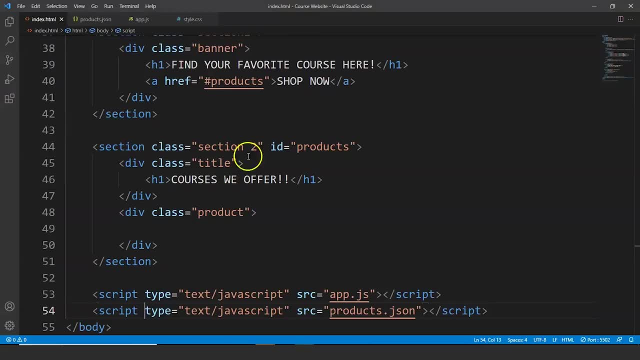 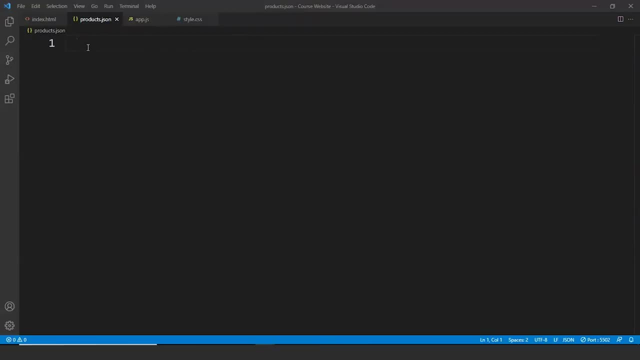 images. now what we'll do is we'll move to the json file and we'll add those images with some properties and pictures. so let's move on to the json file. so here's a json file: products dot json. what we'll do is we'll create an object here, so we'll write here items and then we'll use square brackets. now one thing: 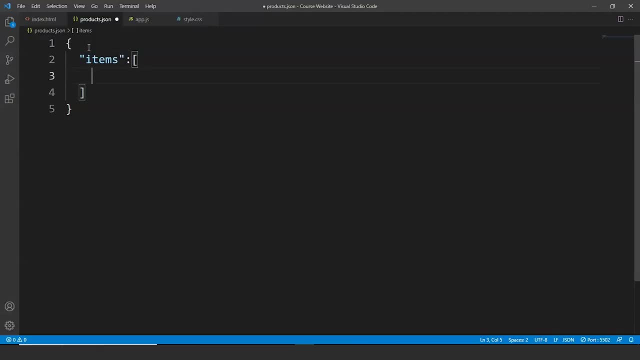 to notice while working on any json file is that json doesn't let us use single inverted commas, or we have to use double inverted commas for json file. so if we write here items like this, it won't work. see, it says this is an error. so in json file we have to use double inverted comma, or 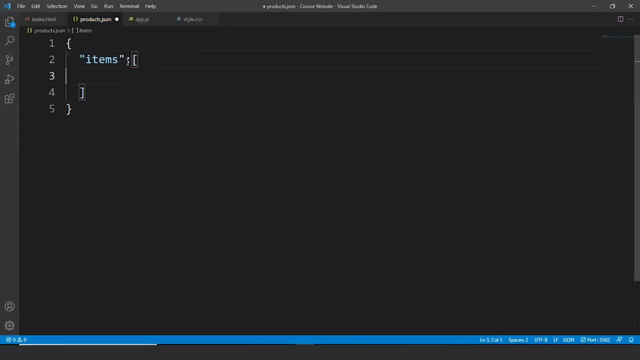 double quotes, not single quotes. so now, inside the items, what we'll do is we'll create the object for first image, so we'll write here sys, and then we'll write here id, so id will be 1. we have to use commas to separate the properties, so now we'll write here fields. 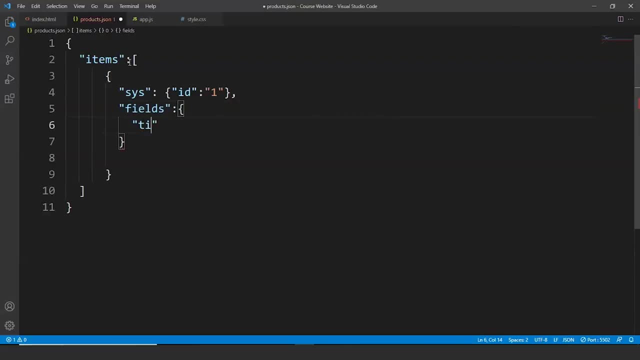 colon, and inside this we have to use title. so the title for first course will be python programming master course. we'll write here just one program: u, c, i, p course. fine, now next thing we'll do is we'll write here the price. the price will be, let's say, one, two, three point nine, nine dollars, and then we'll write: 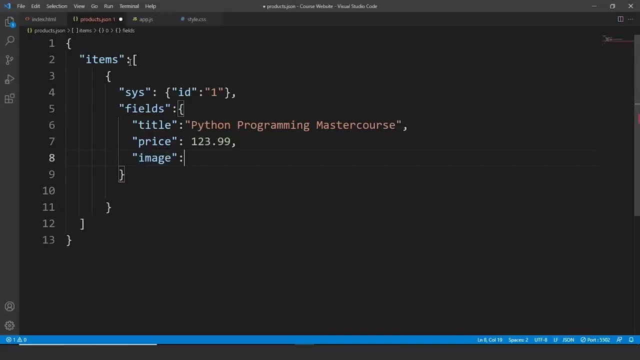 here image. so inside this we will define several properties for the particular image. we'll write fields and we'll use colon. then again we'll use curly braces, will write here file colon. then again we'll use curly braces, will write here URL so you can see it just says there's an error, so we have to remove this curly. 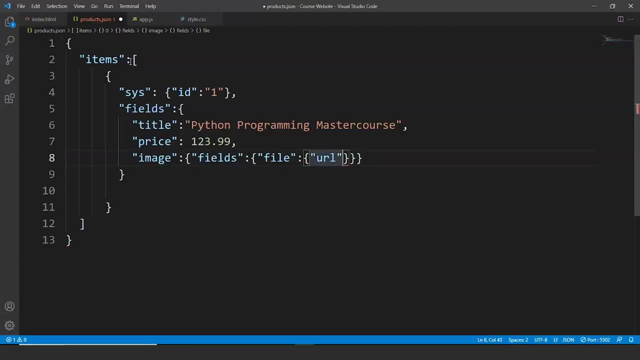 braces from here and we have to put it here now inside URL. what we'll do is we'll give the name of our file. so our file is stored in images folder and the file name is: and the picture name is python dot PNG. fine, so it is. 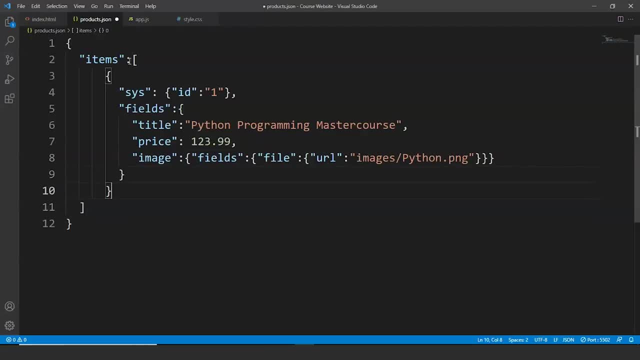 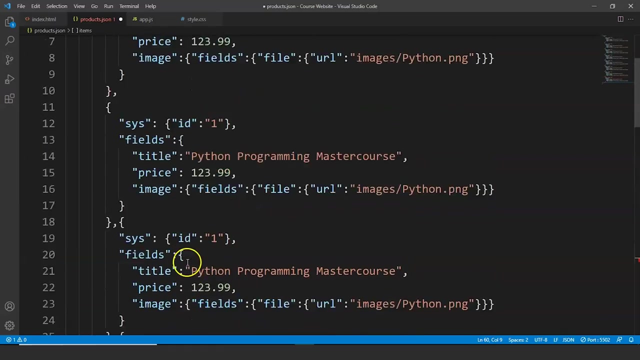 working fine. now what we have to do is we have to put a comma here to again insert one more image property. so we'll copy it from here. we'll paste it for eight times, then. what we are going to do here now is we are going to change the. 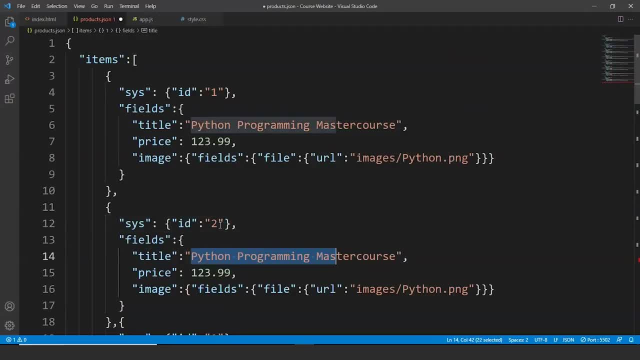 ID the title of the course. so the second course is C++ master course, and the price for this is, let's say, hundred and ten point nine nine dollars. we have to change the path as well. this image is stored as C++ dot PNG. for the third one: 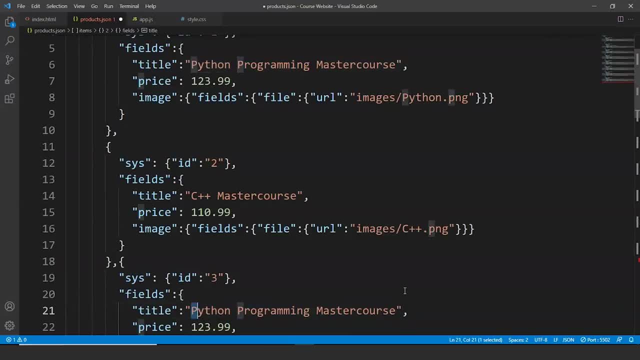 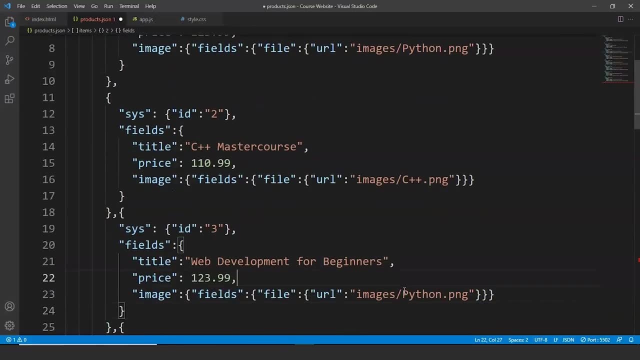 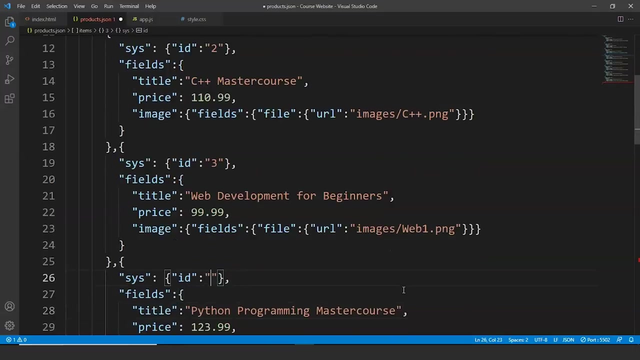 we'll write here: ID is three. the title is going to be web development for beginners, the price is, let's say, 99, because this is a course for beginners, and the file name is, instead of Python. we'll write here: web one dot. PNG will do the same for all the elements, so next up. 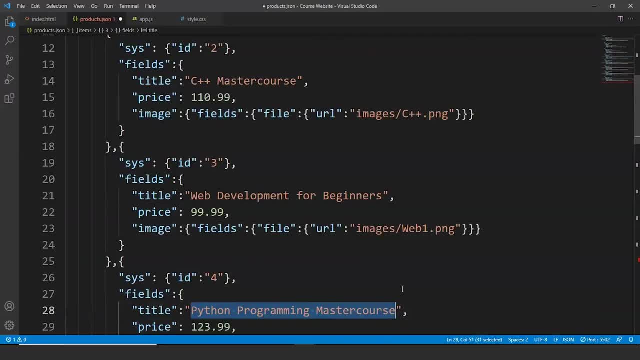 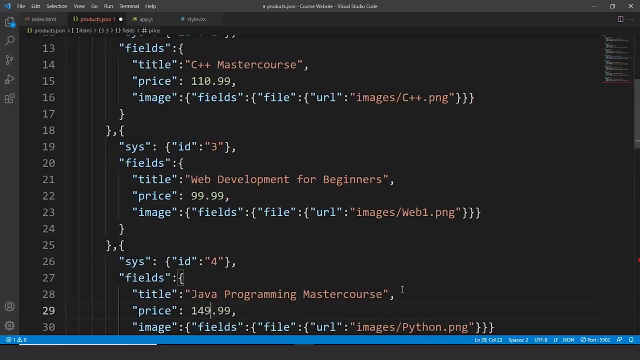 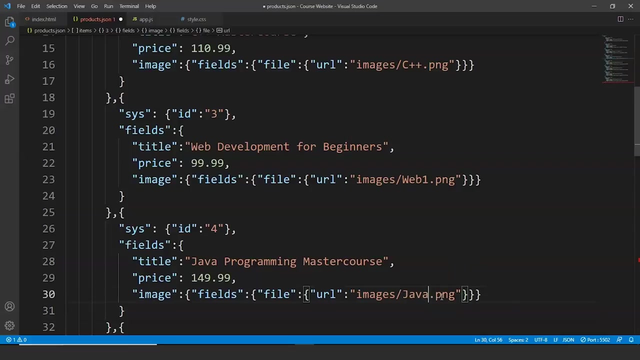 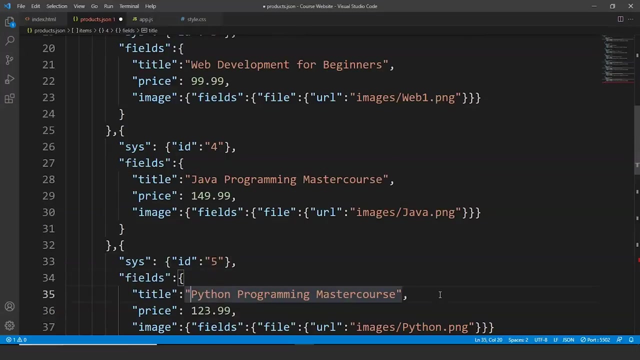 we'll use. ID is four and title is Java programming master course. fine, the price for this course is going to be one fourteen nine point nine nine dollars, and the file name is Java dot PNG. fine, next up, we'll right here. ID is five, the title is going to be digital. 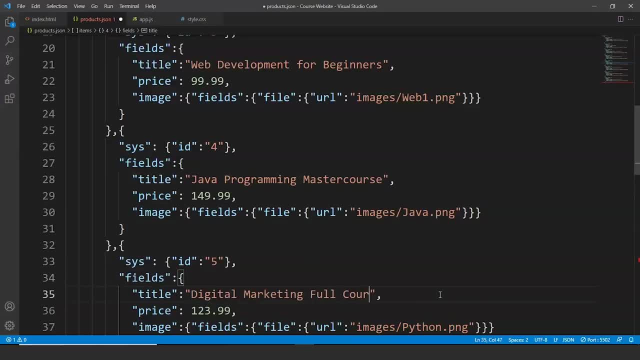 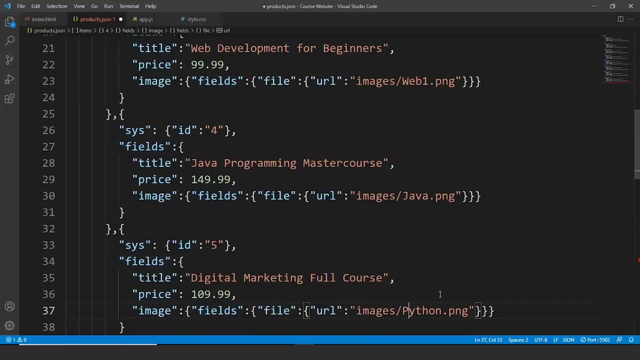 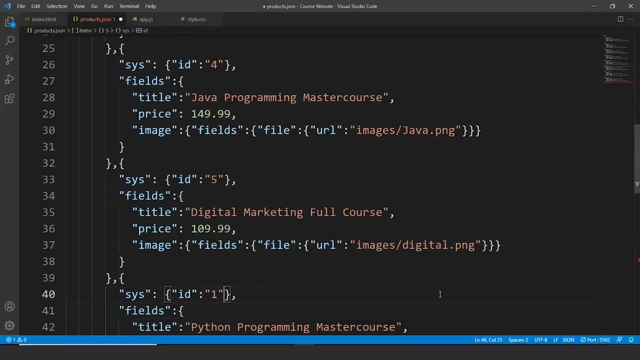 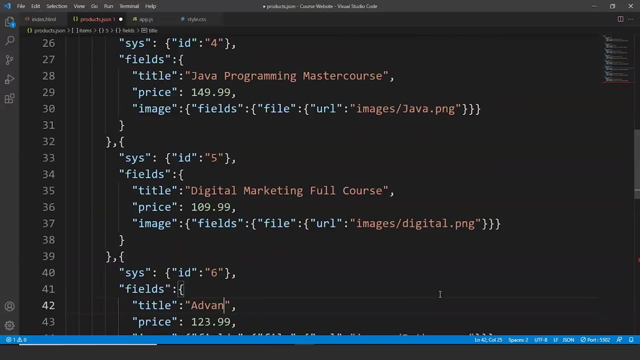 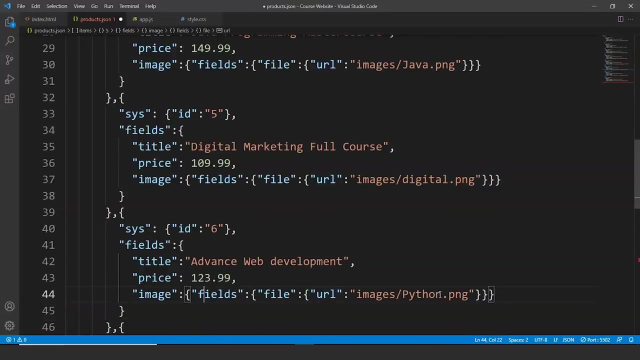 marketing full course. the price is going to be 109.99 dollars and the name of our image is digitalpng. and then we have ID as 6 for another course. this course is going to be advanced web development and the price is going to be comparatively high because this is an advanced course. so instead of Python, 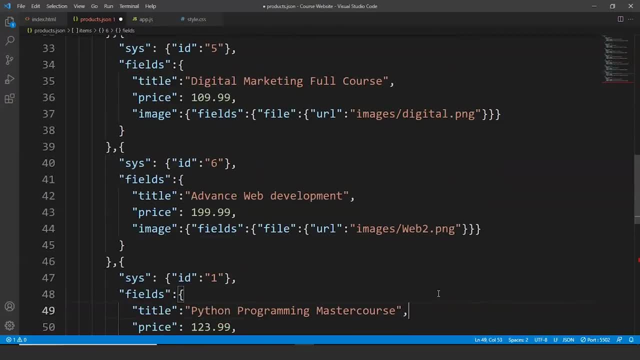 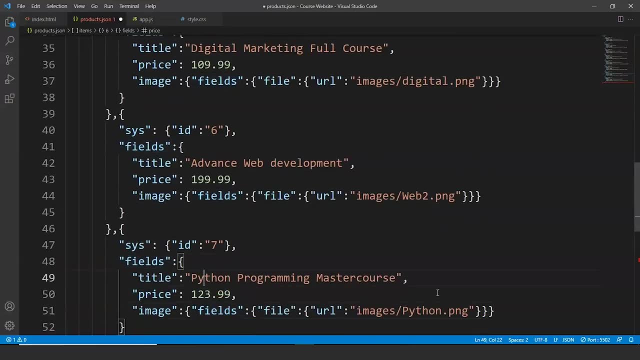 we'll write here web2, because this is the name of our image. then we have ID as 7 and the file name is going to be data structures and algorithms, and the file name is going to be data structures and algorithms- full course prices. you can decide by yourself. so instead of 123, we'll use 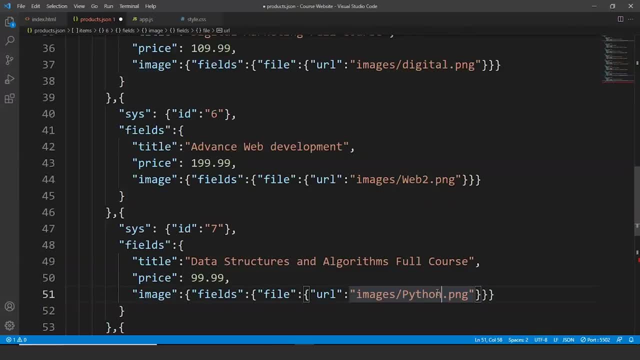 99.99 here and inside this we'll write datapng. this is a file name. then we have the ID as 8 for the last course. the course name is data science full course, the price is going to be 149 and image name is data 2. fine, so here. 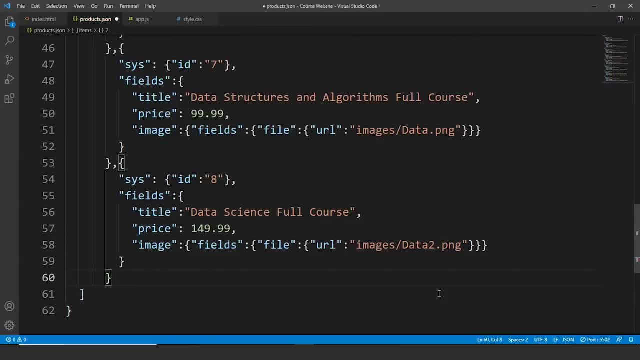 you can see it says there is an error. remove this comma because we don't have any other image remaining. so we are done with the JSON file. all of this may sound a little bit tricky to you guys, but it is what it is and we have to keep certain things in mind. 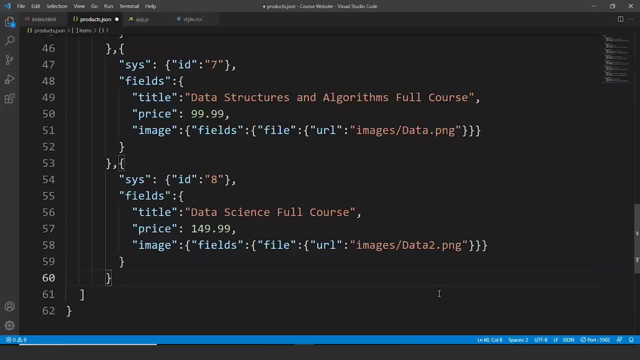 in mind for that. we can't see these products in the browser until we are done with the JavaScript part as well. so let's do the rest of the HTML part first, and then we'll see how this works in JavaScript. save it once. go to the browser. 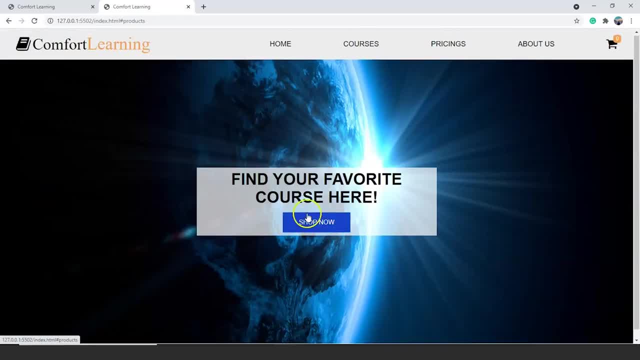 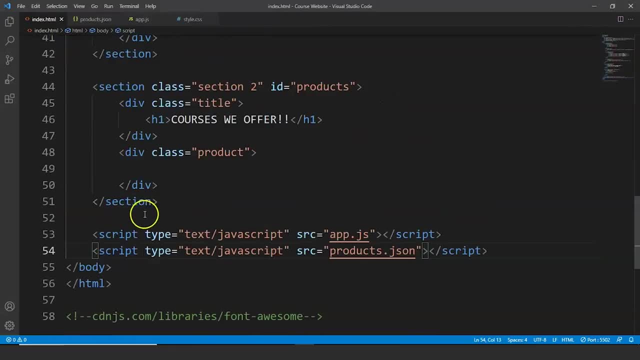 and here you can see, we are not able to see those products till now. so what we are going to do next is we are going to move to a HTML file and inside this we are going to do the remaining of our HTML part. so what we'll do is we'll write. 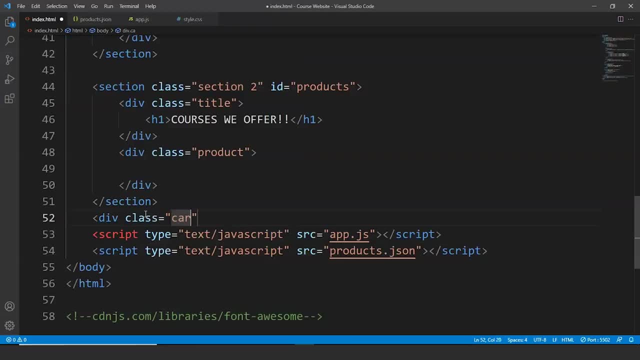 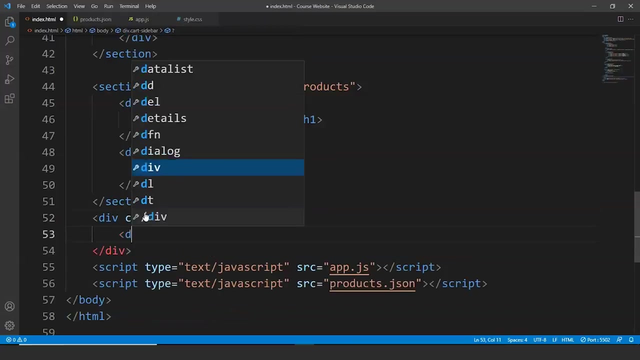 here div class is equal to cart sidebar. now we are creating the structure for our cart sidebar. it means that when we use the hamburger menu or when we decrease the size of a web page or web browser, the cart will open at the side. so we are doing the coding for that. we'll write inside this div class is: 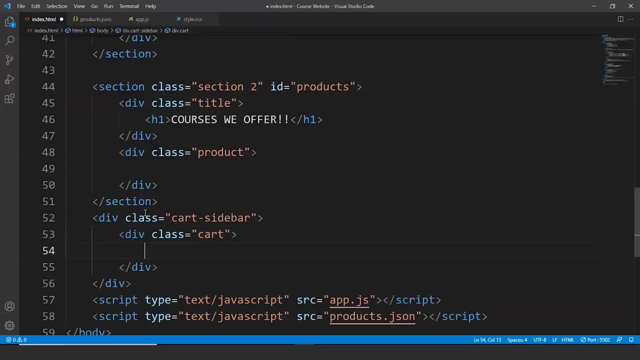 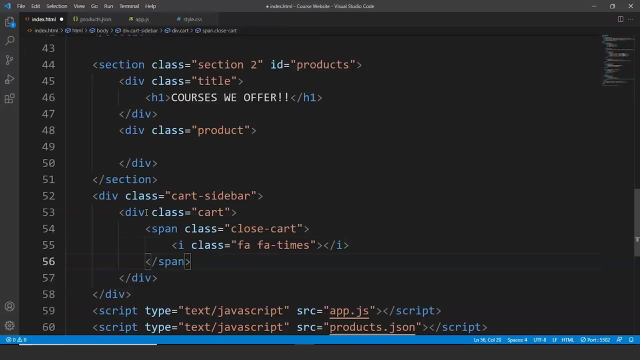 equals to cart and inside here we'll write: span class is equal to close cart. now, inside this we'll add an icon. we'll write here: class is equals 4 times and we are done with it. now, next up, what we are going to do is we are going to 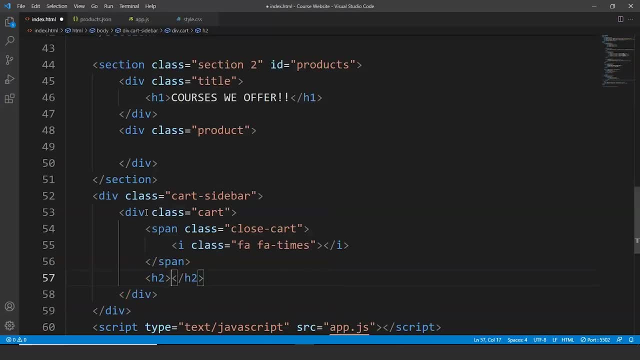 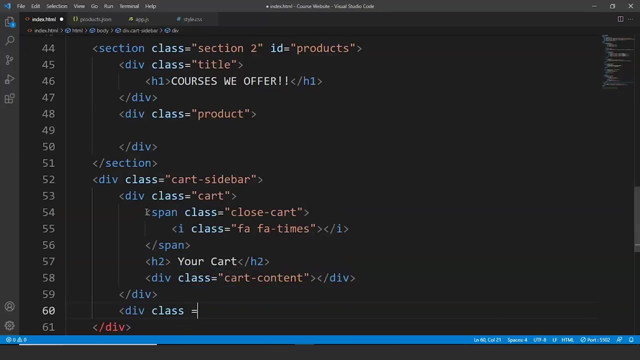 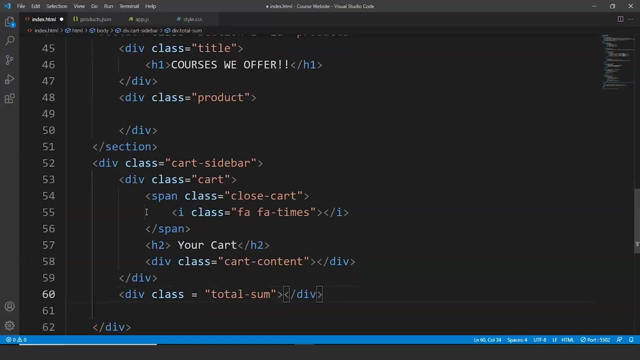 write the code inside of a cart. we are going to write a h2. it will say your cart, and inside this we'll write div class is equals to card content. next up, we'll write here: div class is equals to total sum and we are going to use dollars, right, so we'll write here h1. we'll write here: 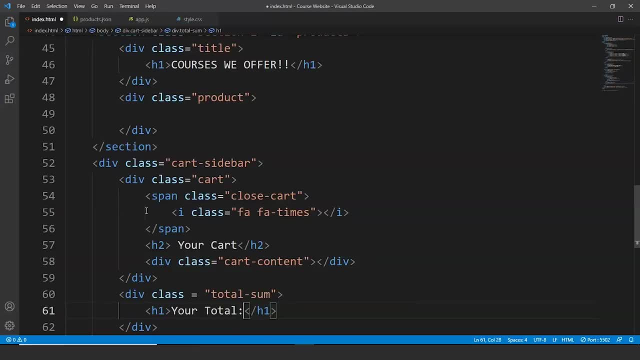 your total and we'll use the dollar sign here. after this we'll write: span class is equals to total amount. let's say we are going to change the class name, it will be total amount. we'll close this here and inside this we'll write zero, because at the start there will be no element. 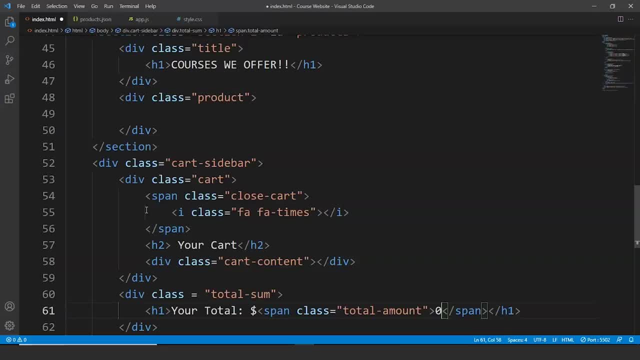 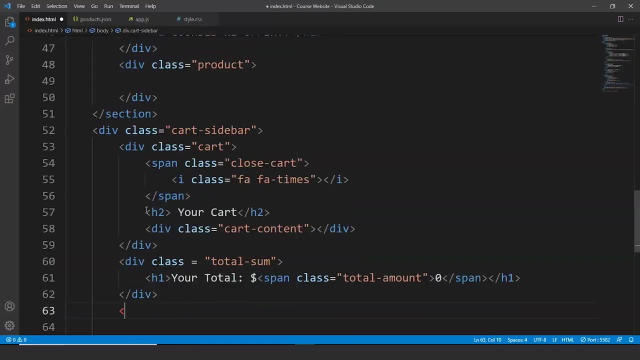 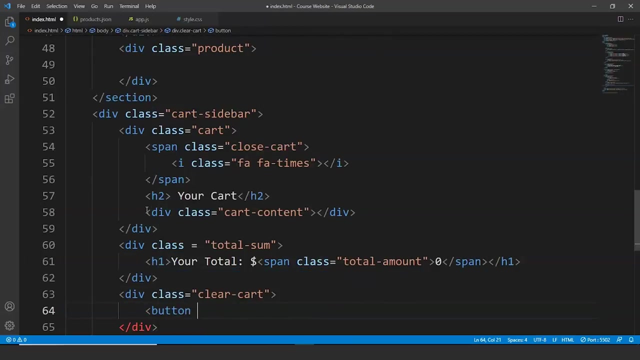 or no product present in the cart. so the total price will be zero at the initial point. so that's why we have written zero here. now we are going to write here: div class is equals to clear cart and inside this we are going to create a button, so the button class will be: 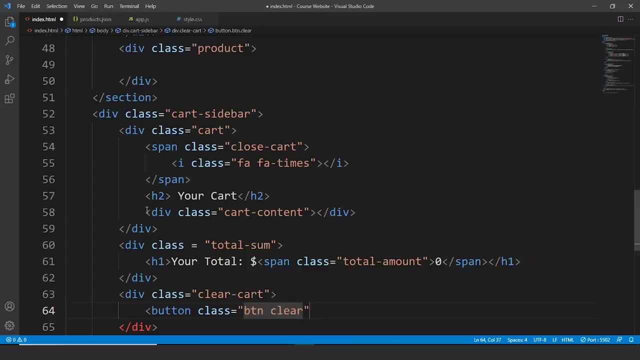 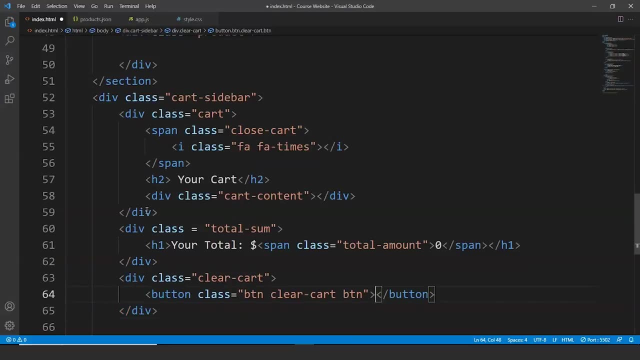 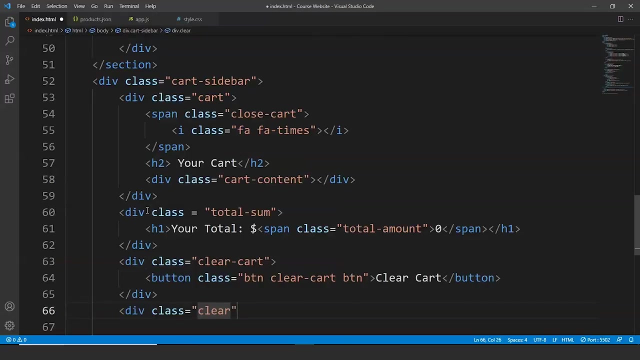 btn- clear cart, btn. so this is going to be a class and here what we'll do is we'll write here: clear cart. fine, we are going to do the same for proceed button as well. so we'll write here: div class is equals to clear cart. we are going to use the same class for both the buttons. 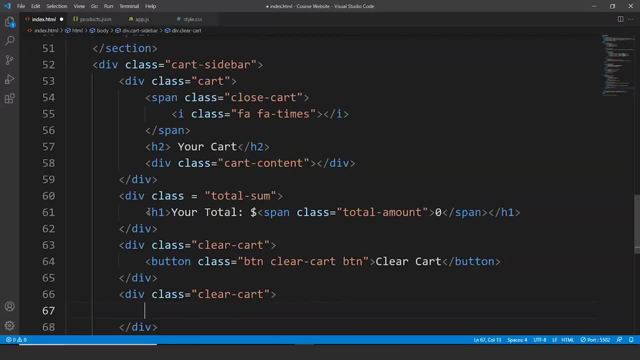 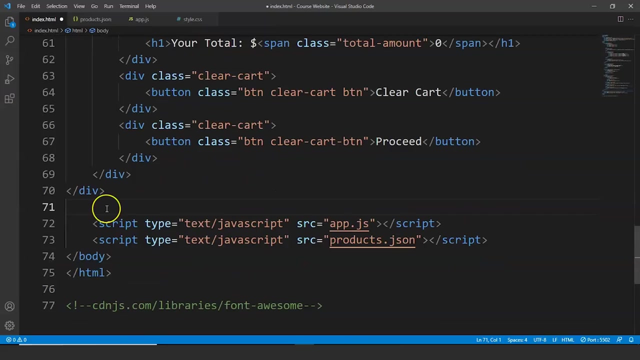 because i'll let you know what, why we are doing this at the end of this project. now we'll write here: button class is equals to button clear cart button. fine, we'll write here: proceed. we are done with the cart function. now what we are going to do is we are going to write: 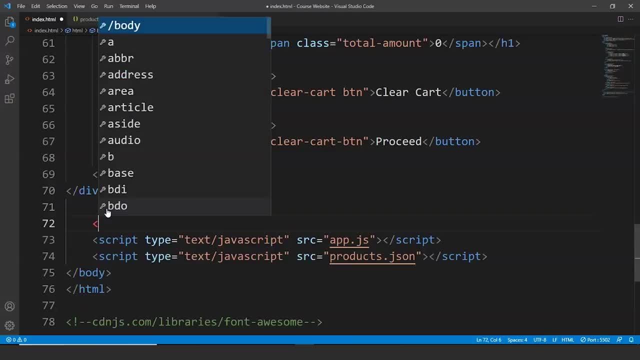 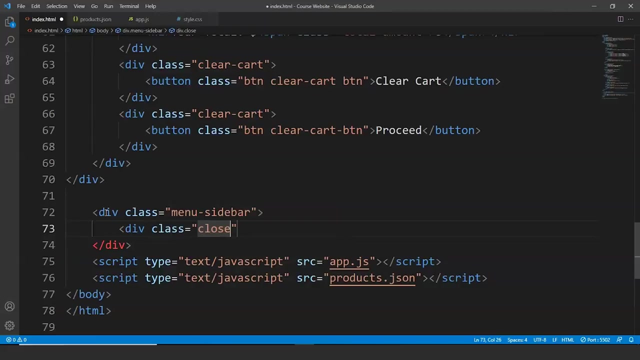 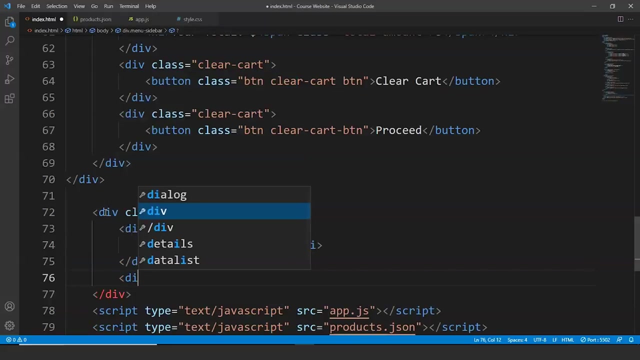 some code for the menu bar side menu bar. so we'll write here: div class is equals to, let's say, menu sidebar. inside this we'll write div class equals to close menu. and we'll write here: i class is equals to far, far times and we'll close this. i tag over here. next up, we'll write here: after this class, we'll write div. 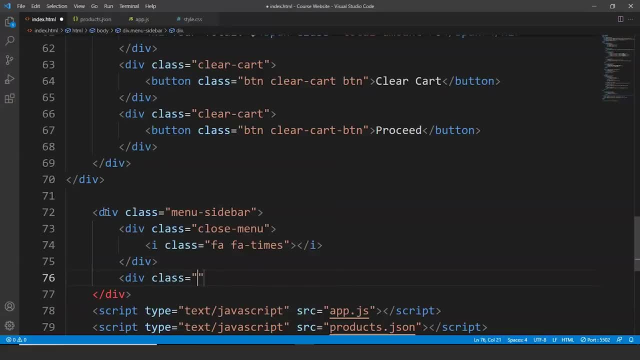 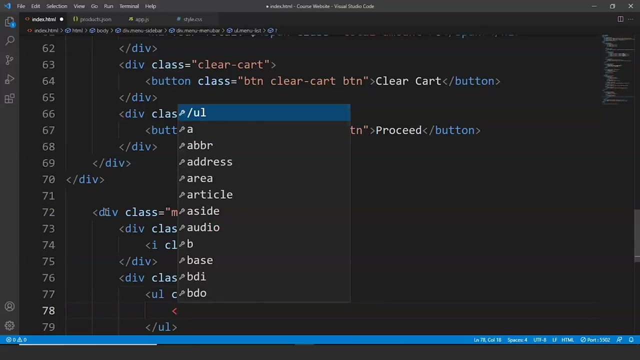 class is equals to menu. let's say this name is menu, menu bar, and inside this we'll write here: an ordered list class will be menu list. we'll write here: li class is equals to menu list items and we'll write here: a href is equals to hash. we'll write here: home. 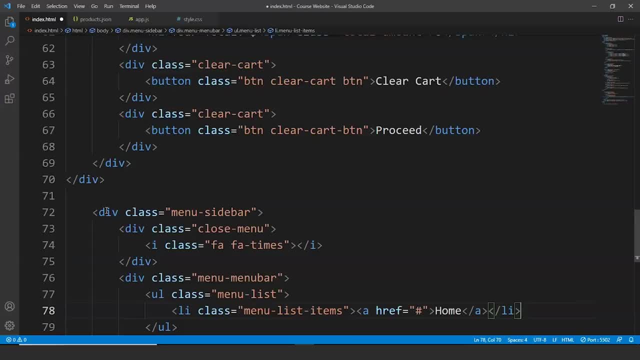 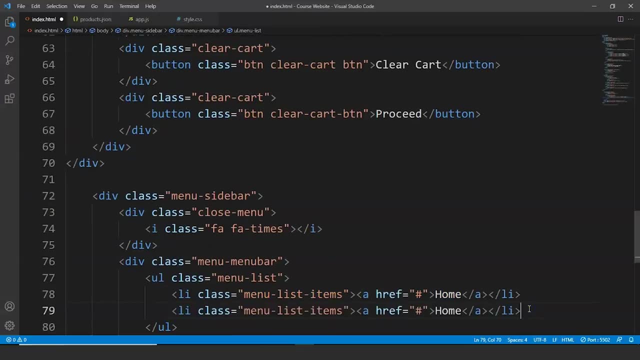 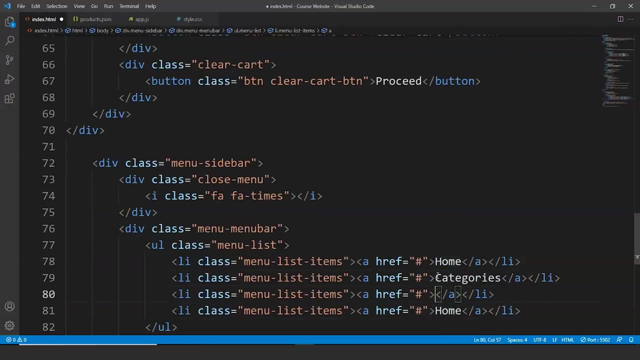 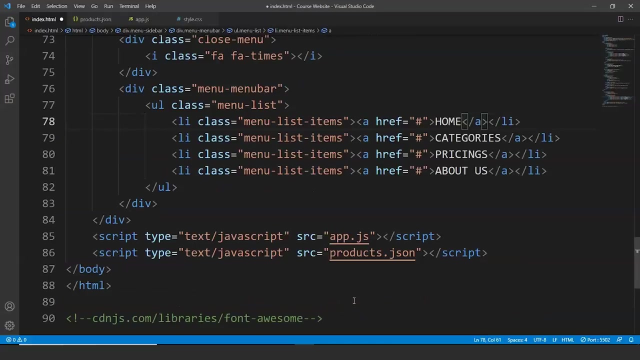 and we are good to go. fine, we'll do the same for categories pricings and about us. so we'll copy this statement. we'll paste it for four times here. we'll write instead of home: categories, pricings and about us. fine, so we are done with the whole html part now and we are left with css. 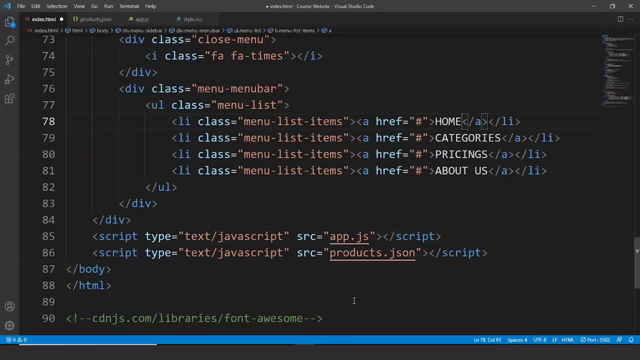 and javascript only. let's do that as well. let's move on to the css part first and do the rest of the styling, except for the products. we'll do it for products at the last. so let's move on to the css file first and what we'll do is: 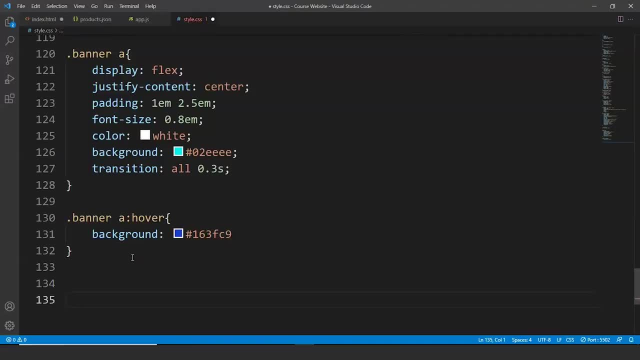 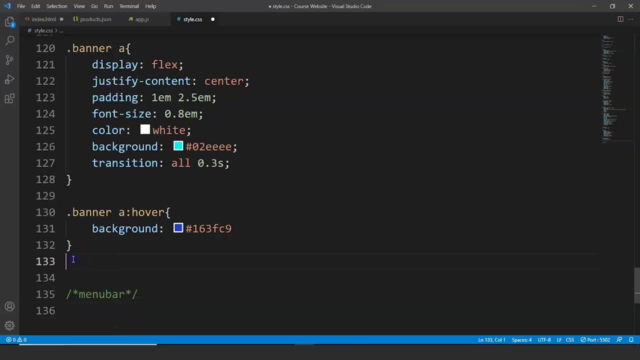 so that it will not create any confusion, we'll write here menu bar, because we have to write the code here between this banner style property and this menu bar for the product section. so that's start writing the code from here, and later we'll add a code. 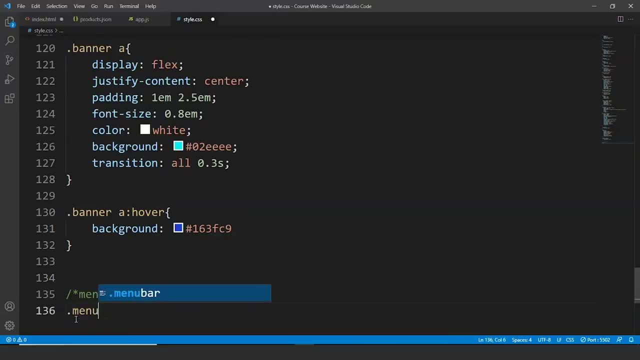 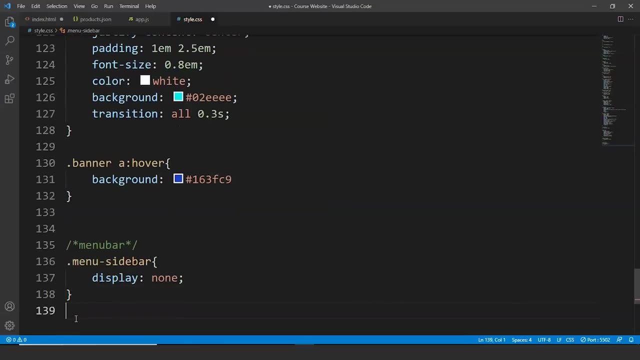 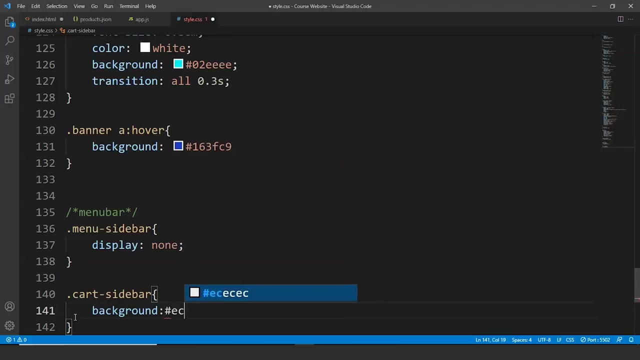 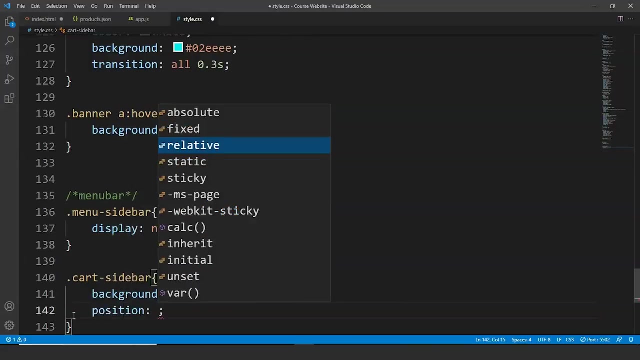 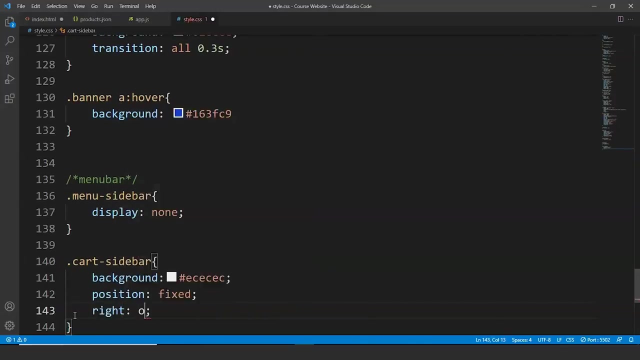 here in between. So we'll write here: dot menu sidebar display will be none. And then we'll write here: dot cart sidebar background is going to be hash EC, EC, EC, So a little bit grayish white. we can say We'll write here: position as fixed, right as zero, and 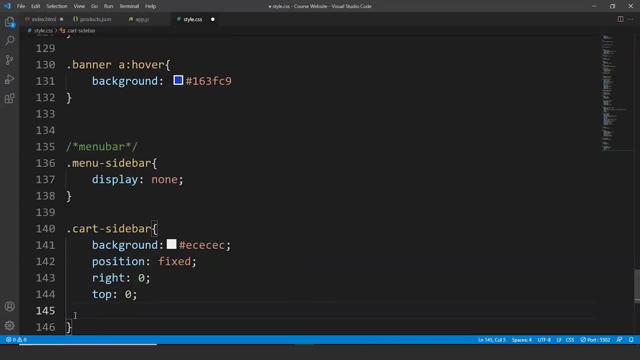 top as zero. So these are the properties we are defining in a CSS part. Then we'll write here: width as 450 pixels and height as zero, 100. viewport height: Fine, We'll define the z-index as well. We'll write here z-index. 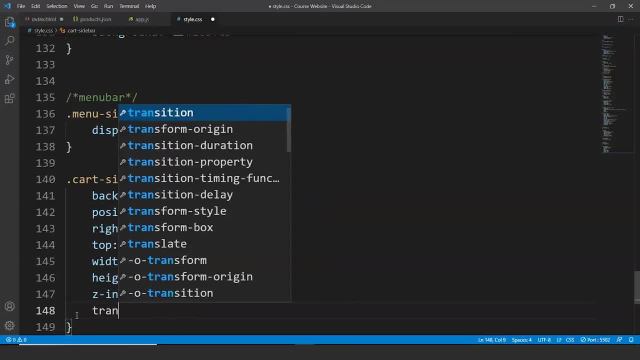 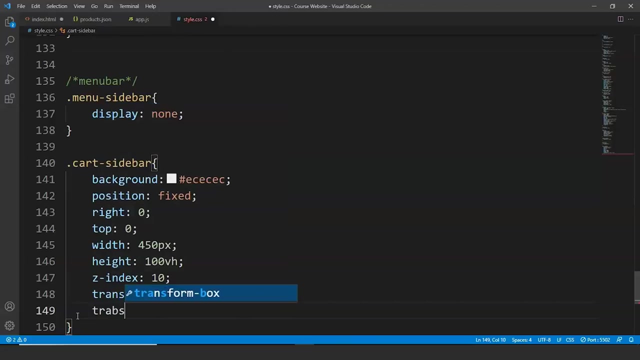 is 10.. Transition is all. it's 0.3 seconds and the transition will be linear. Fine, Next up, we'll write here transform, And inside transform we'll write here: translate x. Fine, So inside, here we'll write. 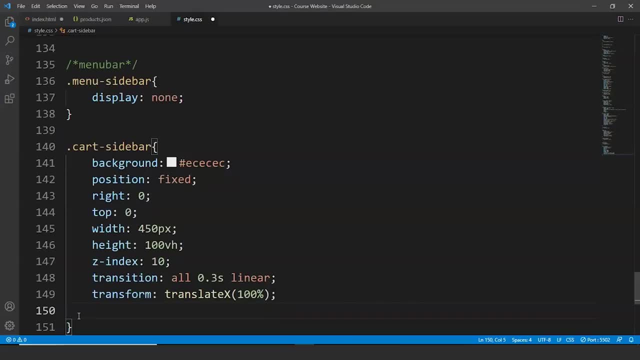 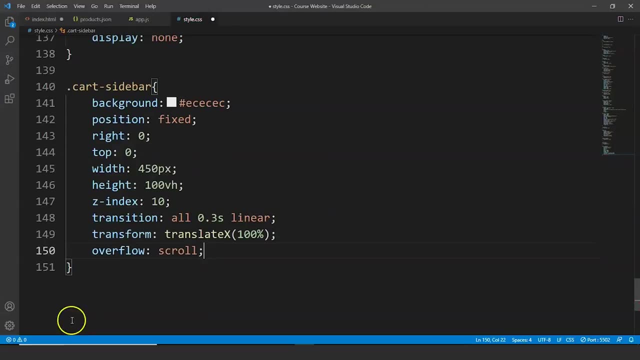 hundred percent it will go along with the X axis. That's why we have written it over here. We'll write here: overflow scroll. We are done with it. Next up, we'll write here Cart sidebar and we'll write herecart as well. So we'll define Padding here. We'll 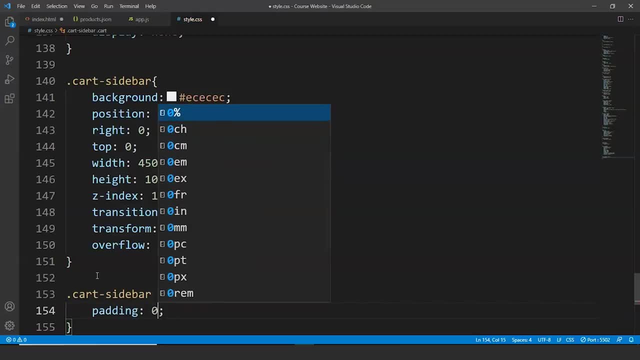 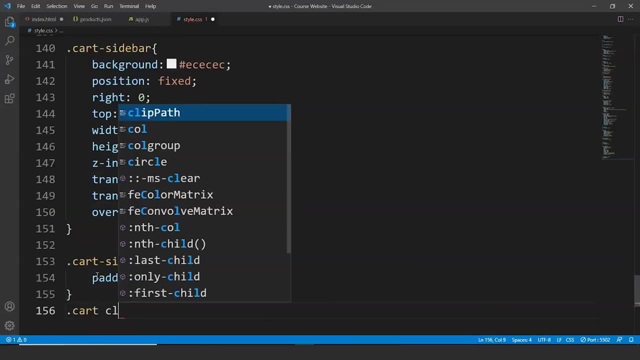 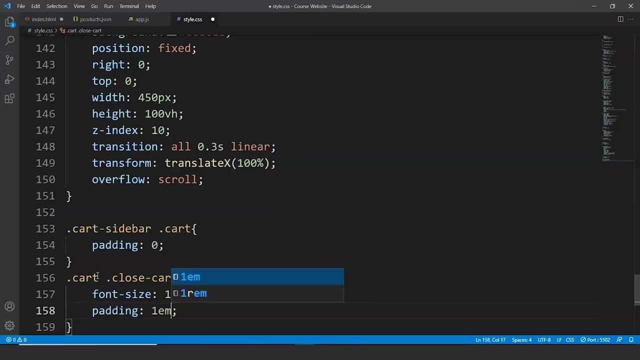 right here. padding is zero in both the cases. Next up we have dot cart and close cart right, So we'll write here for both of them. we'll write here: dot cart space, close cart. the font size is going to be 1.3 m, padding is going to be 1 m and cursor is going to be 0.2. fine, 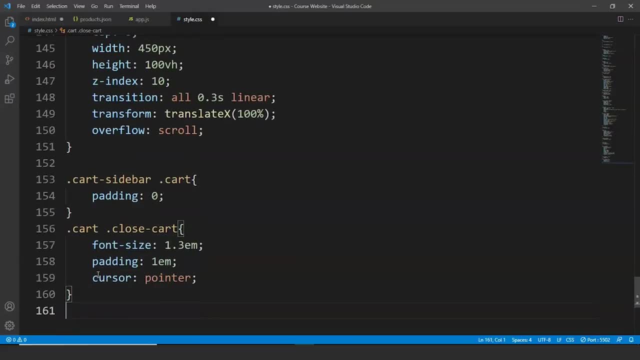 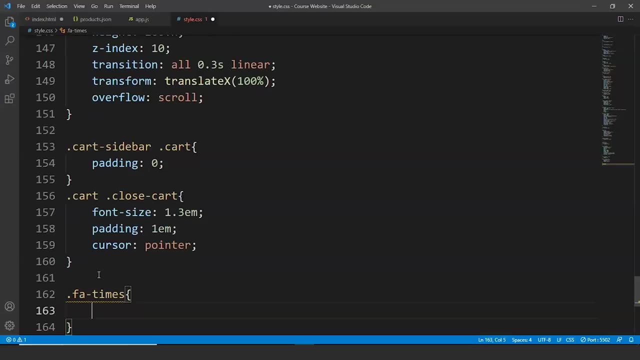 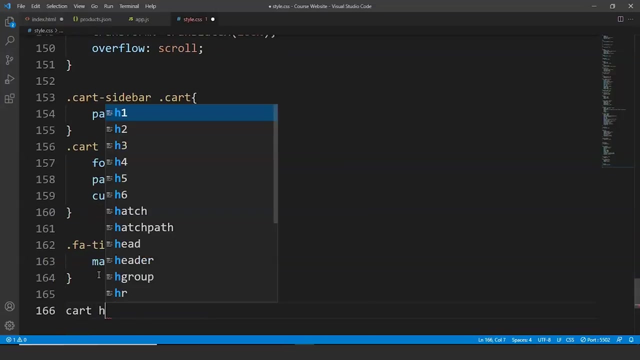 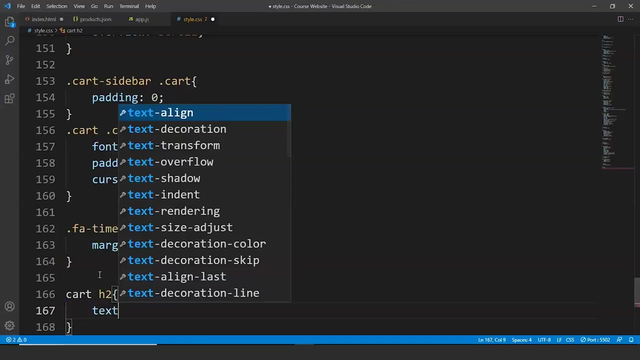 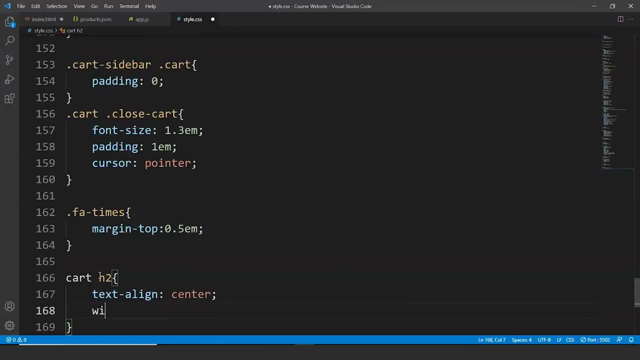 We'll write here: dot for times. inside this we'll write margin top as 0.5 m and we'll write here: cart h2 is text. text align will be center for the heading of our cart, which is your cart. So we'll write here: width is hundred percent. 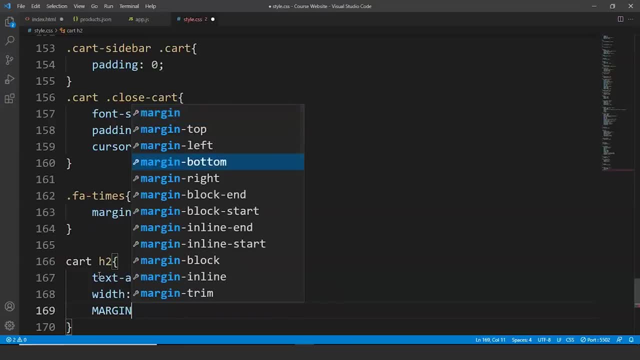 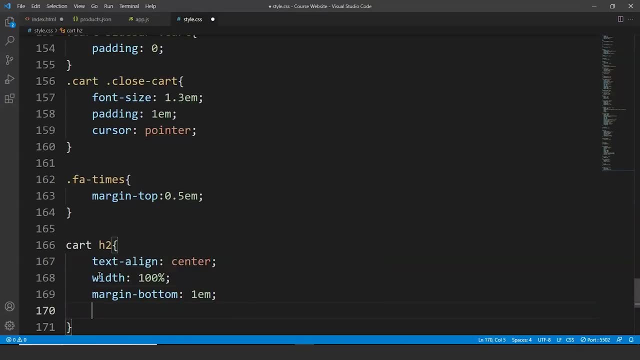 margin bottom is going to be 1 m, And what else we have to do? we have to include the font size as well. So we'll write here: font size is 1.1 m, slightly bigger than the default font size, then we'll. 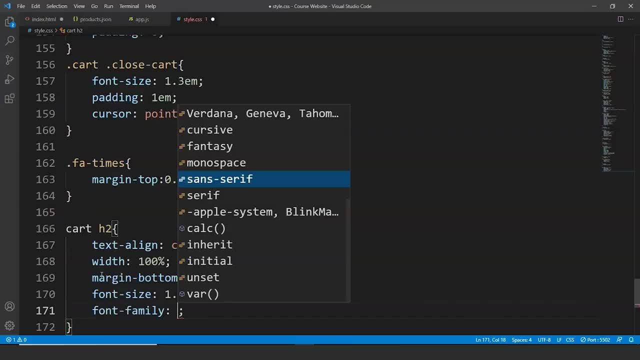 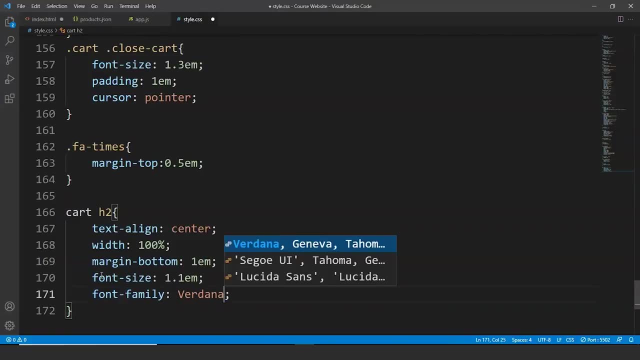 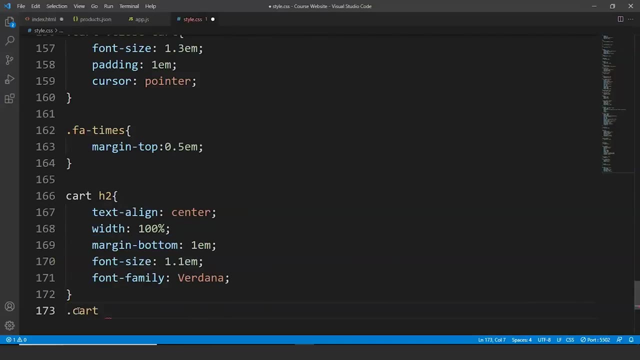 write here font family. let's use only one. fine, Let's use Verdana only. So we'll write here Verdana And next up we'll write here: dot card product space, dot product image space- img. Now we are going to write here something. Now we are going to write the code for. 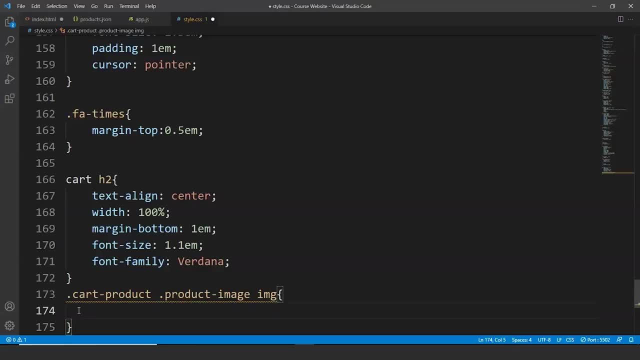 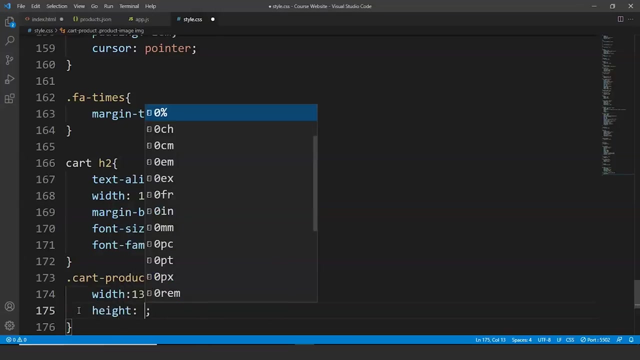 all the images present inside the card. So that's why we are writing here: width is 130 pixels Of that particular image. the width is going to be 130 pixels and the height is going to be 90 pixels. let's say, Fine, We are done with this as well. 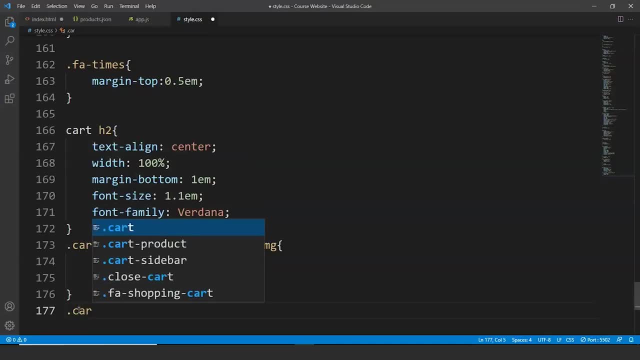 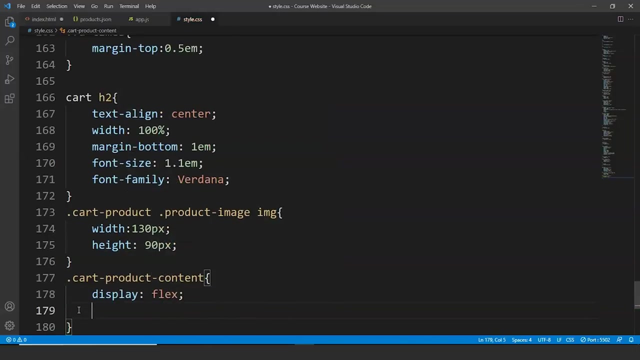 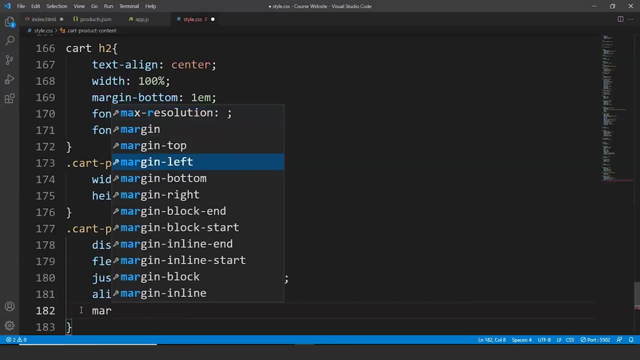 Next up. we'll write here: dot card product content. Fine, Now we'll write here: display is flex, Flex, direction is column And we have justify. content is space around and align items. at the center. We'll write here: margin left is 1 m and height is. 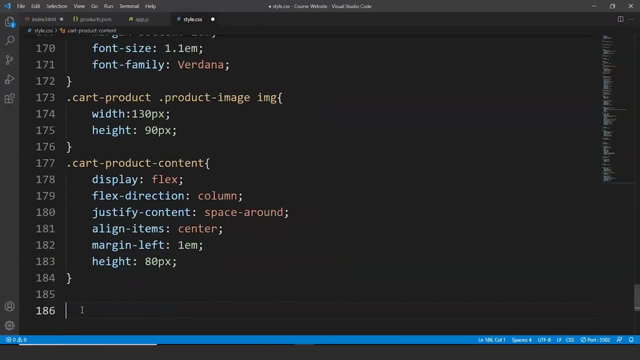 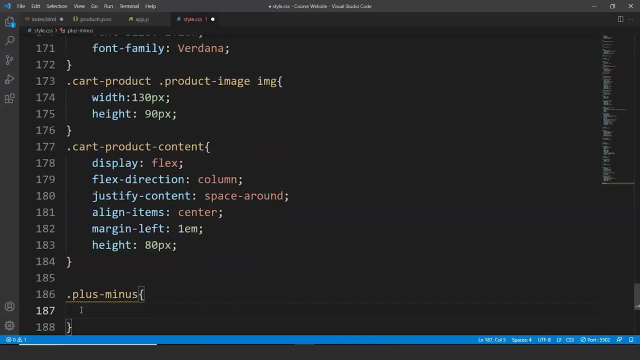 80 pixels. Fine, We are done with this as well. We'll write here: dot plus, dash minus. This is for increasing or decreasing the product number in a card cards, those arrows you must have remember, which we have seen in the website. let me show you again. so these are the arrows I'm talking about. let me. 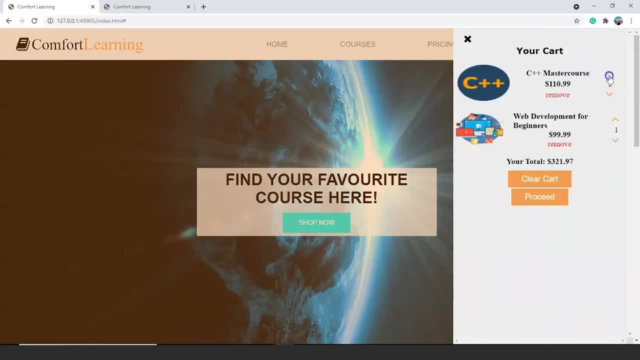 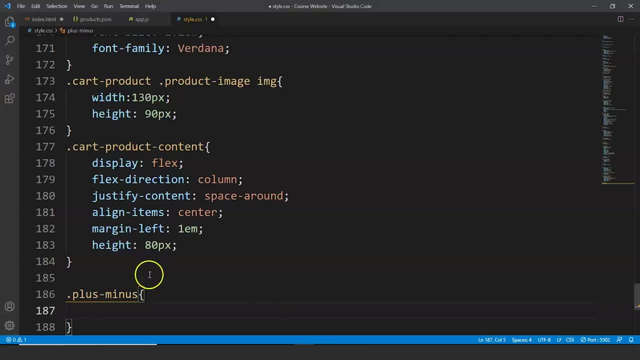 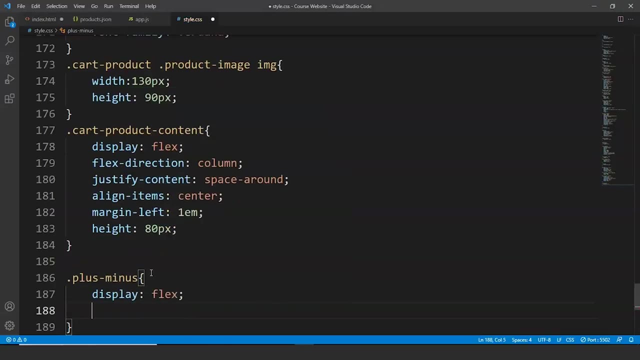 add a product now go to cart, and these are the arrows I'm talking about right now. so we are going to style those arrows as well. so we'll write here: display is flex and transform. we are going to rotate them. so we are going to write here: rotate at 90 degree. that will look cool. so we'll write here: color is: 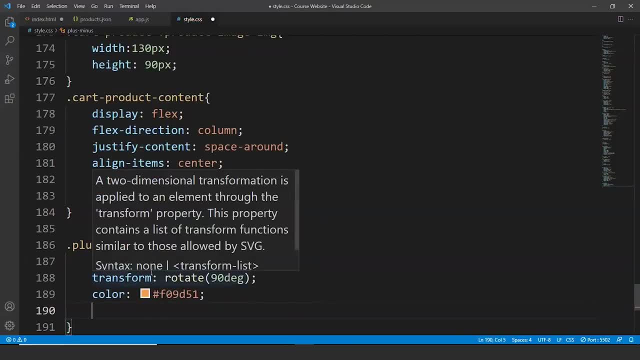 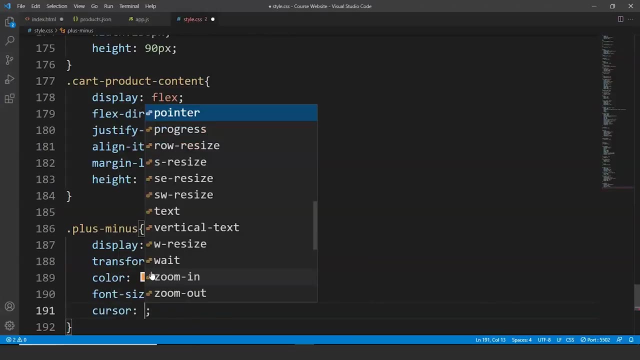 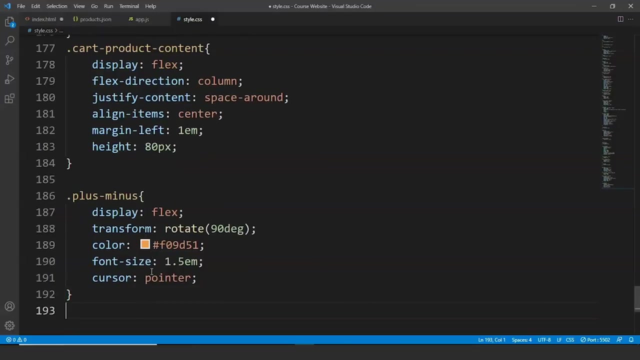 again hash: F: 0, 9, D, 5, 1. so this is the color code for a particular color. we'll write here: font size is 1.5 M and we'll write here cursor as pointer. next up we are going to do the styling for total sum, so we'll write here: total sum. 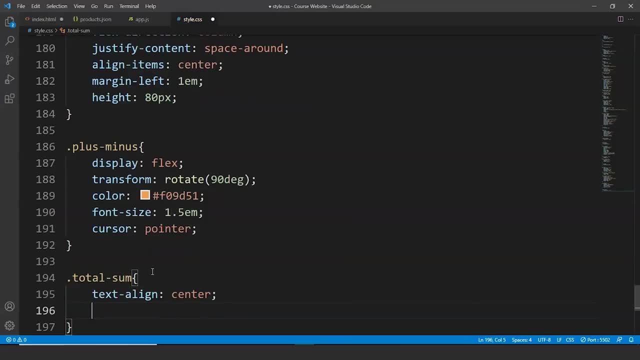 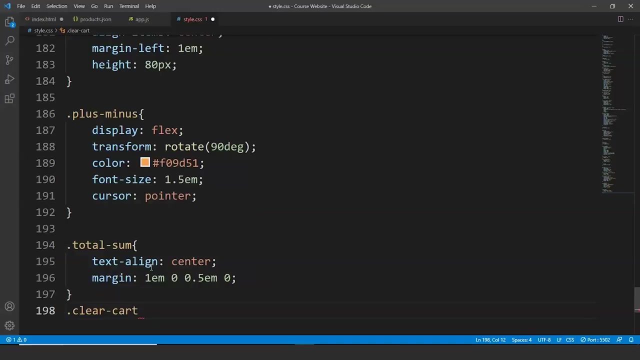 take care. align at the center and margin is going to be 1m, 0,, 0.5m and 0 again. So it's for top, bottom, left and right, everyone. So we'll write here next: clear cart text- align. 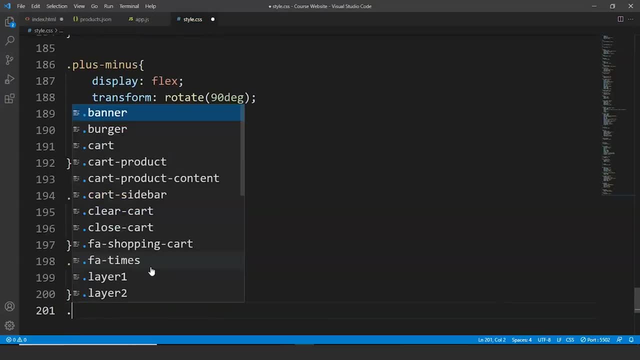 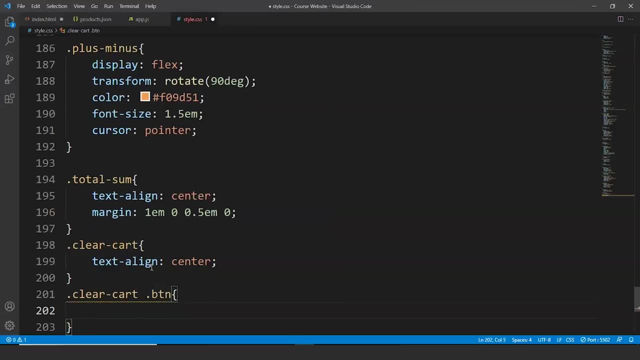 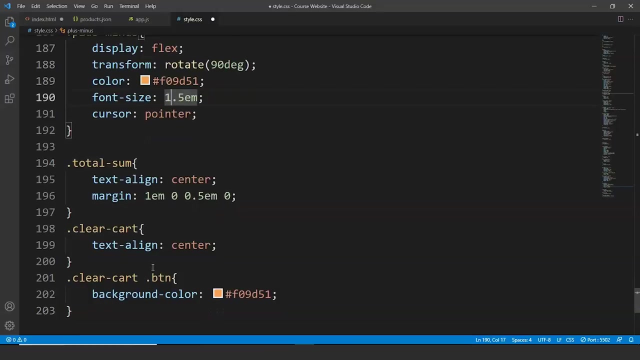 at the center and we'll write here: clear cart button. Now for the clear cart button. we'll write here: background. So background color is going to be again that same one- orange, we can say, or little bit of orange as well, and don't know the exact name for. 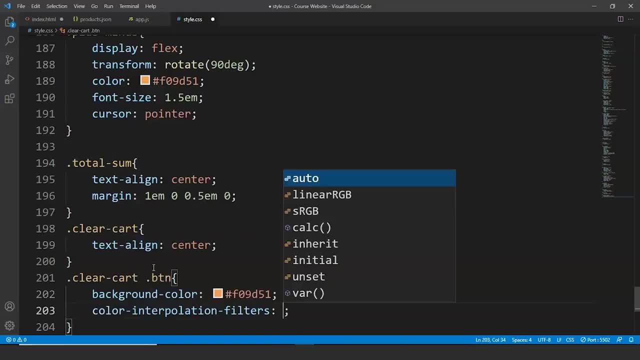 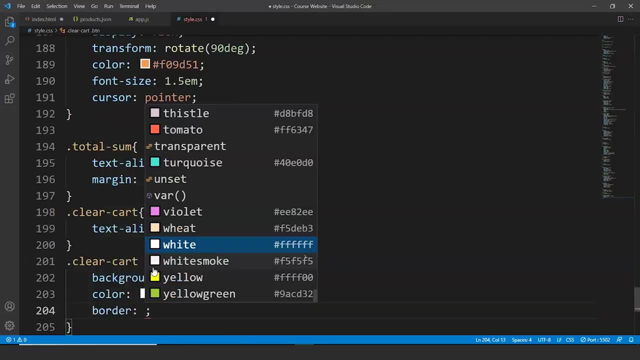 that color. but it doesn't matter, We can do anything, we can use any color. So the font color is going to be white. Okay, So the border is going to be one pixel solid and white in color for the button right. 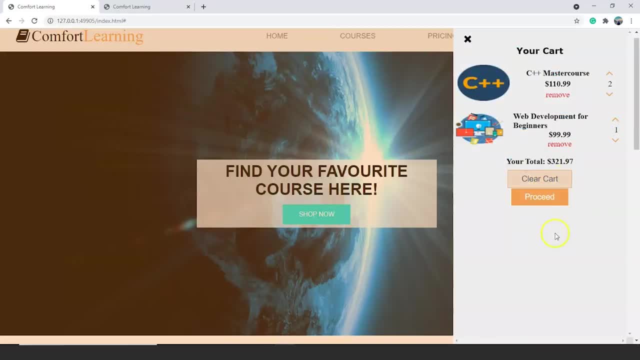 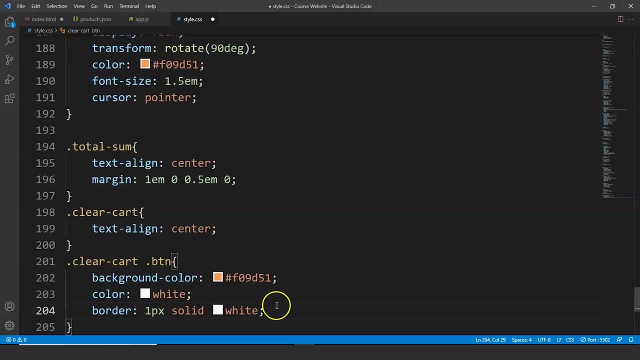 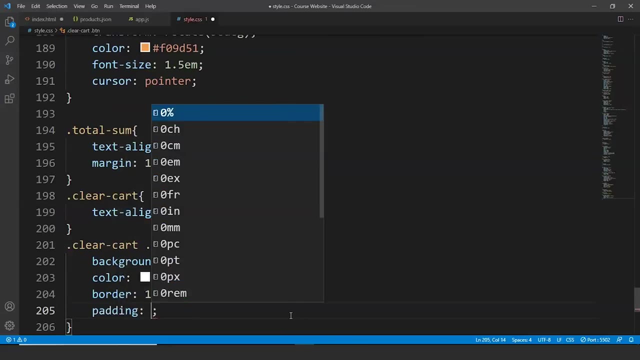 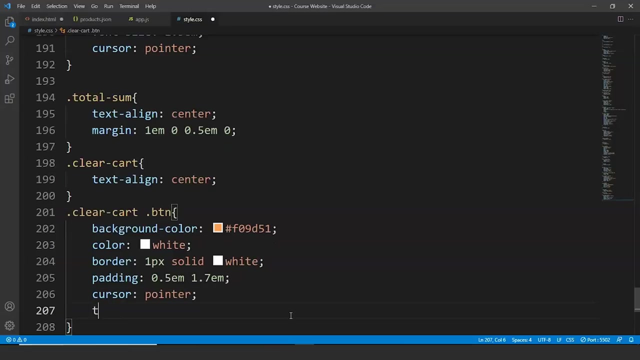 If we go back to our website and you can see here, this is our button, So we are styling this particular button. now Let's go back here and we'll write here: Padding is 0.5m and 1.7m, Fine, Cursor will be pointer and, of course, transition is going. 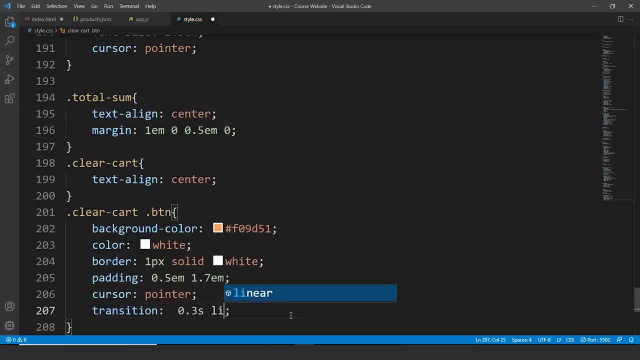 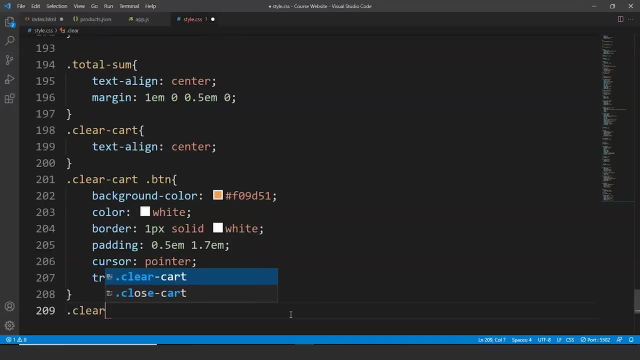 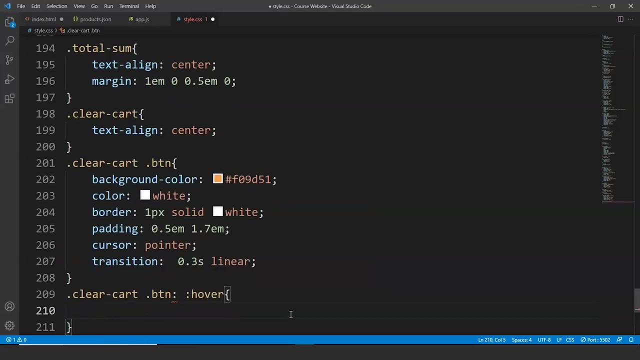 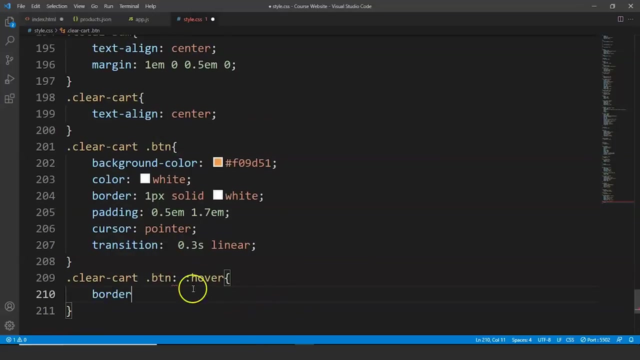 to be at 0.3 seconds and linear, Fine. Next up, we'll write here Clear cartbutton On hovering over it. what we want is we'll write here hover and we'll define the property now. So we'll write here border. Okay, We'll write here border, Border. 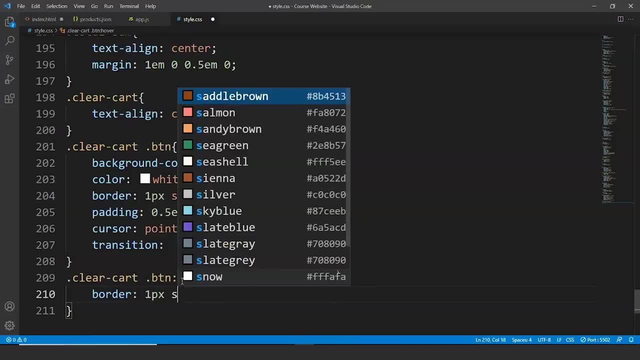 is going to be one pixel thick, solid in nature. Okay, Solid in nature, and of this color, So we'll write here: D4761E. Fine, On hovering, the color will change obviously, So we'll write here this. and now what we are going to do. 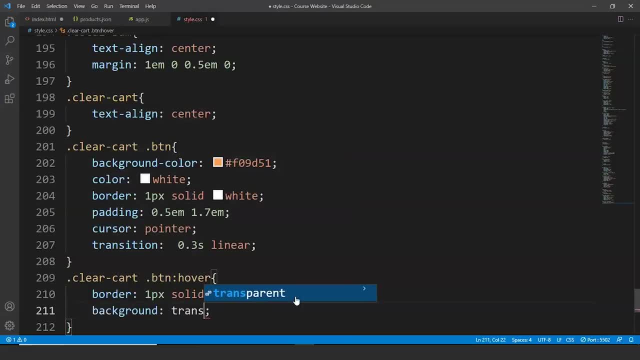 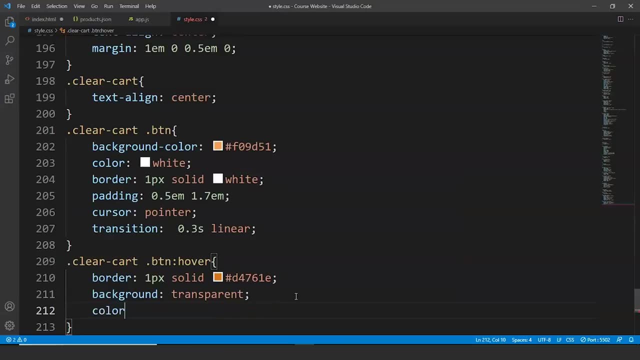 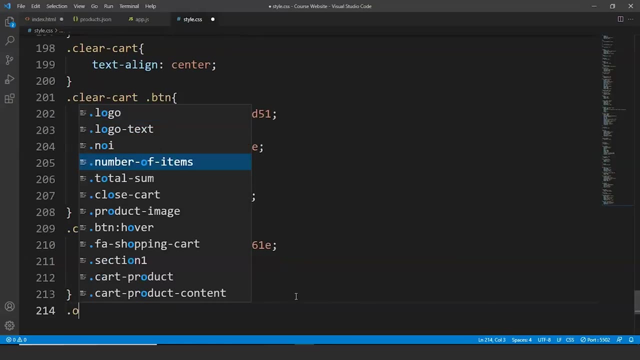 is. we are going to write here: background is transparent and color is black. Okay, So we are going to write here: background black, Superb. Next up, we'll write here: overlay For overlay. the height is going to be 100 viewport height. 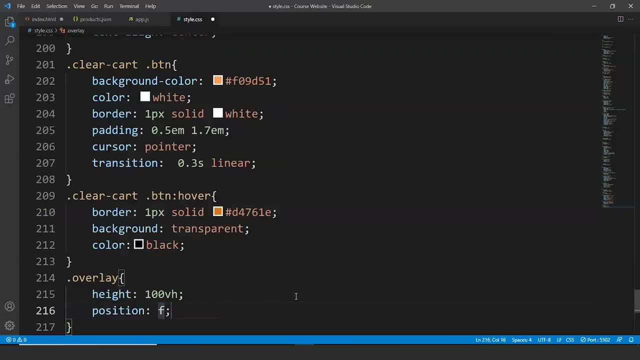 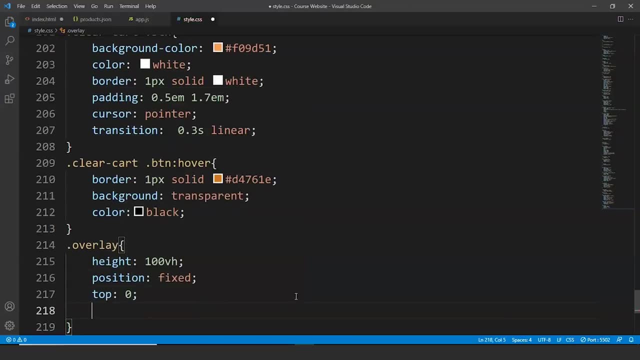 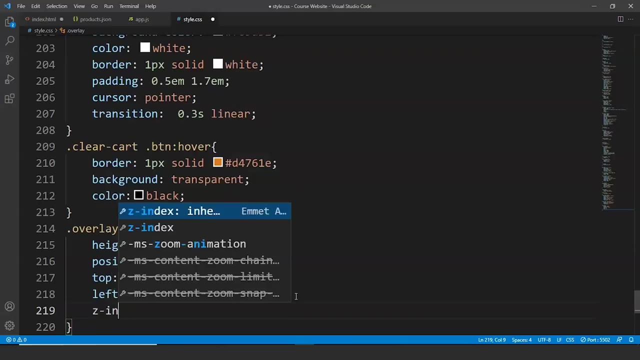 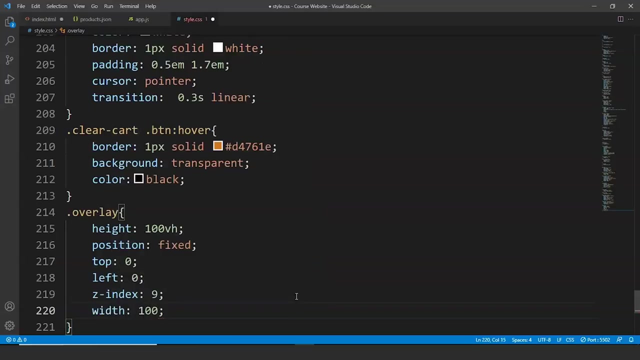 The position is going to be fixed and the top is going to be 0.. Similarly, the left will also be 0.. Okay, define the z-index as well. We will write as z-index as 9 and width as 100%. The background color. 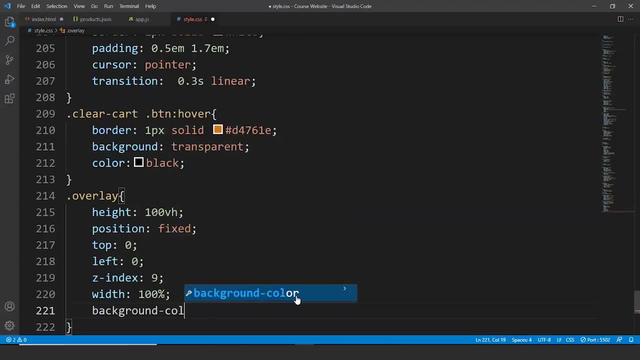 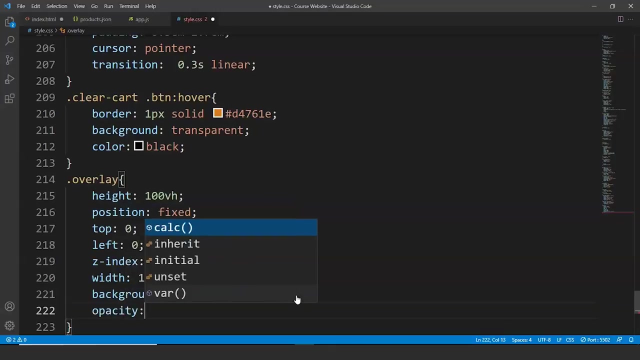 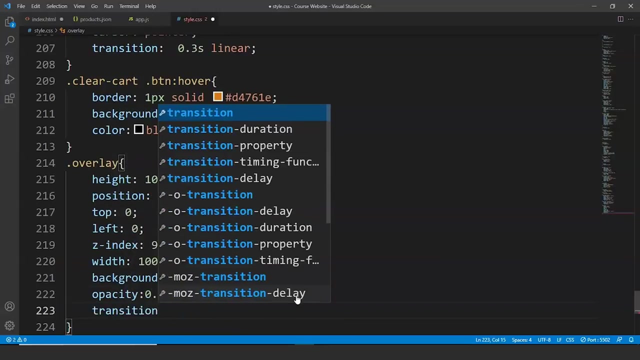 is going to be hash F3851F, So this is for overlay. We will write here opacity as 0.3 and transition is all 0.3 seconds and linear. Fine. So what we are doing is we are writing. 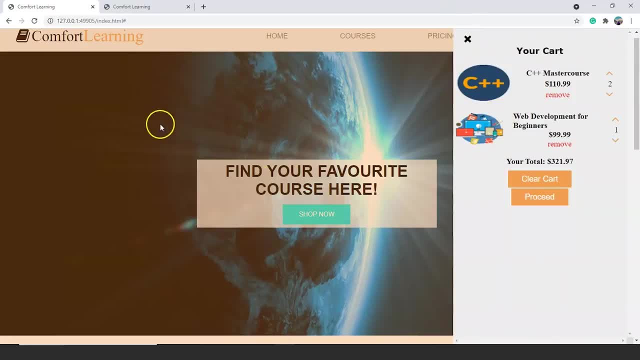 the code for this. If you open our cart, you can see this particular area or this particular field is a little bit different from what it was. It is a little bit different in color and opacity is also different. The opacity is 0.3. here We can make it fully opaque as 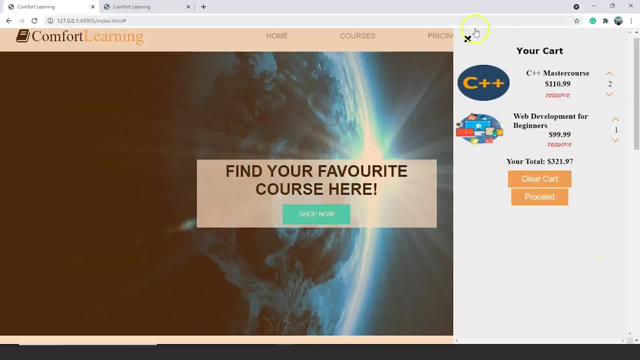 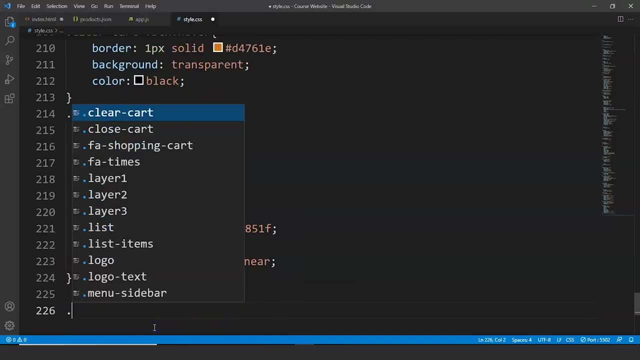 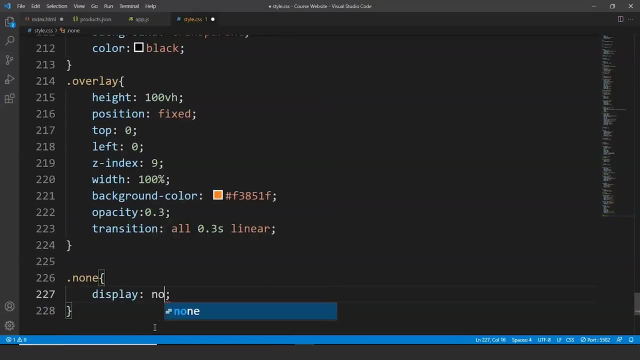 well, So for now, we will use 0.3, only Next up. what we are going to do is we are going to write the property for none. We will write here: none, Display as none. Now, what we are going to do is we: 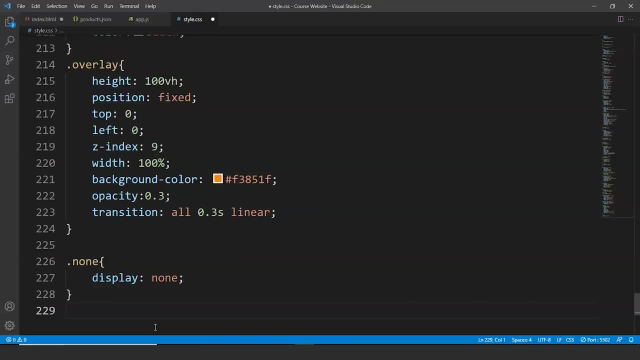 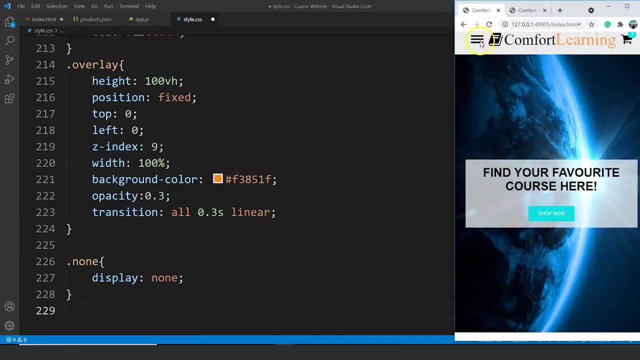 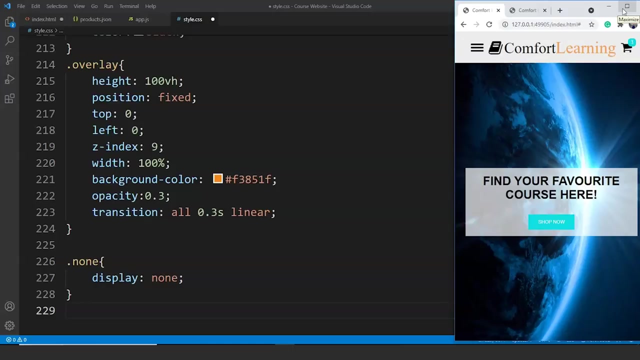 are going to write the CSS part for tablets and for mobile screens. So, if you remember that the size of this Chrome browser, the size of our website, also reduces and it becomes like this. so to achieve this, we have to write particular CSS code for tablet and for food, we have to define the max width and we have to do some. 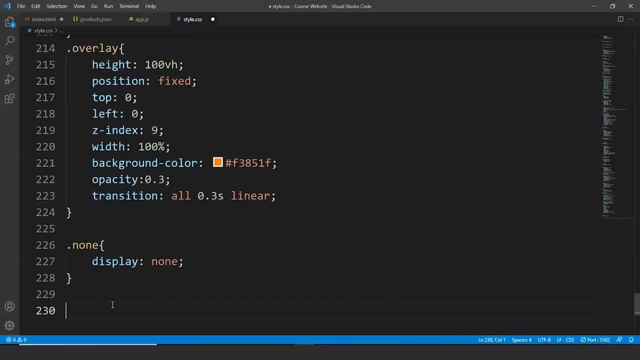 more things in there. so what we'll do is we'll write here at the rate media screen and max width is going to be 768 pixels. fine, now inside this will write dot logo. will change the logo as well. will write here: padding left is 0 and after this, we 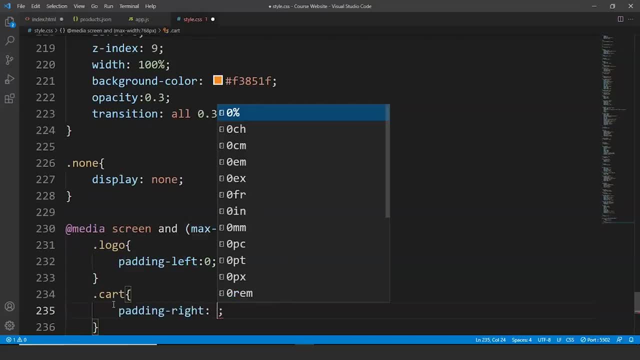 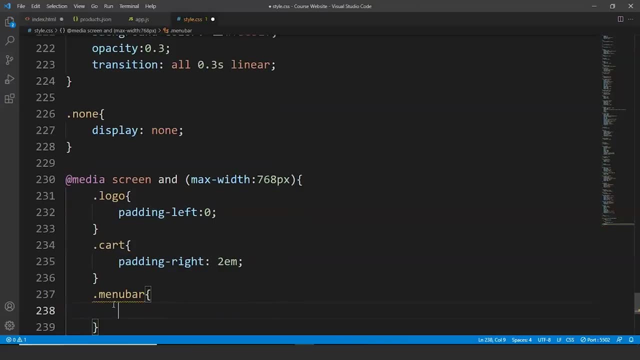 are going to write here: dot cart. heading right is 2m after cart will write here: dot menu bar. so we are going to change all the properties here, almost all the properties which we'll require. so we'll write here: display as none. the menu bar will disappear will. 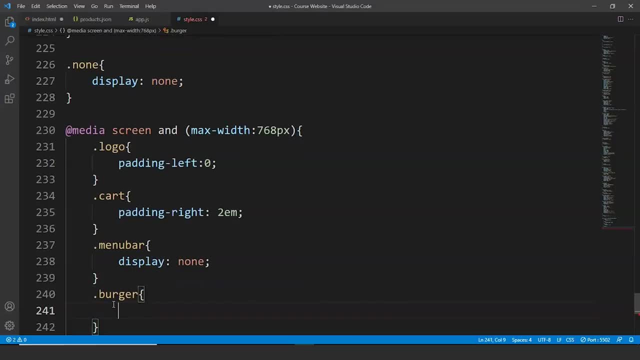 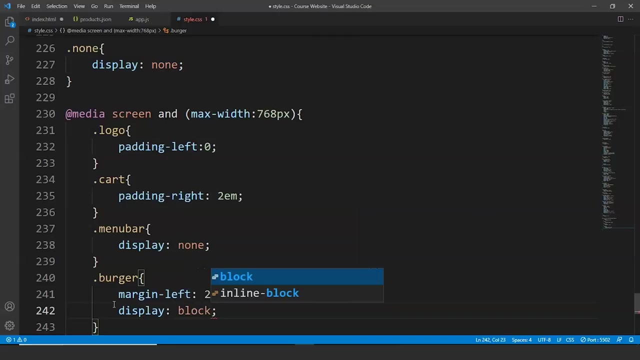 write here: dot burger. and inside this will write margin left. the burger sign will come into existence now. will write here: 2m. for the margin left for display will write here: block next up. we have to do something for section 1 and for product section as well, so we'll write here: dot. 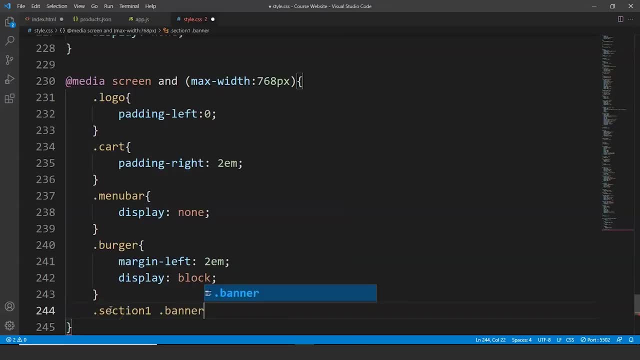 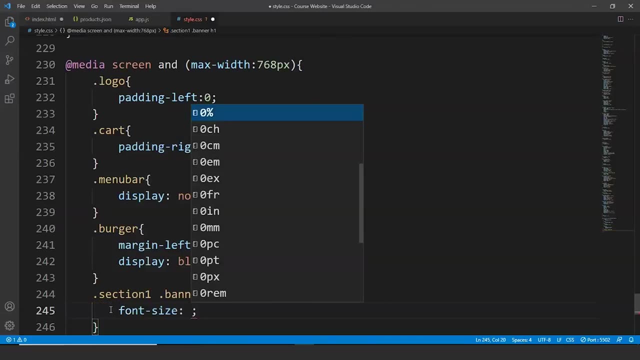 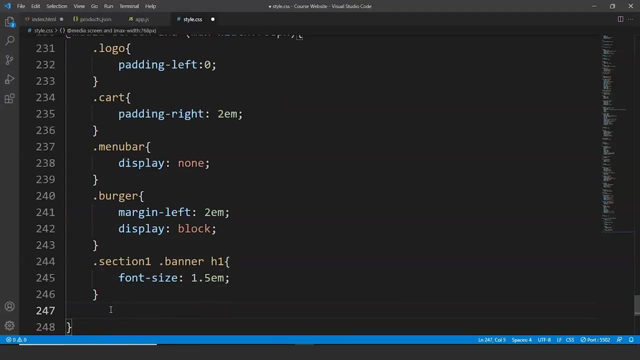 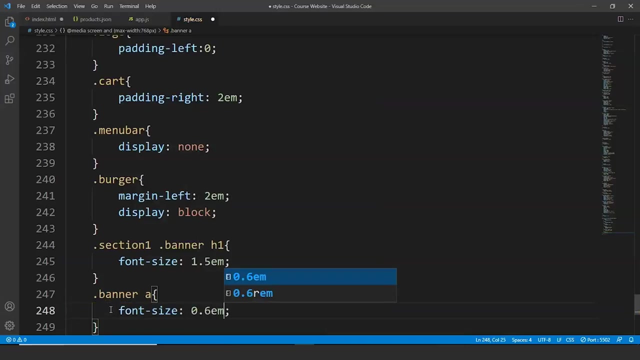 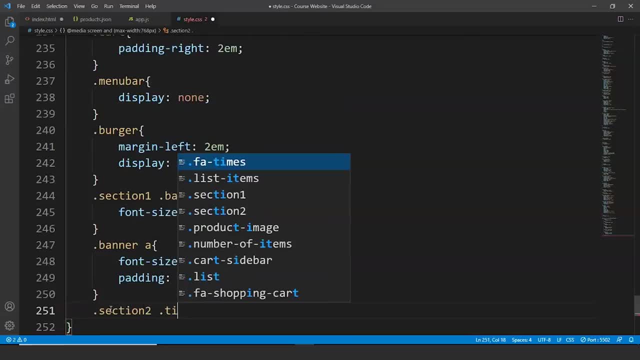 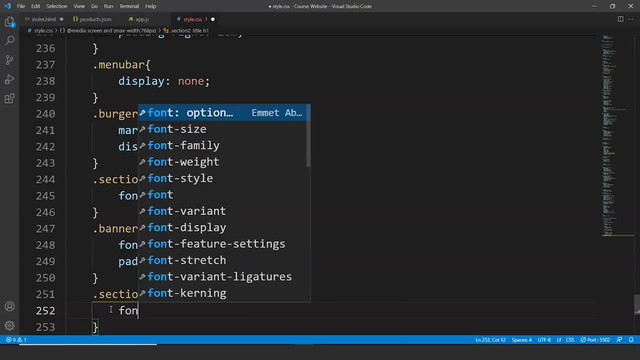 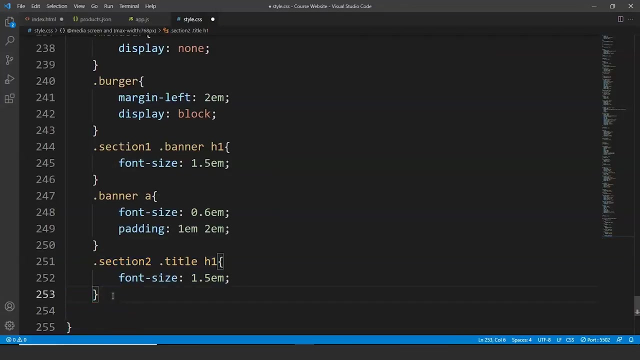 2, dot title and we'll write here h1. inside this we'll write: font size is 1.5 m. so we haven't defined the section 2 and title styling part yet. we'll define it later, but we'll write the code for that as well now, next up, we'll write: 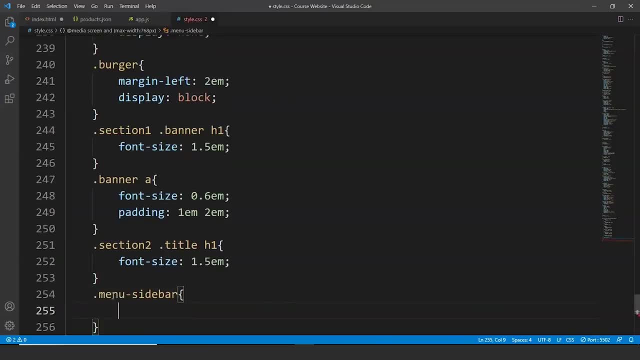 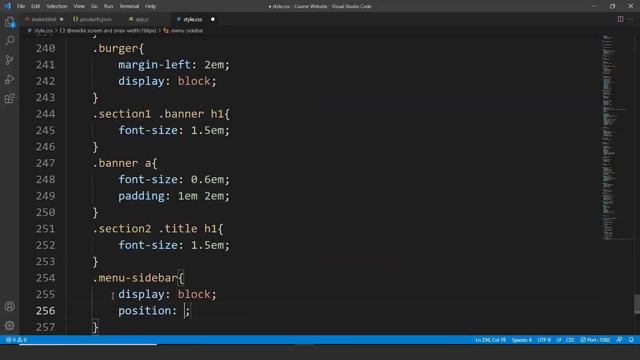 here menu. sidebar display is going to be block. position is going to be fixed, left is going to be 0, top is going to be 0. so we'll write here: left is going to be 0 and top will also be 0. then we have width is. 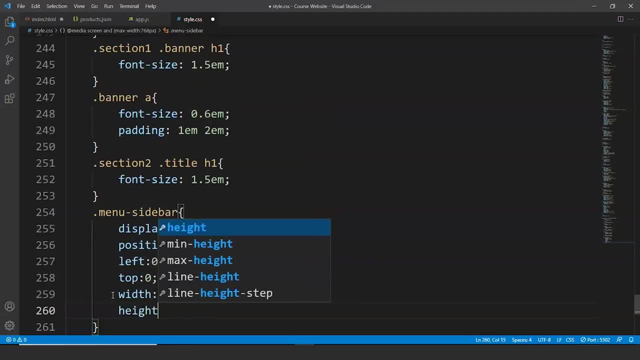 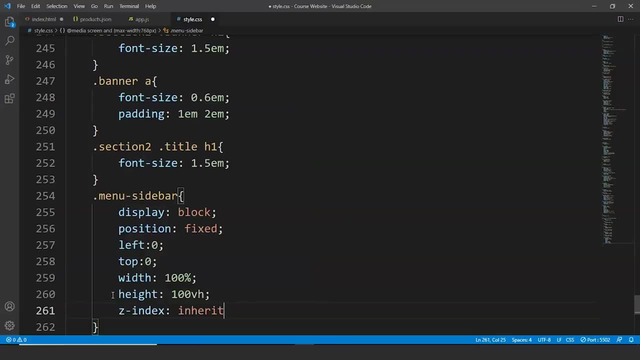 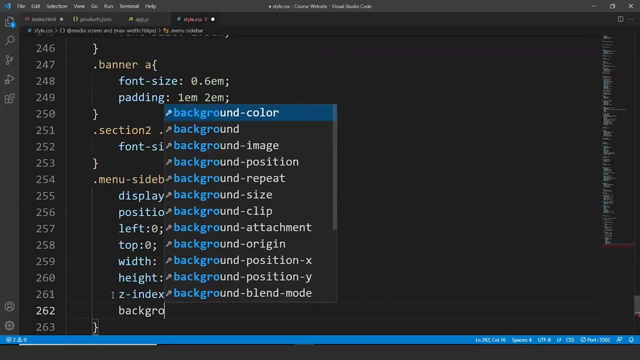 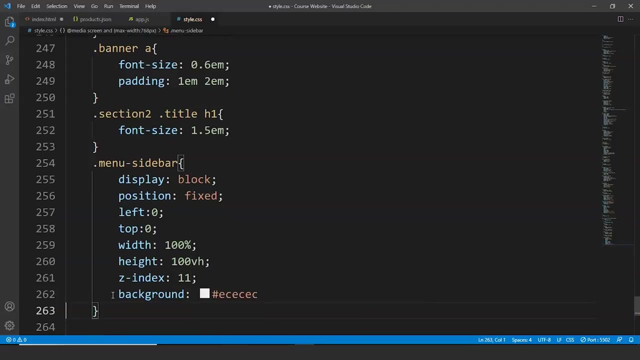 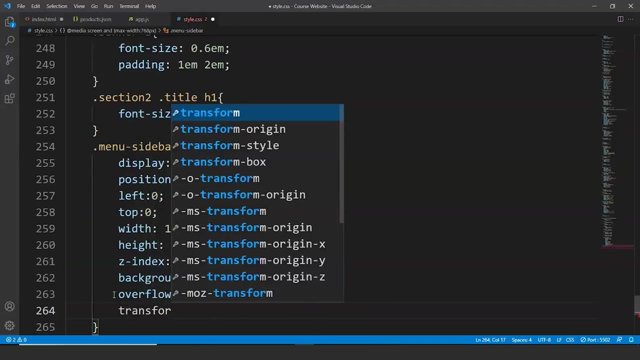 100%. width is 100%, height is 100. we put height and z-index is 11. background is going to be gray again. so we'll write here: ec, ec, ec. then we'll write here: overflow is 초 Mäd Turkey, 스펀erd. 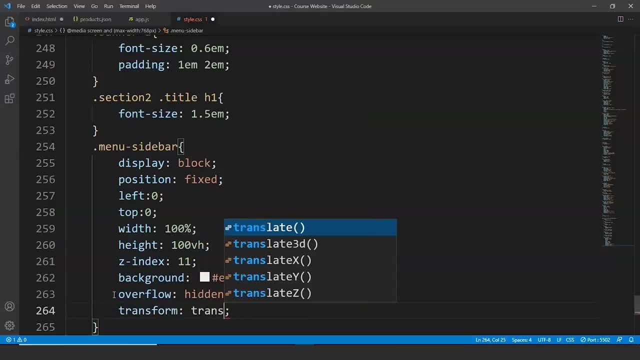 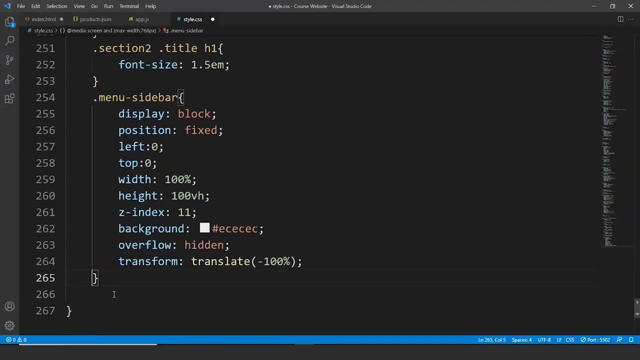 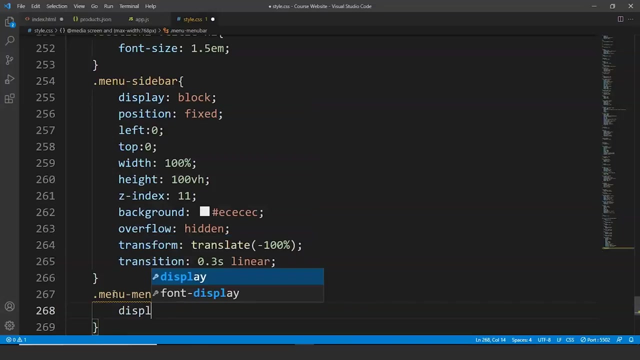 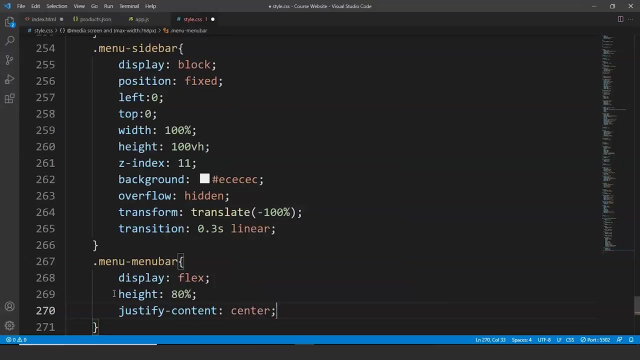 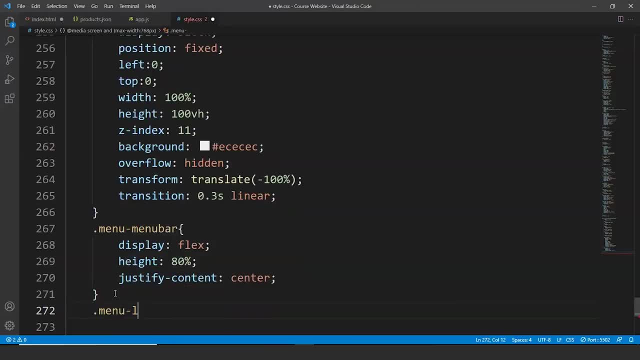 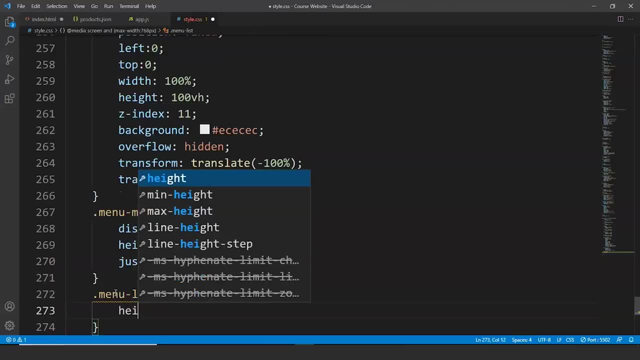 done so. next up, we'll write here: menu list. we'll change the style of menu list as well, so we'll write here: height- height is going to be 100%. then we'll write here: display as flex. we are rewriting the code again and again, but 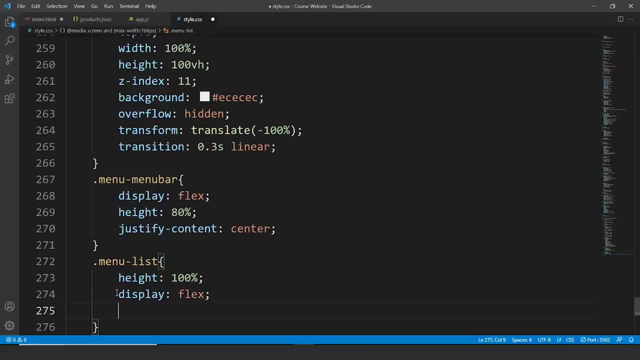 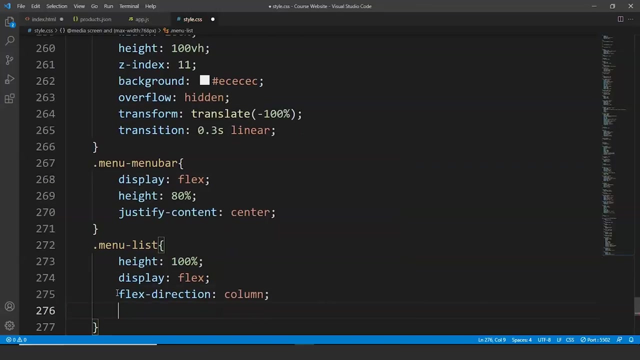 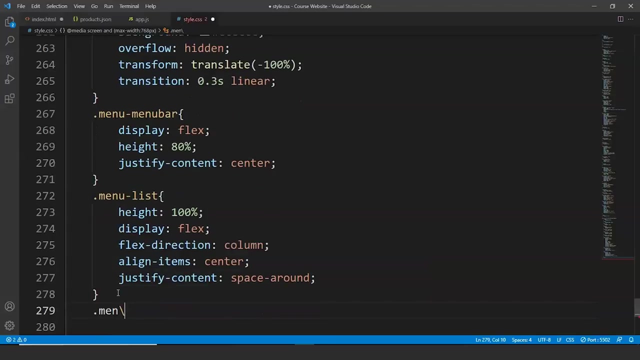 each time we are doing it for different class, we are doing it for different element. so keep these things in mind and we'll write here: flex direct as column, align items at the center and just defy content, justify content as space around. now it's time to do it for menu sidebar, for menu sidebar and for. 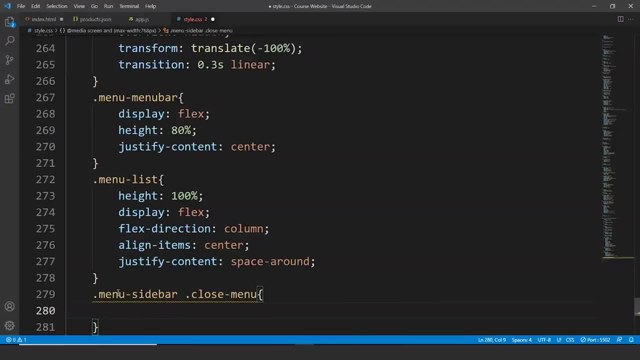 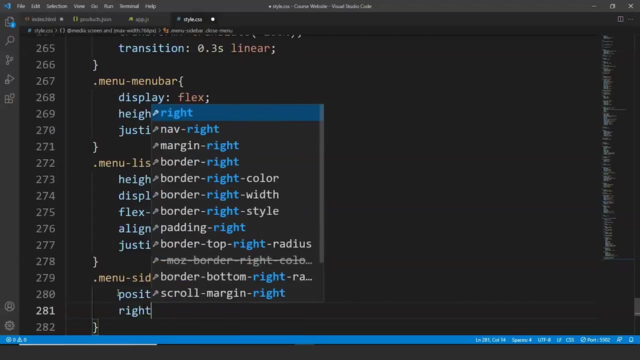 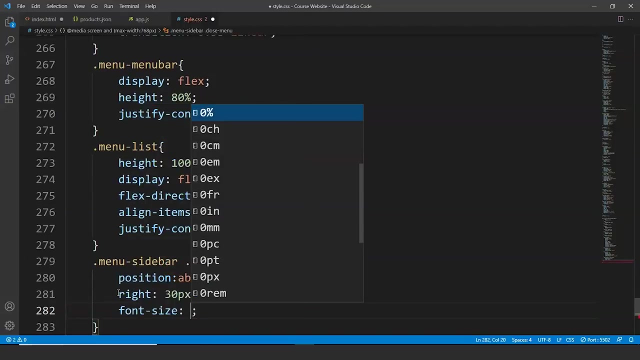 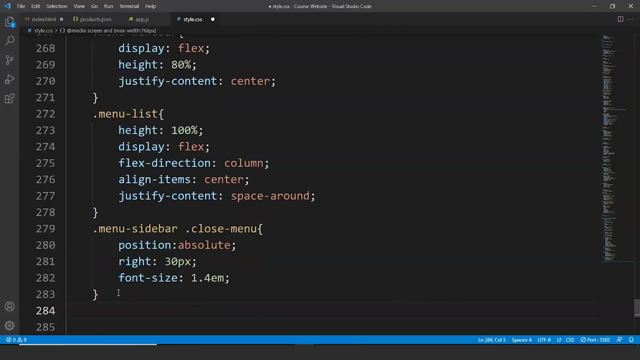 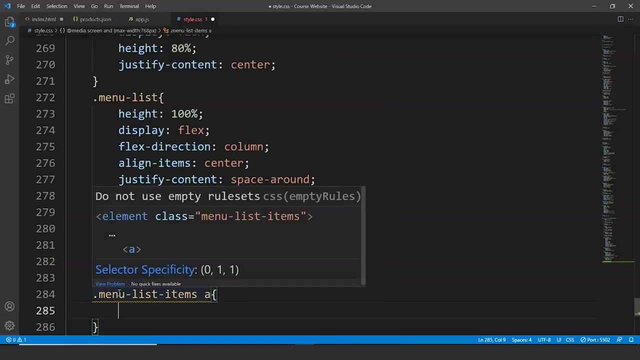 close menu. both will use the same styling properties. you we'll write here: position is absolute right is going to be 30 pixels, font size is going to be 1.4 m and after this we'll write dot menu list этому з. we'll try it here. color. 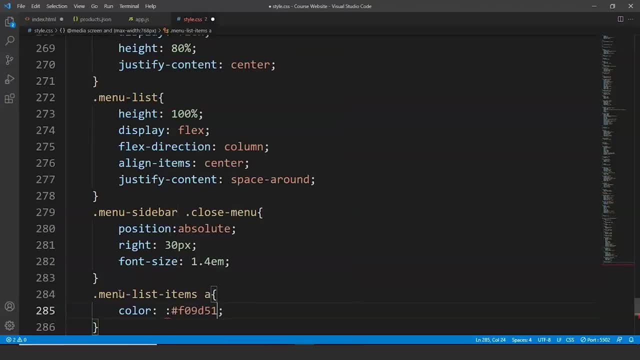 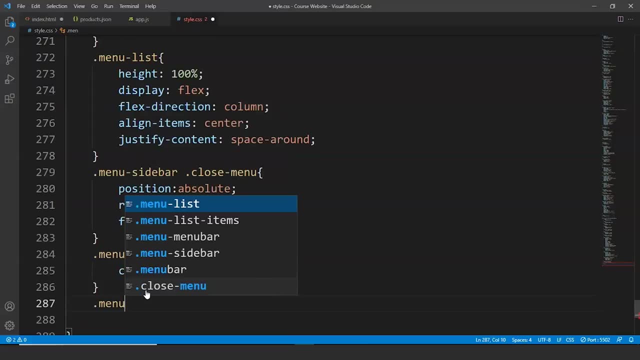 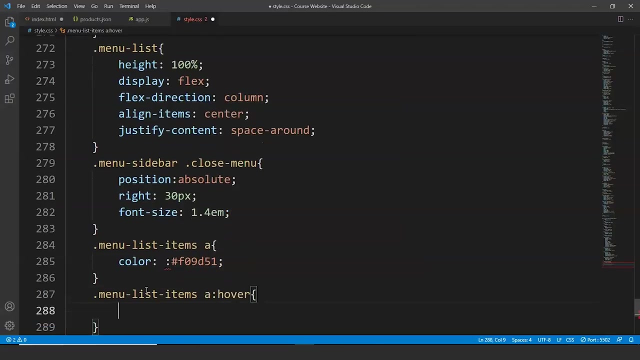 is ash F 09 d51, the default color we are using till now. and lastly, will write you dot menu dash list items, space a on 것 power button and then we'll type in color finish希望 for this. now it looks good over. we'll write here: color is ash F57B09- fine, so here's a mistake we have placed. 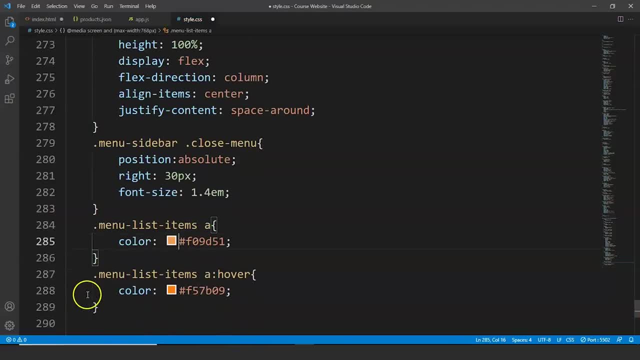 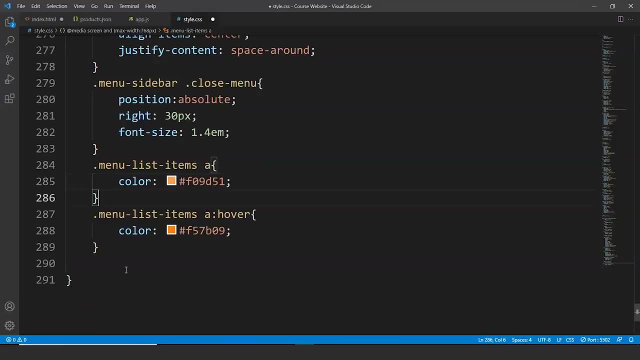 colon here twice, we'll remove it. and now we are done with the tablet part. so we have to change the style of almost all the elements. we are done with the tablet part. next up, we have to write the same code for mobile part as well and we'll. 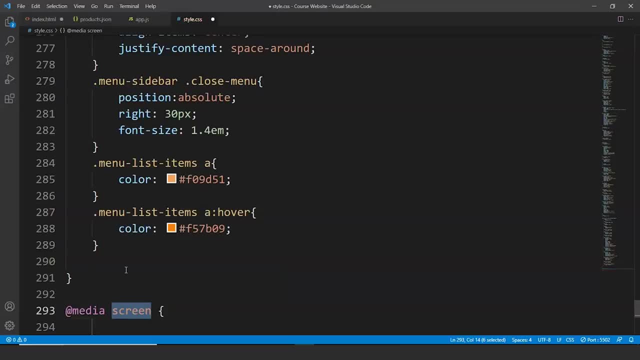 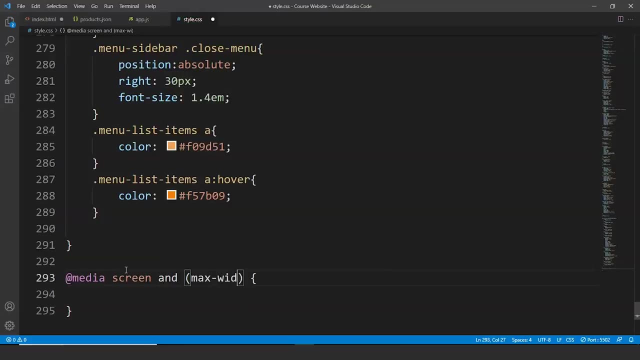 write here at the rate media screen. so we'll write here, and max width is going to be 480 pixels. now what we'll do is we'll write here. a strict font size is going to be 16 pixel here. we have changed the font size for the whole. 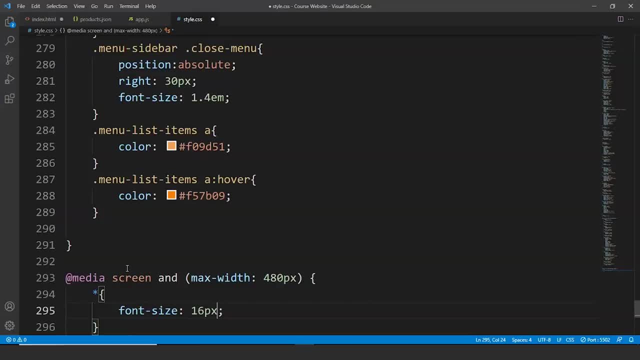 entire HTML document. we have done it because we have used M in place of rem or pixels in this case, or in this video. so that's why we have changed the size here, because we want the screen to be smaller in size. right, if we go back here. 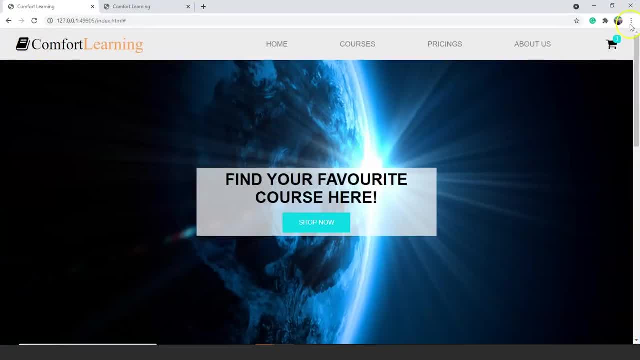 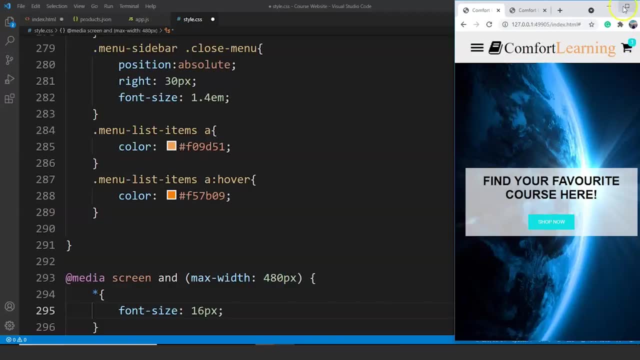 you can see, the font size is 16 by default and if we do it, you can see the font size changes for each and every element right to achieve this. so if we wanna make this really nice, we have to use M in place of pixel or rem. we can say: 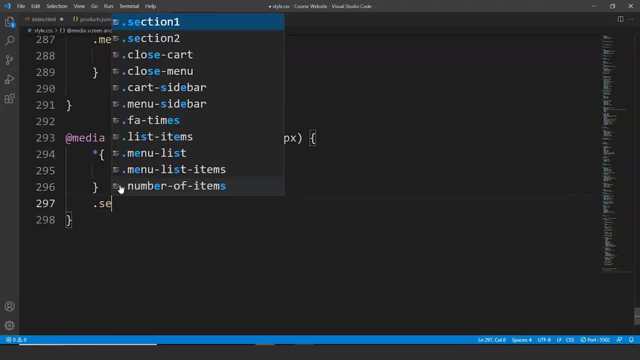 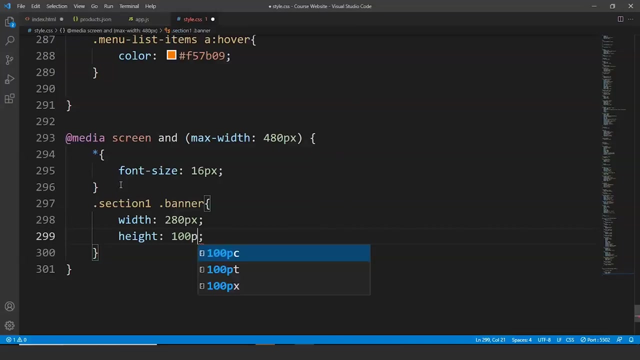 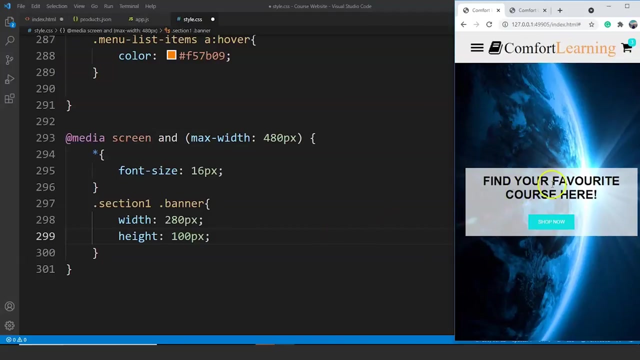 now the next thing we are going to do is we are going to write here section 1, dot banner, and we'll write your width as 280 pixels for both and we'll write your height: it's hundred pixel. fine, you can see here, the height of this image is 100 pixel, or we can say the: 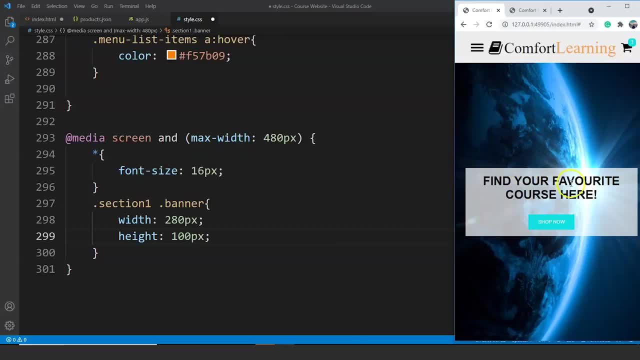 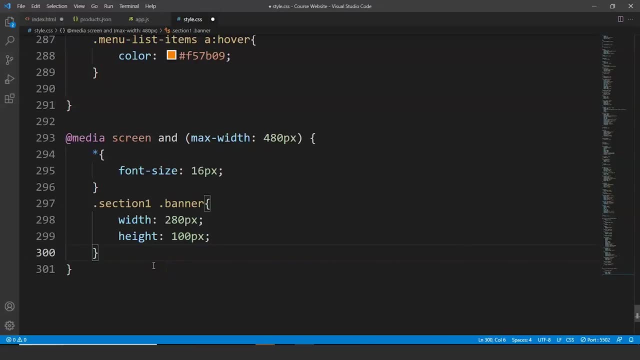 height of this banner is 100 pixel and the width is 280 pixels. so this is why we are changing the style of all these elements, because we want all these elements to fit inside a smaller screen. that's why we have to change the height, or we have to change the width as well. now what we'll do is we'll write here: 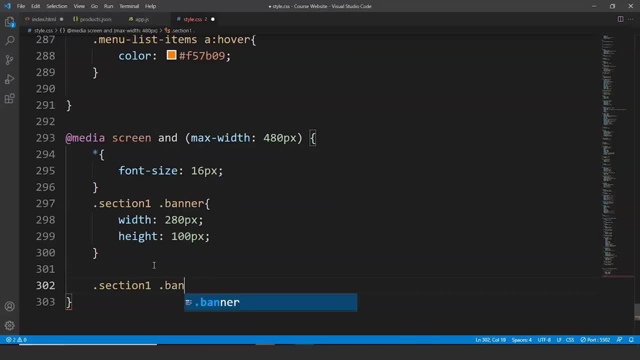 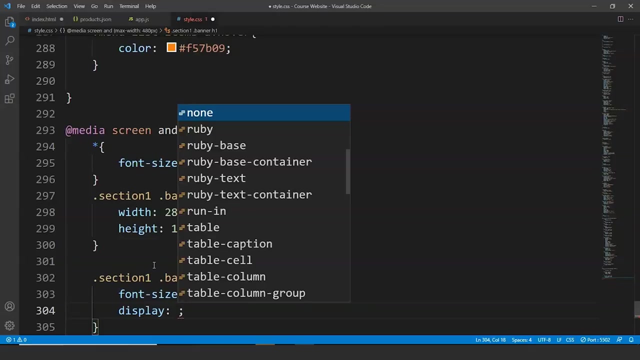 section 1: dot banner will write here h1. inside this will write font size as 1.2 m display is going to be. now we don't have to use display here. I guess let's leave it. so we are done with this. next up we'll write the code for burger: we. 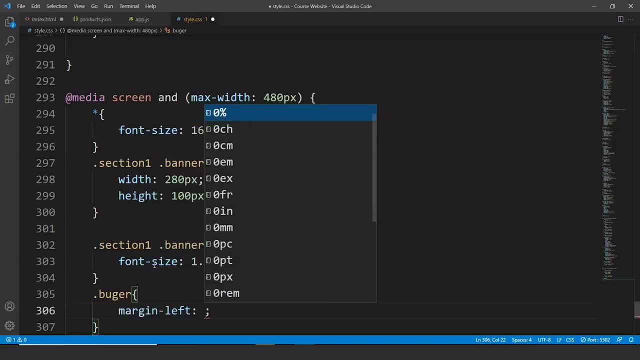 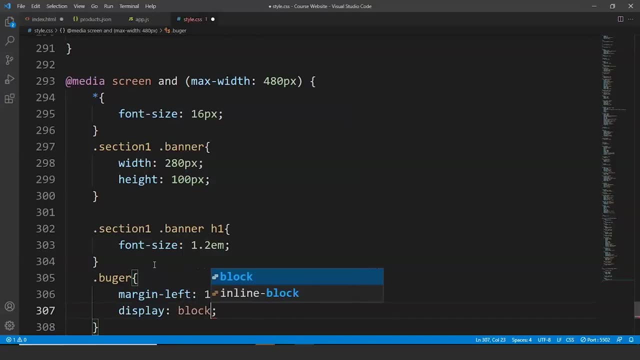 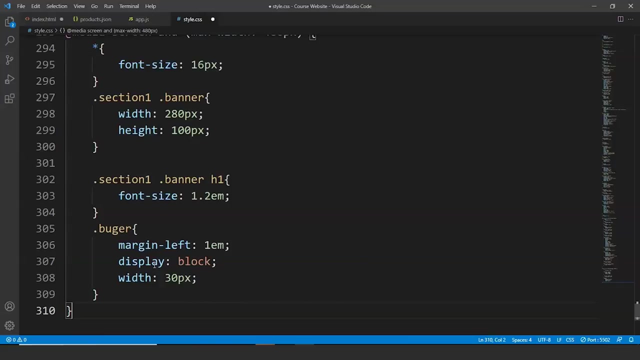 will write here: burger margin left is going to be 1 m for mobile. for mobile, the display is going to be block and the width is going to be 30 pixel. fine, we'll do the same for cart sidebar. will write here width as 100 percent. 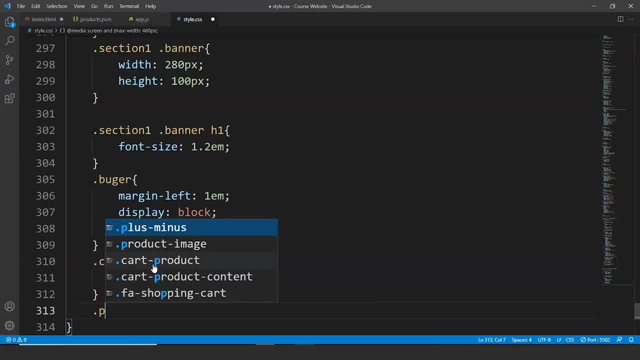 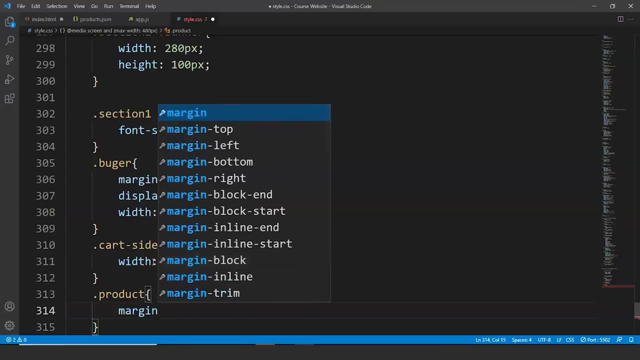 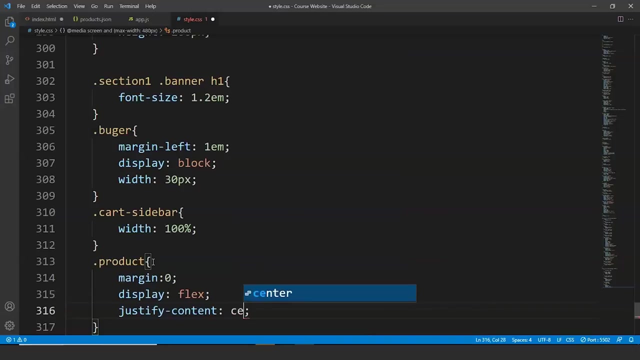 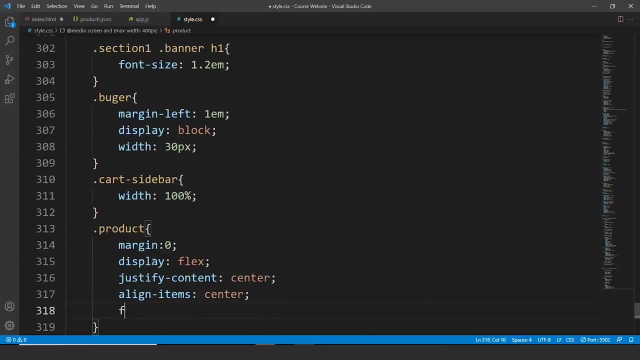 of the screen. the cart will take whole screen and we'll write here at the last for product. so for product will write here: margin is 0, display is flex, justify content at the center, align items at the center and flex direction is going to be column. so we have covered all the features of the product, so let's. 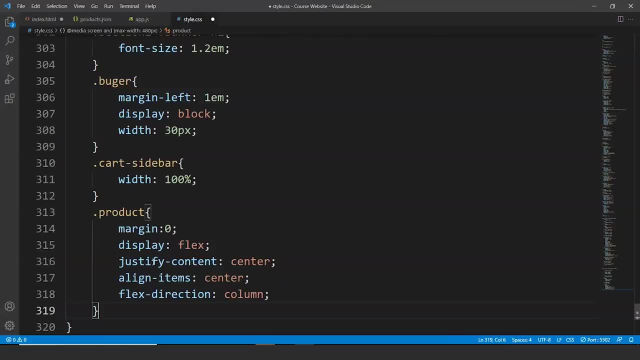 move on to the javascript part now and see how we can fetch those products. so we cannot witness every style change right now, but we'll witness them while covering the javascript part. so let's move on to the javascript part first and we'll start with the cart section and the hamburger menu thing. so save it and if you want to witness, 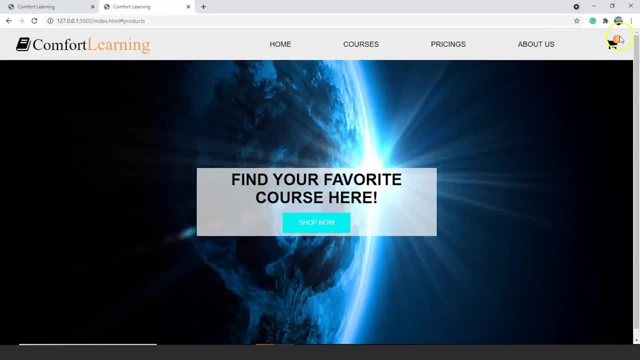 the changes we made. you can go here and you can see the cart is not opening because we need to write the javascript part for that and everything else remains the same. if we reduce the size of our browser, you can see. we have a menu over here. we can increase the. 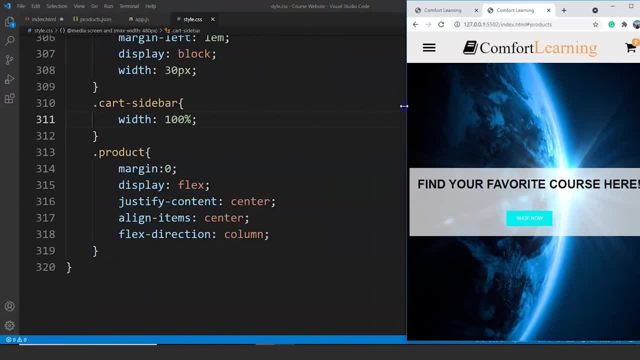 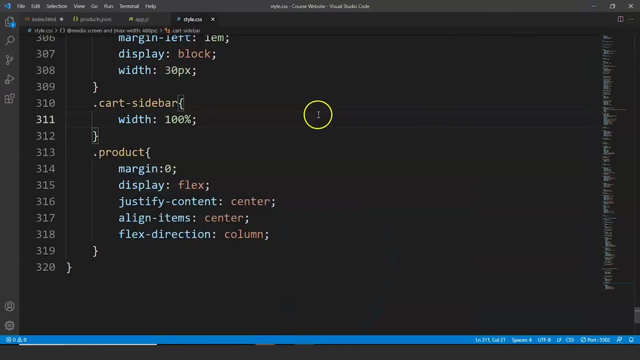 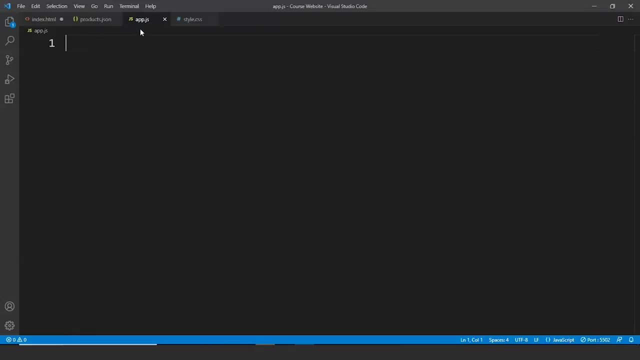 size and we have our image adjusting itself accordingly. so we can use it and it's quite responsive as well. let's move on to the javascript part. now we'll open the javascript file and first of all, we'll access all the HTML elements with the query selector method. so we have several. 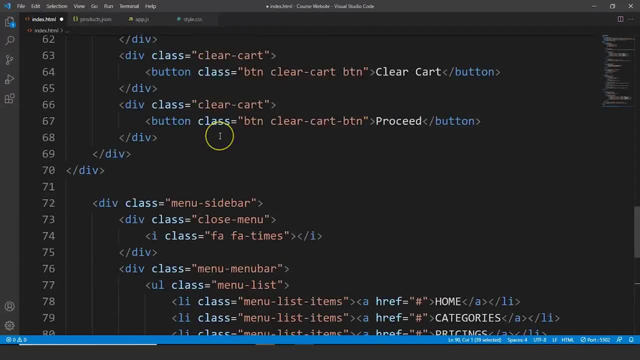 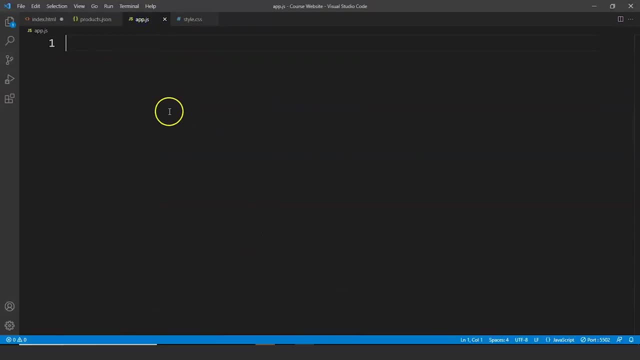 HTML elements. right here you can see we have several elements present in our HTML file. we are going to access few of these elements, so what we are going to do is we are going to write here: const cart is equals to document dot query selector. we are going to write here: nav space dot cart. then we are going. 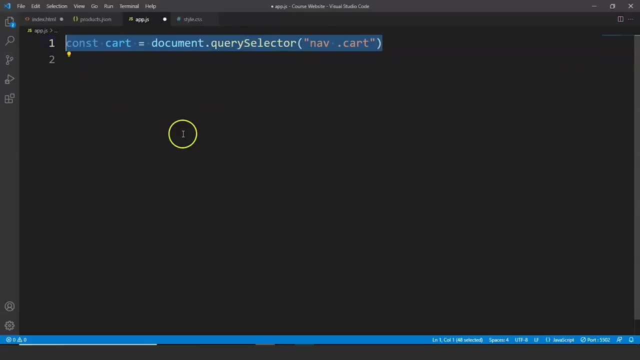 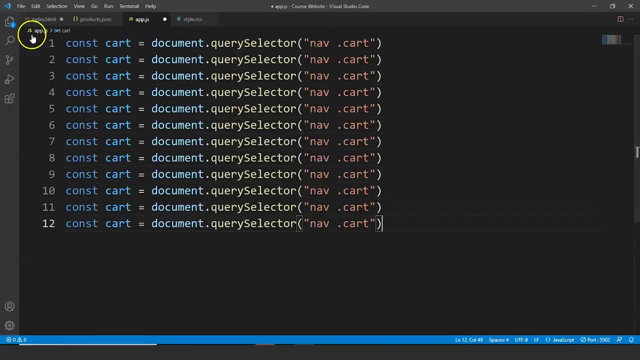 to do the same for a long time. so what we are going to do is we are going to copy paste this piece of code again and again for several times. we are going to change the name of variables, so we'll write here: dot cart sidebar. and instead of this, we'll write here: 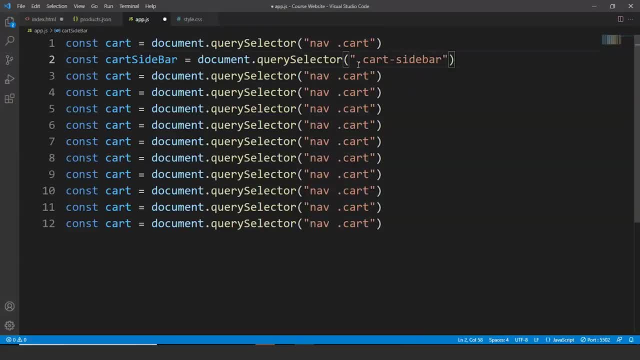 dot cart sidebar. and the next one: we'll write here dot close cart and here the variable name will change to close cart. fine. next up we'll take another variable else, burger, and here will change the query from nav dot cart to dot burger, fine. next up we have menu sidebar. so we'll write here menu sidebar and here what we'll do is. 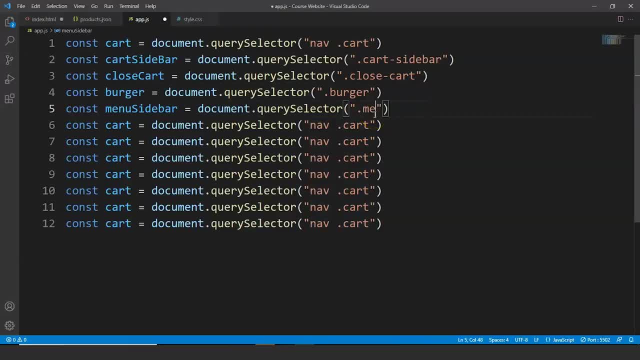 we'll write here dot menu sidebar. here, fine, next up we have close menu and here we'll write close menu. again after close menu we have cart items total, so we'll write here cart items total and we'll use noi. then we have total amount as well, so we'll write here total amount and here we'll write cart price. 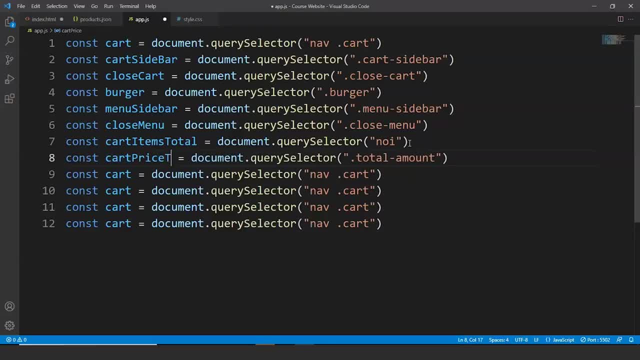 total. we have to access a lot of elements. so then we'll write here cart ui and for this we'll access cart, sidebar and cart. so we'll write here dot cart, sidebar, space, cart. fine, then we have the total sum. so we'll write here total sum. we'll put a dot over here. 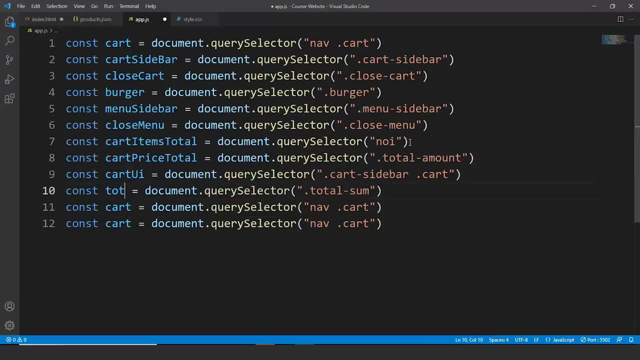 and here we'll write total div. then we have the clear button, so we'll write here clear button, and here we'll write clear cart button. then, finally, we have variable name, cart content to access everything present in the cart. so we'll write here dot cart and here we'll write: 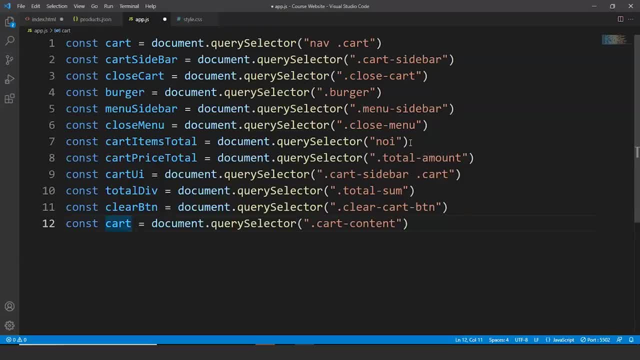 content. here we'll write cart content. so these are our 12 variables and we have accessed almost every element present in a html file which we are going to need further. so i hope you guys understood this. we have used the query selector method to access all the html. 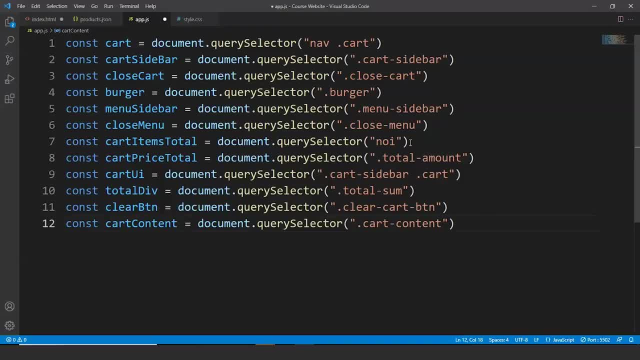 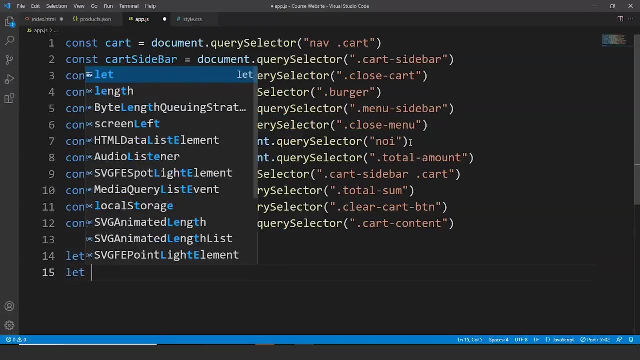 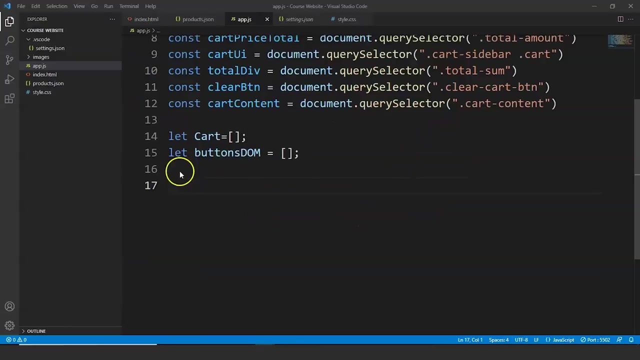 elements here in the javascript part. now next up, we'll take two empty arrays, so we'll write here: let cart is equals to an array, and we'll write here: let buttons dom, and it's again going to be an array. fine, now we'll first create some events to open and close the cart. 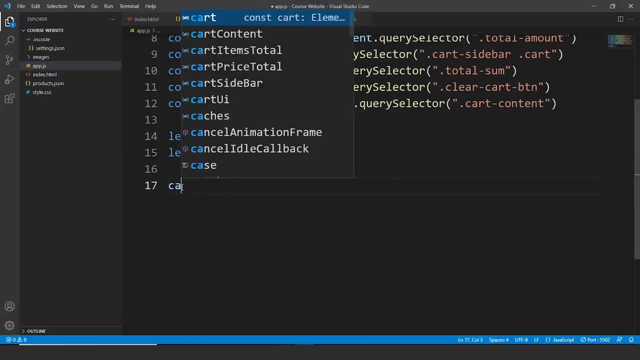 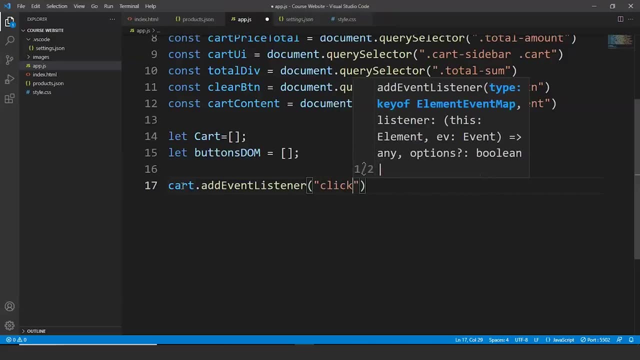 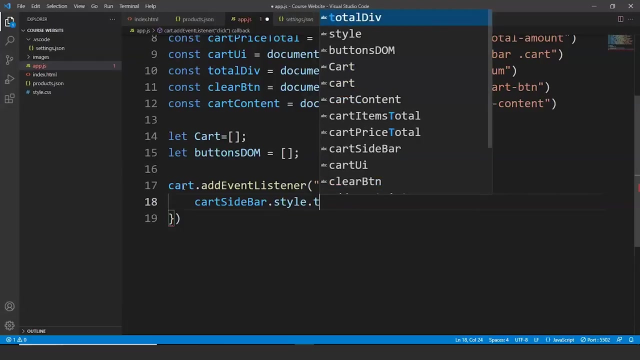 for that. we'll write here: cart dot- add event listener. we'll write here: add event listener. add a click event here. and we'll write here: function. now inside this, we'll write cart dot. will write cart sidebar dot. style dot: transform is equals to translate 0%. fine, so this is. we are changing the style of cart. 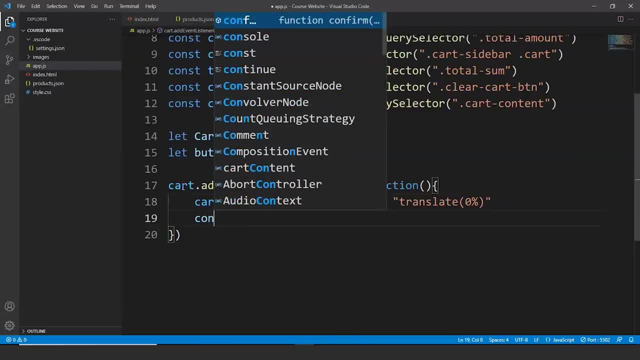 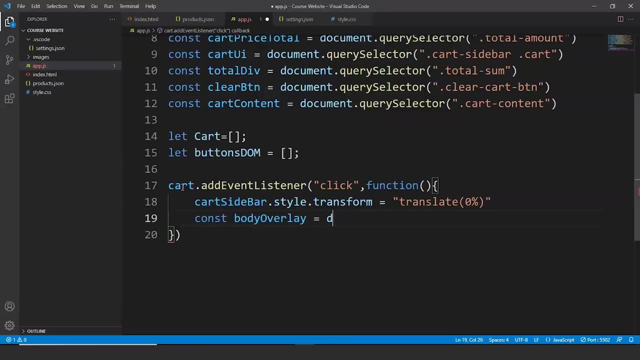 sidebar. next up, we'll write here: const body overlay. we'll take a variable of named const body overlay. we'll write here document dot- create element. and we'll write here div inside this fine. next up, what we'll do is we'll write here: body overlay, dot. 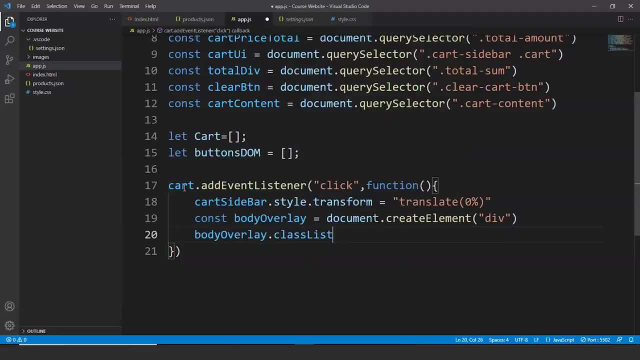 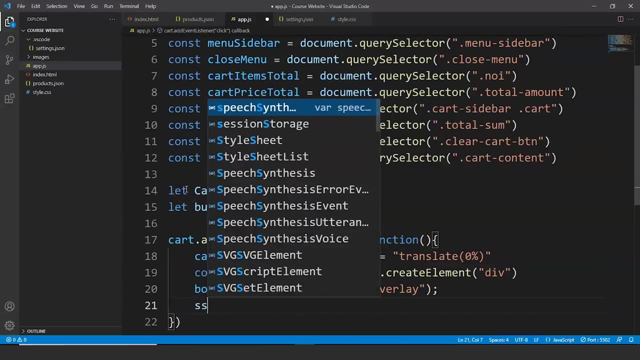 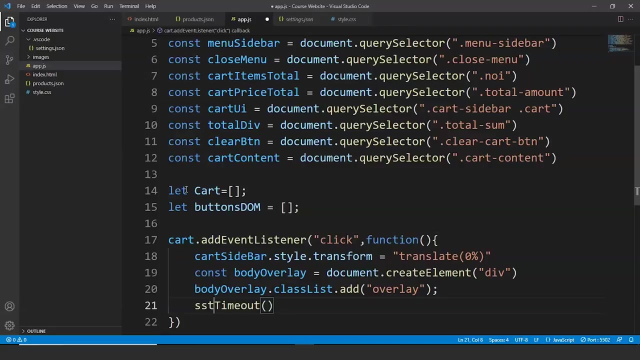 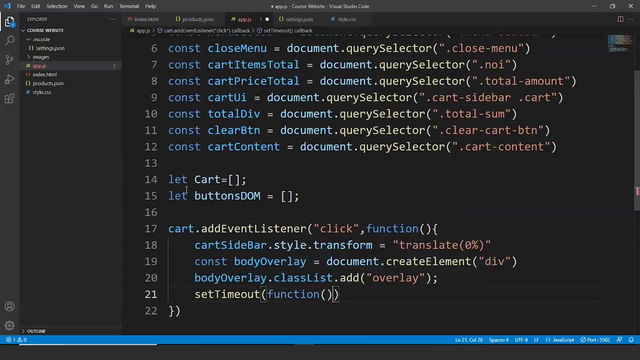 classlist dot add and we'll write here: overlay. fine, we'll use the set timeout method, so we'll. we'll use the set timeout method, so we'll write here set timeout. ok, we have written here sst, so we'll write here: set timeout. then we'll create an anonymous function and inside here what we'll do. 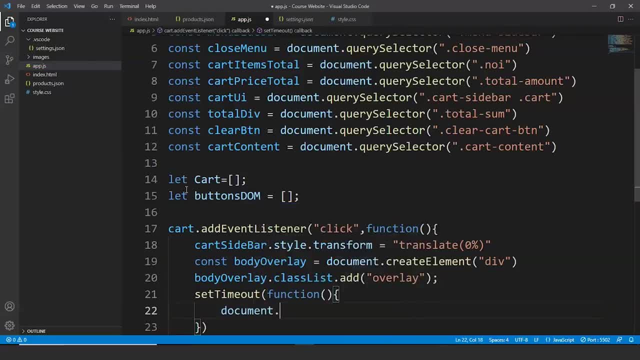 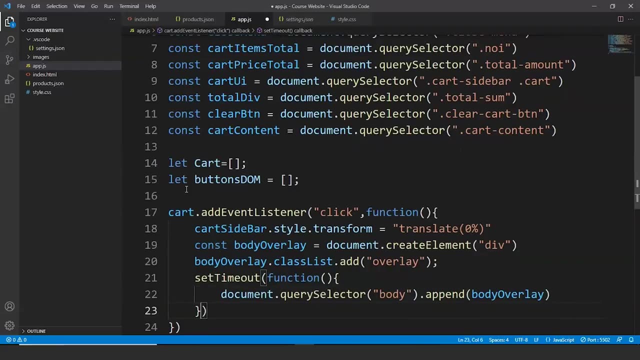 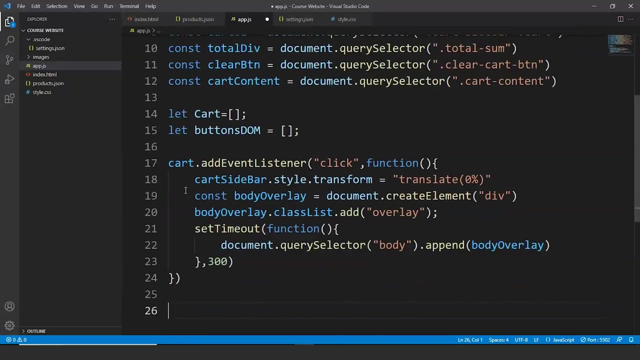 is we'll write document dot query selector and inside here we'll write body. then we'll write here append and we'll append body overlay hundred milliseconds. we are done with this. function will add another ability. so what'll do is will write here: closed cart dot. add event listener. and now we are closing the cart. so we'll write here: click. 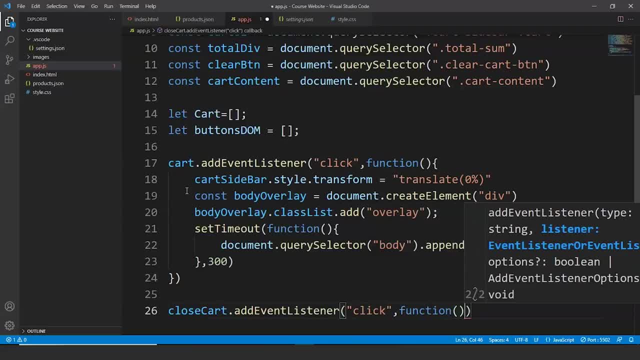 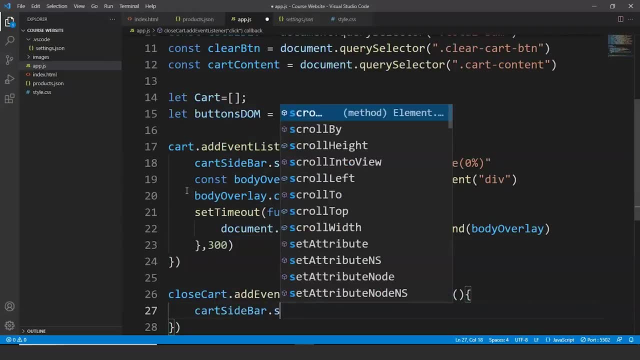 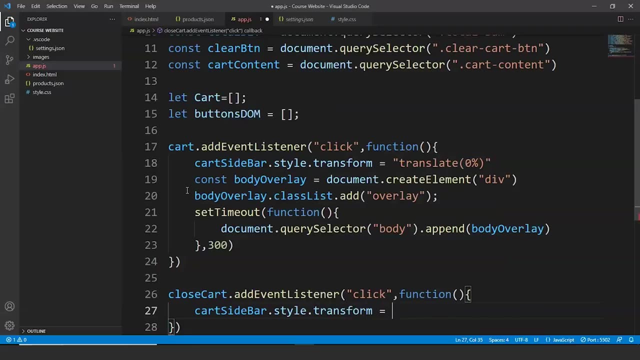 create a function And we will write here: cart, sidebar, dot, style, dot, transform, and again we will translate it to 100 percent. previously we did for 0 percent and now we will translate it to 100 percent again. So we will write here: translate and we will pass 100 percent inside the brackets here. 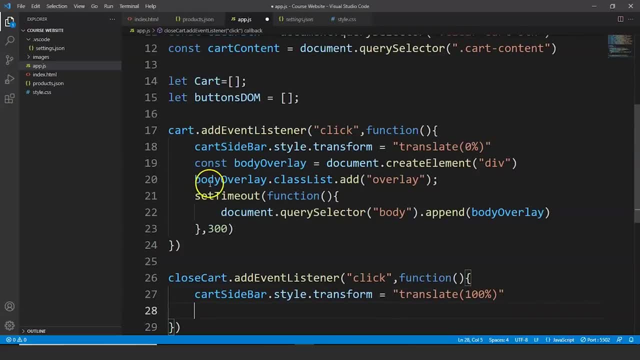 Next up, we will again use the body overlay variable. So we will copy this from here and we will paste it here. We will of course change the create element value. So instead of create element, we will write here document dot query selector and we will 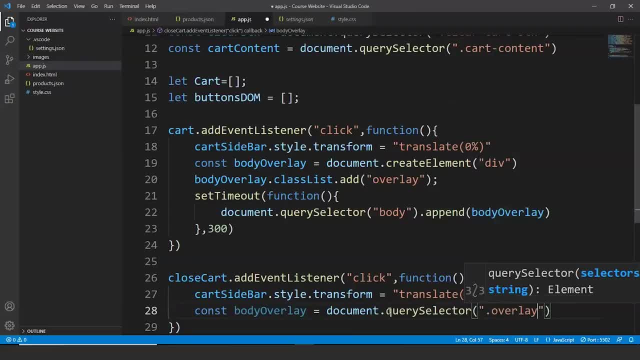 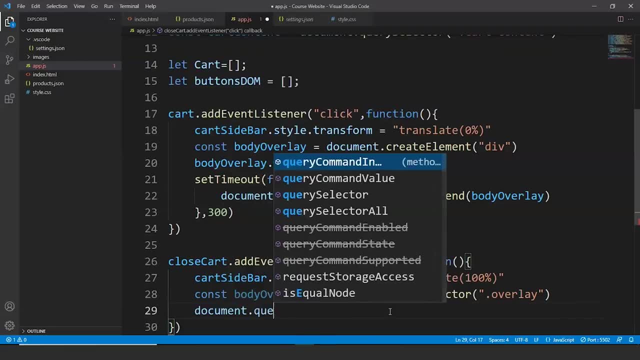 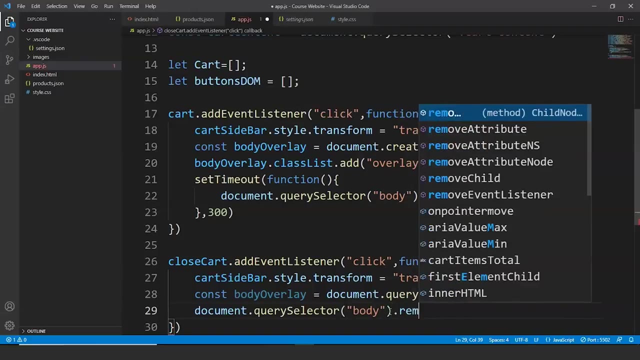 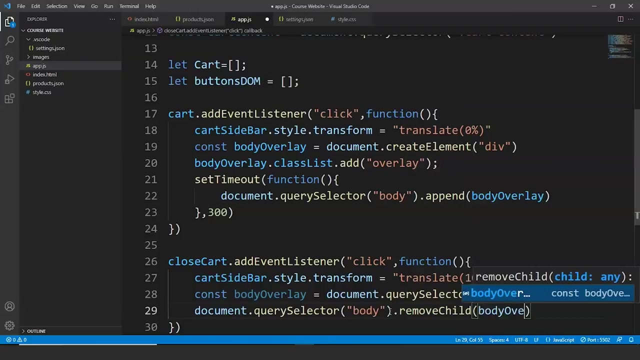 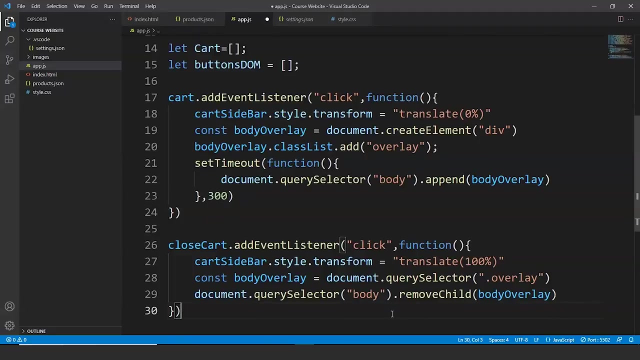 write here: dot overlay- Fine. Next up, we will write here document Dot- query selector. and we will write here body dot- remove child. we will remove body overlay from here. So we will write here: body overlay- Fine, We are good to go. 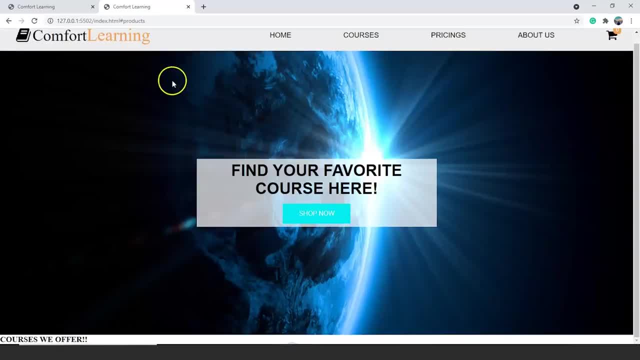 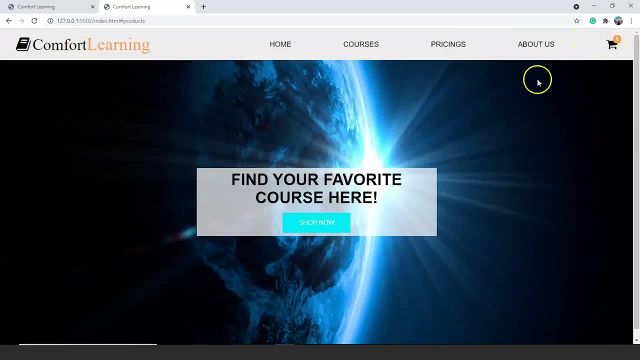 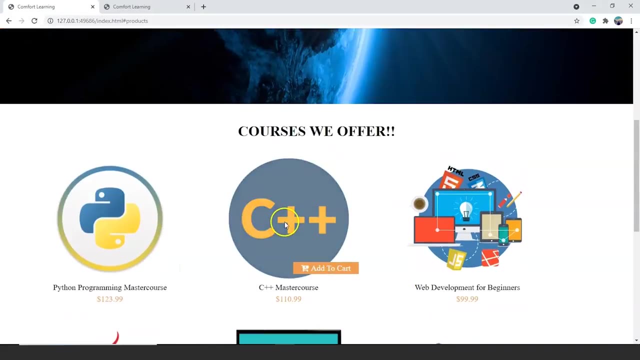 Save it now and go to the browser. So here you can see, on clicking the cart, Our cart is working totally fine. now We are in this particular program, So we are in our website which we are creating right now. This is the original website. 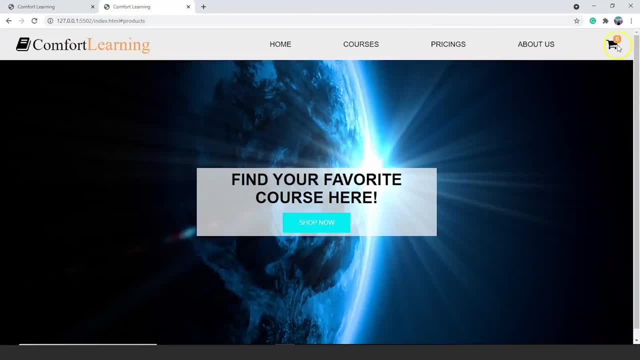 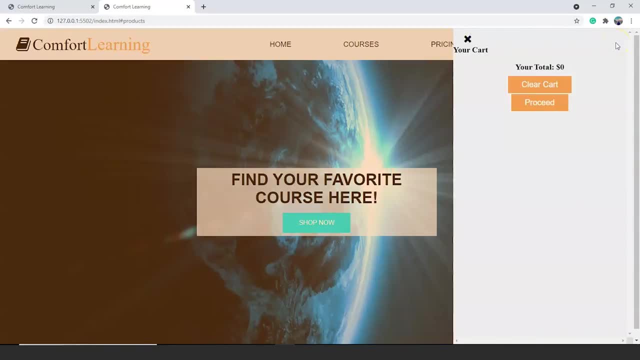 This is the final product, So leave it, and we are going to work on our website only. So here you can see, our cart is working totally fine. Now we can open or close our cart and we have two options over here. 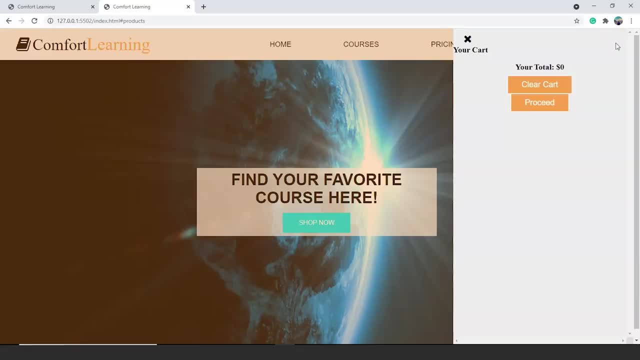 One is for clearing the entire cart and the other one is for proceeding further. Next up, we will add some more events for the hamburger menu. So we will add some more events for the hamburger menu. So we will add some more events for the hamburger menu. 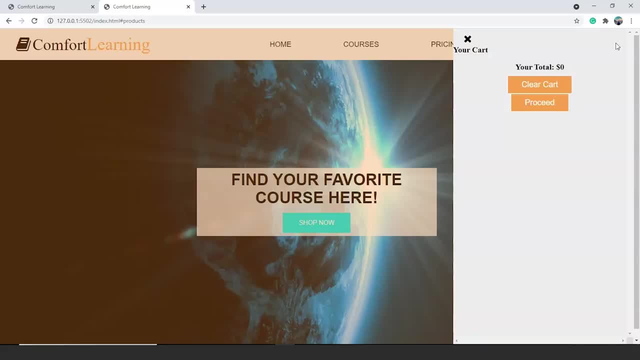 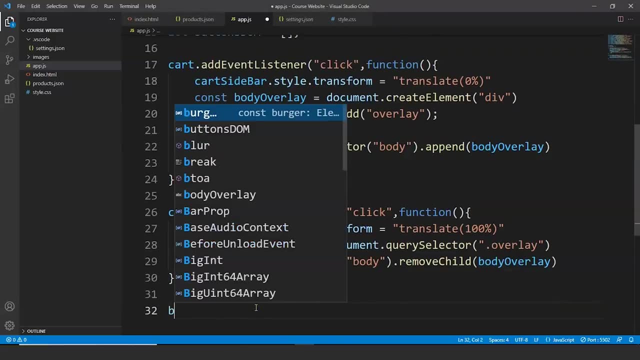 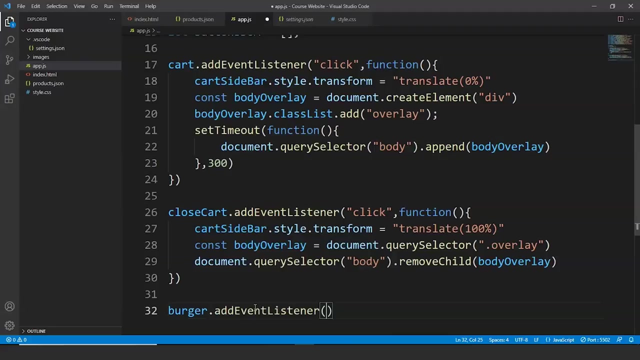 So we will add some more events for the hamburger menu, Now how to open or close that menu and all. So for that we will move to a JavaScript file again and we will write here burgeraddEventListener and we will add a click event. we will write here click. we will write here function and 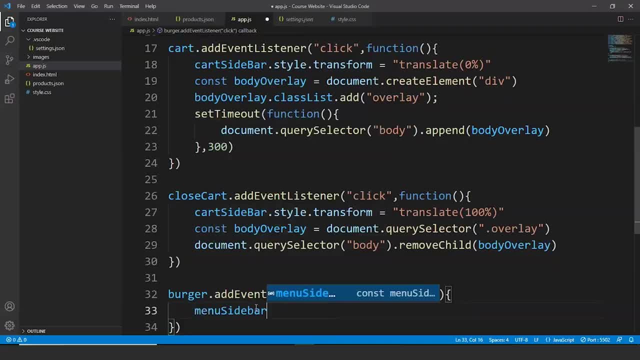 then we will write here: menuSidebaraddEventListener, menuSidebarstyledotTransform, and what we are going to do is we are going to translate again. We are going to translate it to 0%. Now, the same thing we have to do for this as well. 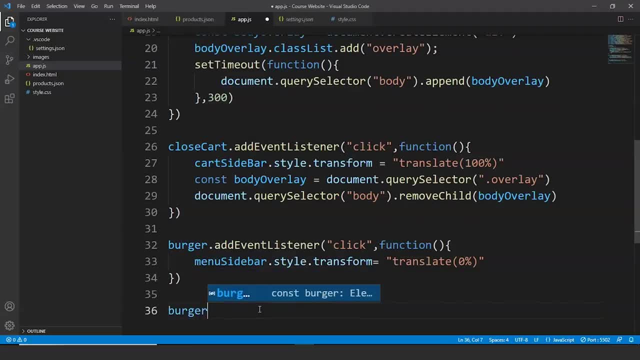 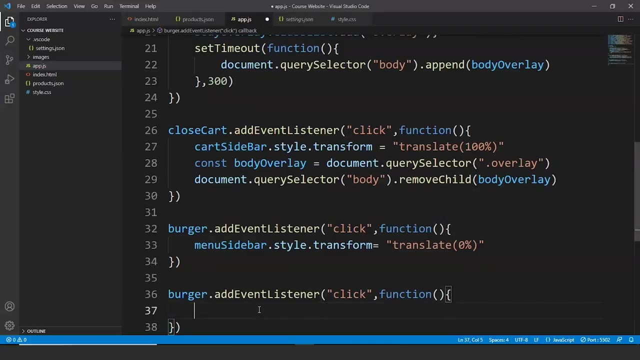 We will write here: burgeraddEventListener. inside here We will write: click, sub, Okay, Click, Join our page now. click, and then we'll write a function which will again do the same task. it will translate to minus 100%. We'll write here: menu sidebar, dot, style, dot transform. and we are again going. 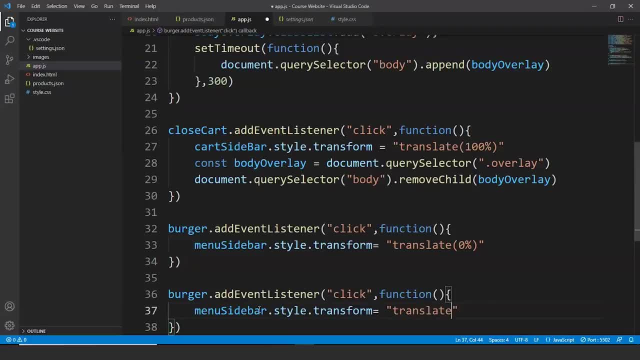 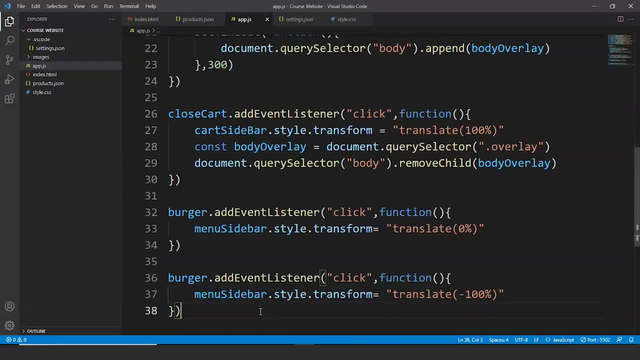 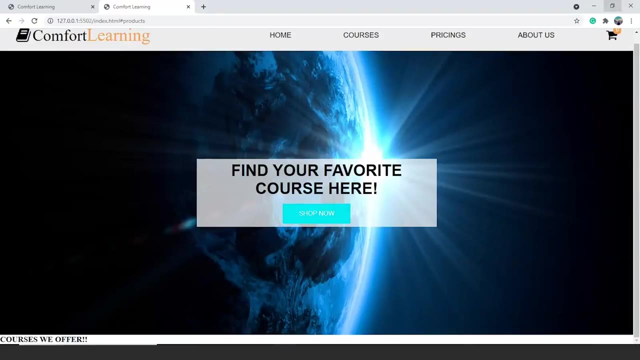 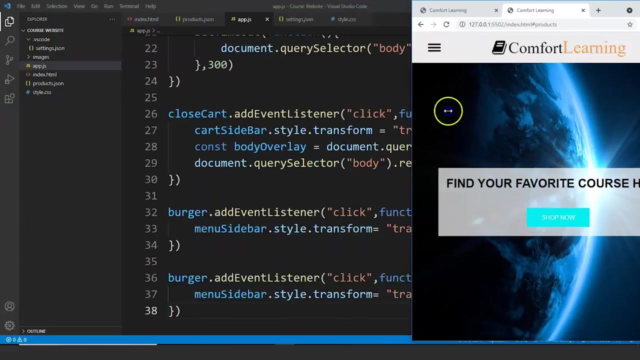 to translate it to minus 100% now. Fine, Save it and go to the browser. Now, if we decrease the size of a web page or if we decrease the size of a browser, you can see. okay, let me decrease it first So you can see the hamburger menu over here and on clicking it's. 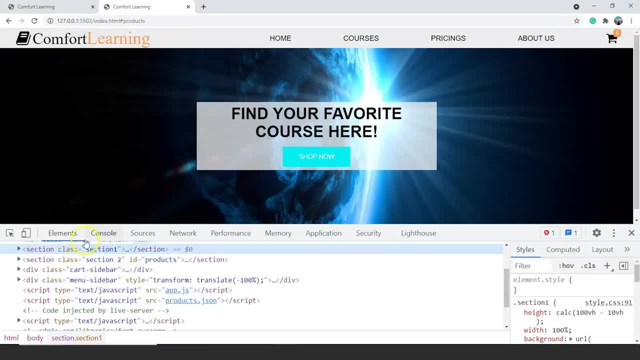 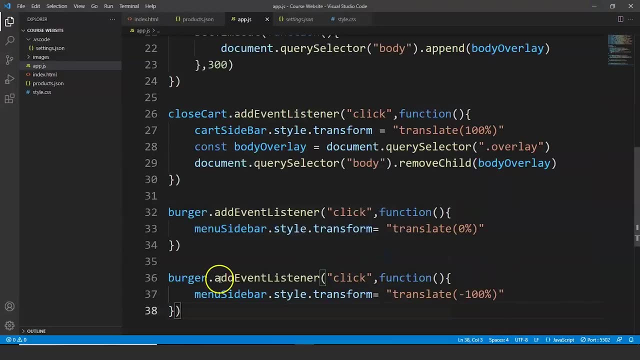 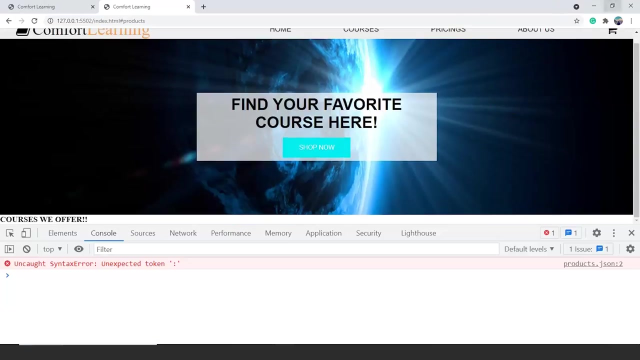 not working right now. So let's inspect those elements once. and there's no error? but let me check if there's any mistake. Okay, So we have to write here: close menu And now I guess it will work fine. We'll save it again and we'll move to the browser Reduce. 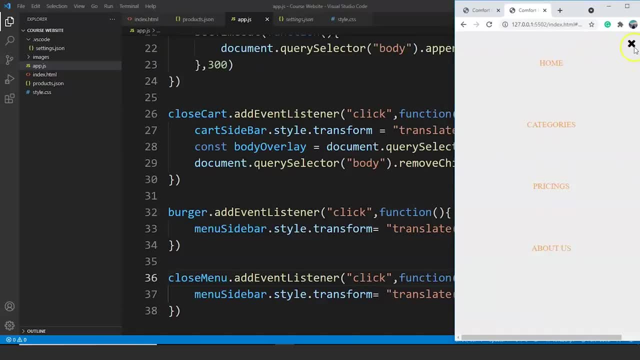 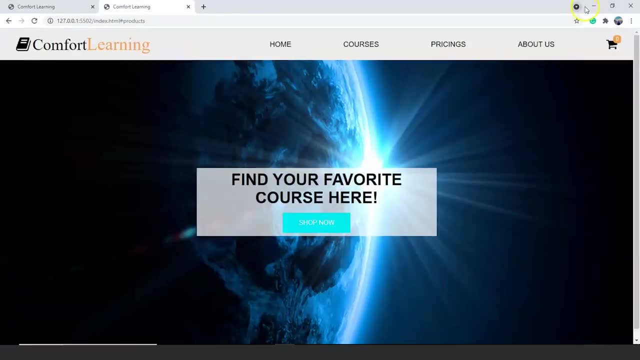 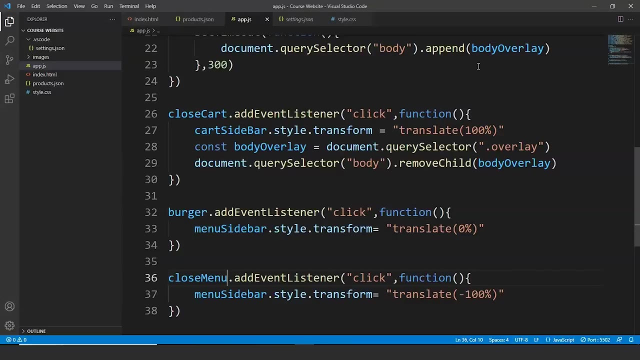 the size. click on this hamburger menu and you can see it's working totally fine. now, Right, So this part is also done. Now what we have to do next is we have to create a class to get those products from the JSON file. So keep your eyes open. now, guys, We'll. 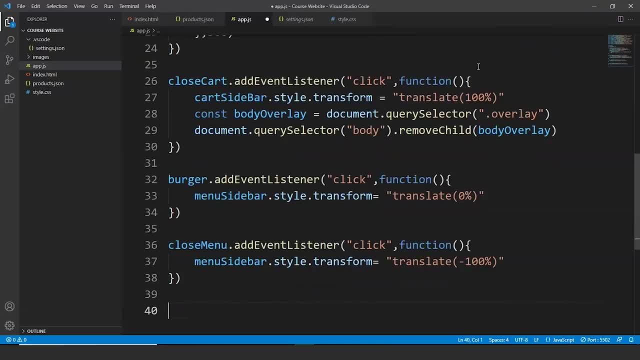 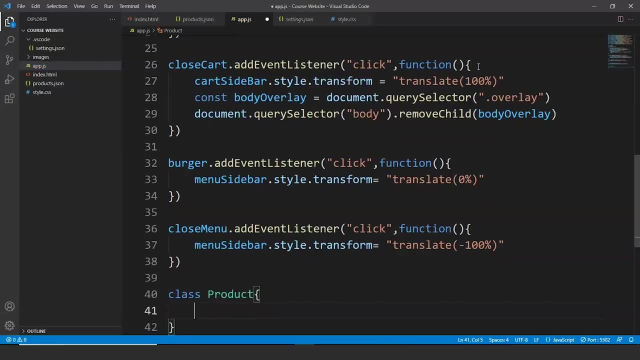 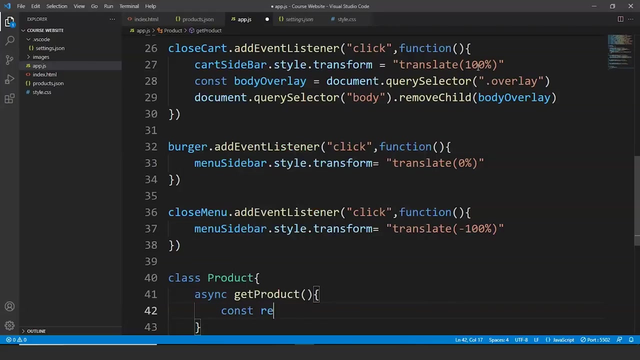 see how it actually works. So what we are going to do is we are going to create a class named product. So this is our class. We'll write here: async- I hope you are already aware of async and await. So we'll write here: get product and this is a function. We'll write here const response. 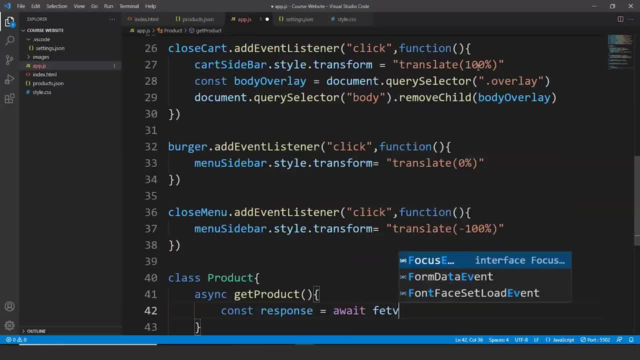 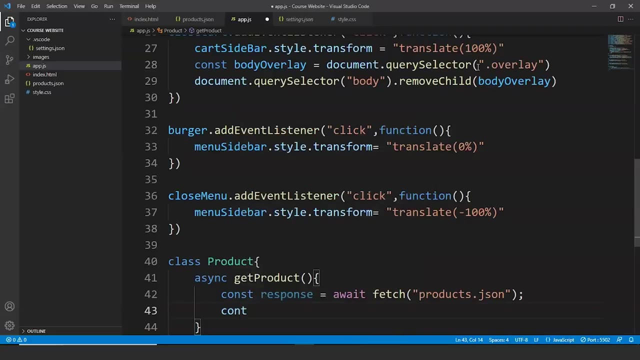 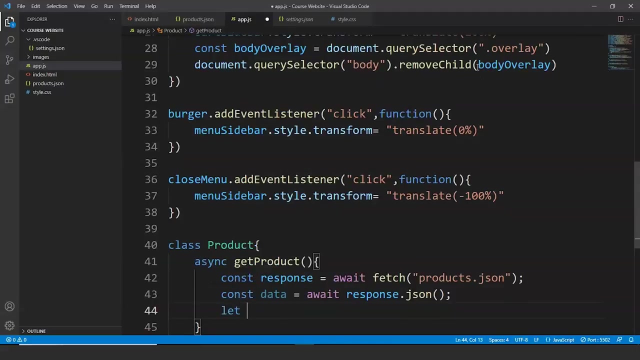 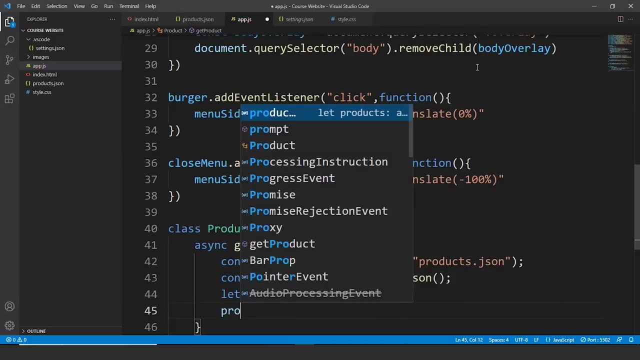 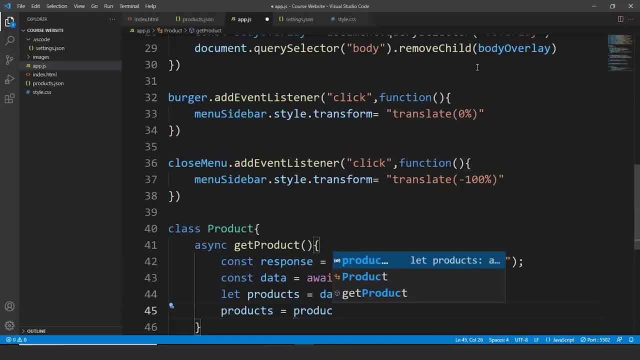 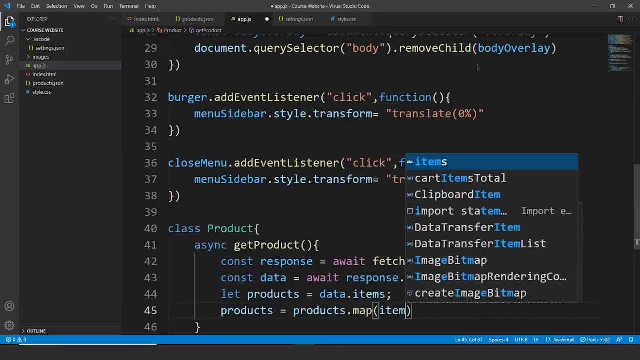 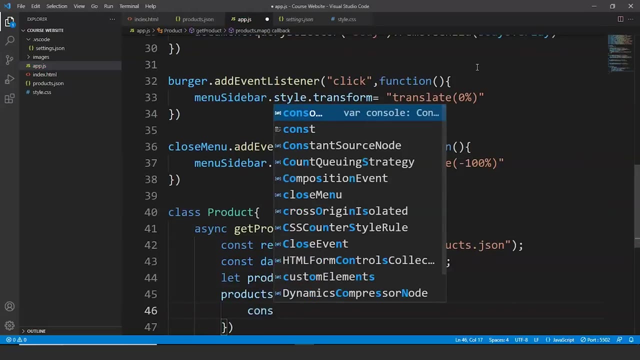 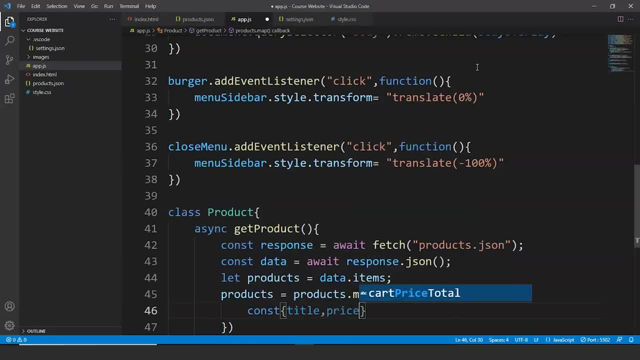 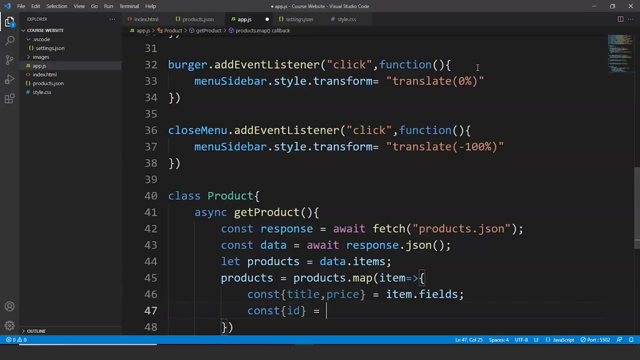 this: we'll pass title and price of the product And we'll write here item dot fields- fine, Okay. similarly, we'll do the same for ID as well. inside curly braces we'll write ID and we'll write here item dot sys. then we'll write here: 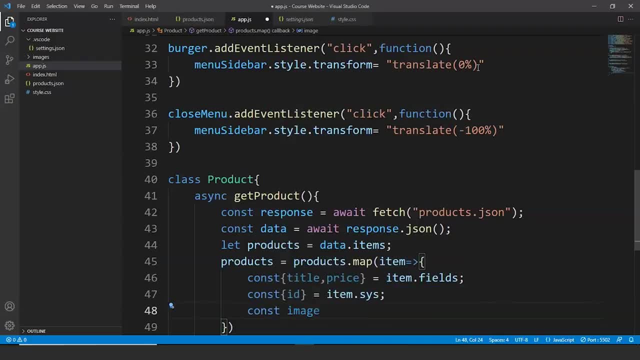 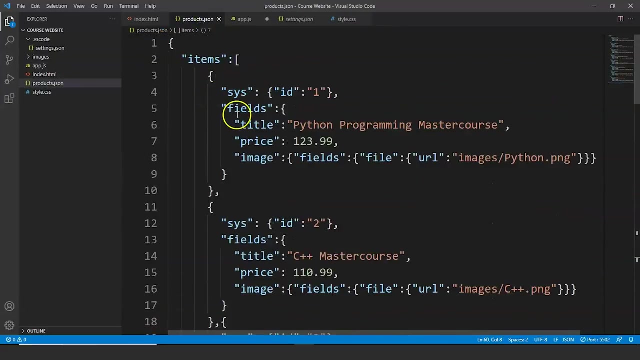 const image. now we are fetching the image so we'll write here: item dot fields, dot image, dot fields. we are actually giving the path right. if you see here in the JSON file you can see inside items we have sys fields, then inside fields we have title, price image and then inside image we have fields, file and URL. so we'll access. 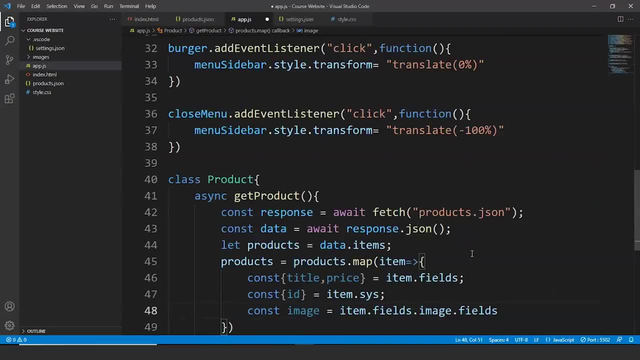 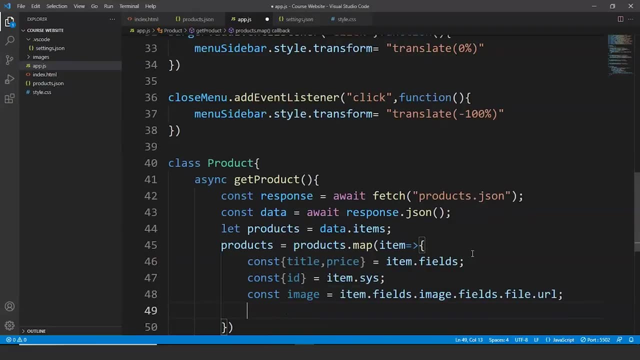 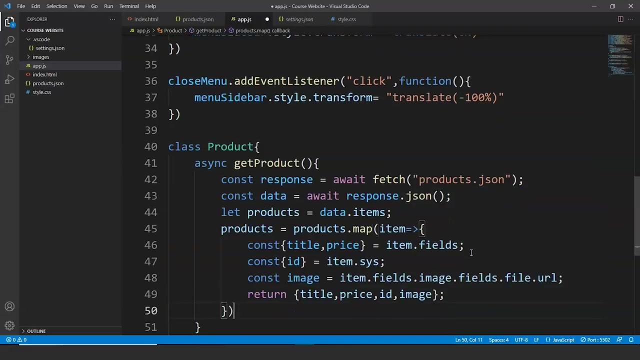 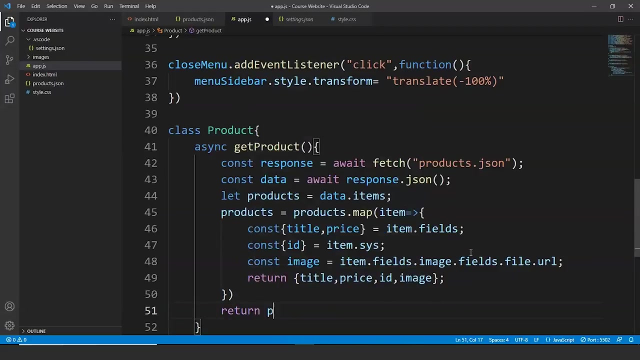 each of them. now we'll write here after fields: dot, file, dot. URL. and, lastly, we'll write here: return title, price, ID and image. fine, finally, we'll write here after this: return products. cool, now what we are doing here is. we are writing here after this: return products- cool, now, what we are doing here is. 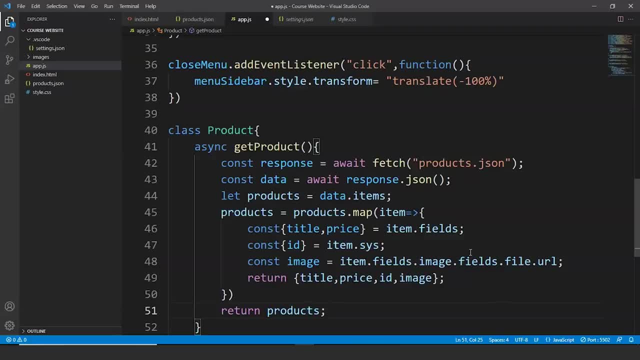 we are getting the details of all the products and storing them inside separate objects, so we have all the objects present over here. all those images were actually stored inside the local storage and now we can fetch them from that particular storage. now we'll create another class for the user. 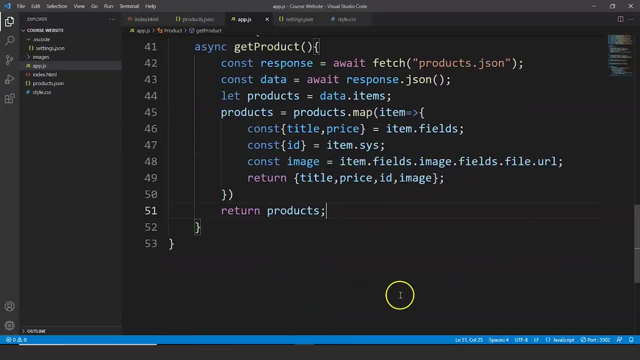 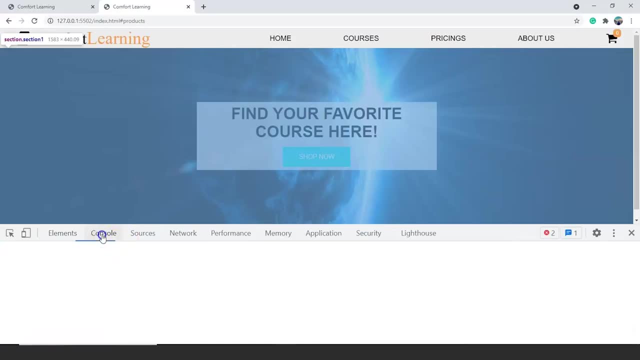 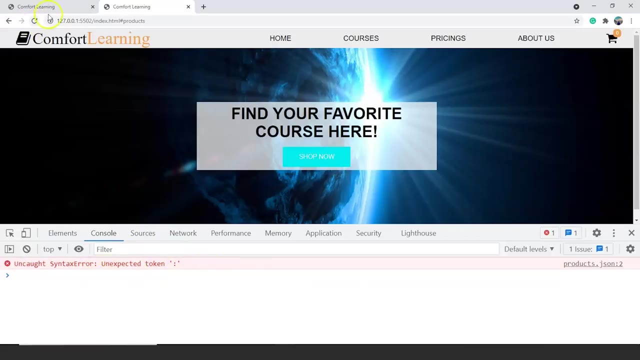 interface of the product. so if you save it now and go to the browser you will see no difference over here because it's not working as of now. if you go to inspect elements and console you can see it says length mismatch. it's because of the live server, so there's no error over here. 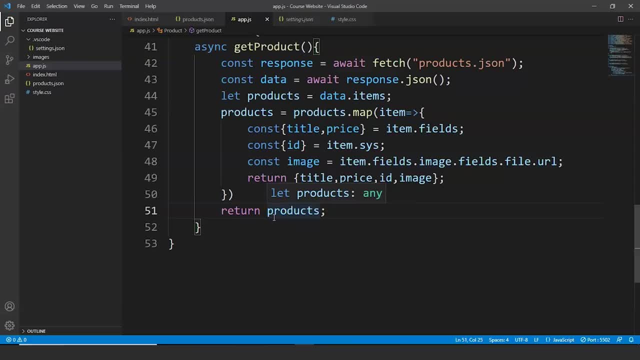 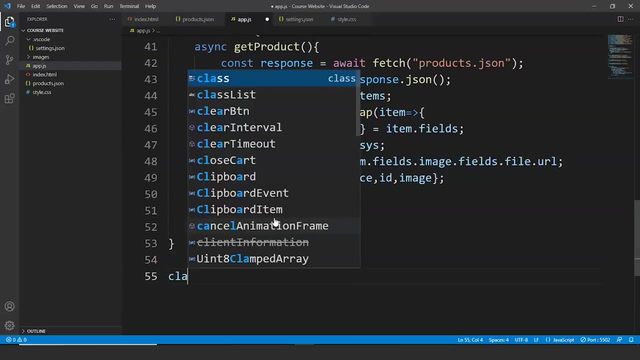 now we'll create another class for the user interface of the products. we'll add those products to the cart and we can delete them from the cart. we'll do everything inside one single class. so let's do it. what we are going to do is we are going to write here class. let's say the class name is UI. 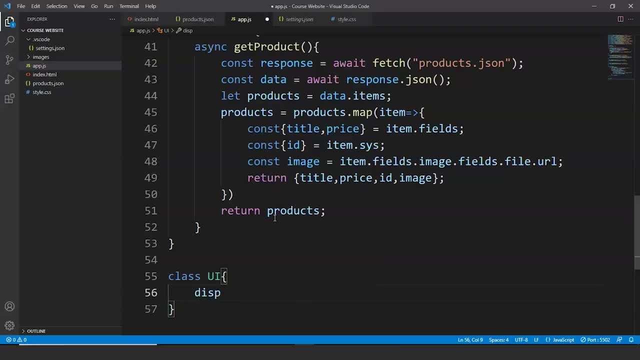 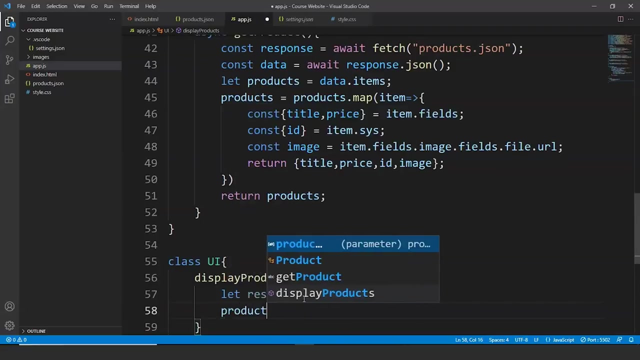 and we'll write here display products and we'll write here products. then we'll write here inside this: let result be a variable and we'll leave it empty. over here next line, we'll use the for each loop. so we'll write here products, dot for each. 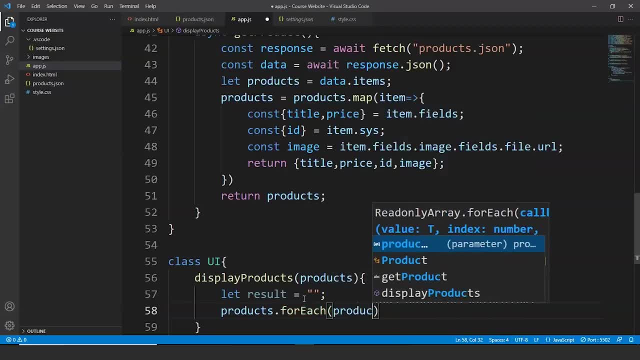 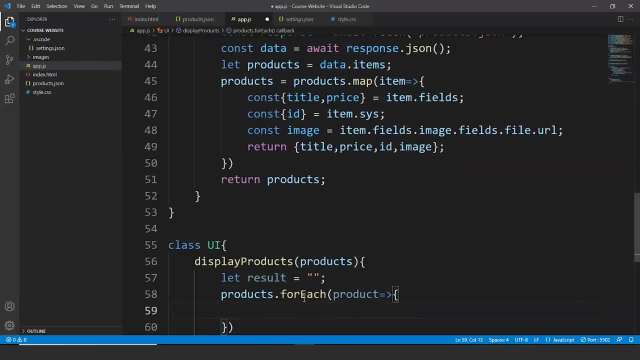 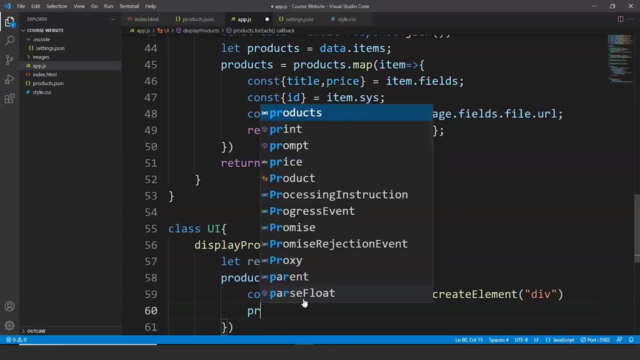 loop and inside this we'll create an arrow function, so we'll write here: const product div, let's say, is a variable. and then we'll write here: document dot- create element. again, we are going to create an element, so we'll write here: here div. and after this, what we are going to do is we are going to write: 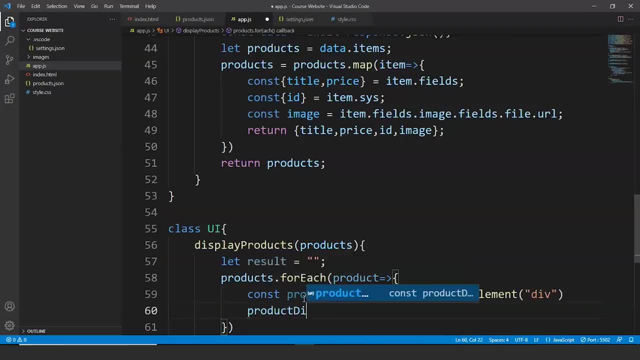 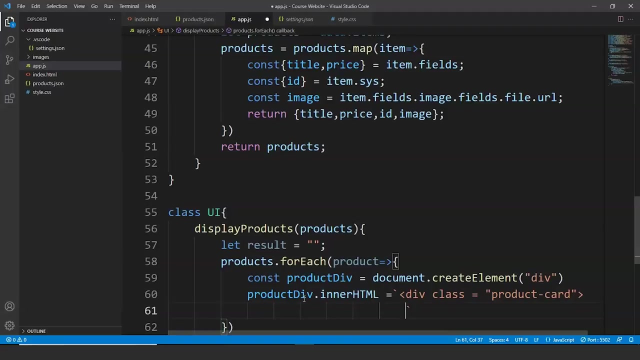 here product div dot innerHTML is equals to: now the main part starts. so inside this we'll write div class is equals to product card, and then we'll write img- we'll add the image. so here we are going to add the image. so here we are going to. 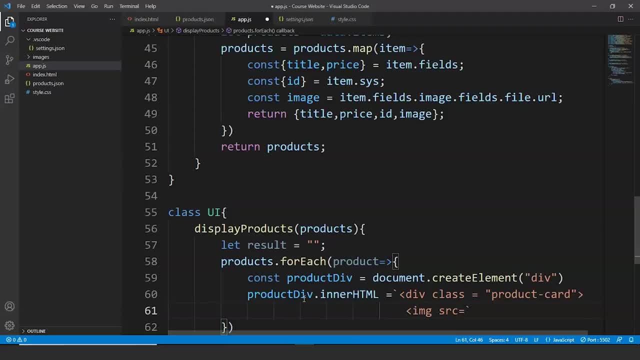 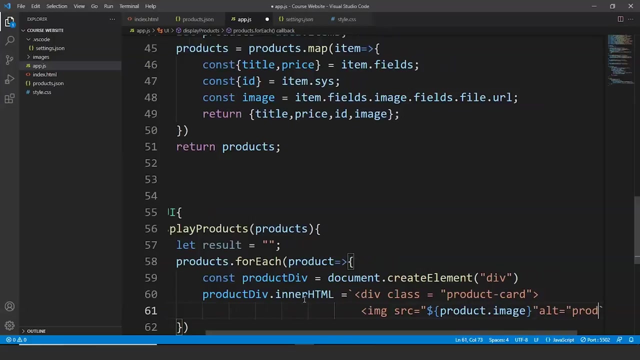 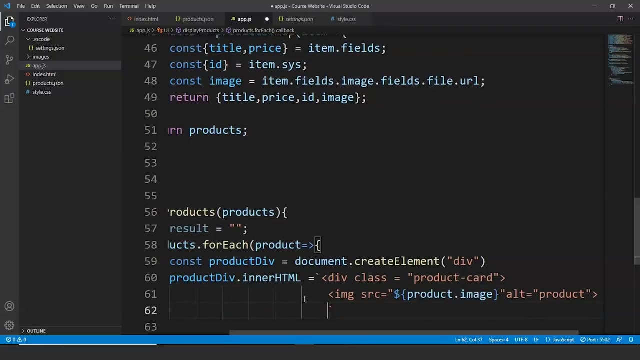 add the image. so here we are going to add the image. so here we will write: img src is equals to dollar. product dot image. we are going to fetch it and instead of alt, in place of alt, we will write alt as product. In the next line we will use the span tag. again, we will write here: span class is equals. 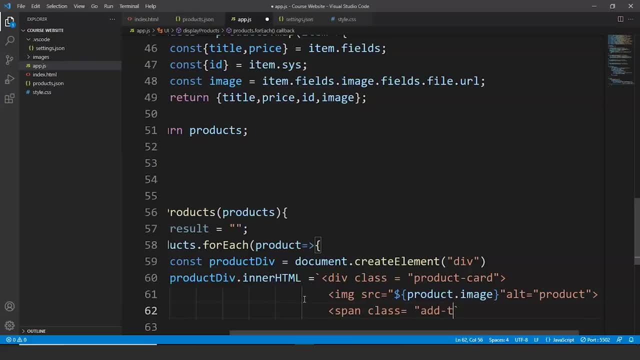 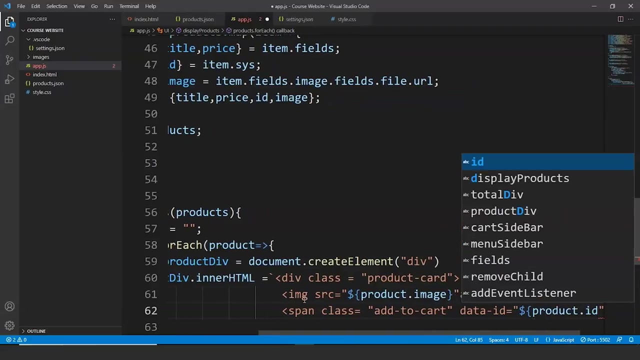 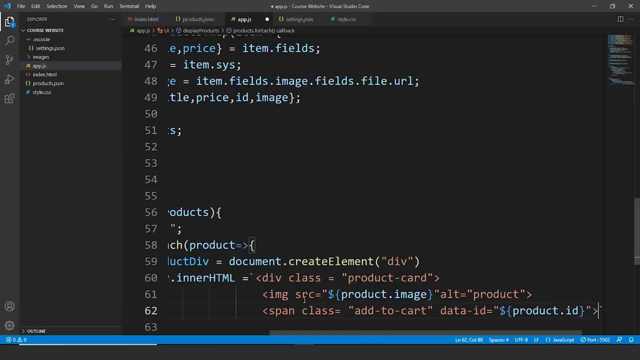 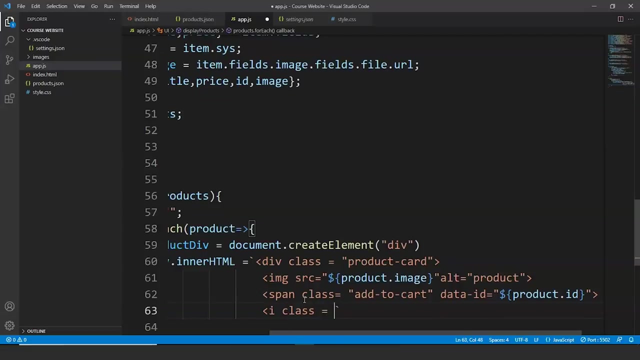 to add to cart. and we will then write here: data id is equals to productid. we will close this tag. we will close this span tag. we can say In the next line: we will use the i tag. we will write here: i class is equals to far, far. 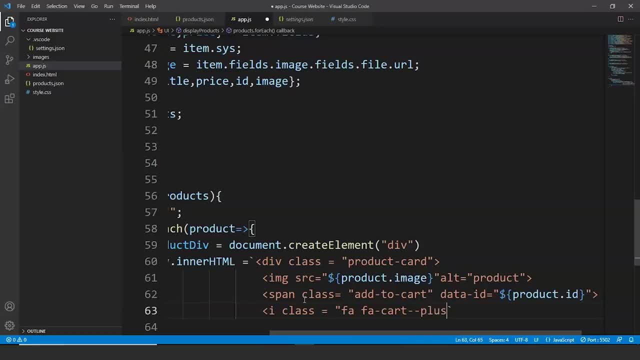 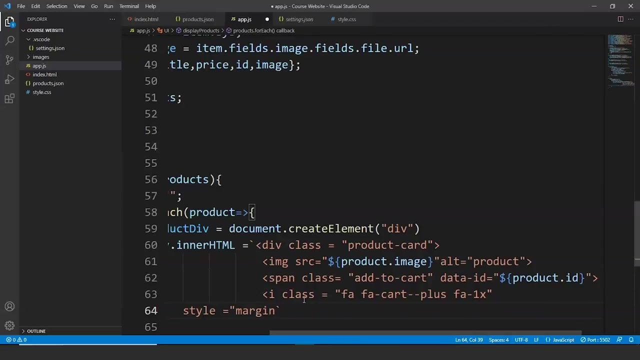 cart plus far1.. Now what we are doing is we are going to show the number of items present in a cart over the cart icon. That's why we are doing all this. So here what we'll do is we'll write: style is equals to margin. dash right, margin right. 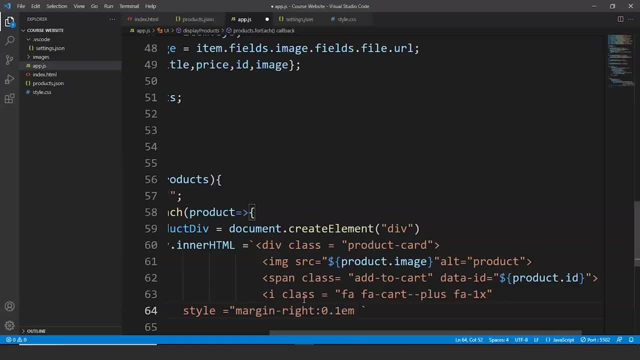 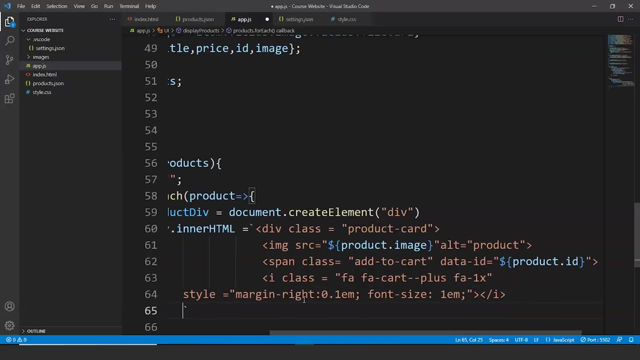 is going to be 0.1 m. Font size is going to be 1 m. fine, Close this as well. close the i tag as well And in the next line right here, add to cart. so the span tag is finally. we are going to. 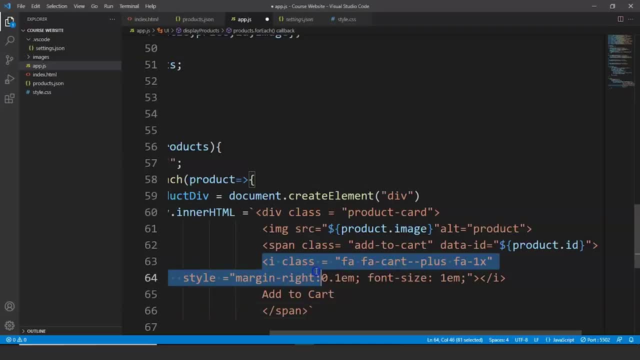 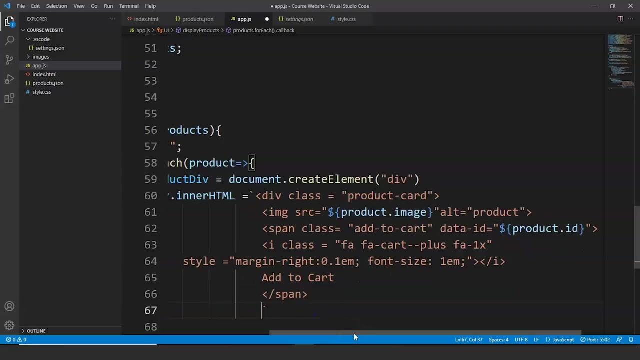 close it Now. This is a single tag. I have written it in such a way because I don't want it to create any sort of confusion for you guys. So the span tag starts from here and goes till here. Now we are remaining with some more part of it. 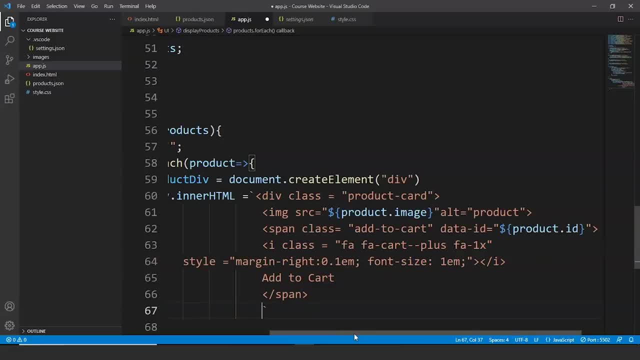 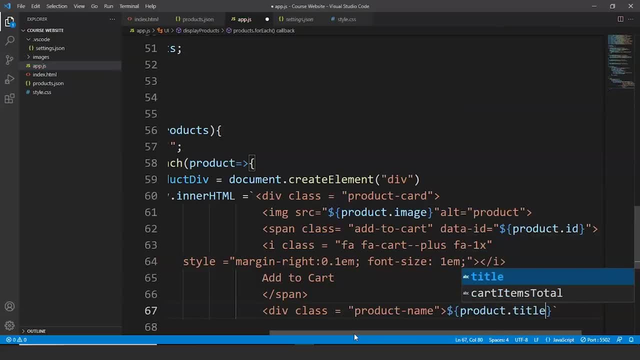 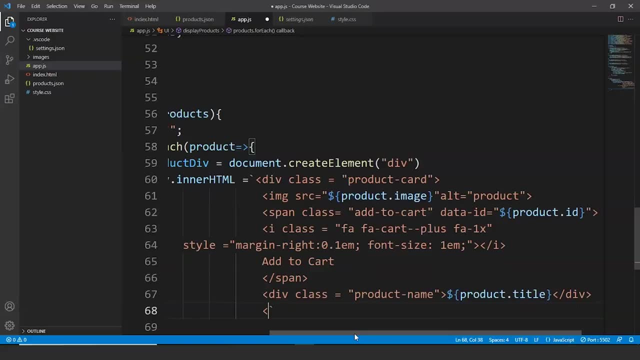 Product dot title, And here we are going to close this div tag. In the next line we are going to write div again. Class is going to be product pricing And in changed: here we'll write product dot price And here we'll write productprice. 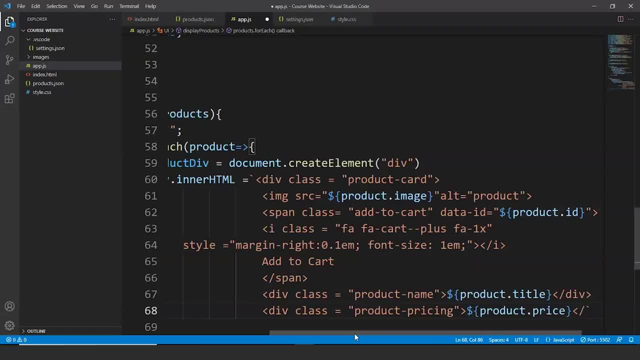 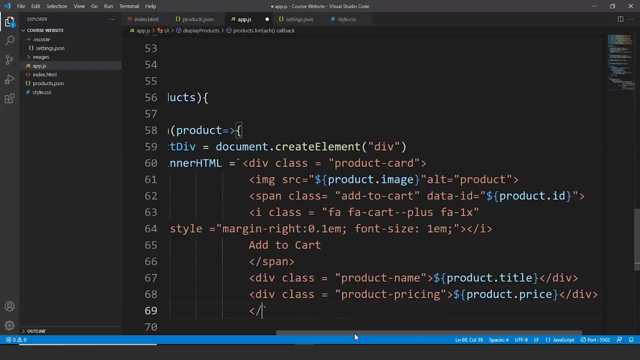 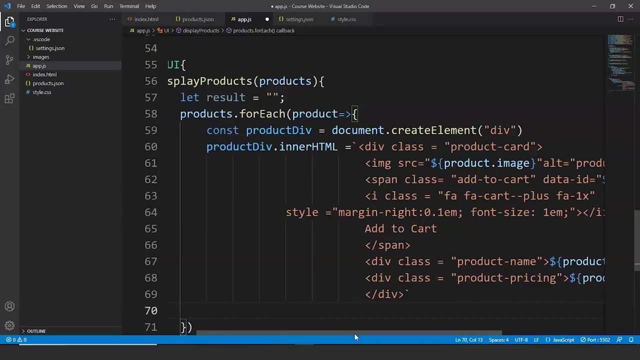 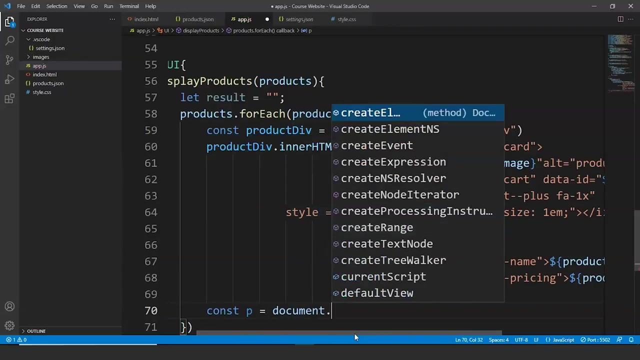 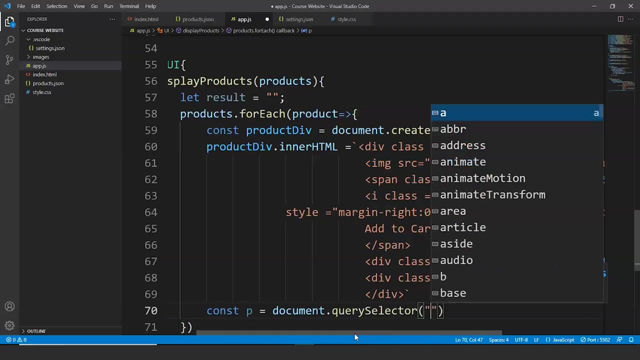 Nice and we are going to close this div tag here, close the first div tag as well, and we are good to go in the next line. what we are going to do is we are going to write here: const p is equals to document dot querySelector, and inside this we'll. 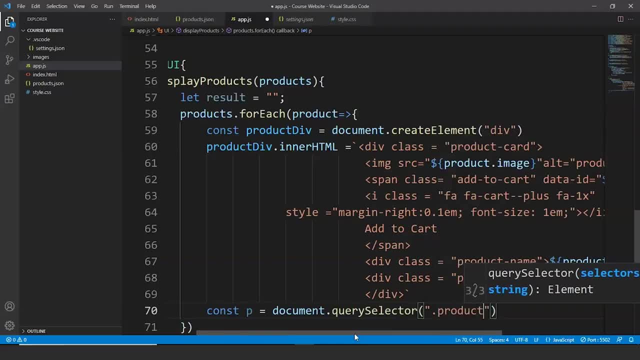 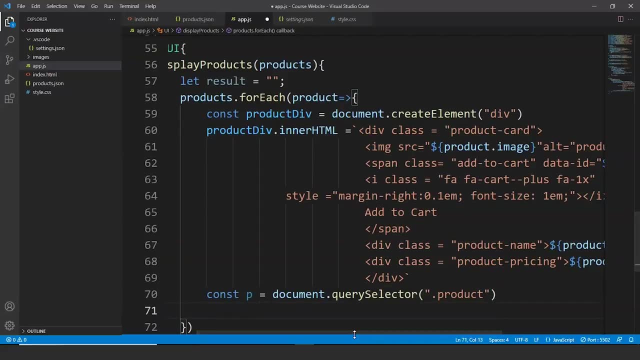 write dot product. we are going to access the element with product as class or we are going to access the product query. then we'll write here: p dot append product. What we are doing is any item we are adding to cart is we are going to append. 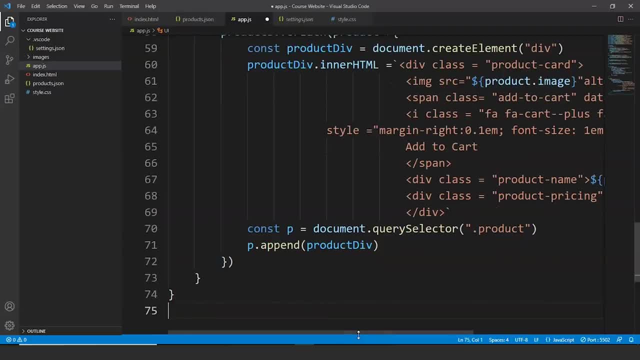 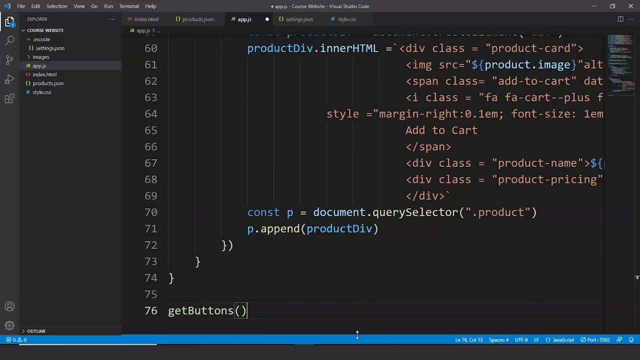 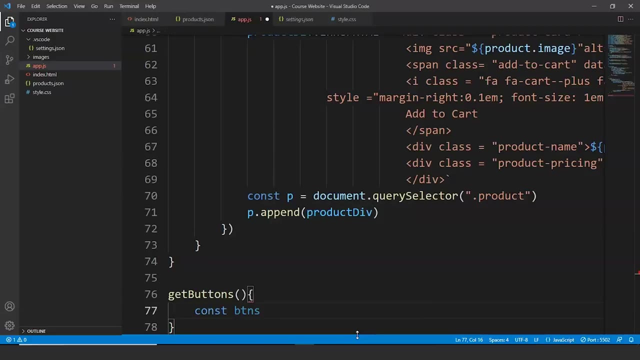 that item inside the cart. so that's what we are doing till now. now the next thing we are going to do is we are going to write here a function, get buttons, basically a constructor. we can say: we'll write here const buttons, we'll write here const buttons is equal. 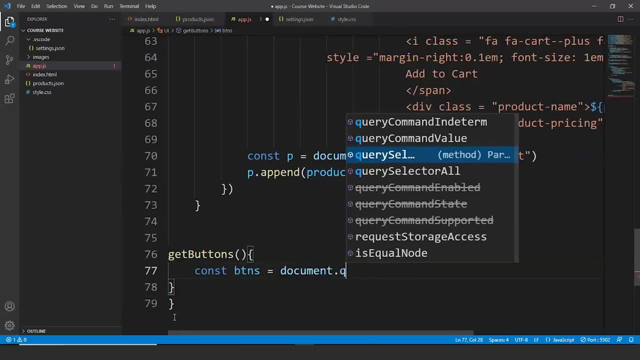 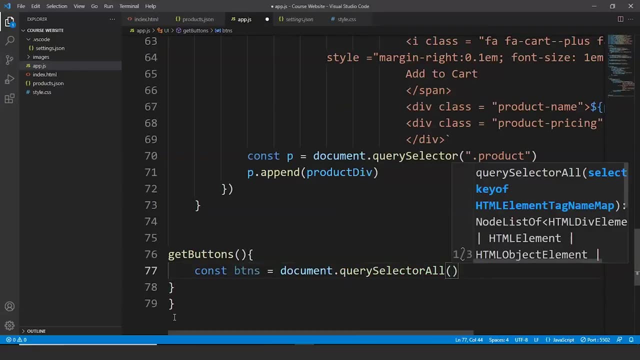 to document: dot querySelector. we have to write a querySelector, all, and then we are going to write here inside this dot: add to cart. fine, we have been through all these querySelector methods previously, so I don't think that this is going to create any sort of problem for you guys. so let's move ahead and we'll write here. 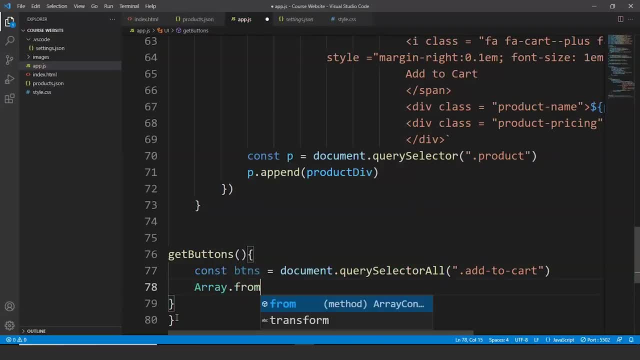 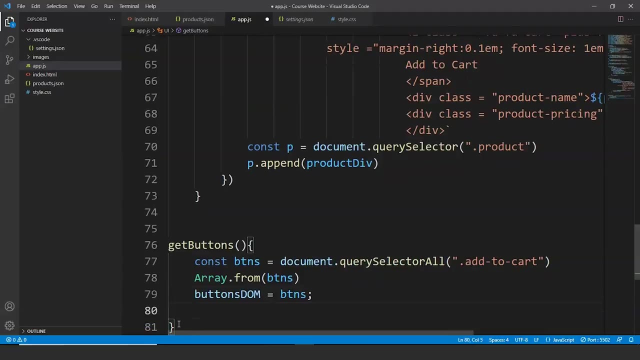 array dot from. we'll write here buttons. then we'll write here buttons Dom is equals to buttons. we are going to pass the value of buttons to buttons Dom. then we'll write buttons dot for each, and inside here we'll write button. and we are going to create a narrow function over here. here what we'll. 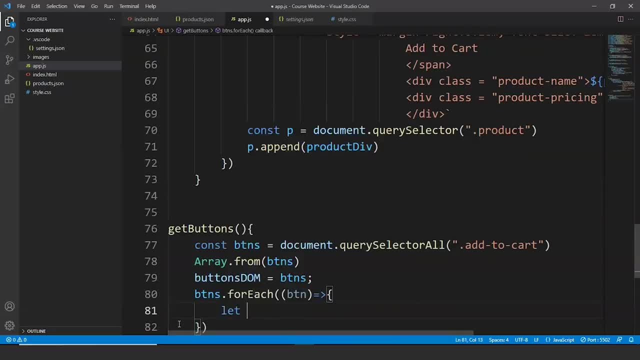 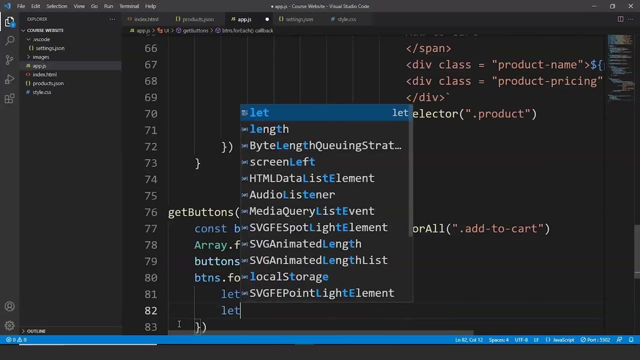 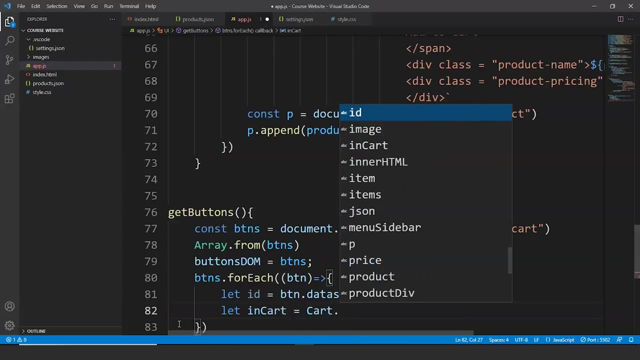 do is we'll write here: let ID is equals to button dot data set dot ID. in the next line we'll write let in cart is equals to cart dot find and we are going to pass item to this function. so we are going to write inside here: item and. 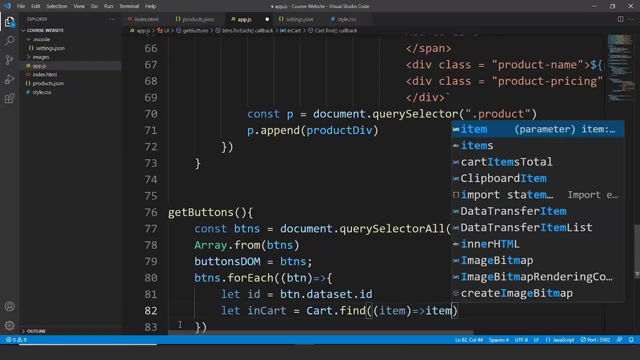 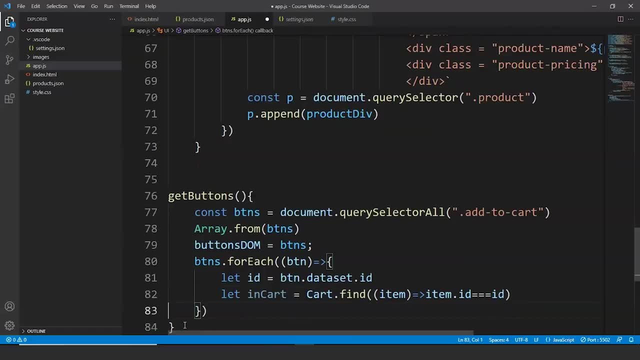 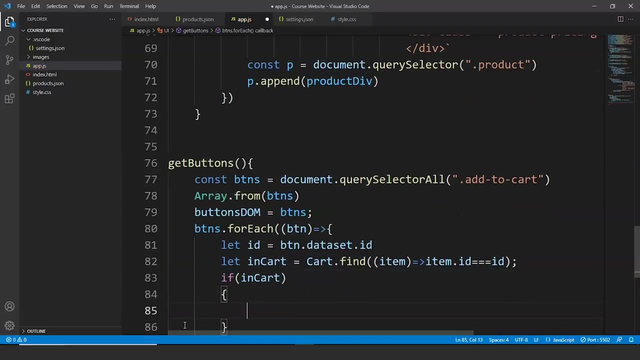 again, an arrow function will write here: item dot. ID triple is equals to ID. fine, we are going to check the condition here. if we will write here: if in cart, then will write here: BT end dot- inner HTML is equals to in cart. so what we are doing is if we have added the product to 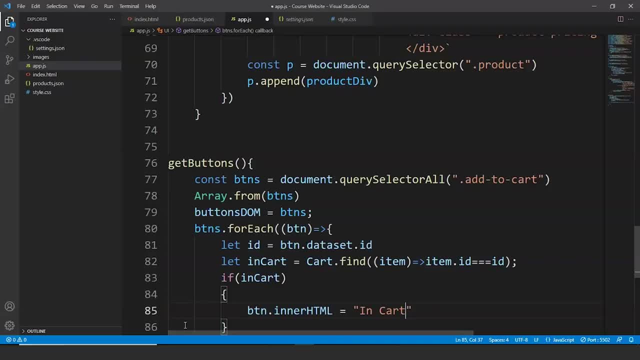 cart already. then the button will change as we have seen earlier, that on adding the product once to the card, the button will change to in cart. fron of theensed appi you created add to cart. so this is what we are doing here. next up we'll write here: button dot. 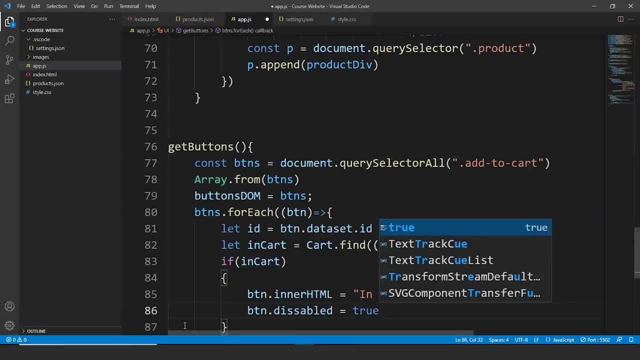 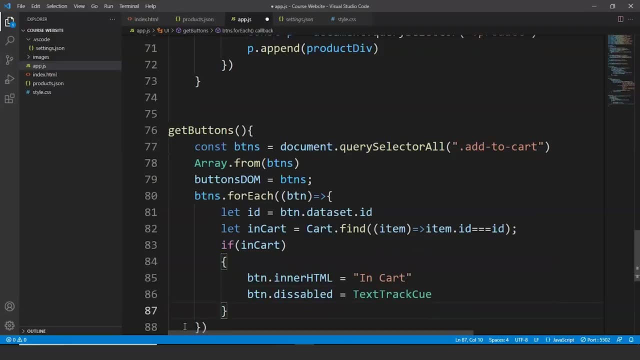 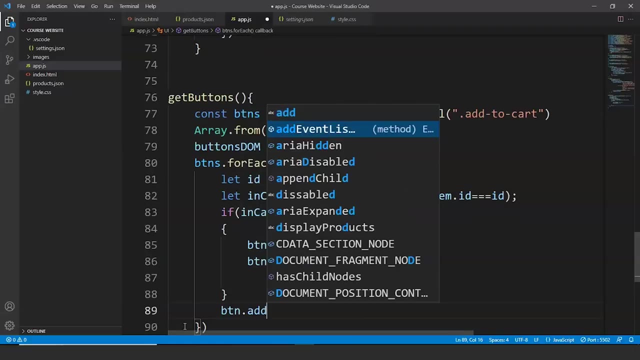 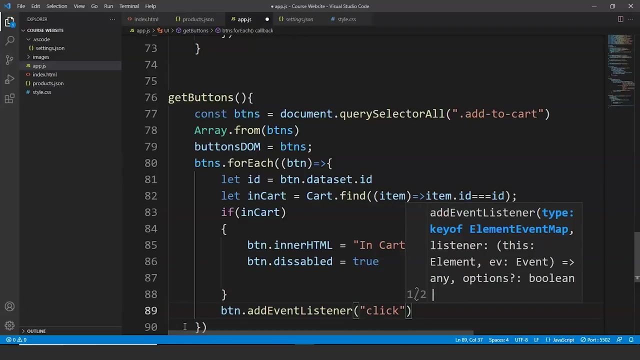 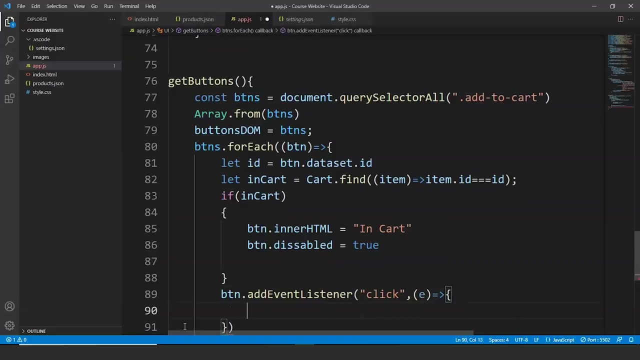 disabled is equals to two. we are going to disable that button once the product is added to cart. fine. next up we'll write here: button dot- add event listener. and we are going to create an event. we'll write here: click and let e here. then we'll use the arrow function and we'll write it here: e dot. 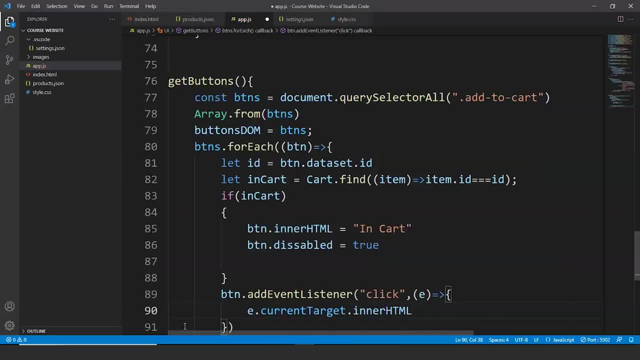 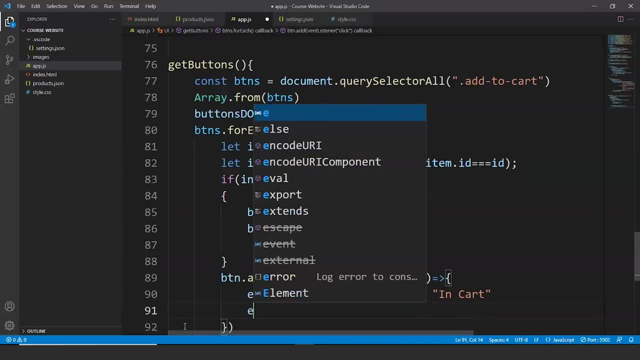 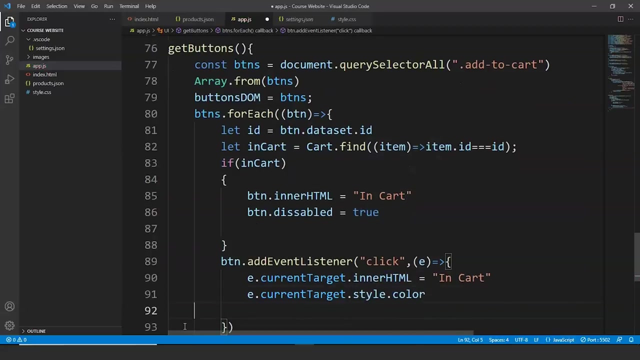 current target dot inner HTML is equals to in cart, then we'll write here: e dot. current target dot inner HTML. okay, we'll write here: e dot. current target dot style dot color is equals to white. e dot. current target dot style dot pointer events equals to none And we are done with it. Next up, we are going. 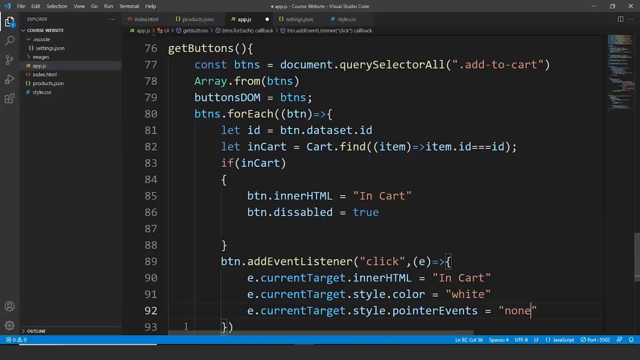 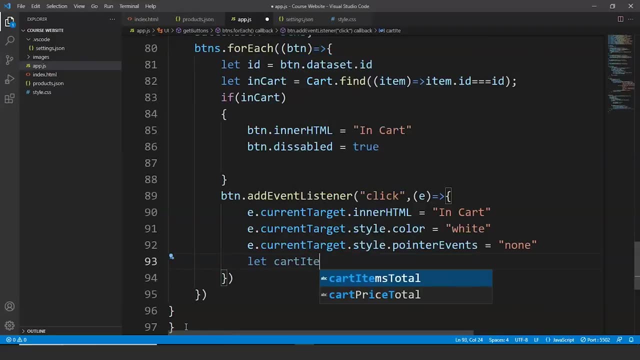 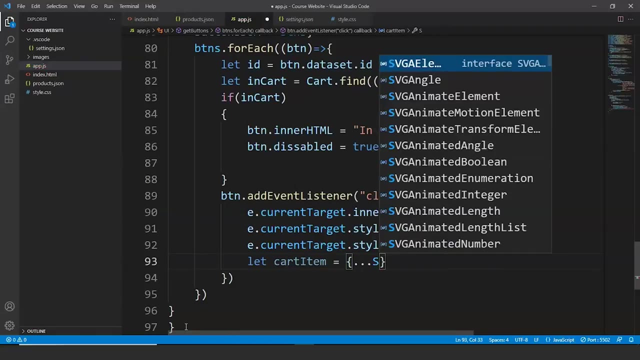 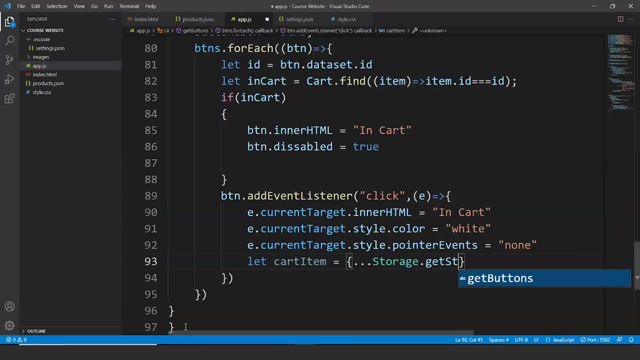 to store the products in the cart. So for that, what we are going to do is we are going to write here: let cart item is equals to. so we are going to use a little bit of JSON now. We'll write here: dot storage, dot get storage products will write your. 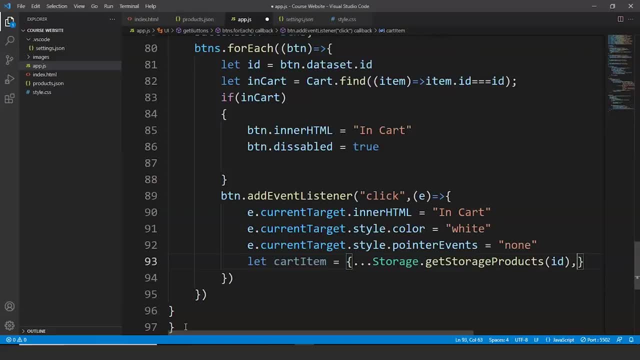 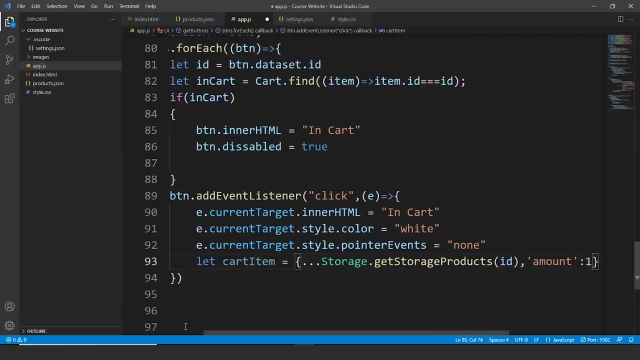 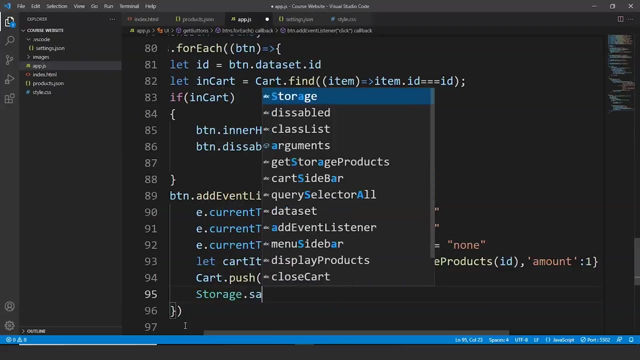 ID, comma, amount, and the amount is going to be. one will write here: cart dot push. we are going to push the cart item to the cart, So we'll write here: cart item. Then we'll write here: storage. we are going to store it inside the cart, So we'll write here: 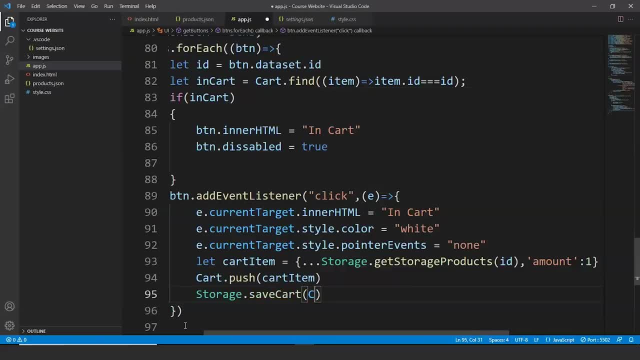 storage dot save cart And we'll pass cart over here. Fine, Now we have to calculate the total and we have to set the total items as well. So for that we'll write here this dot set cart values. We'll write here cart And to display. 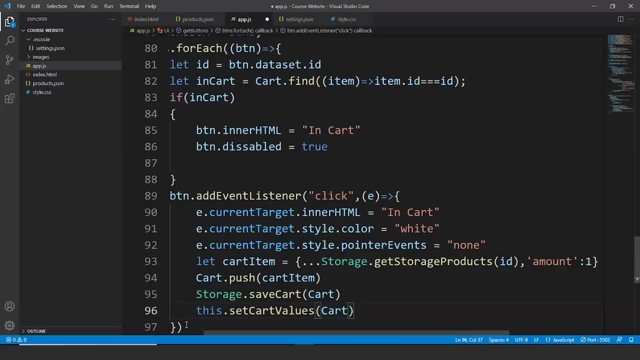 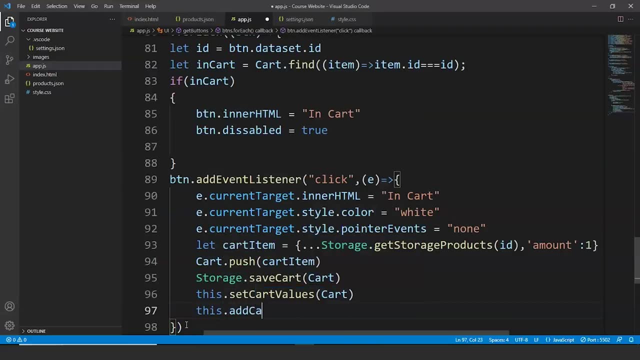 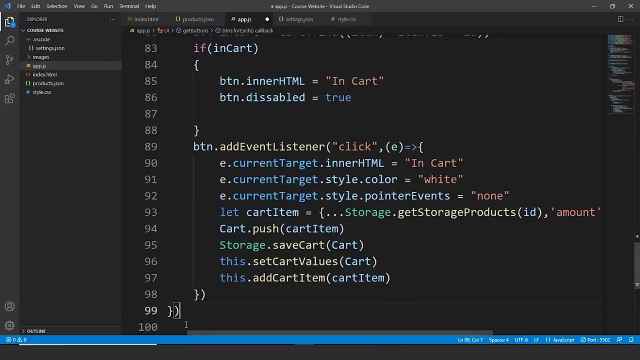 those cart item. we have to write here this dot: add cart item and we have to add that cart item. So we'll write here this dot: add cart items item and we'll pass cart item over here. Fine, We are done with the working of cart as well. Next up, what we are going to do is we: 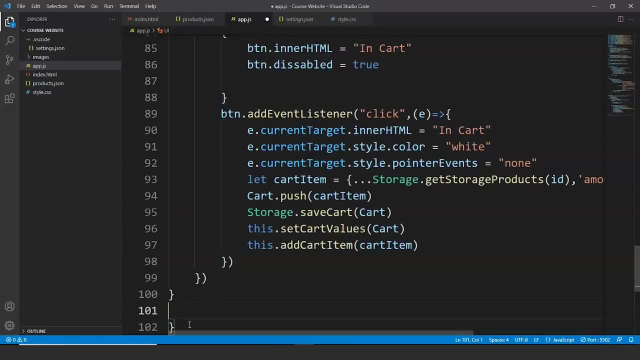 are going to change the total value of cart. we are going to change the value of cart on increasing or decreasing the cart products. So first of all we have to write here: set cart values and we have to pass cart over here. we have to write here: 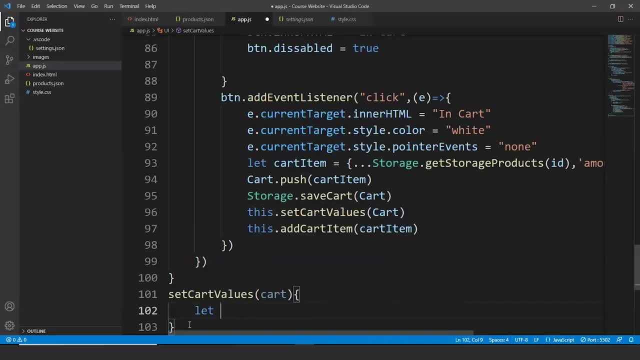 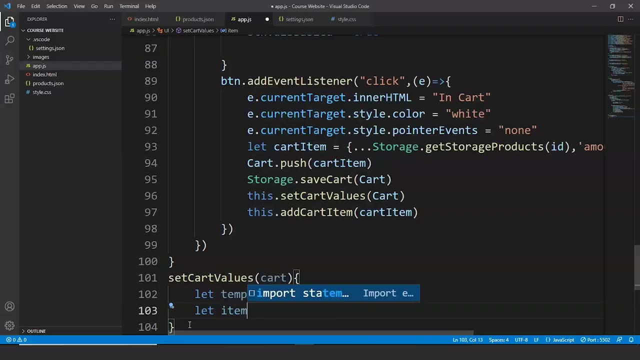 cart. Let's say we have a variable temp total. So this is going to be a temporary variable. will write here: temp total is equals to zero And we'll take another variable For that. we'll write here item total. So item total is. 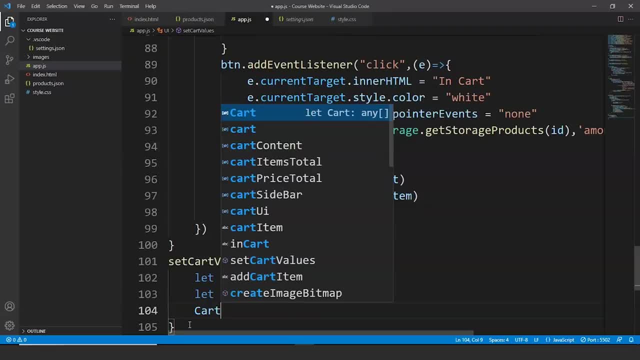 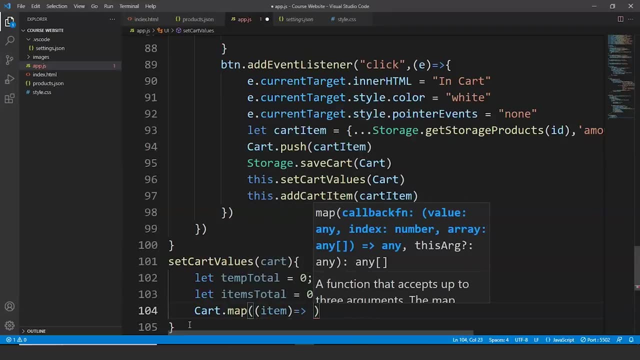 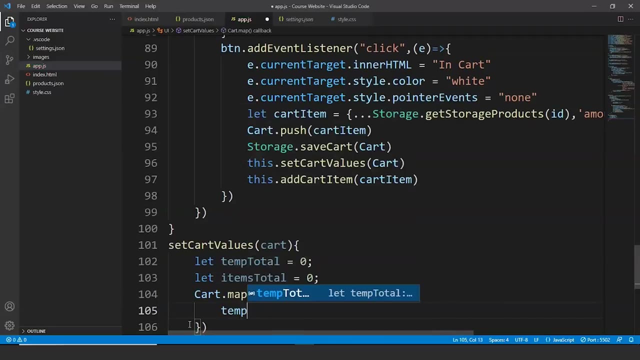 also going to be zero. Now we'll map this cart, So for that we'll write a cart dot map. We'll write the item will use error function, So for that we'll write here: temp total plus is equals to item dot price into. 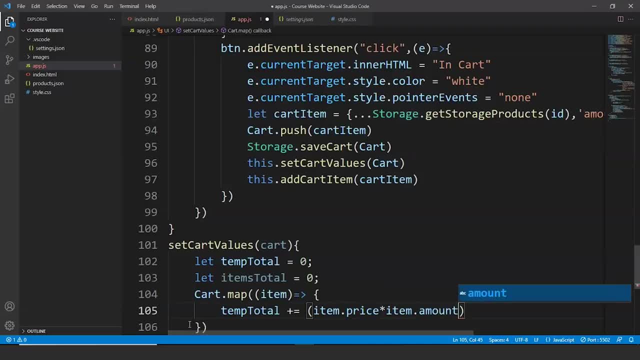 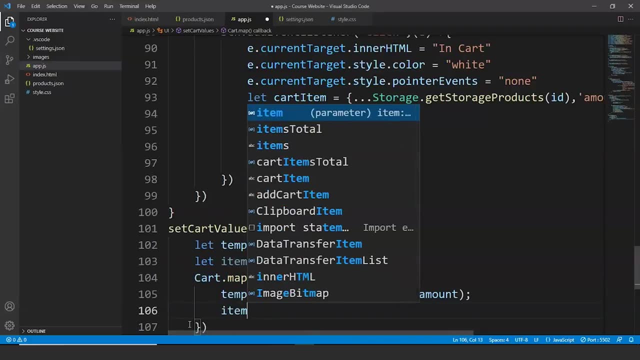 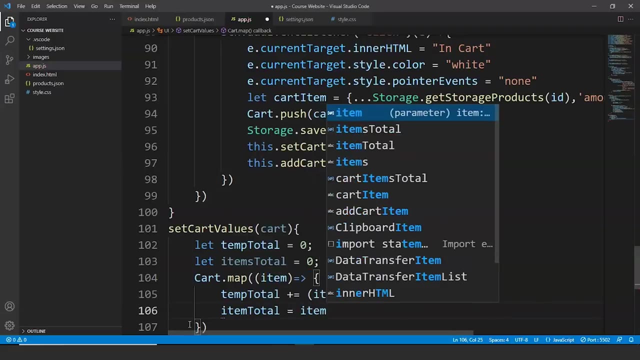 item dot amount. So this is how we are going to get the total amount and then we will write here item. basically we are swapping all of that, so we will write here: item total is equal to item dot amount. we have to add these two values, so we will write here: item total plus is equals to item. 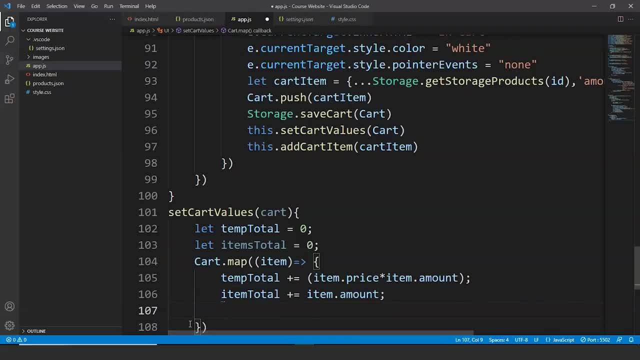 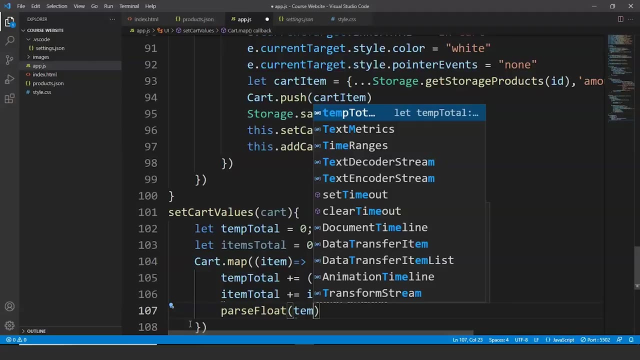 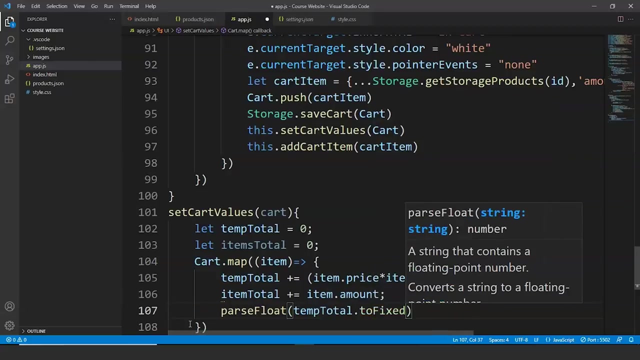 dot amount. fine, now we will write here parse float and we are going to change these values just like parsing. we have parse float as well, so inside parse float we will write time total dot to fixed and we are going to fixed it until two decimal units. fine, 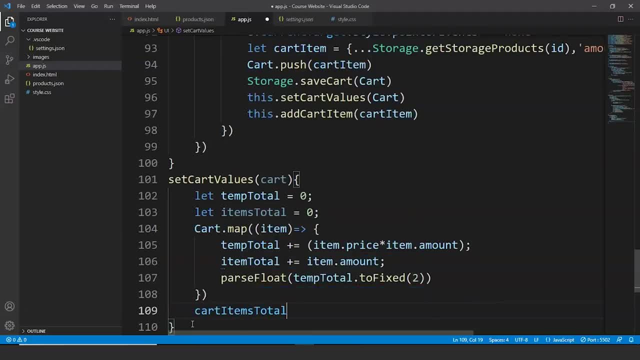 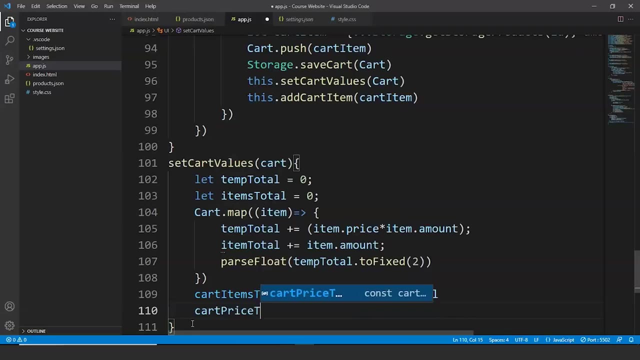 Next up. we will write here: cart items total dot. inner html is equals to items total and we will write here: cart price total dot. inner html is equals to parse float and we are going to change these values. so we will write here item total dot. we will write here: temp total. 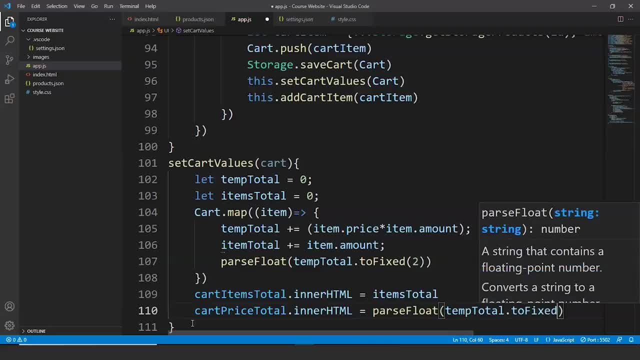 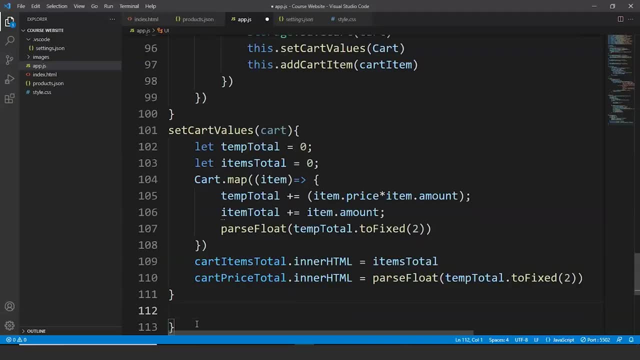 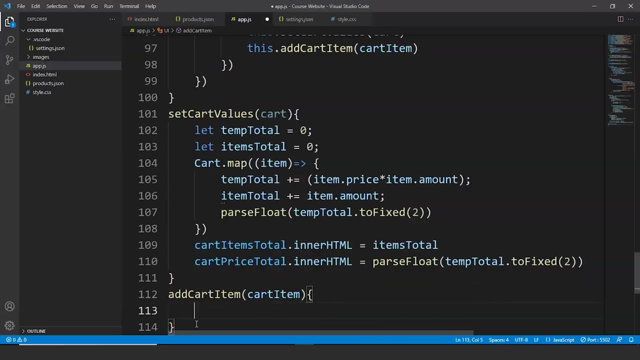 dot to fixed and we will fix it up to two decimal units. fine, Next up we will write here: add cart item. now we will write here cart item and we are going to change these values and inside this we will write: let cart item ui is equals to document. 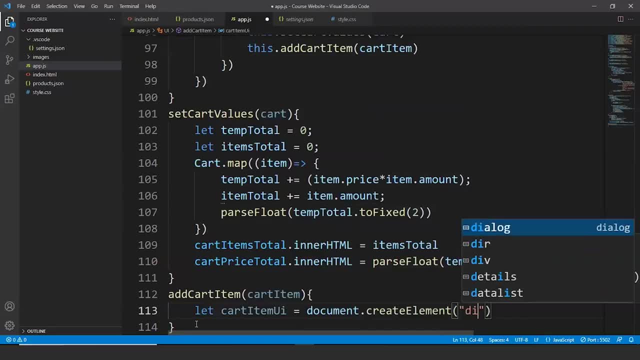 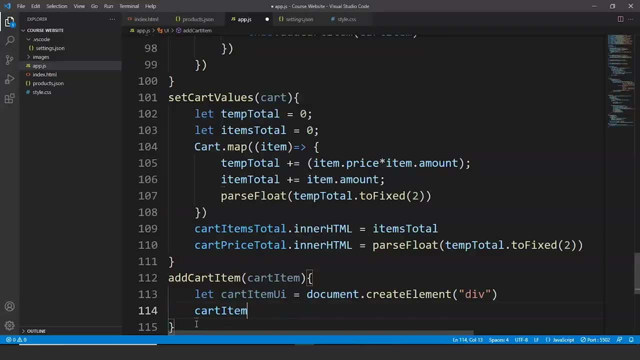 dot: create element. we will write here div. we will write here: cart item ui dot. inner html is equals to. we are again going to do the same task, so we are going to use the back tick for that. so here we will write div: class is equals to cart product. and we will write. 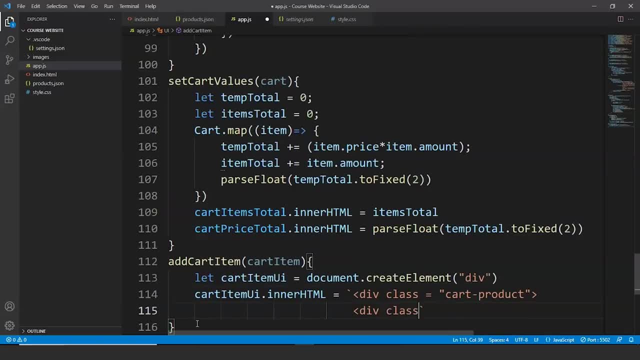 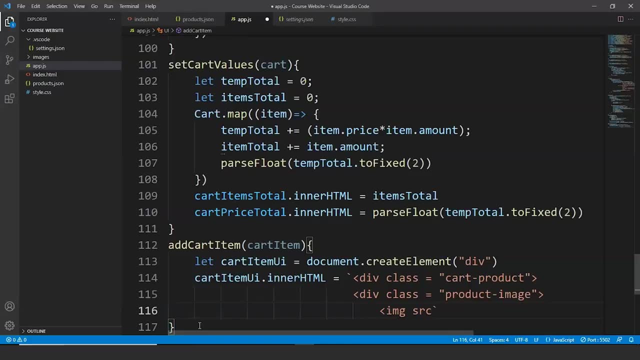 here div class, So we will write here div class is equals to cart item. and we will write here div class is equals to product image. we will write here img src is equals to- we are going to fetch the image again, so we will write here dollar and inside this we will write cart item dot. 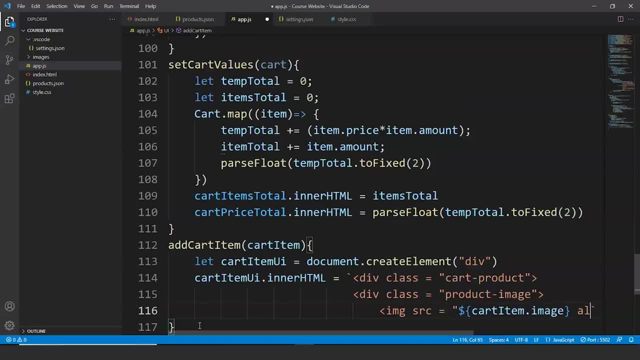 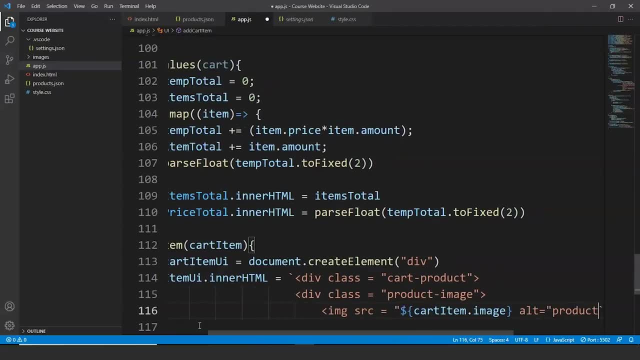 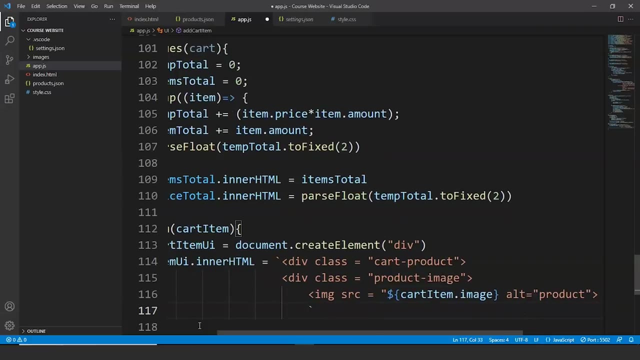 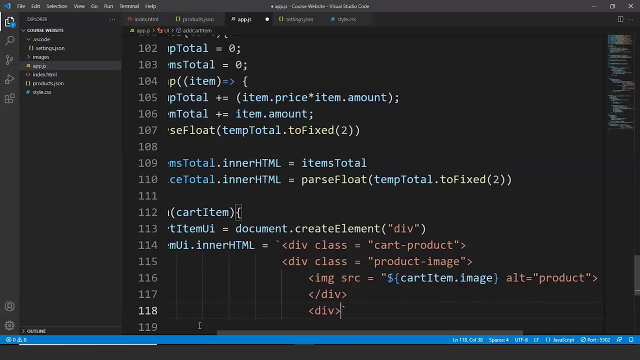 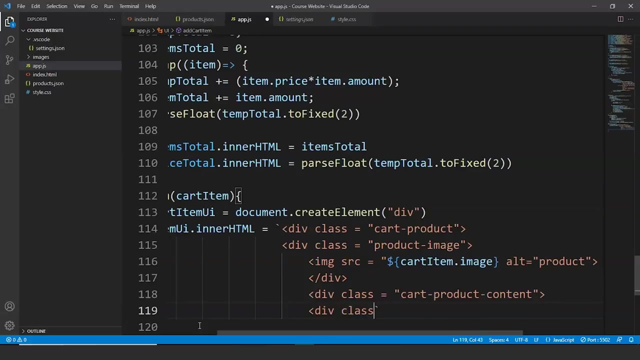 image and alt will be product in this case as well. next up, we are going to close this div tag and we are going to start another div tag here, so we will write here: div class is equals to cart product item. sorry, cart product content. we can say and then we will write here in the next line: div. 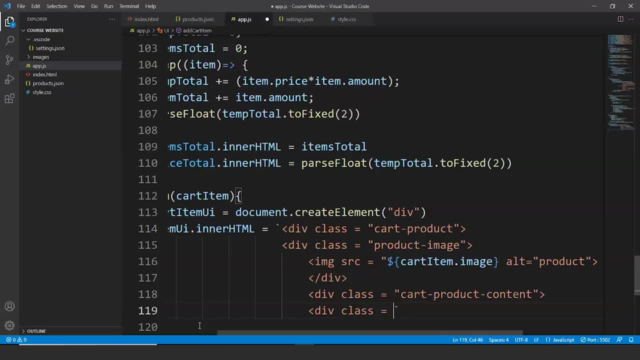 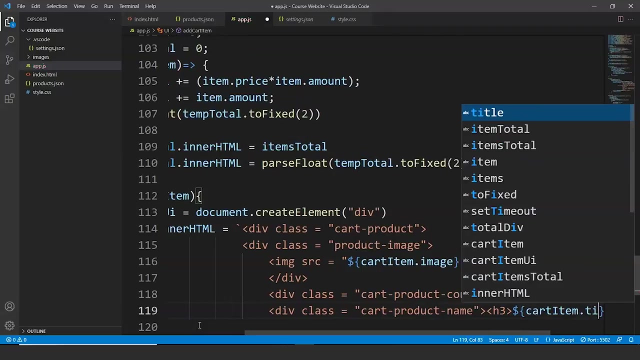 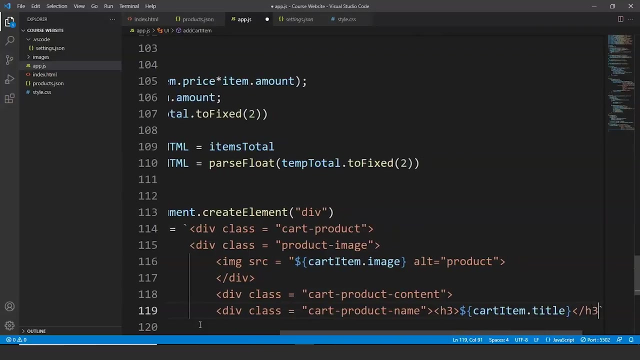 class is equals to halt src. div class is equals to good product name and then we will keep writing. sorry, we will write here inside h3 tag. so inside h3 tag we will write dollar cart item dot title and we are going to close this h3 tag over here. then we will close this div tag. 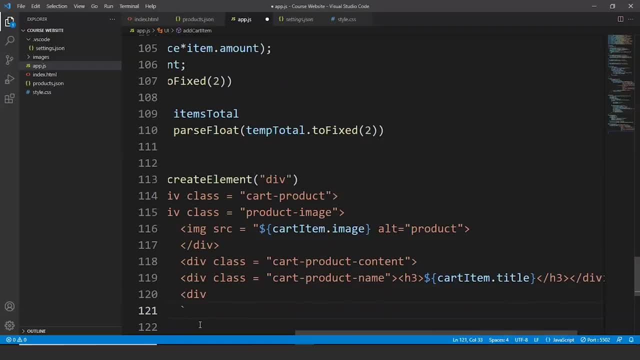 as well. we are again going to create another div tag. this time we are going to write: the class is cart product price. we are going to fetch the price now. we will write here again: h3. so our price is in dollars. so we will use dollars for now. we can use rupees here as. 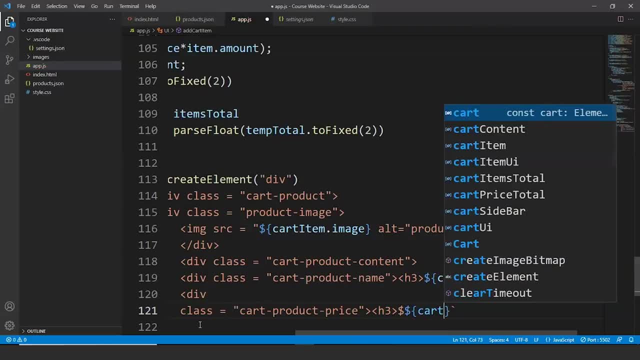 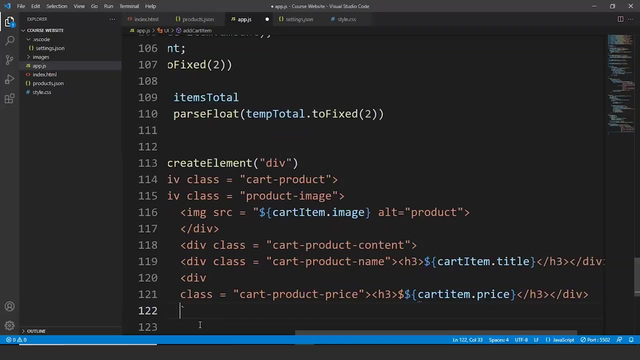 well, so we can write here: cart item dot price. the price is going to be in dollars. then we will close this tag and we are also going to close the dev tag here. fine, in the next line we are going to create the product removed cart. so we are going to create 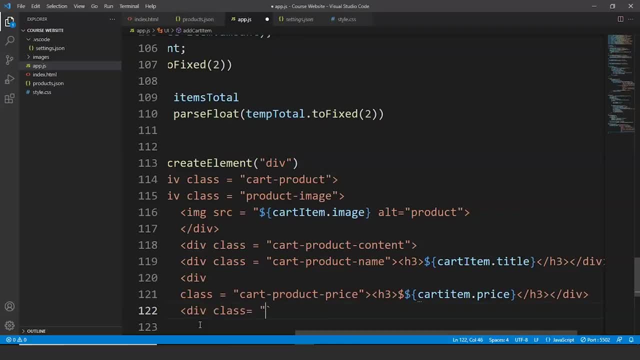 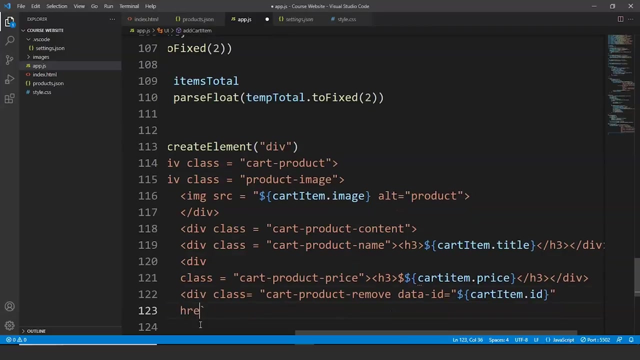 a div tag for that and the class is going to be cart product remove. data. ID is going to be cart ID, So we'll write here: cart item dot ID. And then we'll write here: href is equals to hash And style is going to be, color is going to be. 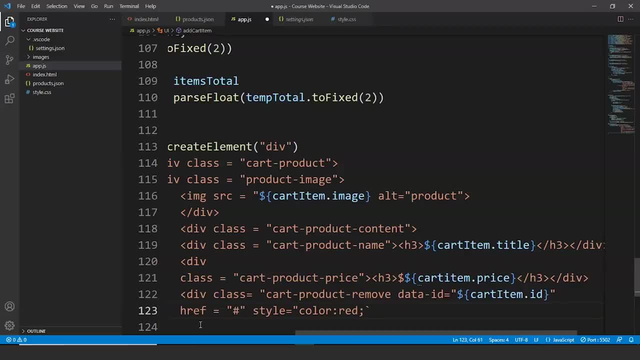 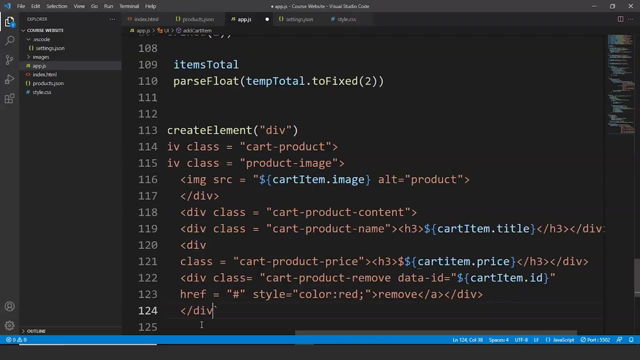 red. Then we'll write here: remove. I'm going to close the anchor tag and then the div tag. Fine, So we are done with this till now. then we are going to again close this particular div tag we used previously. Now what we are going to do is we are. 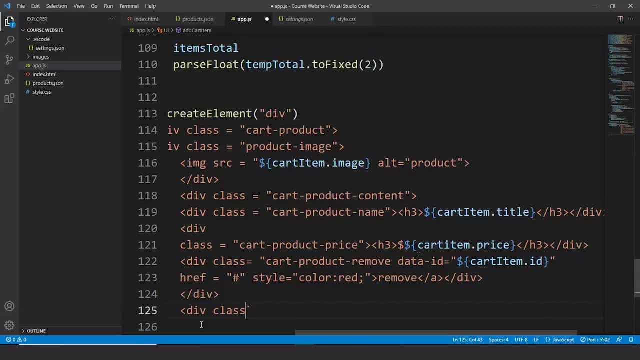 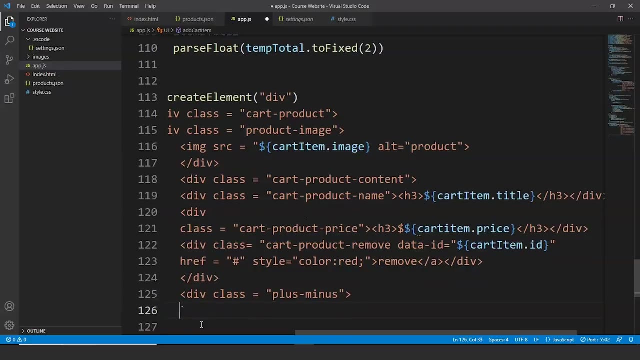 going to change the number of products, So we are going to use here: class is equals to plus, minus and here we'll write inside the I tag: class is equals to far, far angle left add amount. Fine, This is going to be the class. 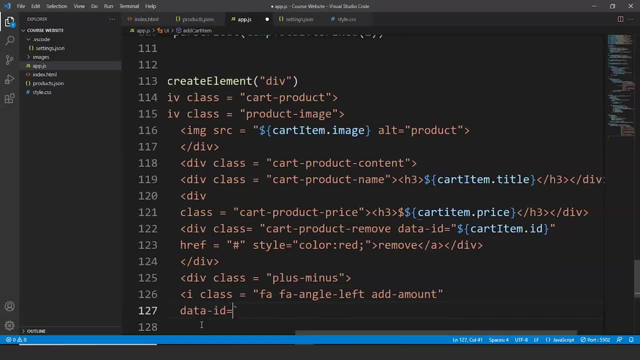 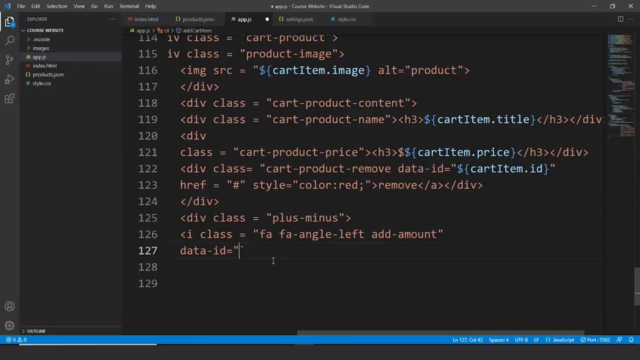 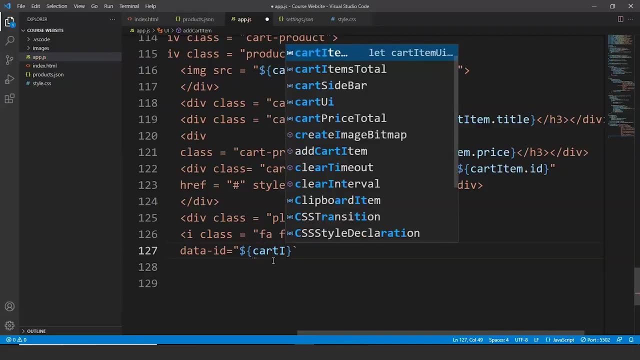 And the data ID is going to be cart item ID. So we are going to write here: data ID is equals to dollar And inside this will write cart item ID, dot ID, And then we are going to close this tag and we are going to close the. 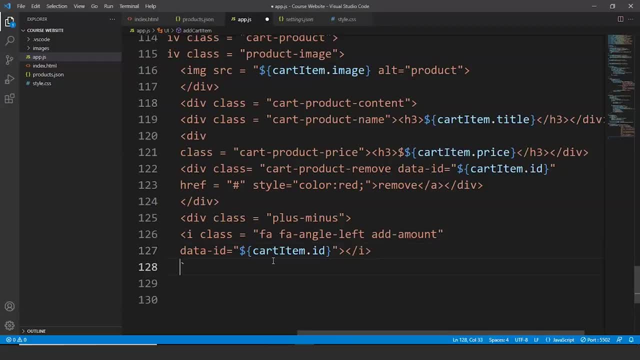 I tag here: Fine. Next up, we are going to use the span tag Again. we are going to write here: span class is equals to number of items, And we'll close this tag. here we'll write dollar cart item dot amount. We are going to close the span tag here, So we'll. 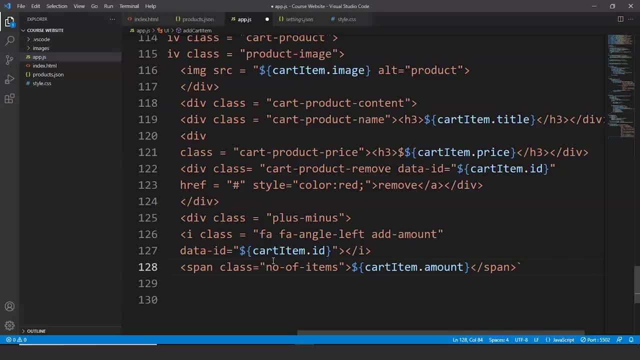 write here slash span. In the next line we are again going to use data ID, And here what we'll do is we'll write here dollar and we'll write here cart item dot ID. We are going to close the I tag again And in the next line we are going to: 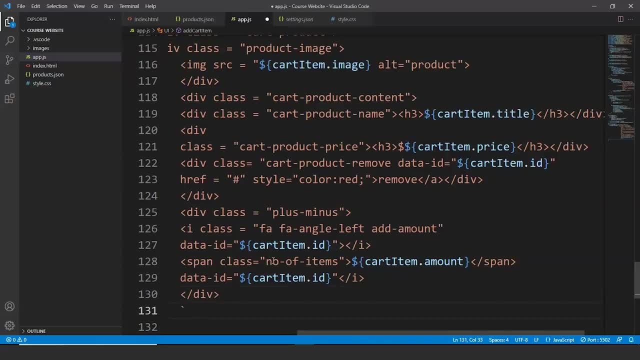 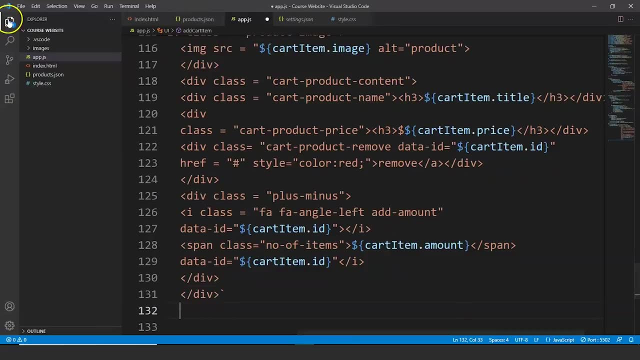 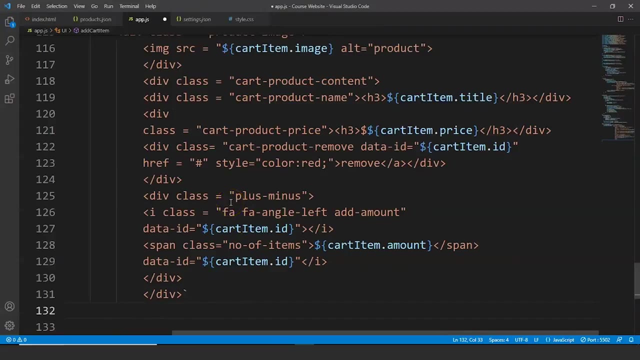 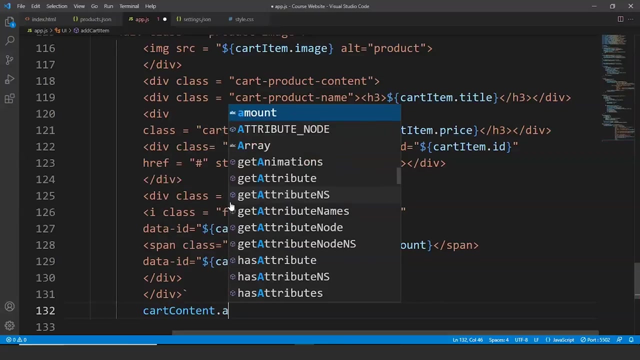 close the div tag And one more div tag. Fine, Now we are done with it. Let me close this first And next up, we'll append this cart content to the cart item UI. So we'll write here: cart content, dot append, And inside this: 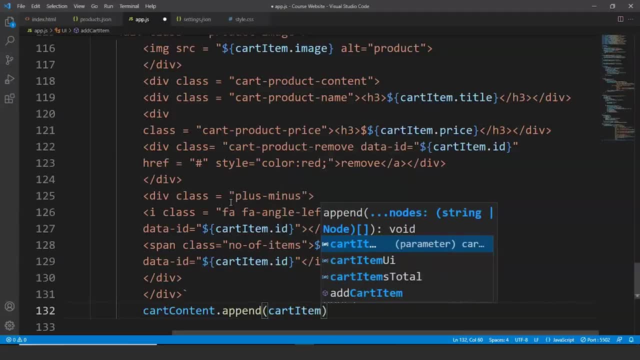 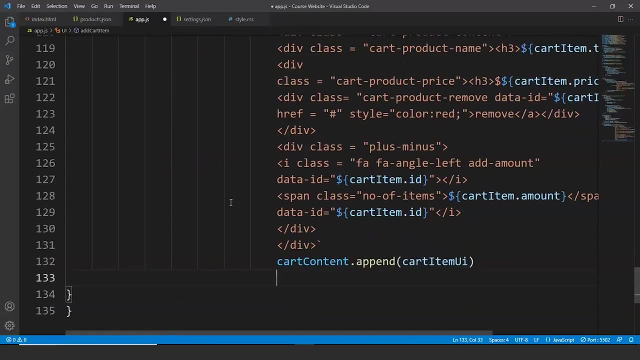 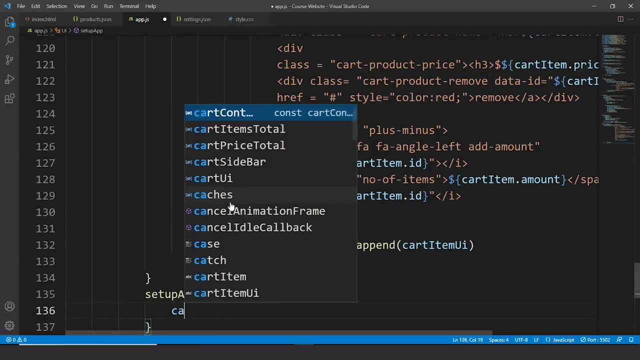 we'll pass cart item UI: Fine. So here you can see we are going to close. close this, So this is the closed one, And inside here we'll write setup app Again, constructor. we are going to write here: cart is equals to. 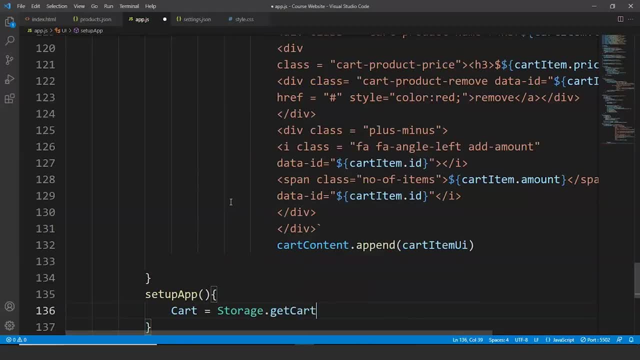 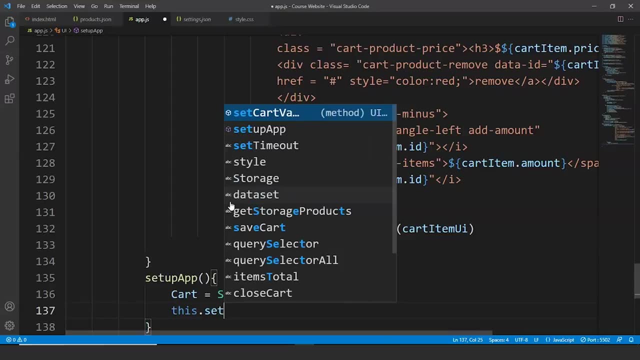 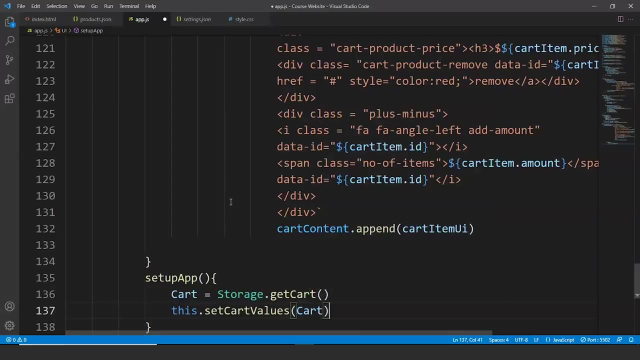 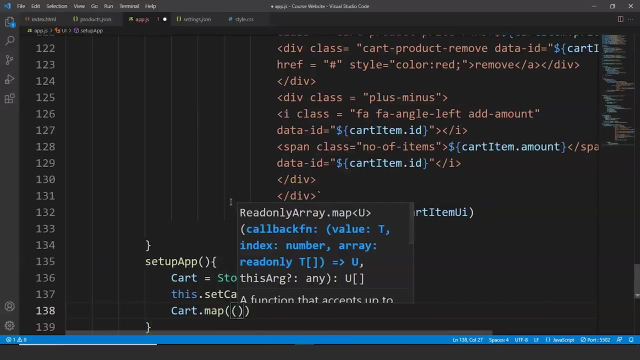 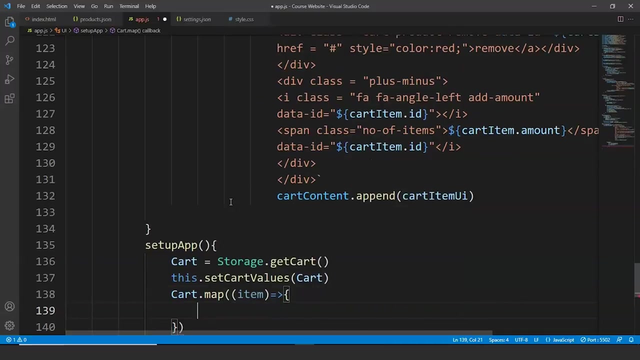 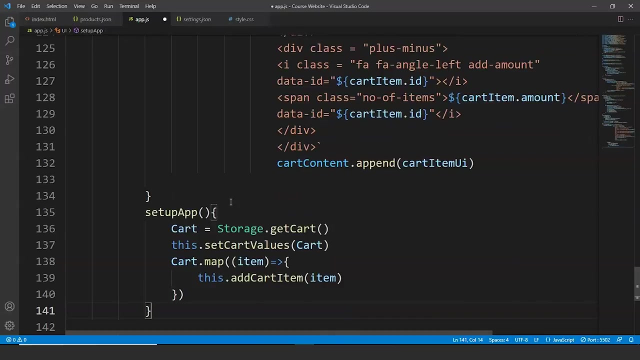 storage dot get cart. We'll write this dot: set cart values cart here And then we'll write cart dot map. Inside this we'll write item And inside the body we'll write this dot: add cart item, item. Fine, I hope you guys are getting this. Next up, we'll write the cart. 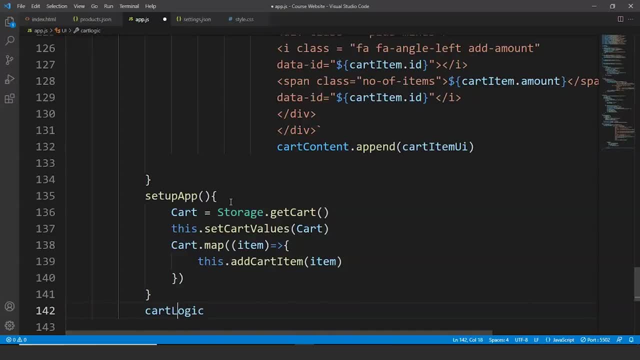 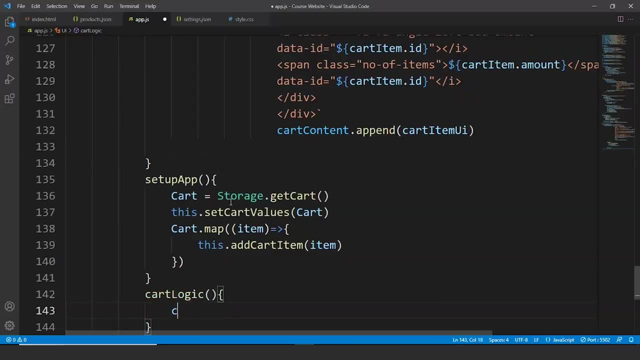 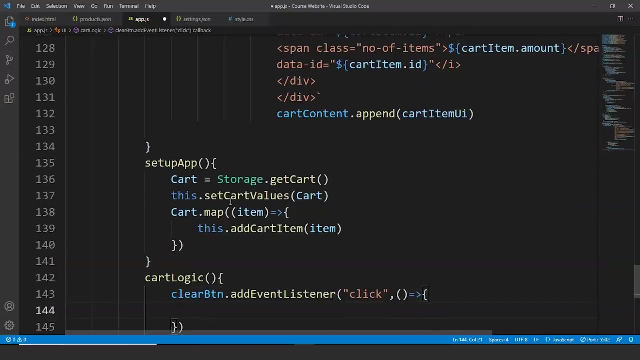 logic. here We'll write a cart logic And we'll write here: clear button- dot. add event listener. We are going to create an event again. we'll write here: click comma function. Inside this we'll write this: dot clear cart. we are going to call this function over here. Now we have. 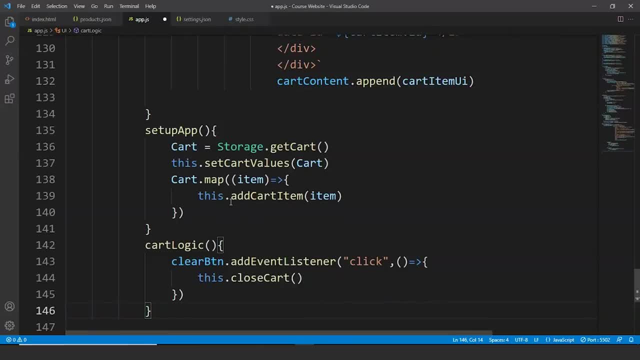 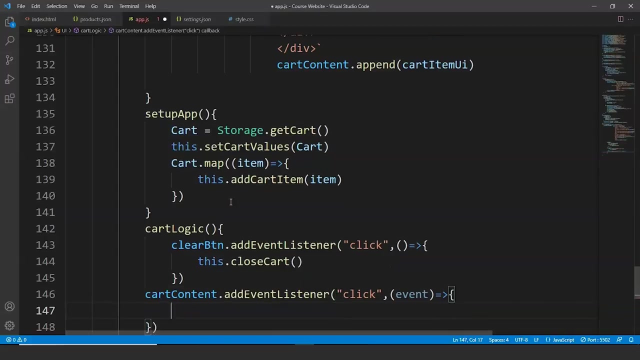 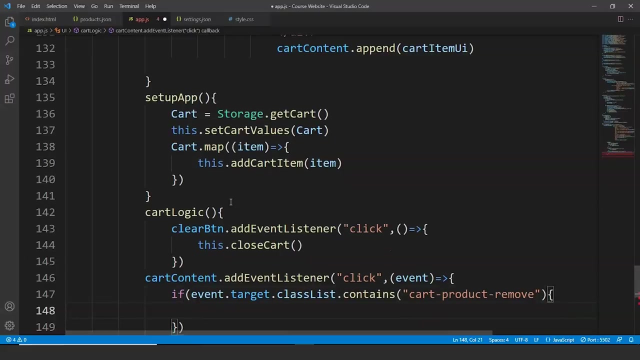 to write the logic for remove button. So we'll do it here. We'll write here: cart content dot. add event listener, Click comma event And we will write here inside this: if event dot target Class List dot contains cart product remove, then will again create a variable. let's say the variable is let. 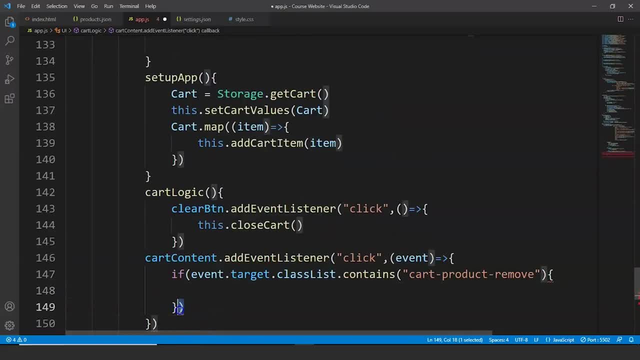 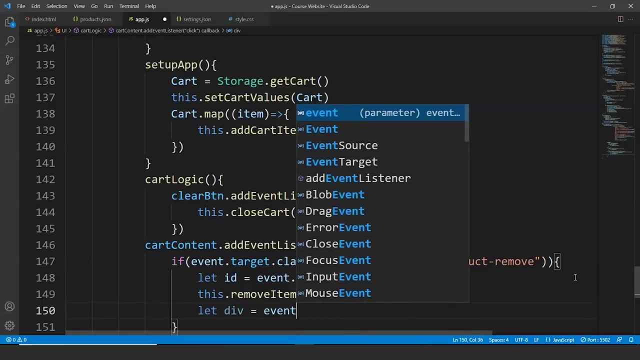 okay, we have made a mistake over here. we have to close this bracket here and then we have to write here: let ID is equals to event dot. target dot. data set dot ID. the next line will write this dot remove item and will pass ID here. fine, in the next line we'll write here: let div is equals to event dot. 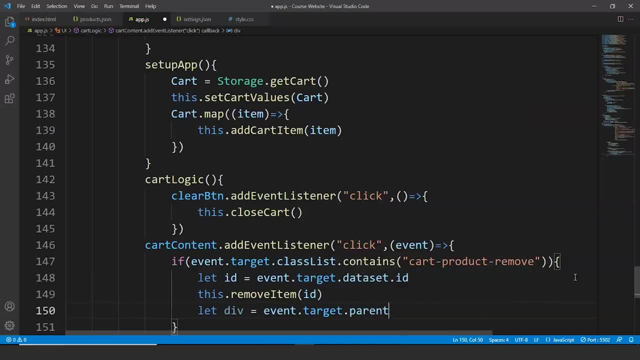 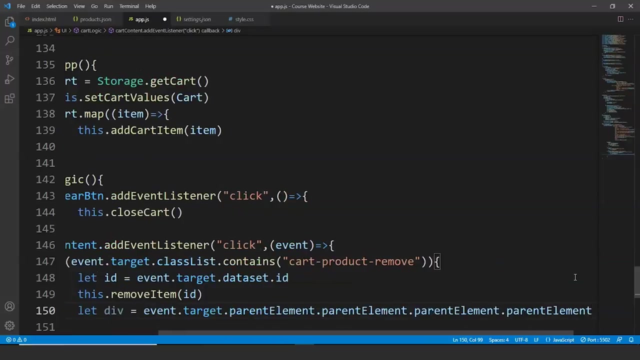 target: dot parent element. and we are going to use parent element for quite some time now, so we are going to write here dot parent element again for four times. so we will write here: parent element, dot- parent element. so we have written it four times here. in the next line we'll write here: div- dot remove. 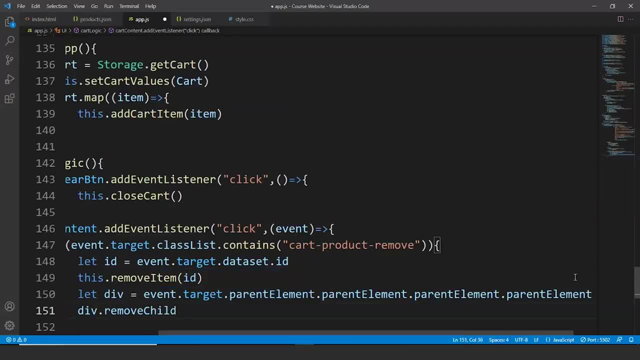 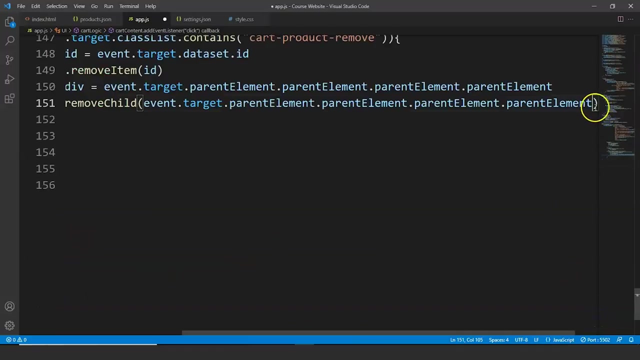 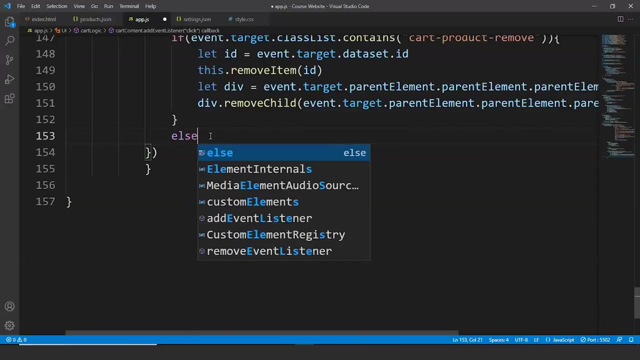 child and will write here: event dot, target dot will copy this like that. it from here and we'll paste it here. fine, now in the next line, we are going to close this bracket and we are going to start writing here else: if event dot, target dot, class list dot contains: 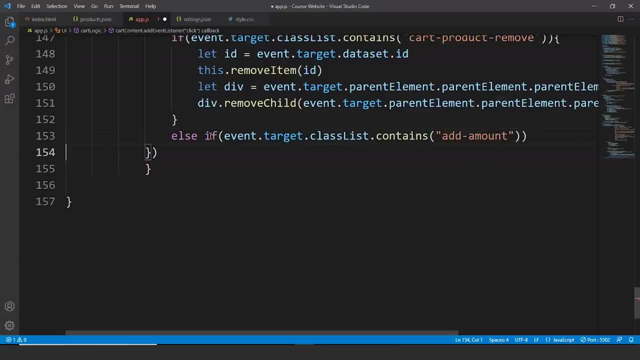 add amount. then what we are going to do is we are going to use the ID variable again. we are going to write a: let ID is equal to event dot, target dot, data set dot ID. let item is equals to car dot. fine will pass item here and 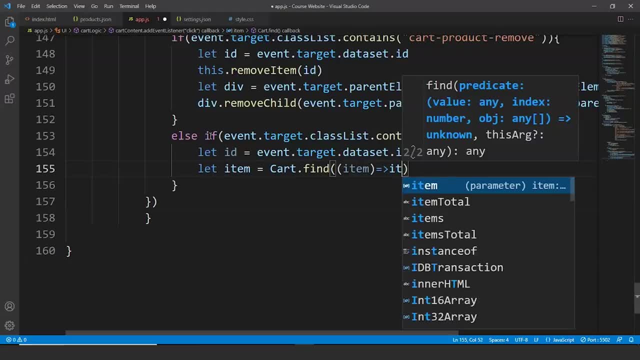 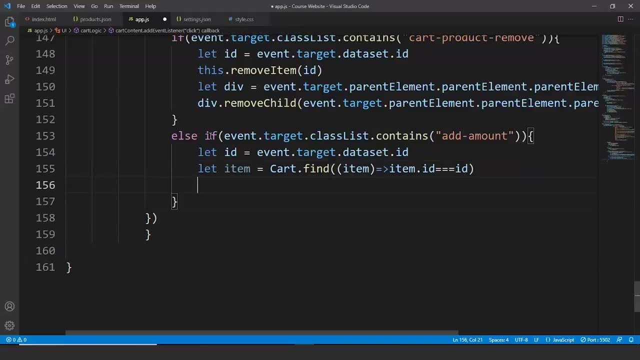 will use arrow function. so we'll write here: item dot- ID equals to ID. fine, then we'll write here: item dot- amount plus plus. so we are going to increase the amount of items. then what we are going to do is we are going to write a storage dot. 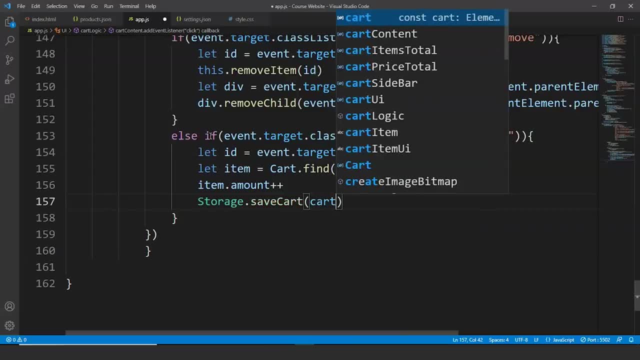 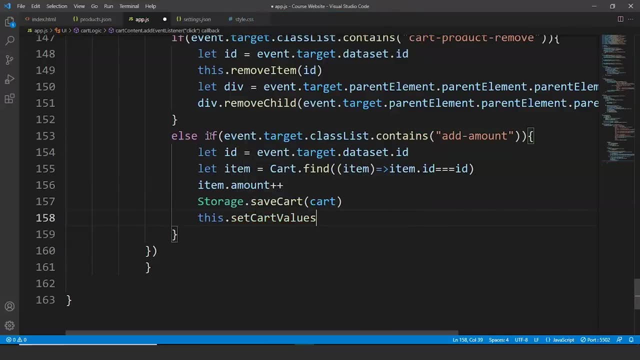 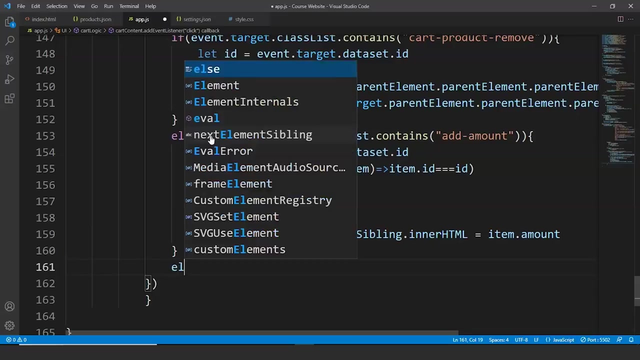 save cart and we are going to pass cart here. we'll write here this dot: set cart values cart. we'll write here: event dot. target dot. next element: sibling dot. inner HTML is equals to item dot. amount. fine, now we are going to use another else if here so 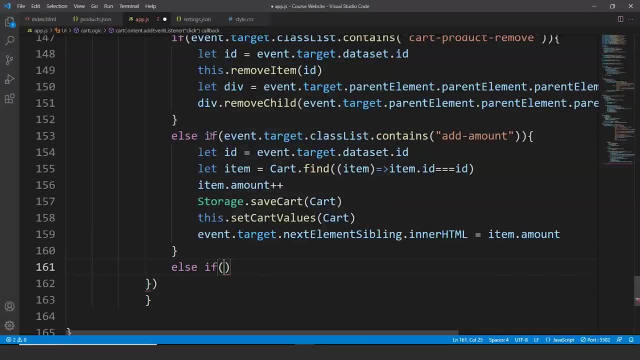 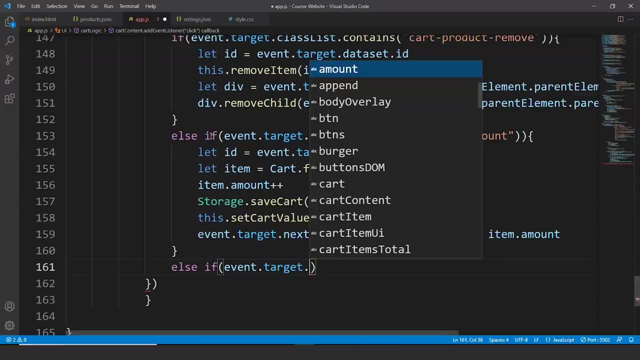 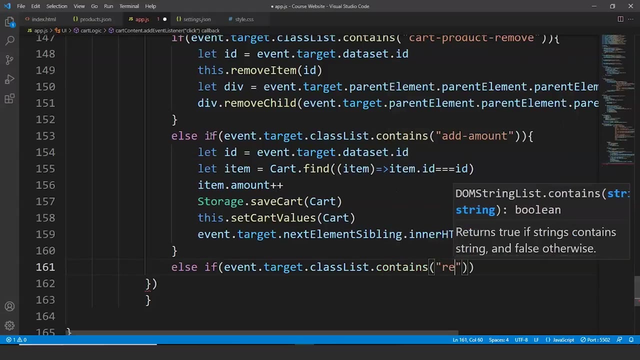 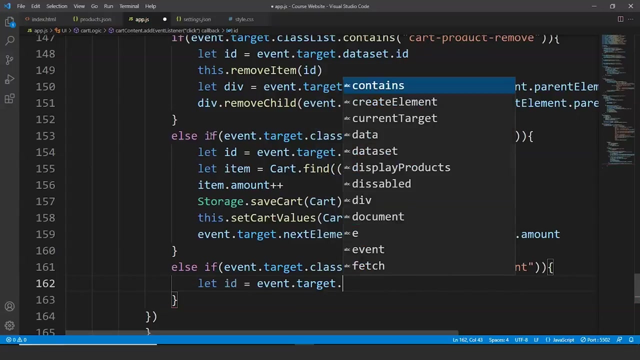 we will write here. else, if event dot targetclasslistcontains reduce amount. So we are going to change the number of products in our cart. So for that, what we'll do is we'll write here: let id is equals to eventtargetdatasetid, fine, and item will be. 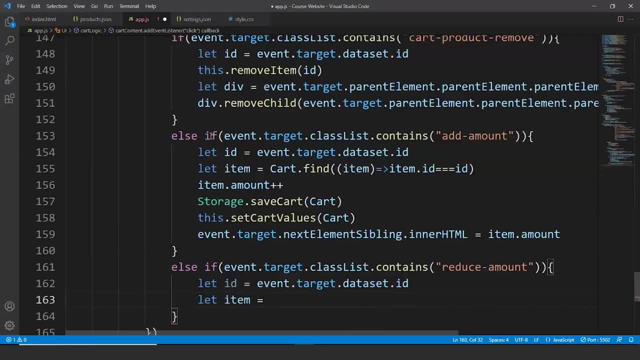 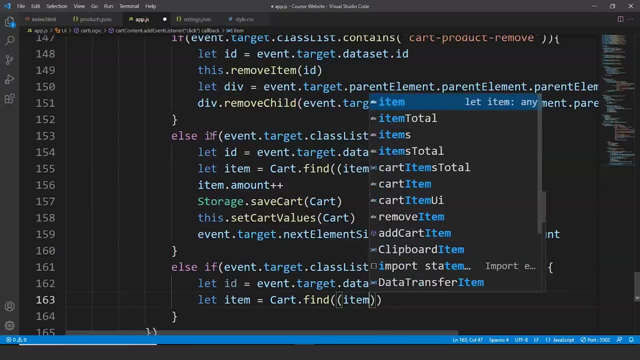 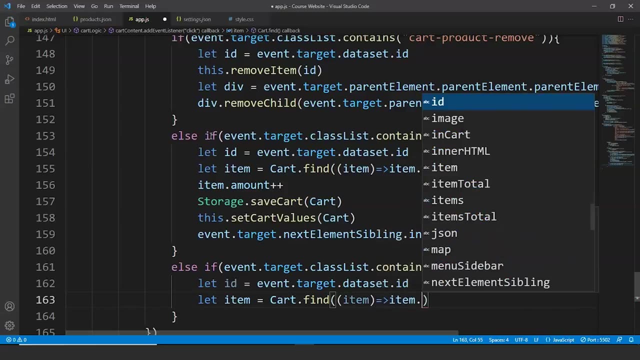 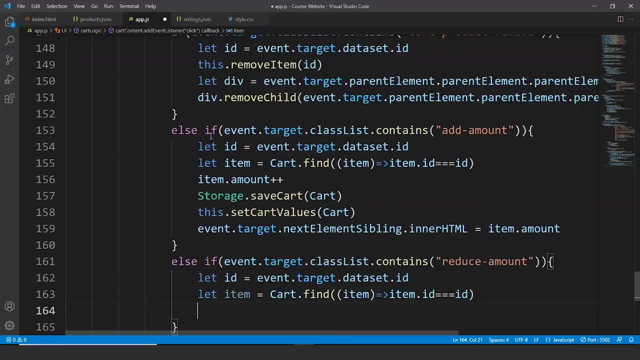 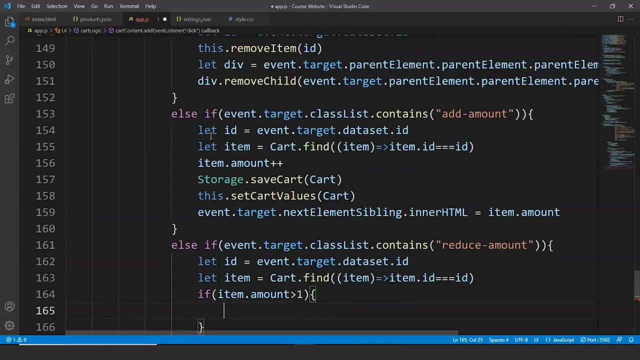 let item is equals to cartfind. itemid triple equals to id. if we are again going to use an is statement, so we'll write here: itemamount is greater than one. if the number of items is greater than one, then itemamount minus minus and store it inside the cart. 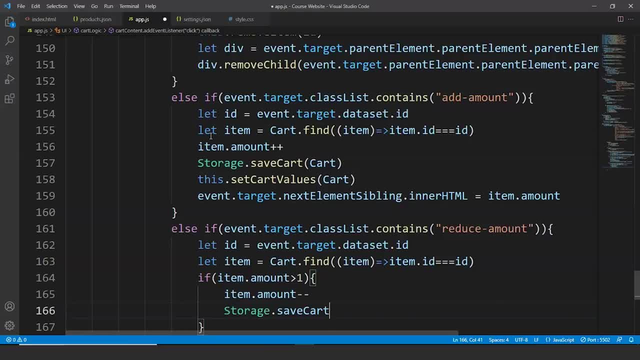 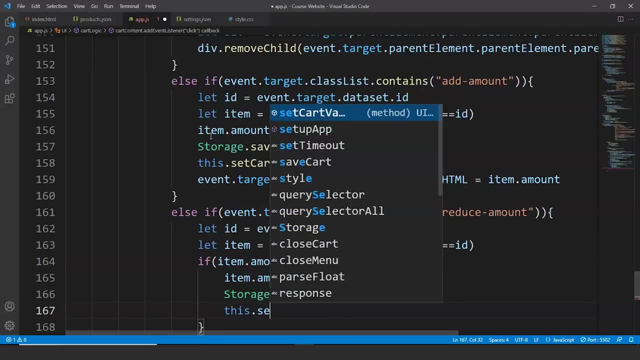 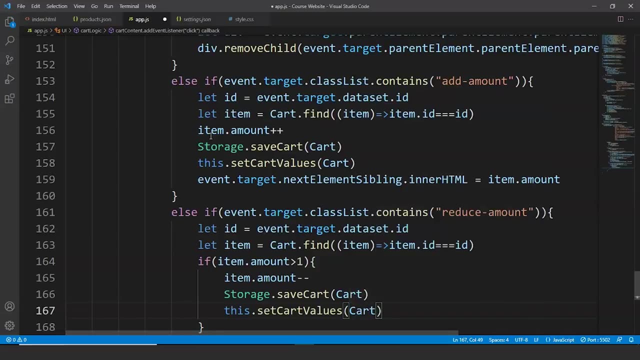 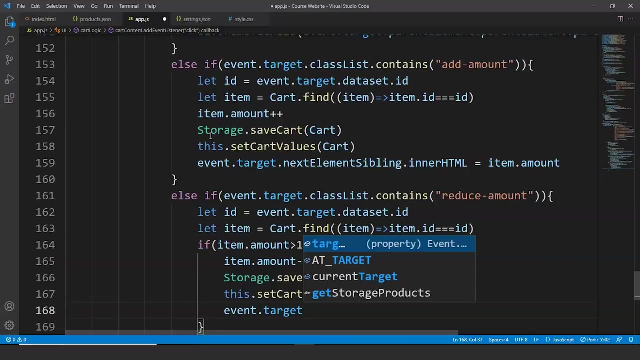 So we are going to write here storagesavecart, and we'll pass cart here. Then we'll write here thissetcart values and we'll again pass cart here. In the next line We'll write here: eventtargetprevious element siblinginnerHTML is equals to itemamount. 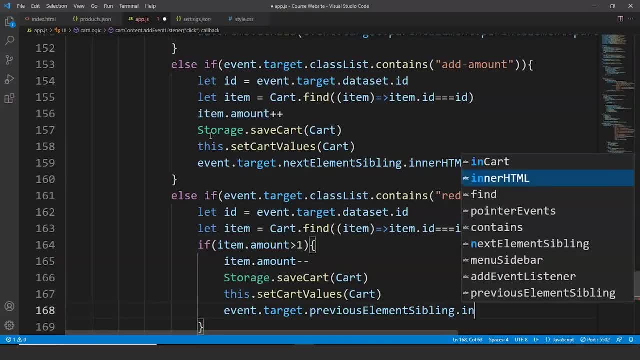 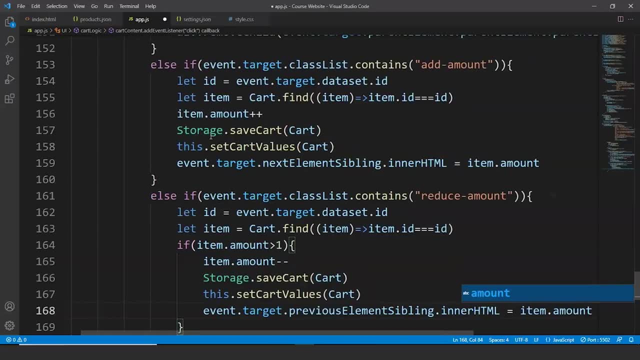 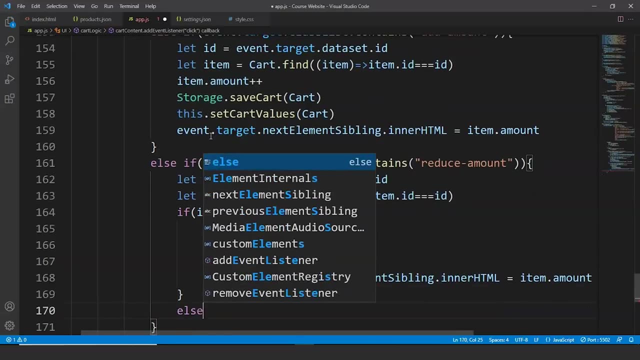 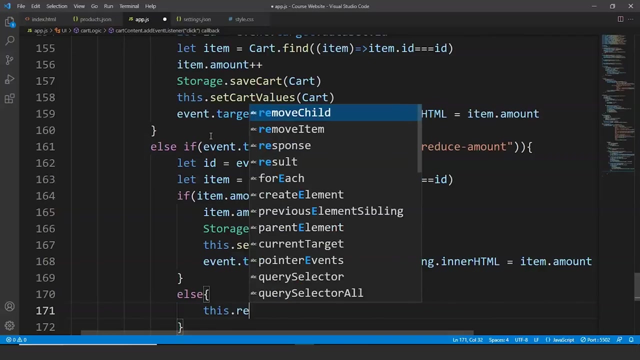 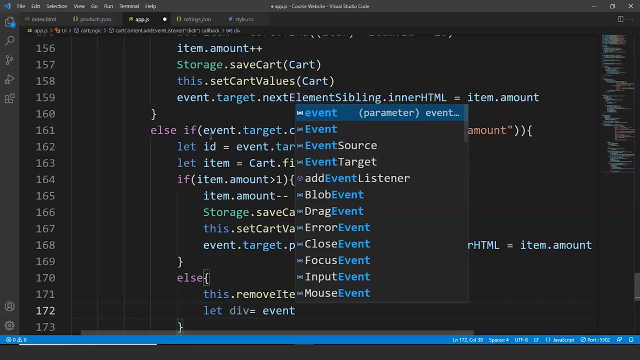 And finally we'll write here else inside the else, what we'll do is we'll write here this dot remove item and we'll pass the ID. you will write here: let div is equals to event dot target. we are basically targeting the events. we are creating conditions for certain. 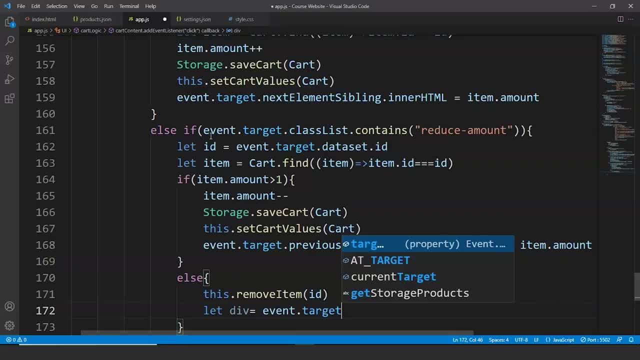 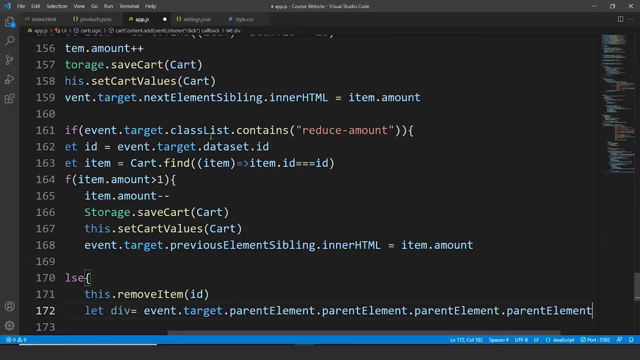 different events, like when the user increases the number of products and the user decreases the number of products, and if the user removes the product from the cart. so we are writing the code for that. so we'll write a event, dot, target, dot, parent element and we'll write here parent element again for four times. fine, 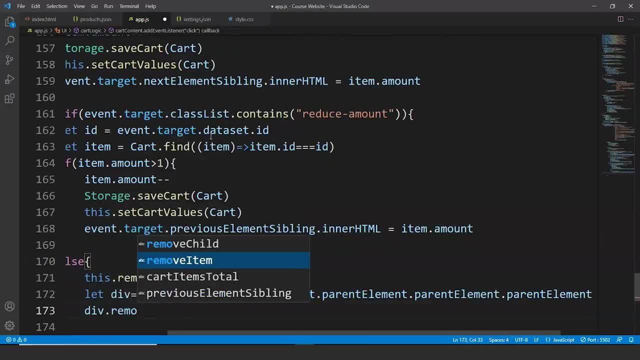 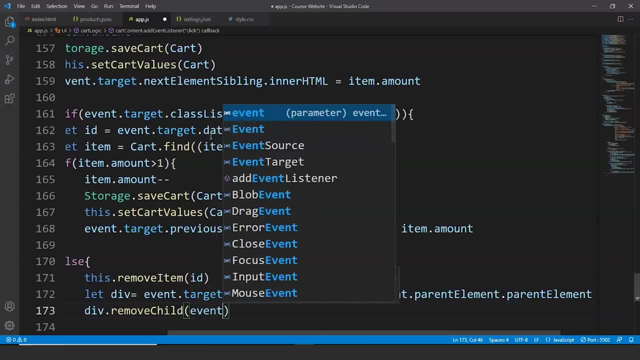 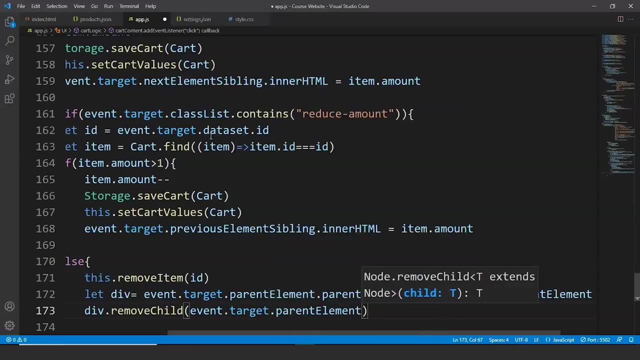 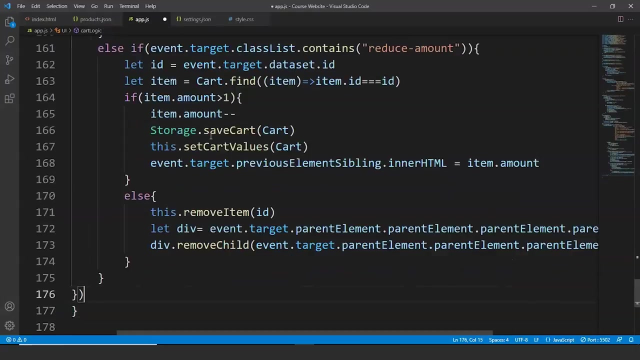 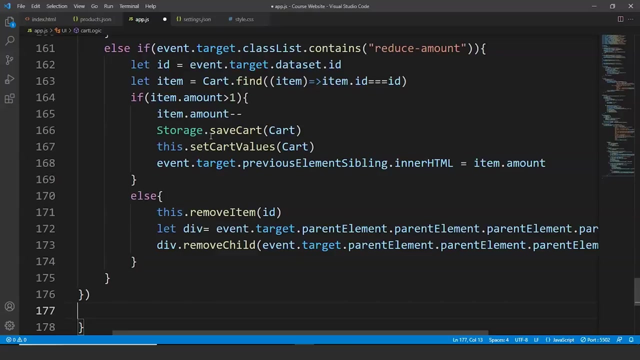 we'll write here: div dot- remove child, and inside this we will write let event dot. target dot, parent. Schritt 2, element four, four times again it will check each parent element. so here we are done with it. next up, we have to create two functions for ad amount and. 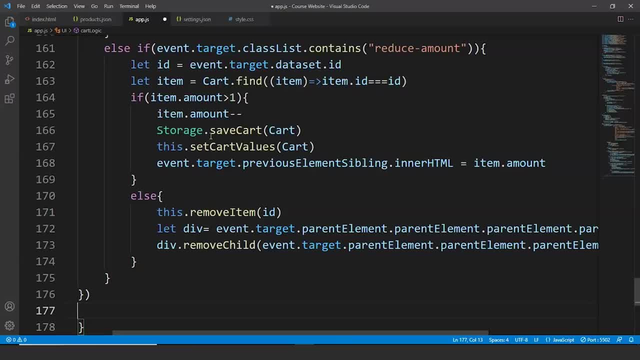 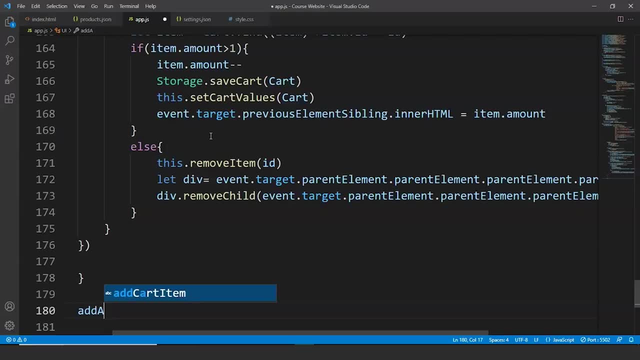 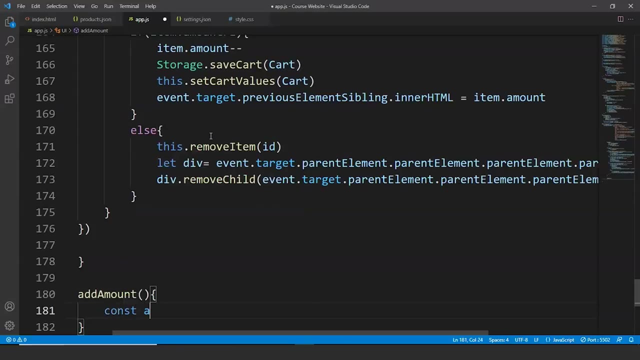 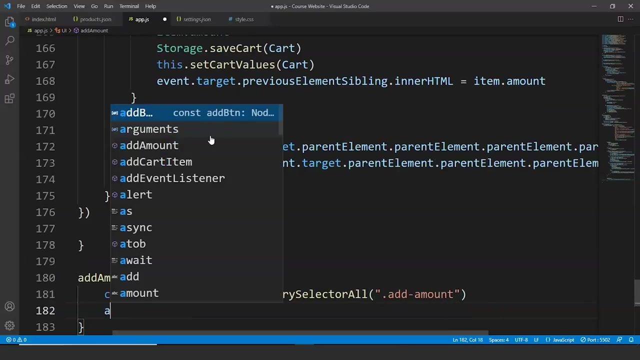 and for reduce amount. so what we are going to do is we are going to write here add amount and we'll write here const. add button is equals to document dot query selector. all inside this we'll pass dot add amount. fine, we'll write here: add button, dot for each. 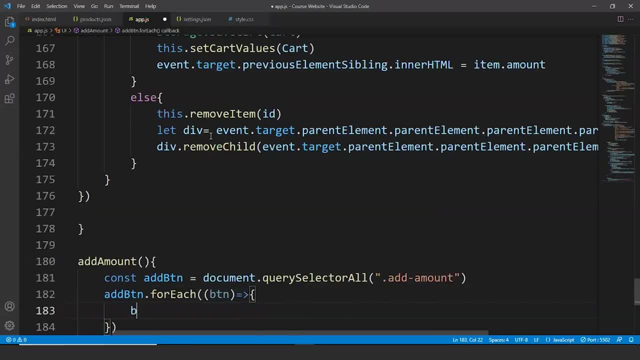 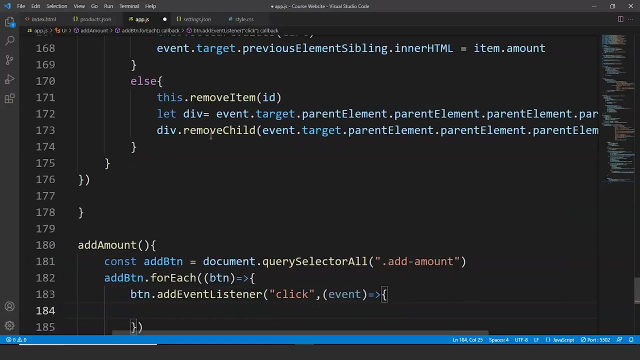 and we'll write here inside this button: dot add event listener and we'll add an event over here. we'll write here: click comma event. we'll pass event here and then we'll write here like this: let id is equals to event dot. current target dot. data set dot id. fine, we'll write here: cart dot- map. 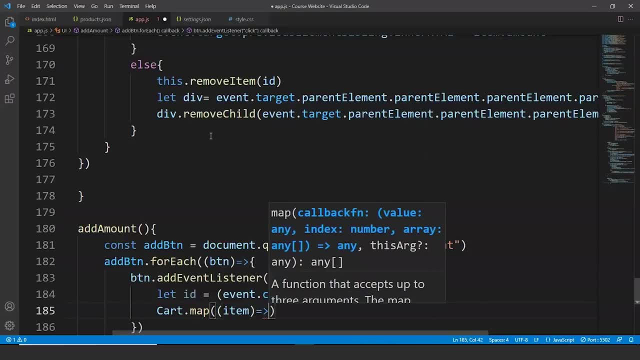 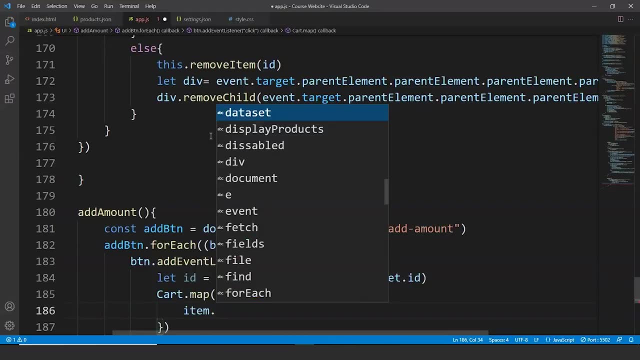 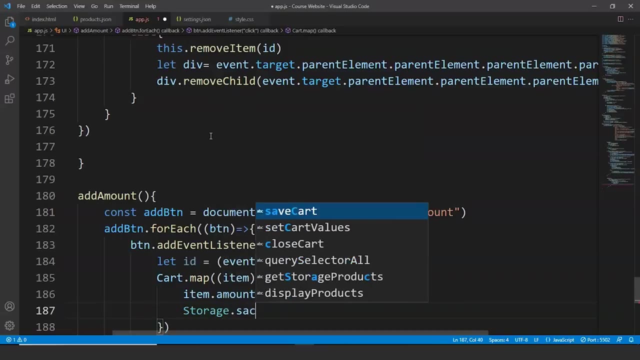 and we'll pass item over here. we'll write here again arrow function and inside this what we are going to do is we are going to write here item dot. amount plus plus storage dot. save cart. we are going to pass cart here. we'll write here this dot. 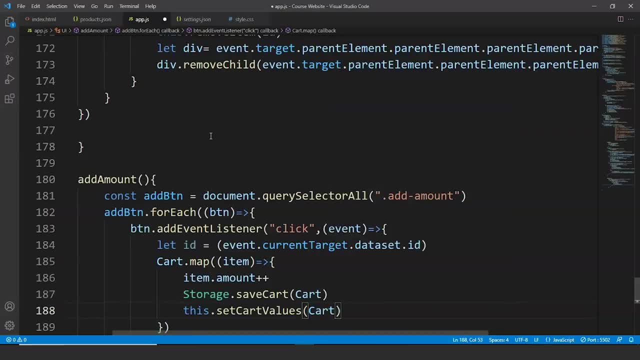 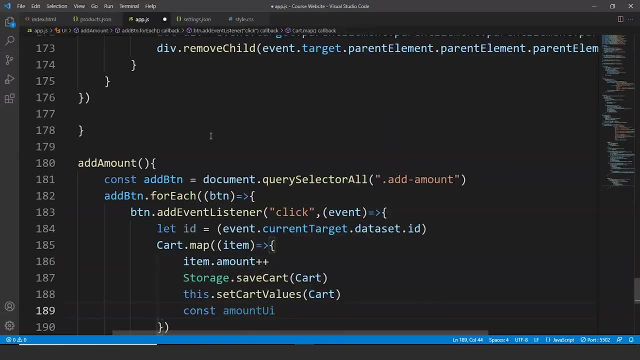 set cart values. we are again going to set the cart values and we'll again use amount ui, a new variable, and we'll write here: event dot. current target dot. parent element dot- children. fine, so we are targeting the parent element along with the children, so we'll write here: 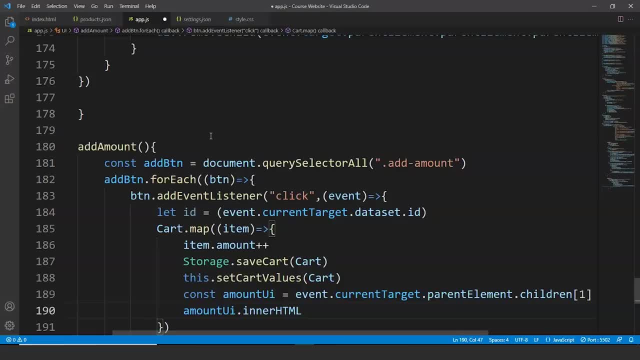 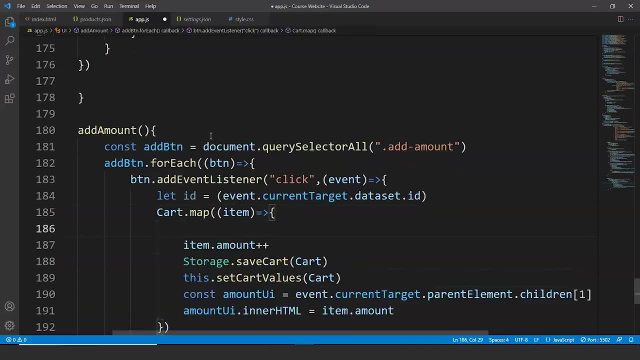 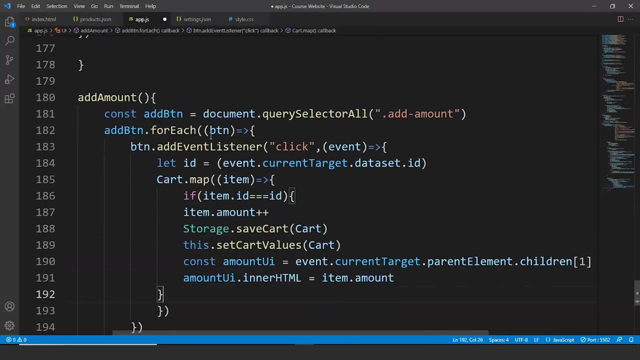 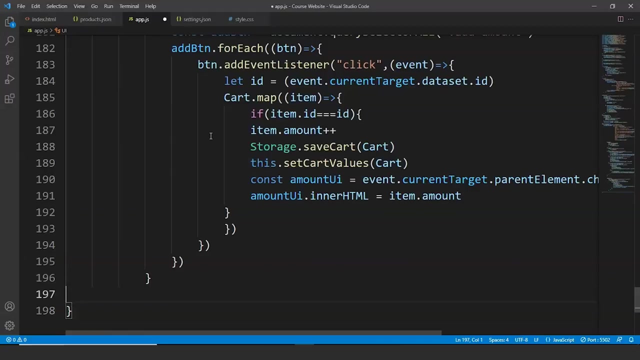 amount. ui dot inner html is equals to item dot amount, so we have forgot to mention here. if item dot id is equals to id, then do it fine. now we are going to do the same thing for reduce amount as well, so we'll write here: reduce amount. 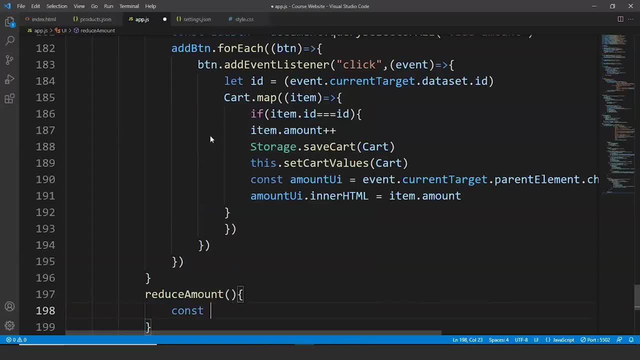 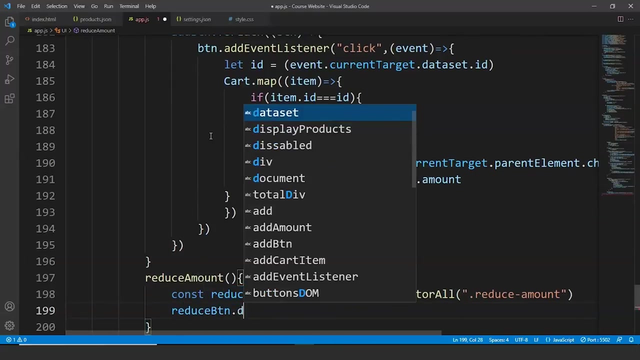 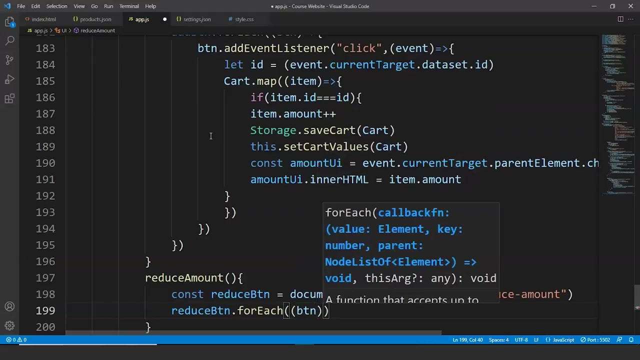 and inside this we'll write: write const reduceButton is equals to document dot, querySelector all. and we are going to pass here dot reduceAmount. fine, we will write here: reduceButton, dot foreach. then we will pass button over here and we will use the arrow function again. finally, we will write: 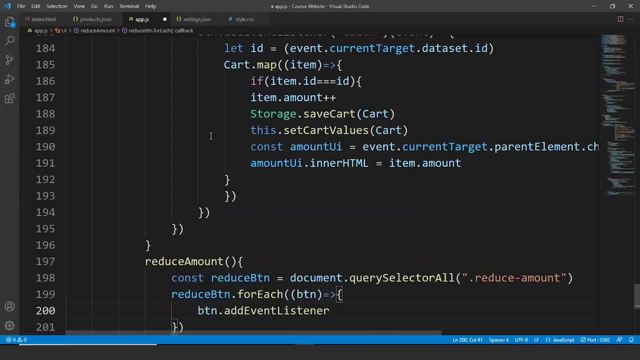 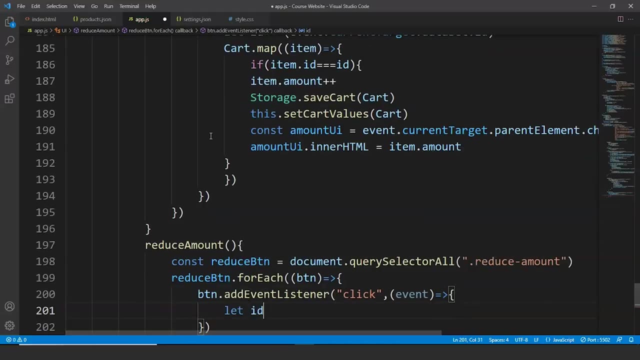 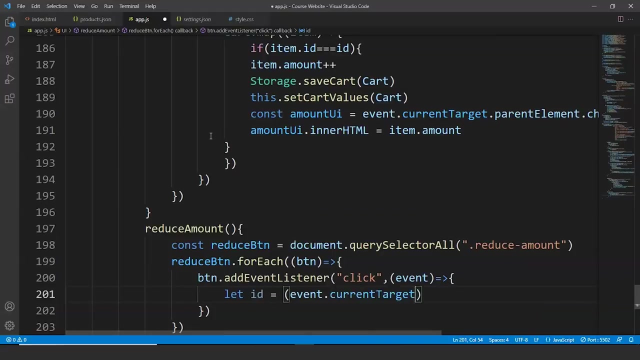 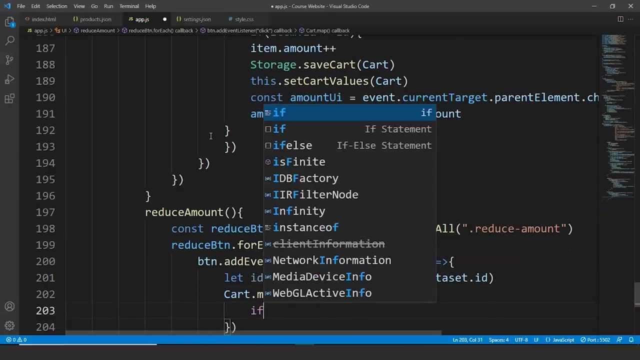 here button dot addEventListener, click event, let id is equals to event dot. current currentTarget dot dataset dot id. eventcurrentTarget dot dataset dot id. fine, we will write here cart dot map. we will map it to cart and we will write here item. then again we will write here: if item dot id triple equals to id, then we will write. 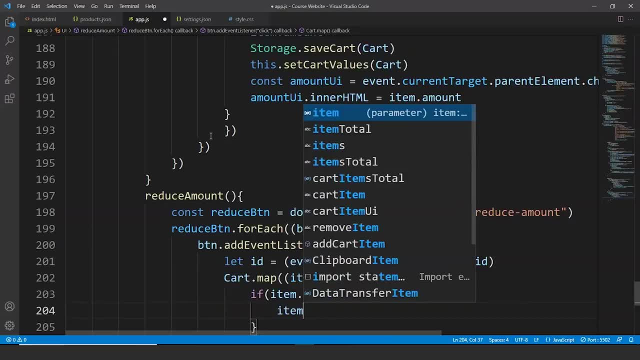 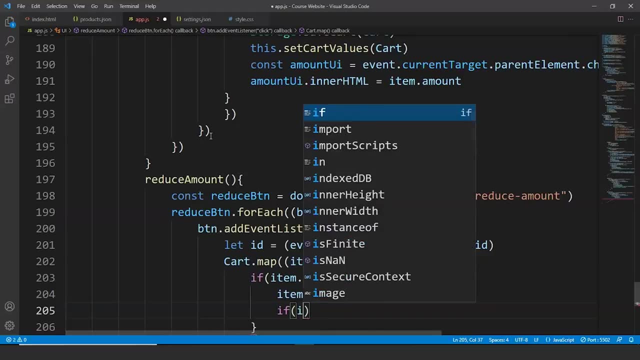 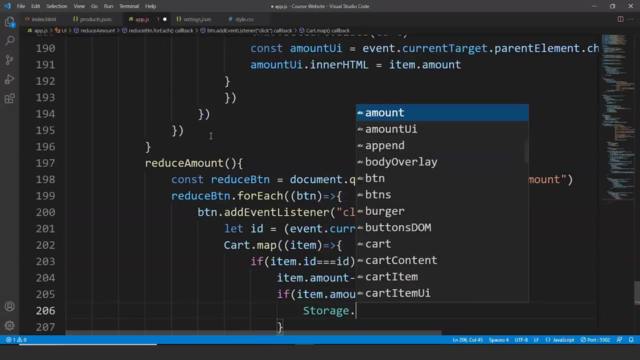 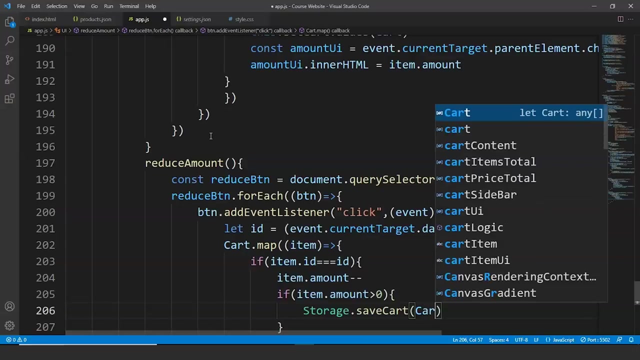 here item amount minus minus. So we will write here item dot amount minus minus. and if item dot amount is greater than zero, then what it will do? it will store it inside the local storage. So we will write here storage dot save cart and we will write here cart. 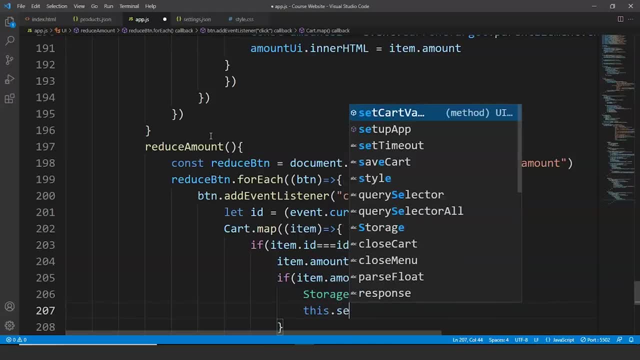 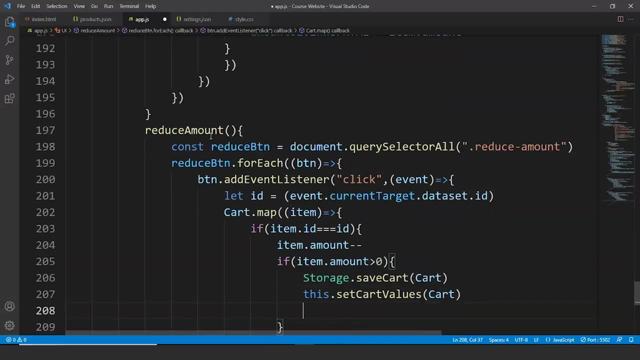 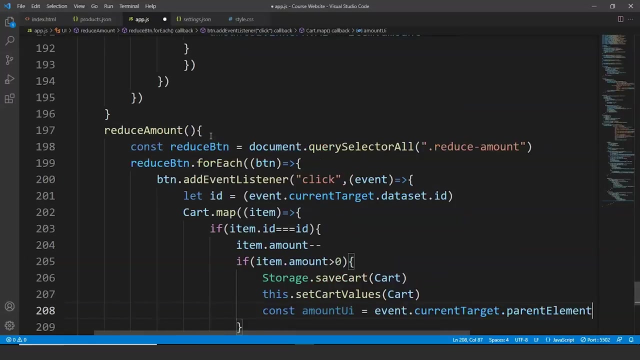 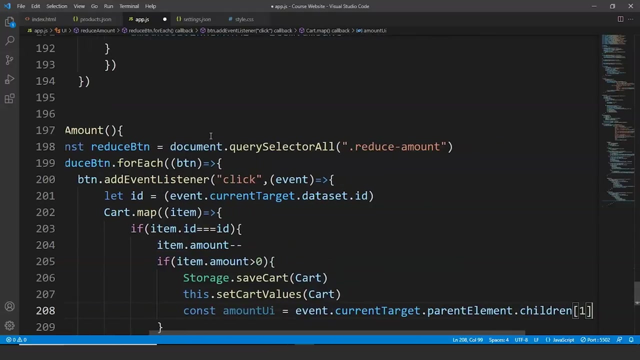 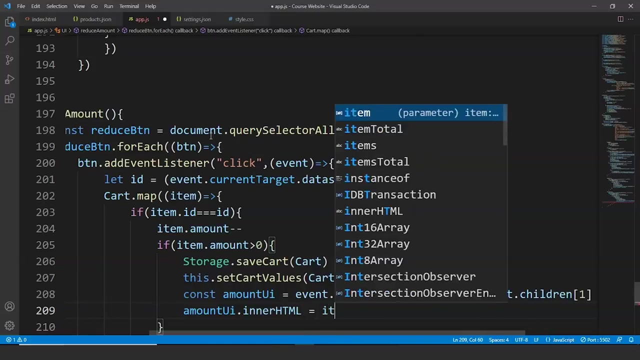 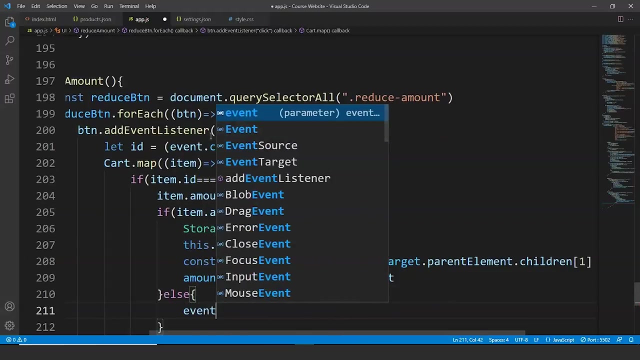 then we'll write this: dot set cart values. cart const amount ui is equals to event dot currentTarget, dot parentElement and dot children amountUiinnerHTML is equals to itemamount. fine, again, we will write here else. else what will happen? we will write here: eventcurrentTargetparentElement. 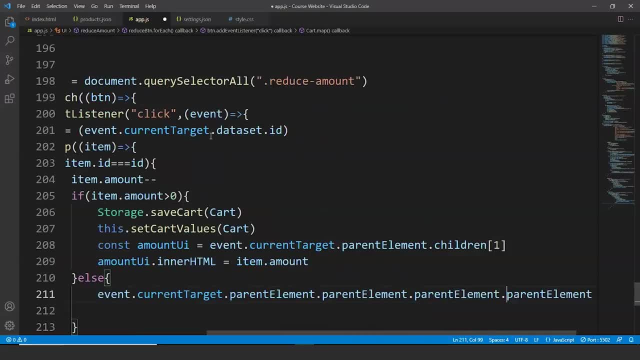 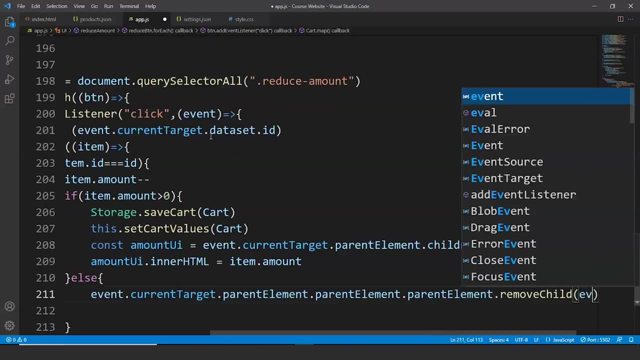 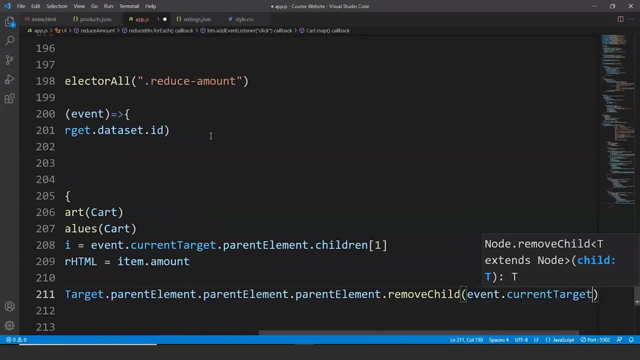 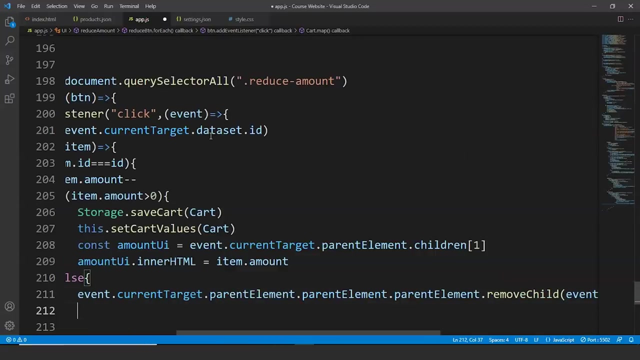 so here instead of parent element we will write removeChild, and we will write here: eventcurrentTargetparentElement- dot. parentElement, dot. parentElement. fine. and the next line we will write this: dot- remove item and we'll pass ID. here We are done with this part as well. Next up, we have 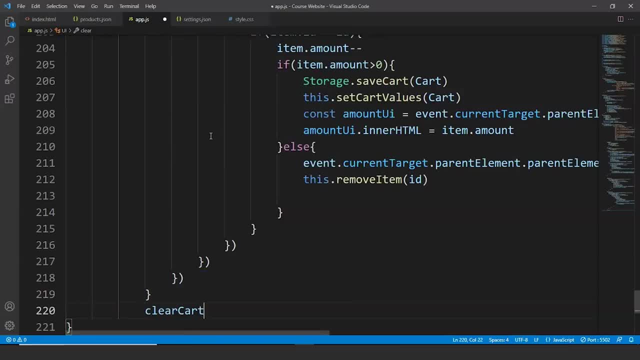 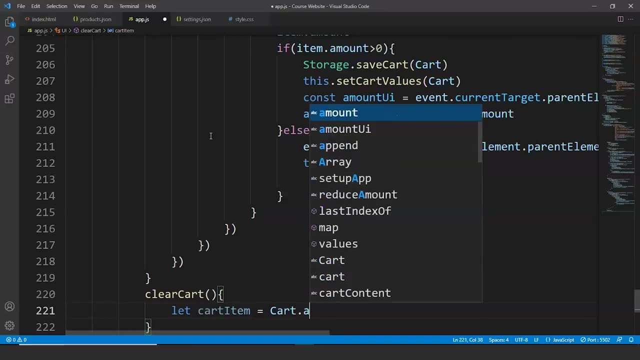 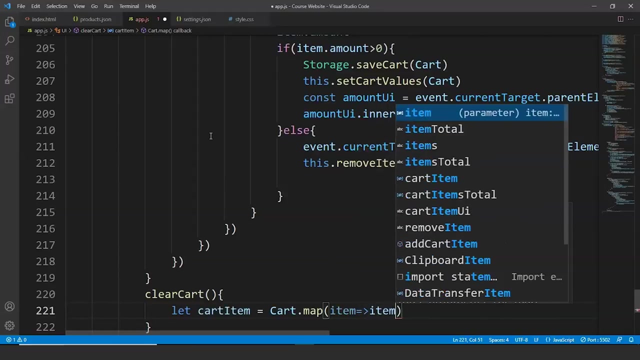 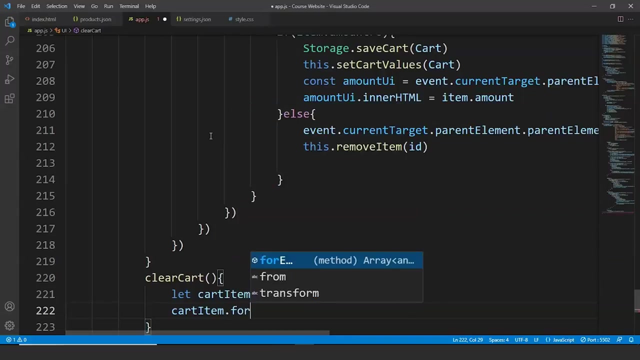 to clear the cart. So for that we'll write here: clear cart. We'll again do something. for that we'll write here: let cart item is equals cart dot map. inside this we'll write: item implies item dot, ID, cart item dot. we'll again use the for each loop. here we'll write: 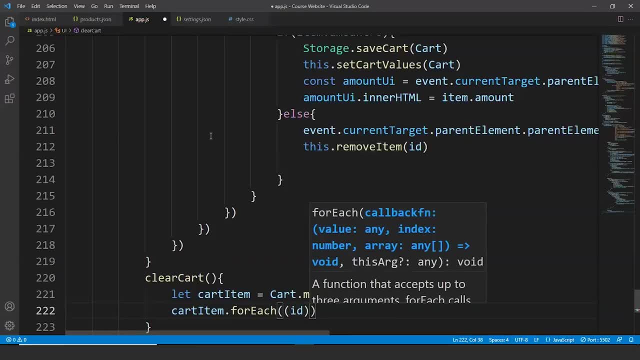 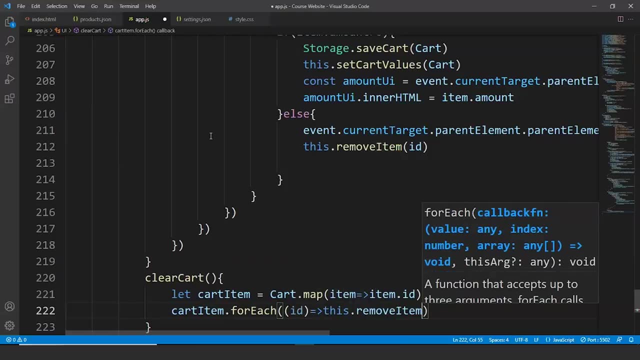 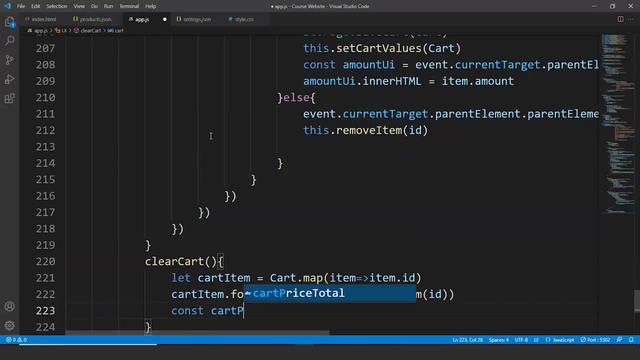 here this. then we'll provide ID here and we'll write here this: dot remove item. we'll pass the ID over here. Then we'll write here this: dot remove item. we'll pass the ID over here. Then we'll write here: const cart product. we'll create a new variable here. we'll write here: document dot. 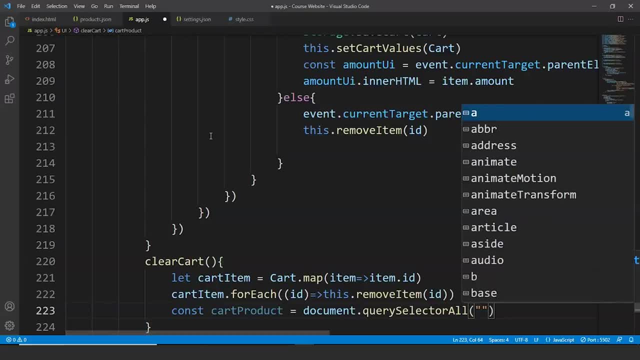 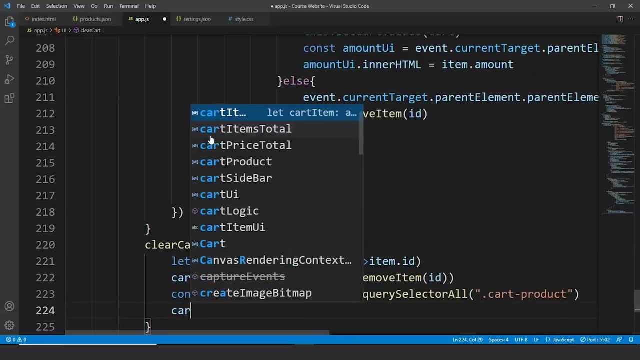 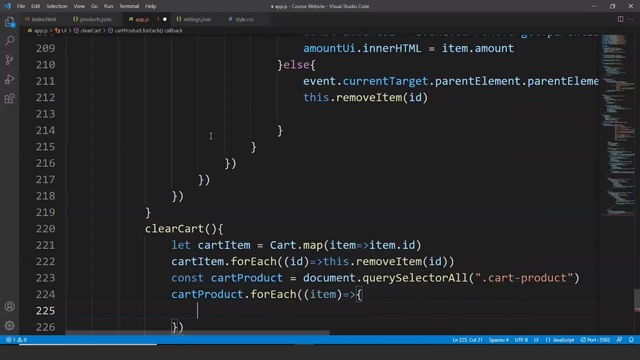 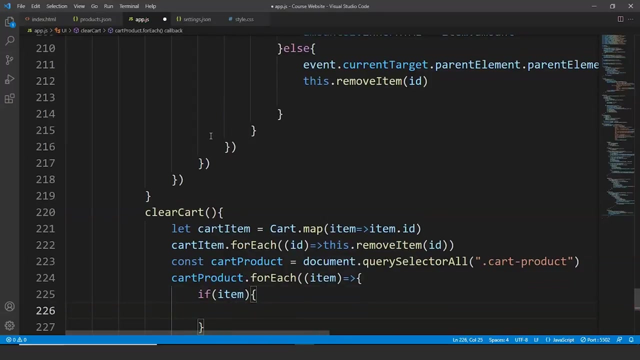 query selector all, and we'll write here: dot cart product. We'll write here: cart product dot for each, for each item. what we're going to do is we're going to create an arrow function here and we're going to write here if item is true, if item is there, then item dot parent. 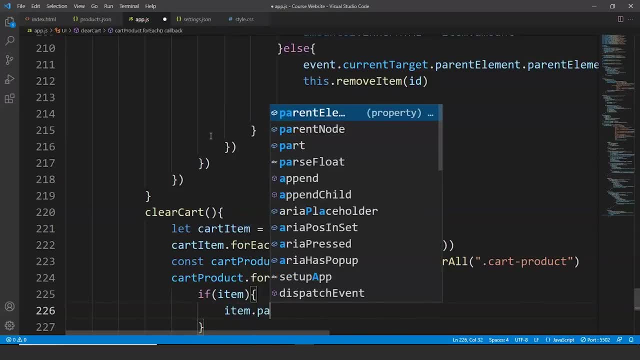 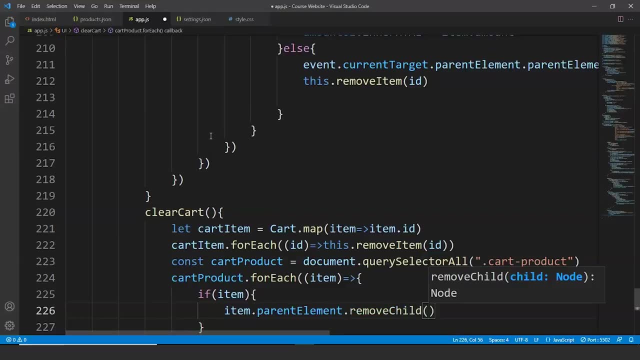 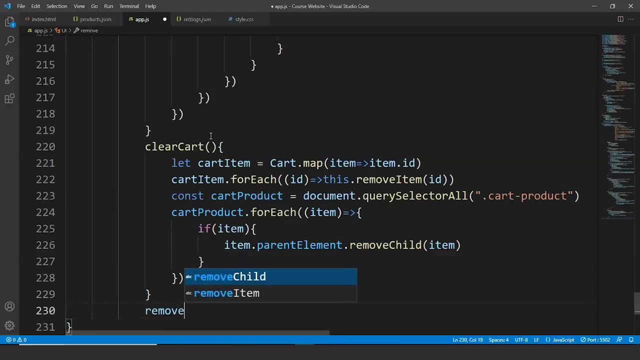 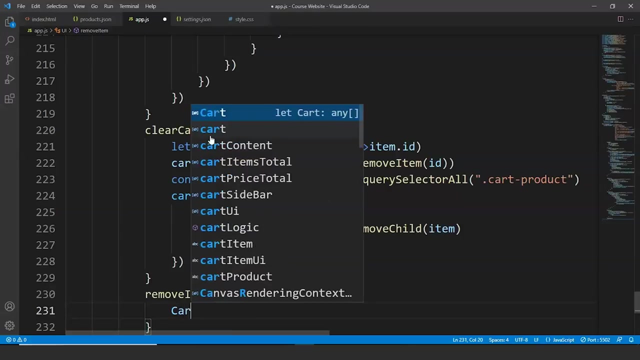 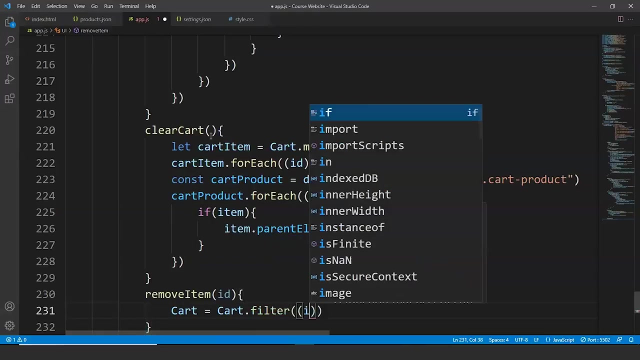 element: dot remove child will remove the item. Now we have to remove the item sofa that. we'll write here: remove item and we'll pass ID to that item. will write here: cart will update the value of cart test cart dot filter. we'll write here item and then we'll right here item dot Id, not a filter I'm gonna take. 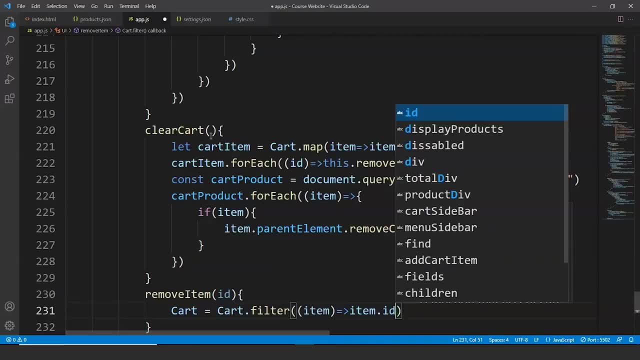 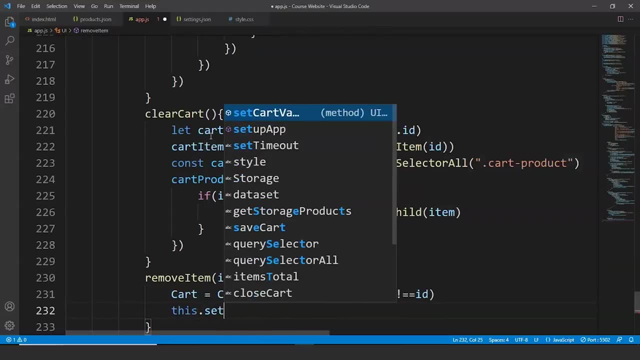 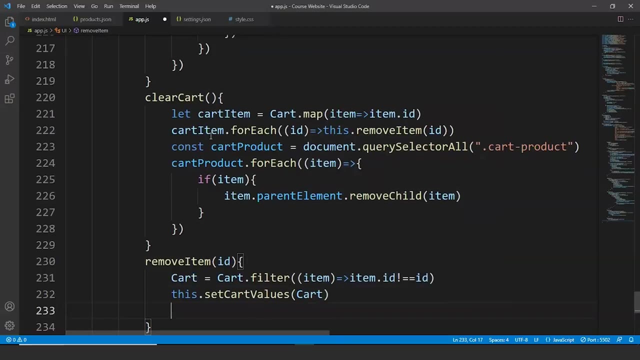 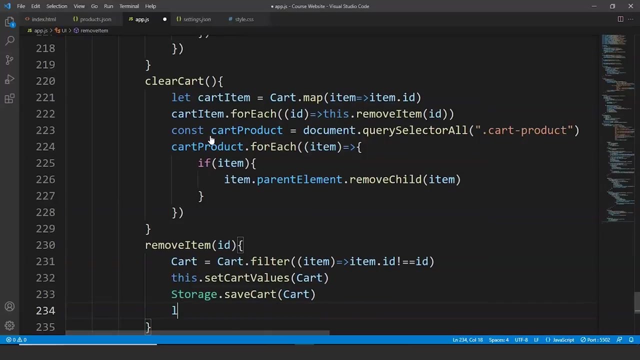 that out equals to id. this dot set cart values and we'll update the cart. then, similarly, we'll again write here storage dot, save cart and we'll pass cart here. then we'll write here: let button is equals to this dot get single button. we'll write here id and we'll change the button style. we'll write here button dot. style dot. 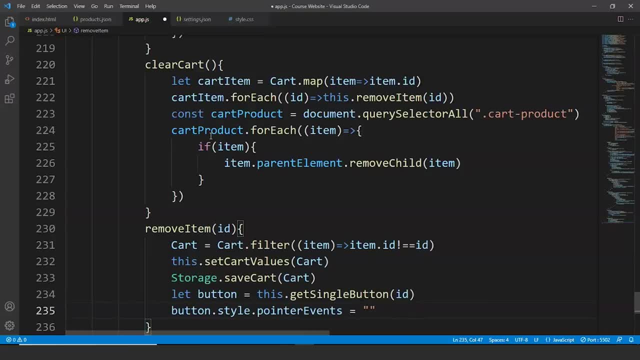 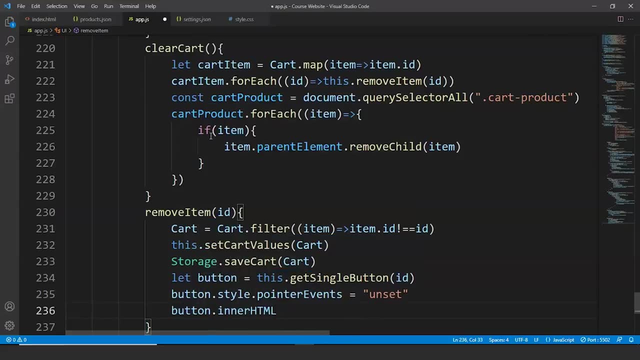 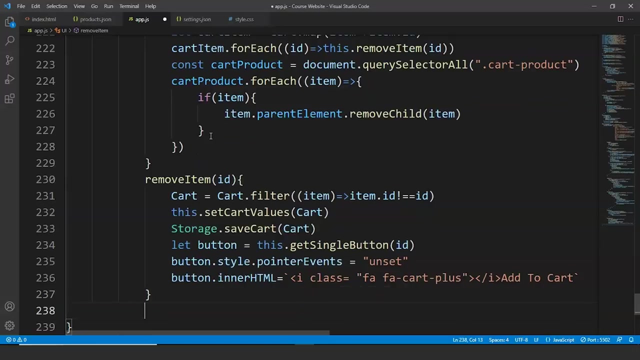 pointer events is equals to unset, Then we will write here: button dot. innerHTML is equals to backtick. I class will be far, far cart plus. We are going to close the I tag here and we will write here: add to cart. Next up we will write here: get single button. We will pass id over here. 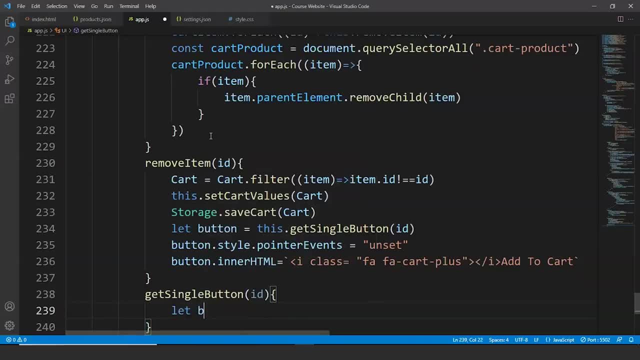 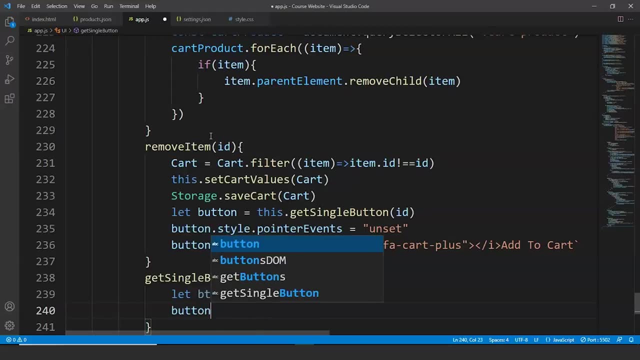 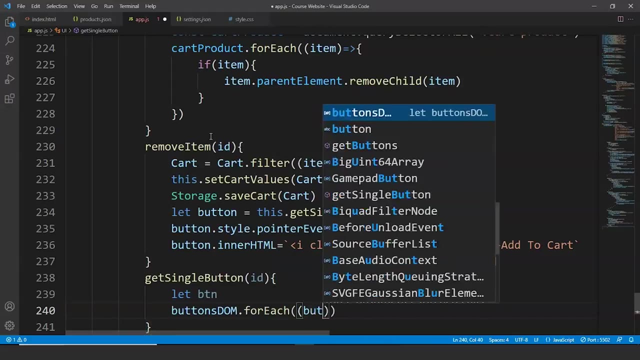 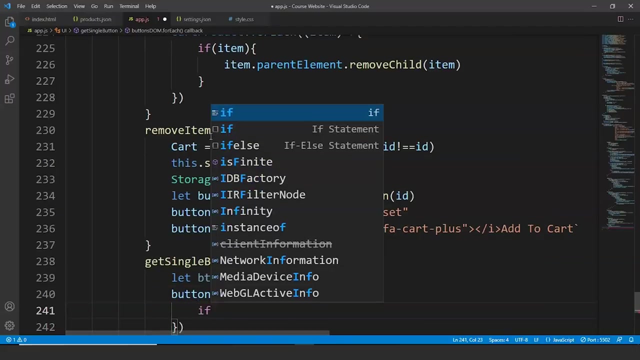 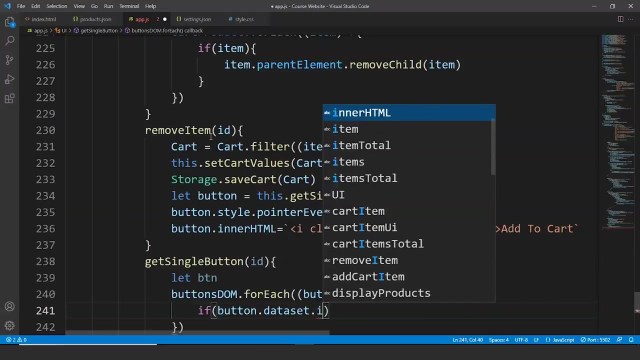 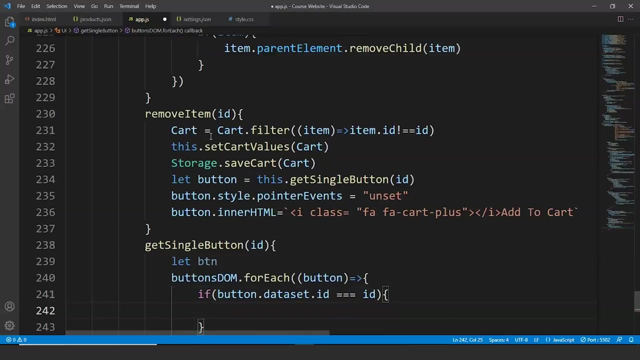 and we will write the code for here. We will write here: let btn. Then we will write here: buttons dom dot. add to cart For each button. what it will do is we will check if button dot dataset, dot id is equals to id, then btn equals to button. 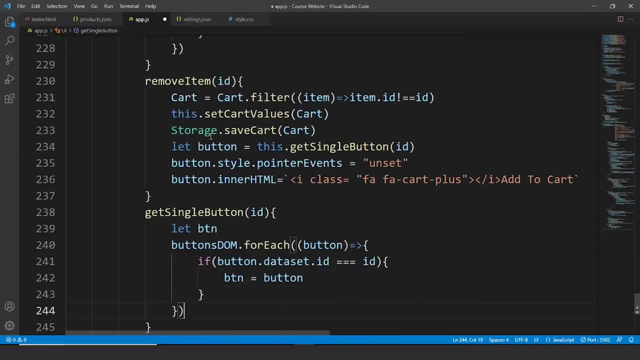 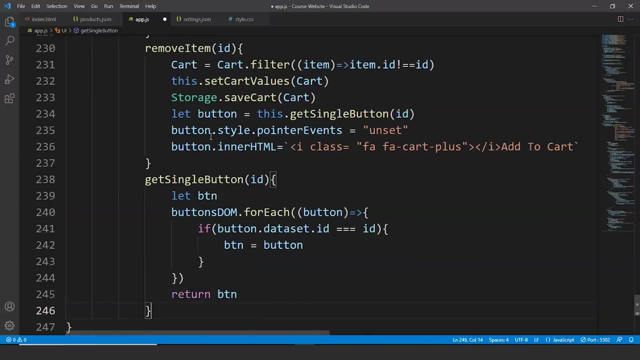 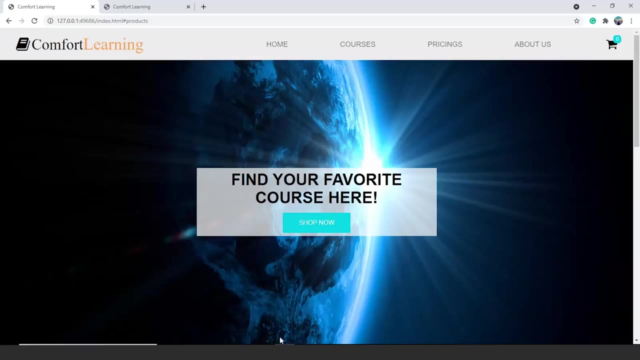 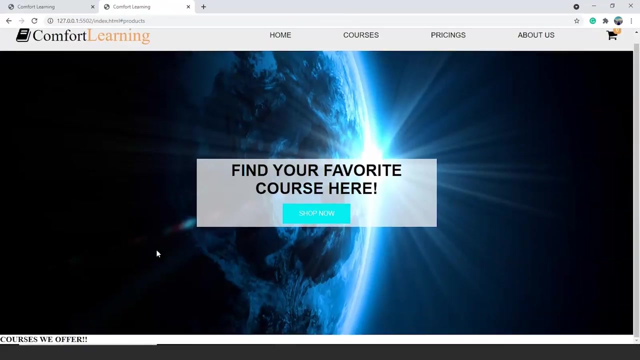 Fine, Here we will return button. Now save it. Save this program. go to browser, and this is our website. Go to browser and you can see nothing is visible till now. We have to write a little more code to make everything visible here. Now we have to start our javajs. 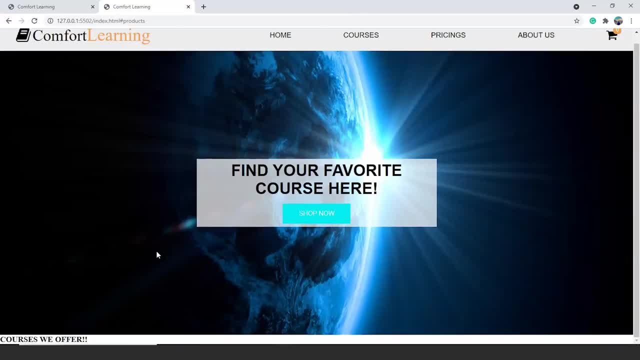 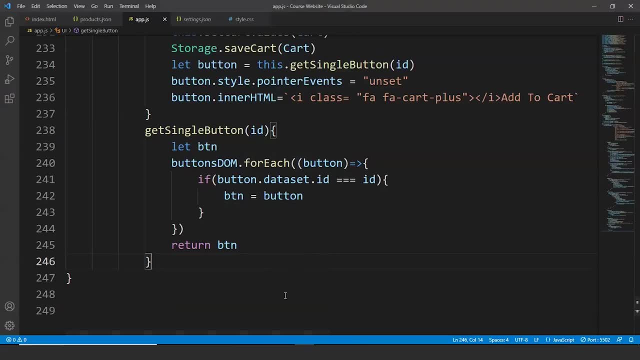 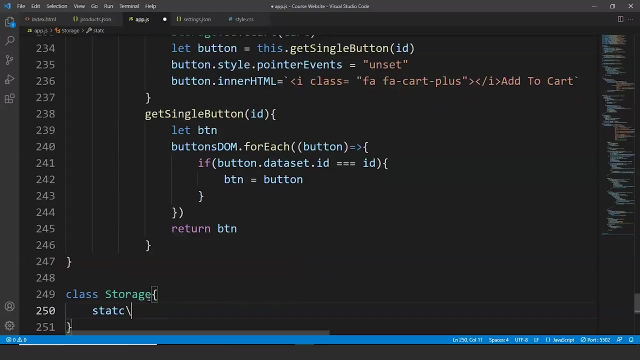 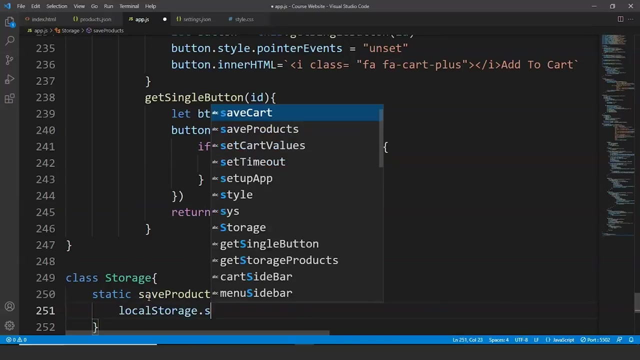 content, the data in local storage so that on refreshing the web page we don't lose the data. so what we'll do is we'll go back to a JavaScript file and we'll write here: class storage equals to static save. products will pass products here. then we'll open curly braces and we'll write here: local storage dot set. 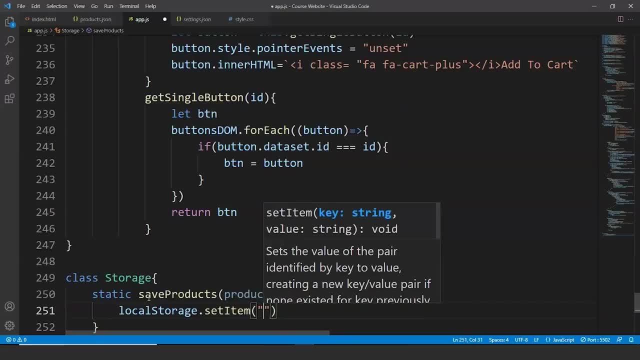 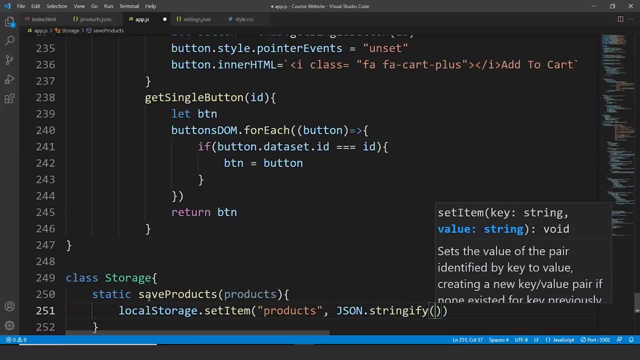 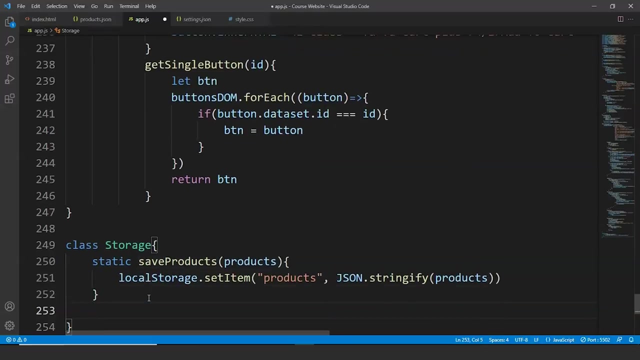 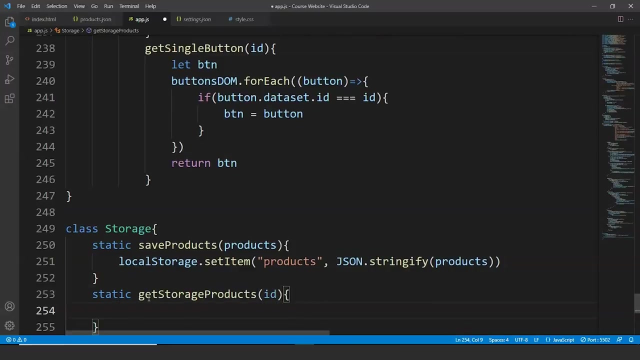 item and inside this will write products, dot, comma, json dot, stringify products. you and we are parsing the products from our JSON file. now next up, we'll write here: static get storage products will pass the ID here and we'll write here: let products is equals to json dot. 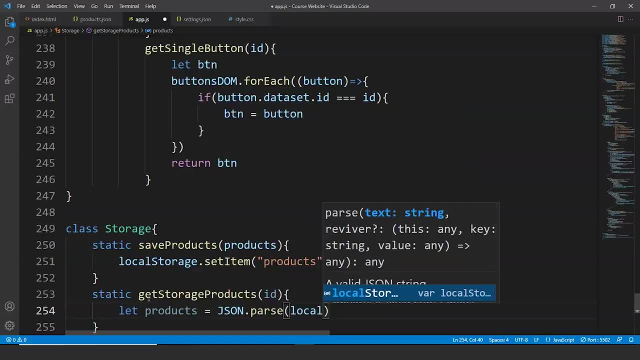 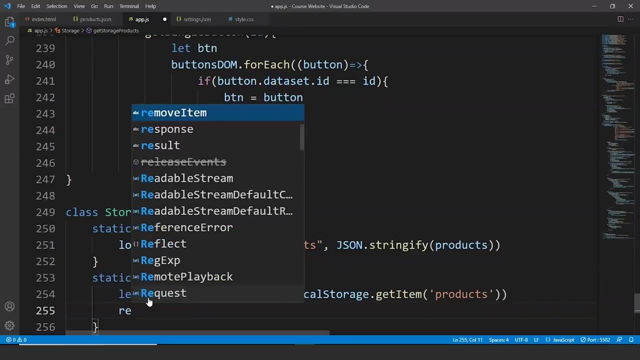 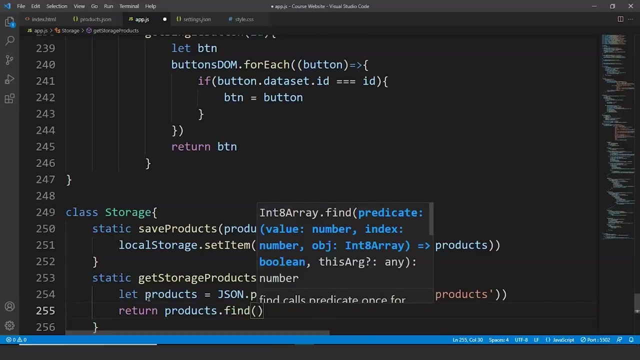 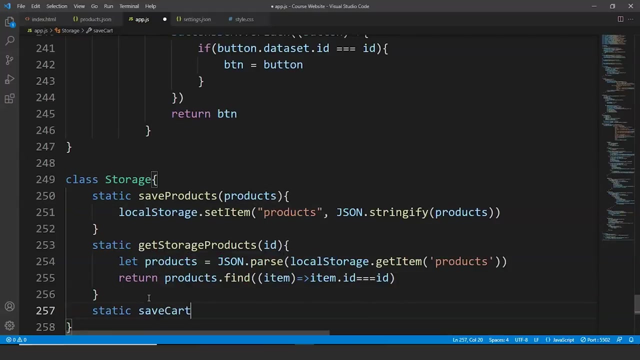 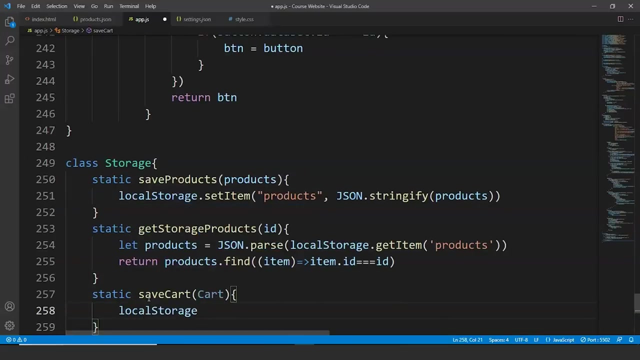 parse: local storage, dot. get item and we'll pass products here. fine. in the next line we'll write return products dot. find will write your item item dot. id is equals to id. fine. next up we'll again write here: static save cart. now we are saving the products or in our cart, so we'll write here: local storage, dot. set item. 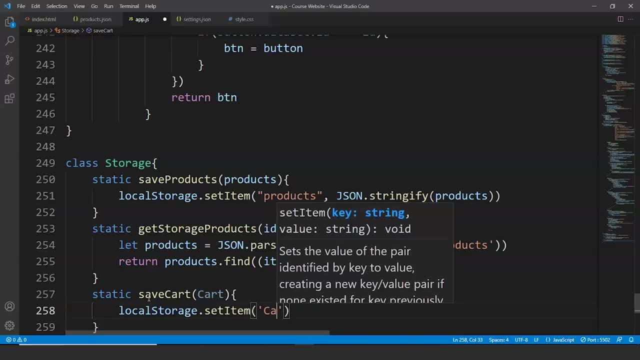 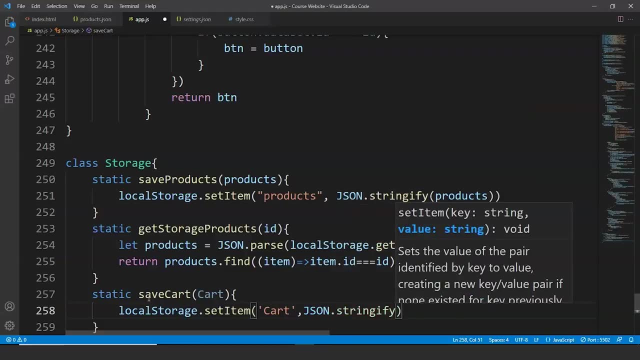 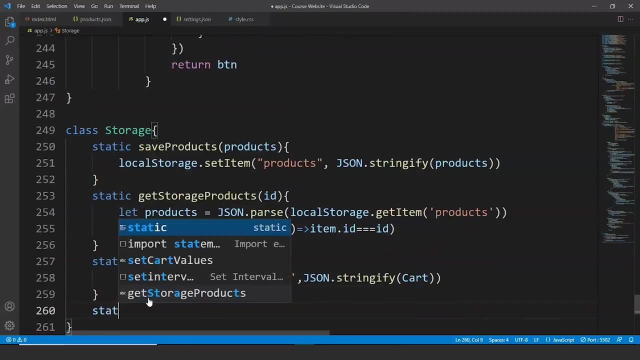 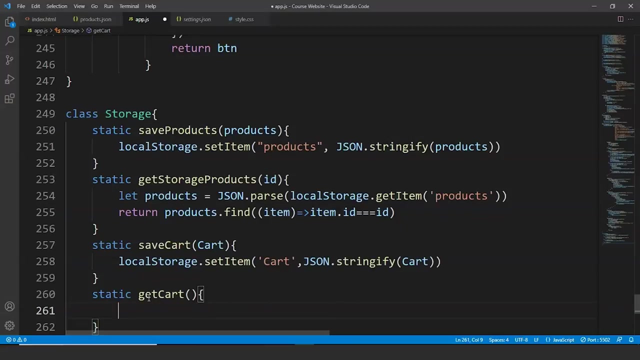 inside. here we'll pass cart and here we'll write json dot stringify and we'll pass cart over here. next up we'll write here: static get cart. we are getting the items from the cart. we'll write here return local storage dot get item cart. here we will write question mark. 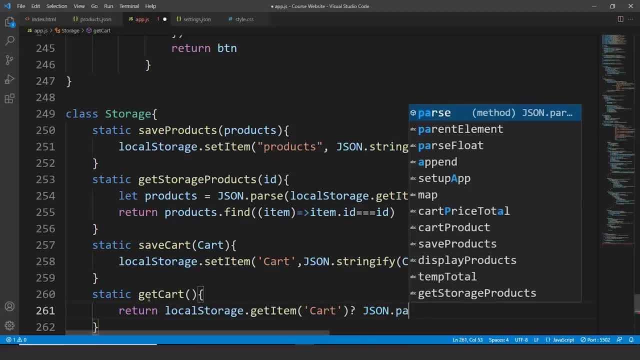 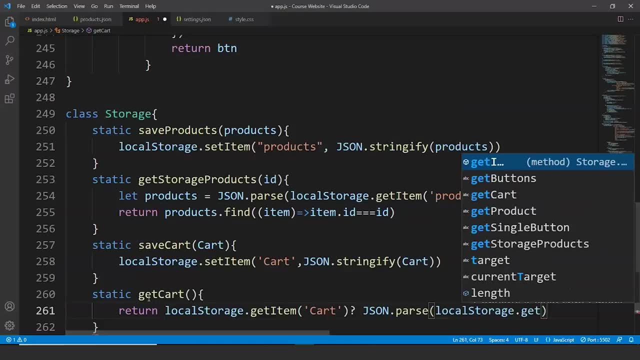 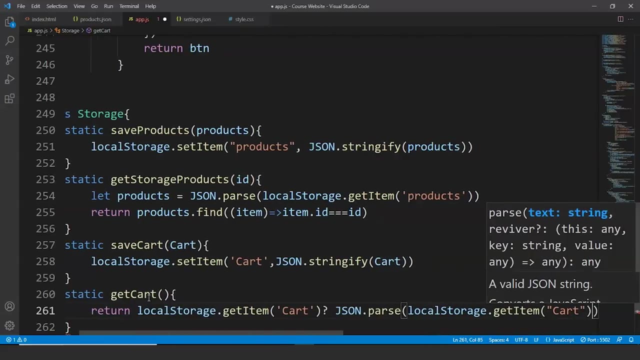 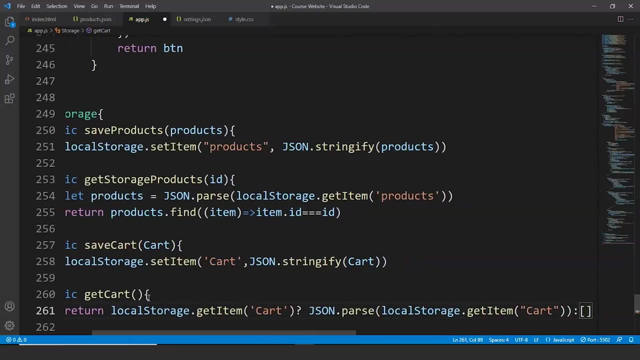 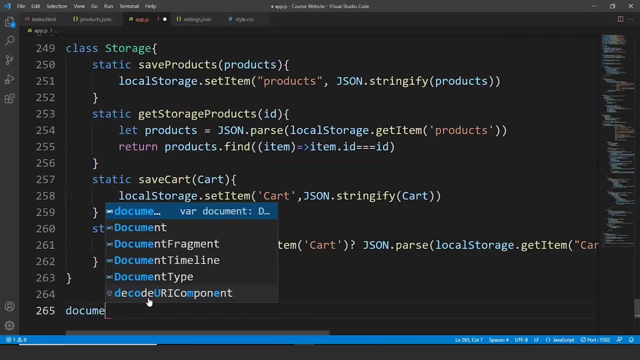 we will parse the json file here. we will write here: json dot. parse local storage dot. get item from the cart. fine, here we have to put a square bracket, a pair of square brackets, and lastly, we have to write a few lines of code. so we will write here: document dot. add event listener. 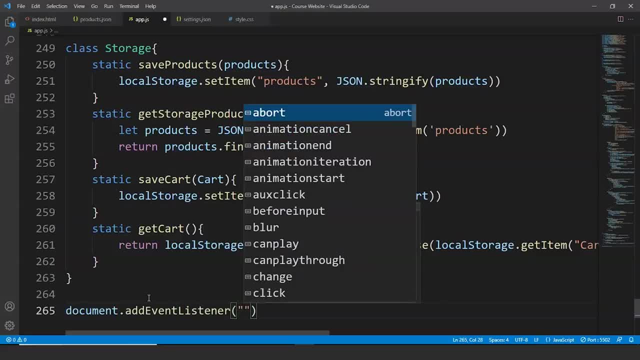 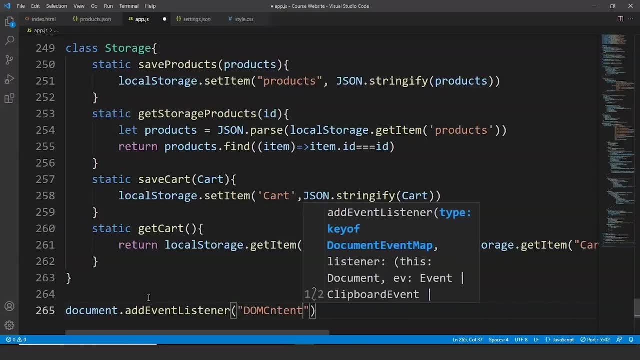 and we will write here dom content loaded. so we are adding one more event to our json file. here we will write here json dot javascript file, which is the dom content loaded. so we have to write here dom content loaded. and here we have to write inside the function. 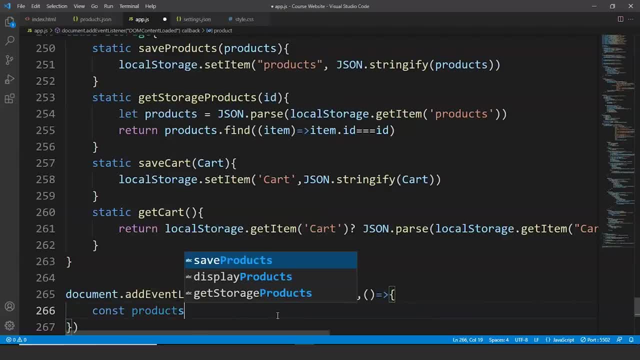 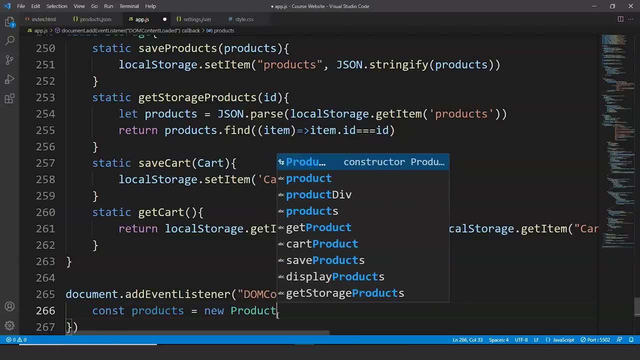 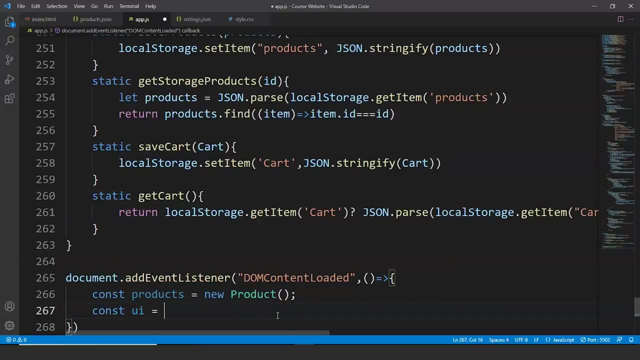 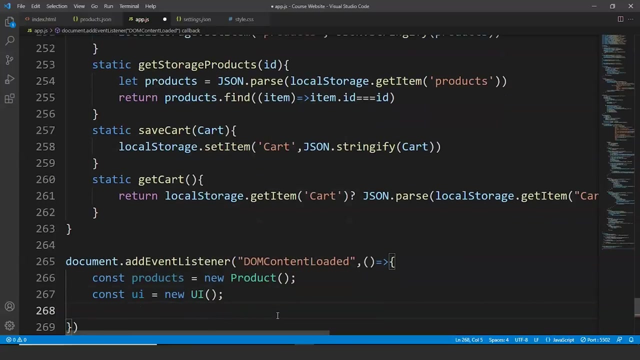 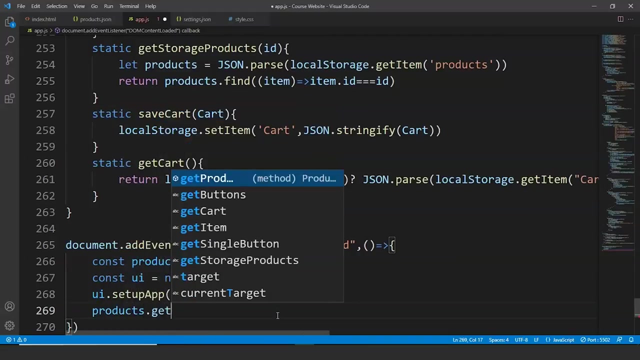 const products is equals to new product, and we will write here: const ui is equals to new ui. now we have to show cart from local storage, so we will write here: ui dot setup app and we will write here: products dot, get product dot then and we will write here: products dot, get product dot then. 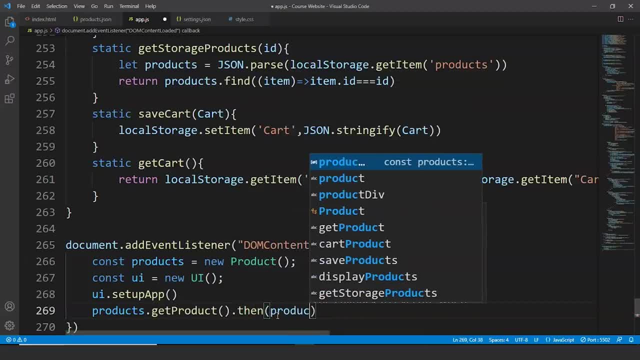 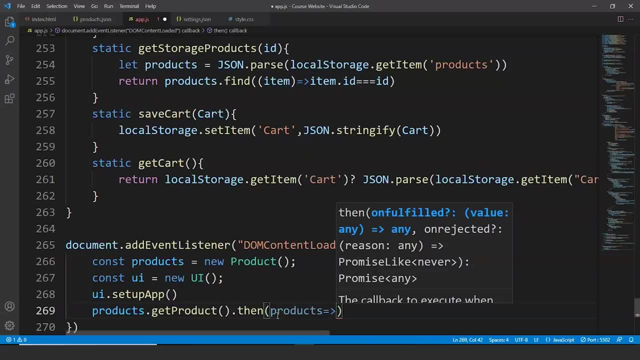 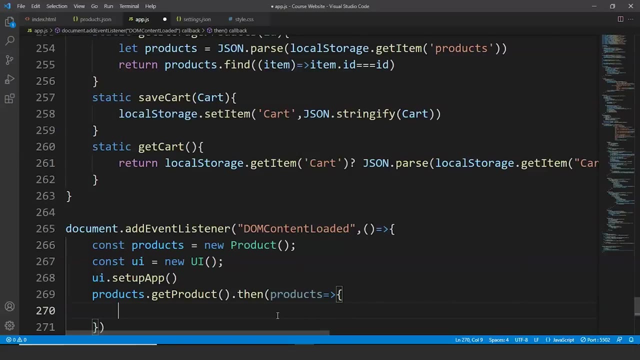 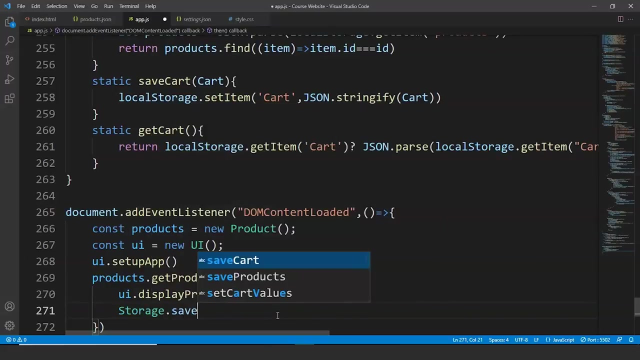 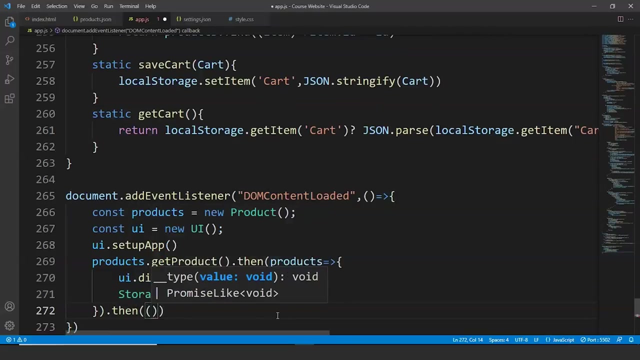 and inside this we will write products. equal implies ui, dot. display, display products. we will write here: display products, products, storage dot. save product and we will pass products as well. fine, we'll write here dot. then we are using promises, so type in a sweet word and inside of standard. 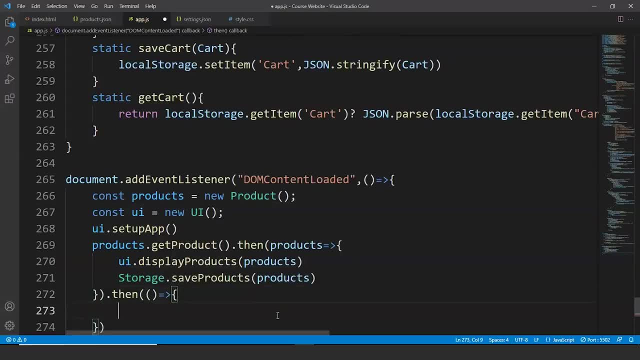 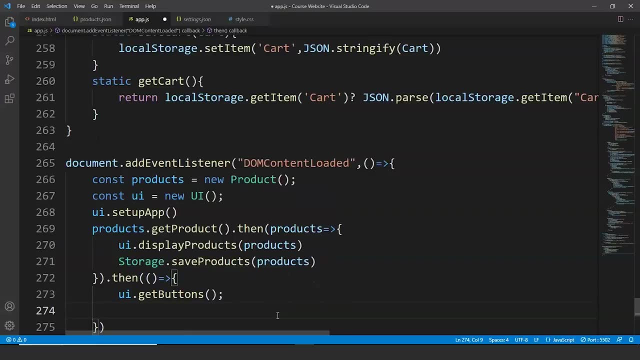 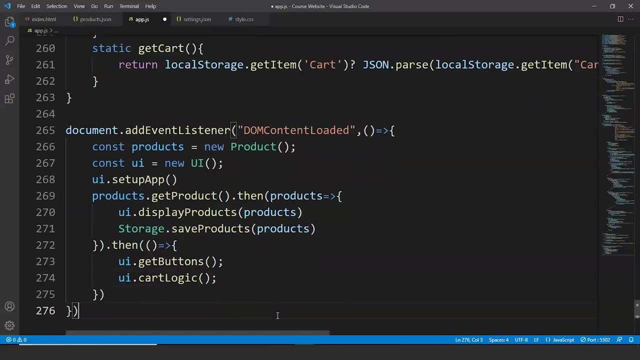 ui dot get buttons and ui dot cart logic. fine, now the javascript part is done. we have used json here to make our web page more responsive towards several aspects. apart from that, we have used json for adding products to our website as well. now we are left with one more task only. 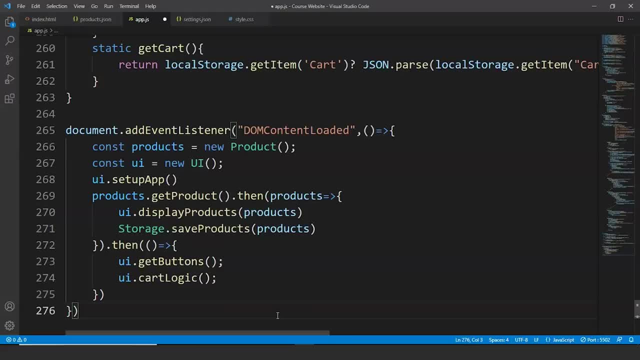 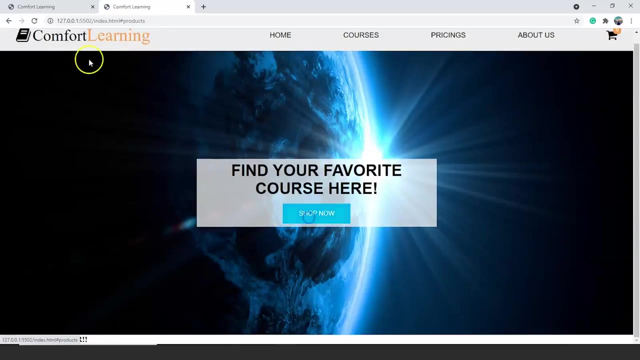 let's do it and then we'll see the final outcome of this extended code. so we'll move to the css file and we'll start starting the products part. let's try if it's working or not. let's save this piece of code and go to browser. click on shop now and it's not working? we can see. 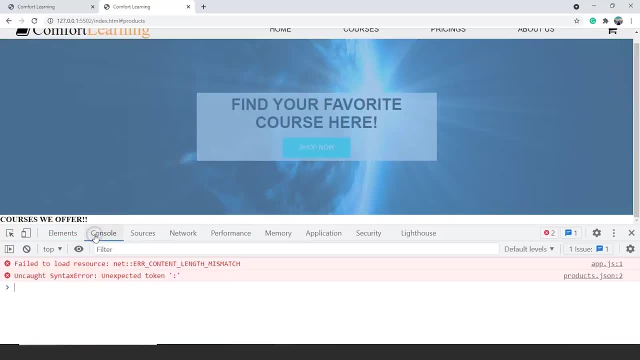 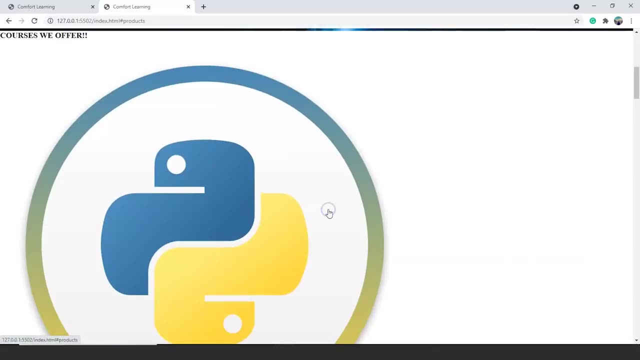 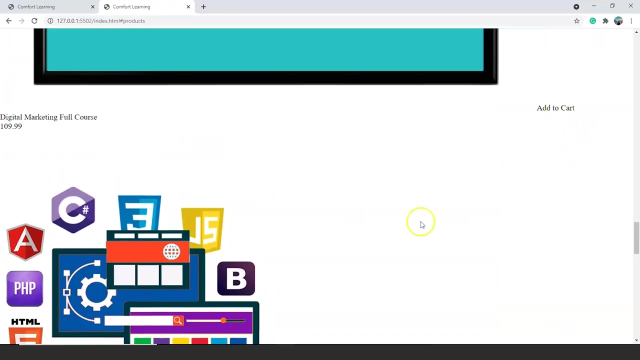 you okay. it says it's failed to load the resource. refresh it and you can see. now it's working totally fine. we have all our product images over here. we have all of our products, we can add them to cart and we can use the cart as well. so the last thing we have to do is to use products now. 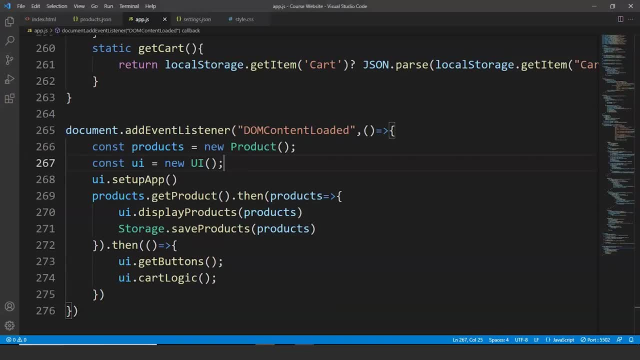 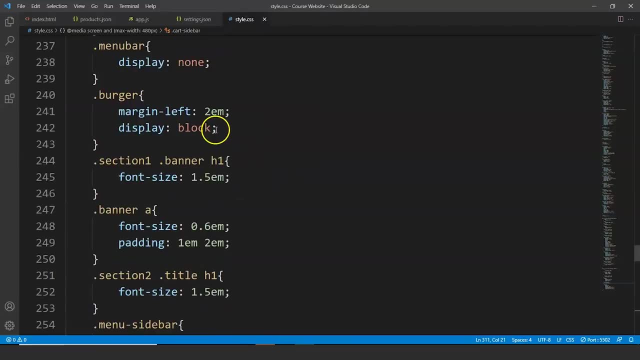 now we have to style those products, so for that we'll move to our css file. so here's our css file and we'll move to our css file. and we'll move to our css file. and inside this we have to write here. so we have put a comment over there when we were not here. so 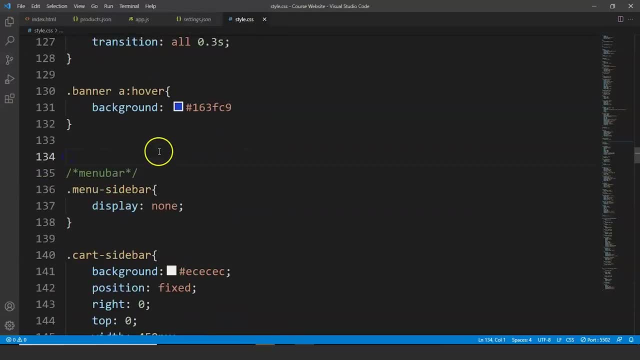 we have to style the products over here, so for that we'll write here: dot, section 2, dot. title and text align at the center. then we'll write here, section two, here and so on, so we're going to change to headline. so then we were not here for this one where we have to use the text for the great title. 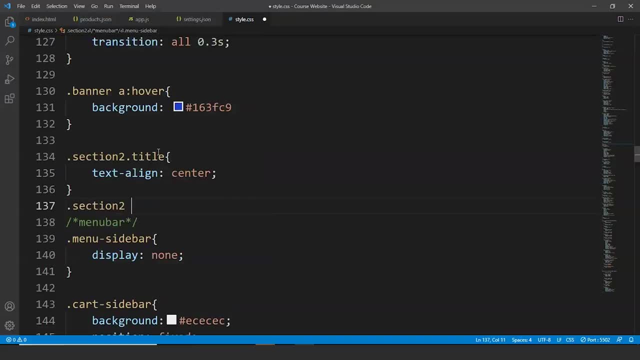 and we have to be correct with int cost correction. we will apply it in gpub on this file to provide some results which we will see today, we have to change the default file to css file to the gpub implementation. 2 dot title h1: the font size is going to be 1.8 M. the margin is going to be 1.3 M. 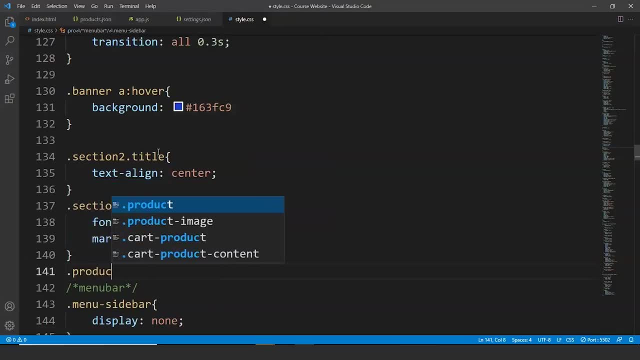 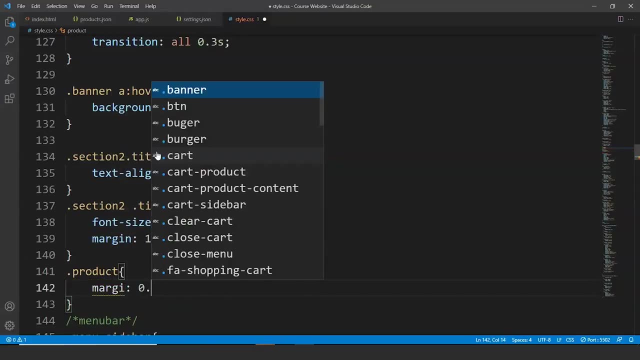 then we have to write the code for products here. so we'll write here dot product and inside this we'll write margin as 0.5 M. we have to write here margin, right here: 0.5 M, and auto max width is going to be thirteen hundred pixels. display is going to be grid. 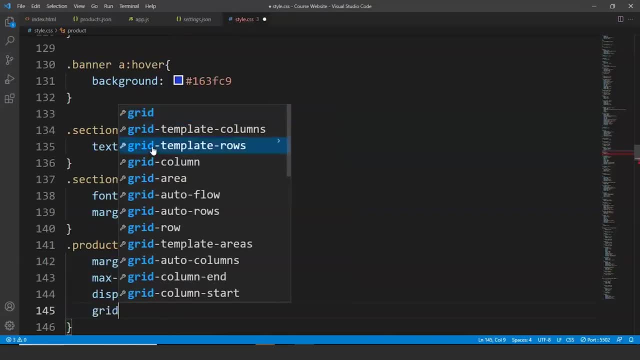 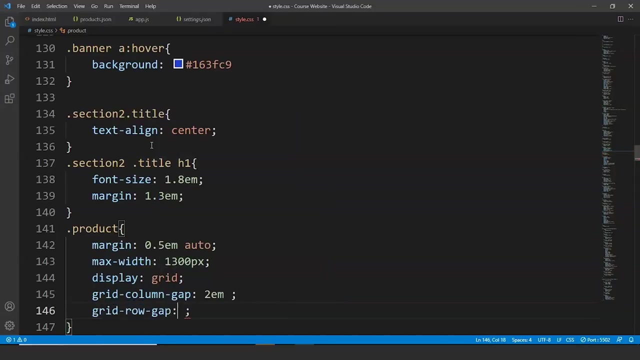 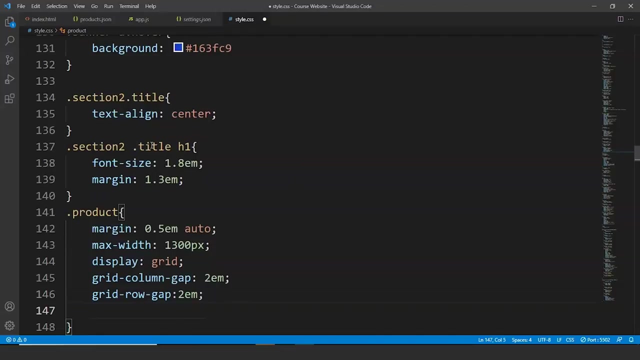 grid column is going to be so here it is going to be grid column gap and it is going to be 2 M. then we'll write here: grid row gap and grid row gap is going to be 2 M as well. then we'll write here grid template columns and we'll write here- repeat: we are going to 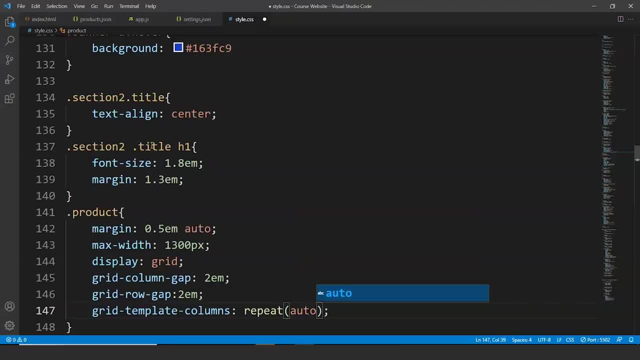 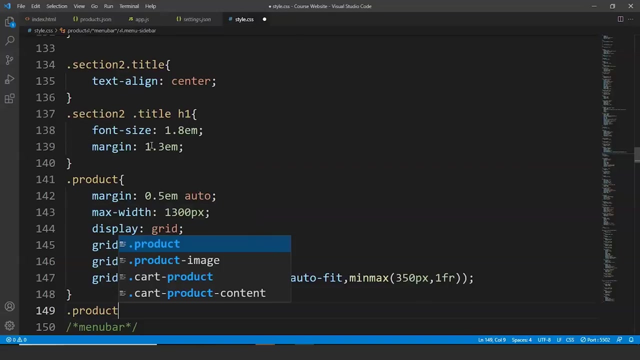 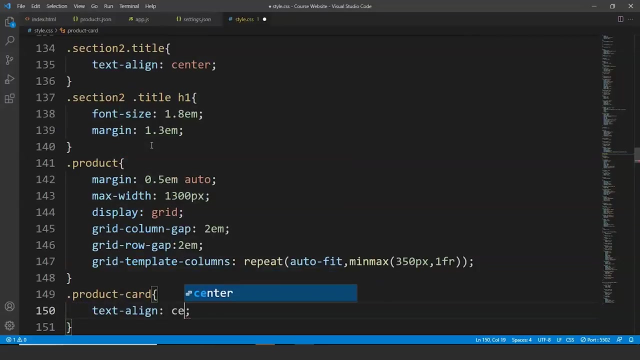 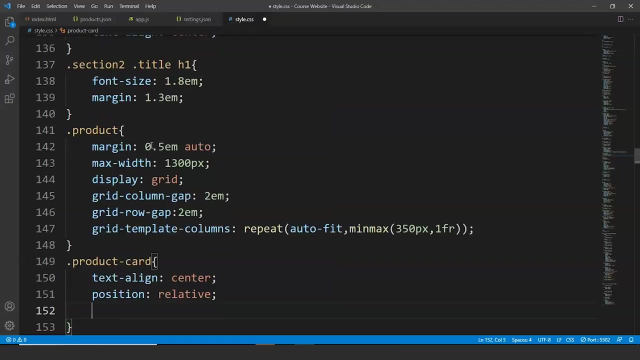 create a grid for a products right. so we'll write here Auto fit comma min max. will write here three, 50 pixels and one draw fine. next up, we'll write here dot product card. and now we are going to write here: text align as Center, position as relative. 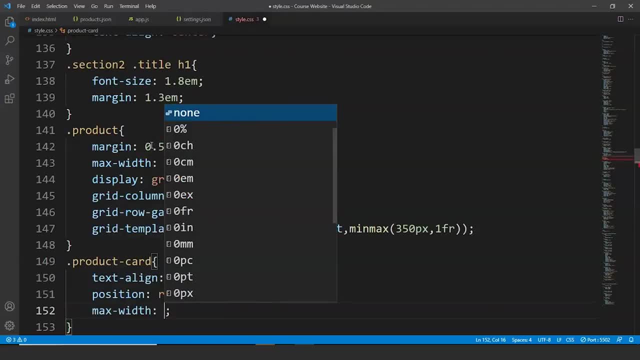 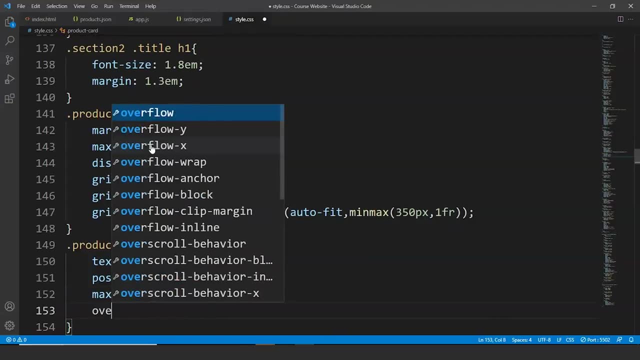 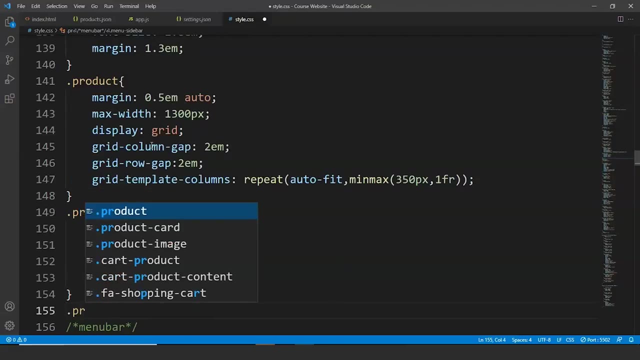 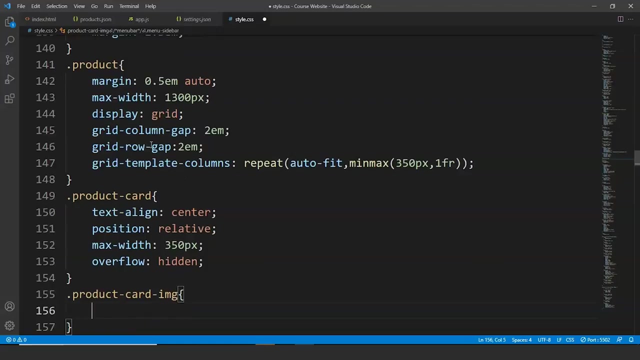 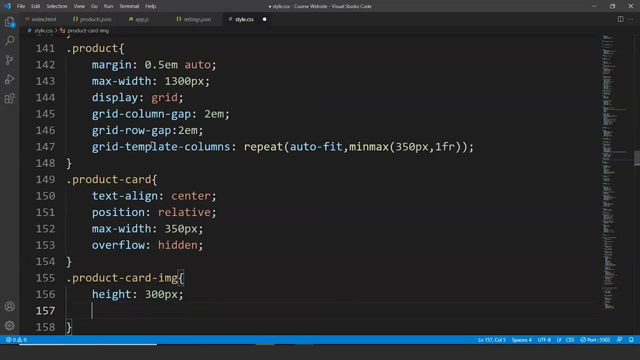 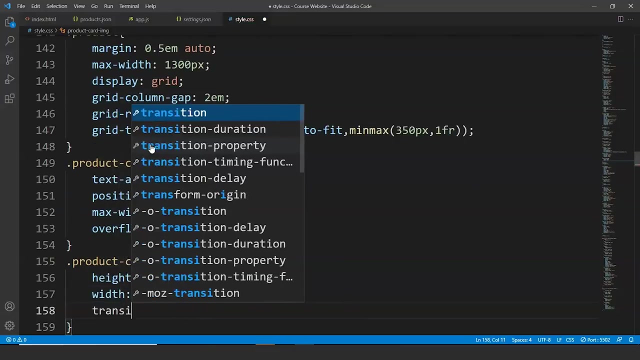 max width of the grid is going to be 350 pixels and overflow is going to be hidden next up. we'll write here product card image. we'll write here height as 300 pixels, width as 300 pixels and transition is 0.3 seconds, linear. fine, so early we'll do. 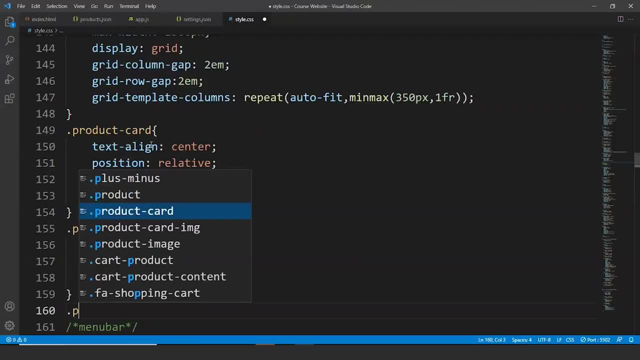 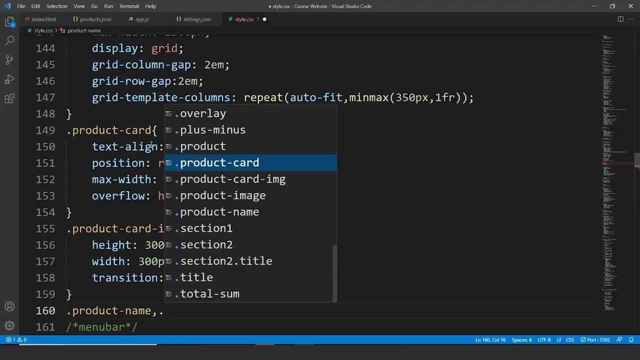 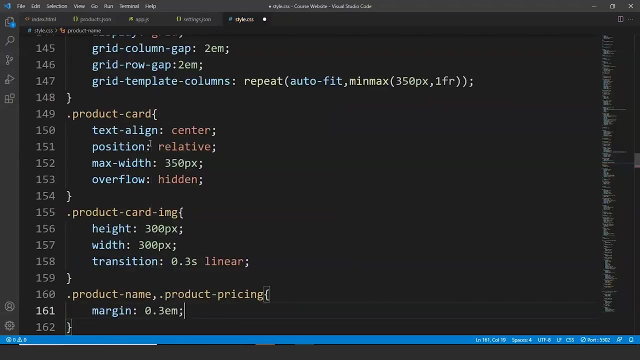 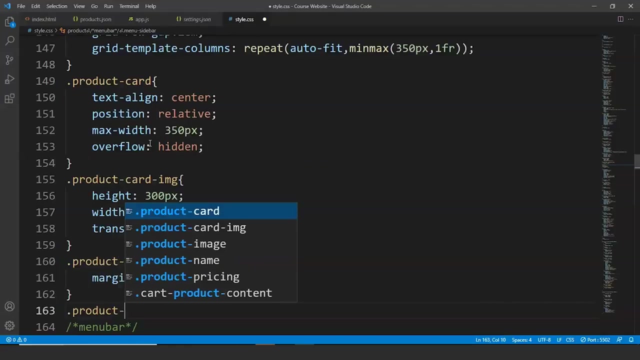 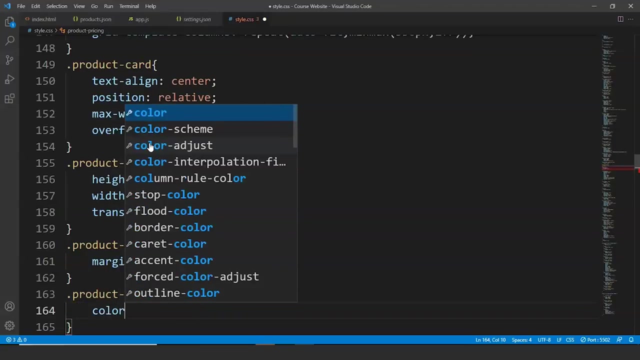 the same for product name and product pricing. so we'll write here product name: comma- product pricing margin for them is going to be 0.3 m. we'll write here dot- product pricing, and the color of the product pricing is going to be the one we have. 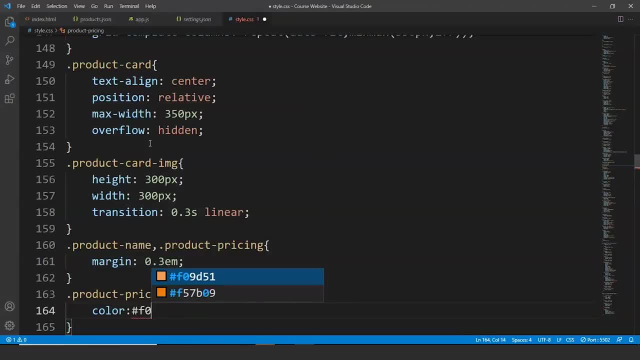 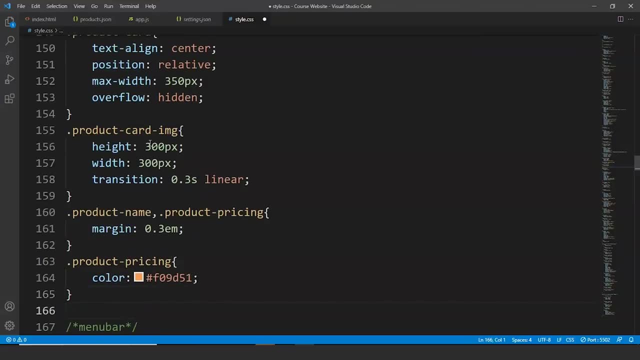 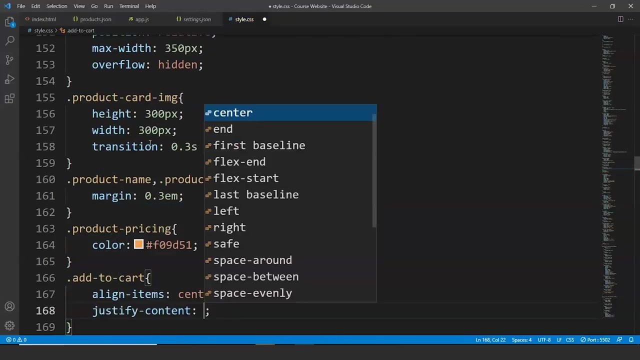 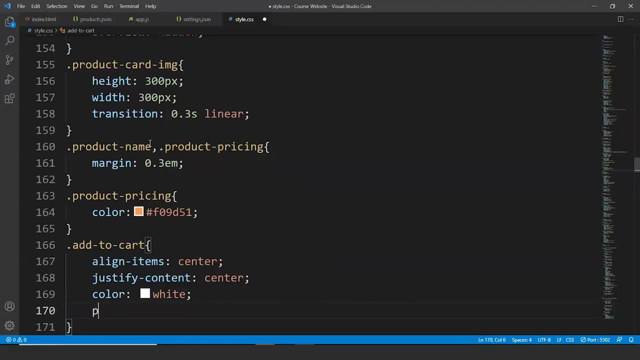 been using till now, so we will write here: F09D51. then we have to write the code for add to cart button, so we will write here: add to cart. we will write here: align items to the center, justify the content to the center and color is going to be white. padding is: 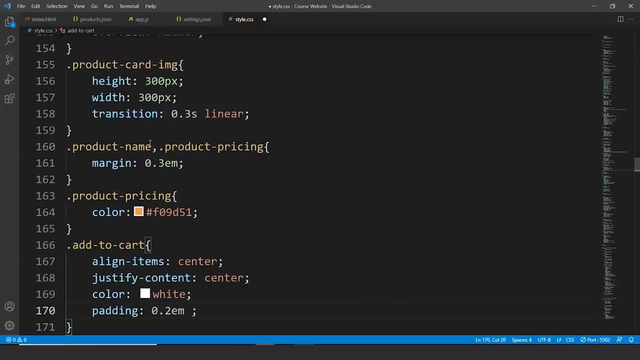 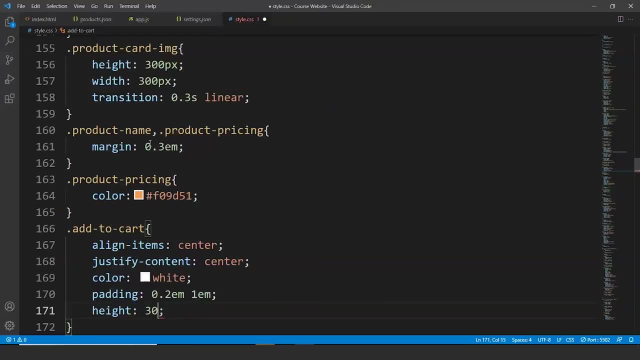 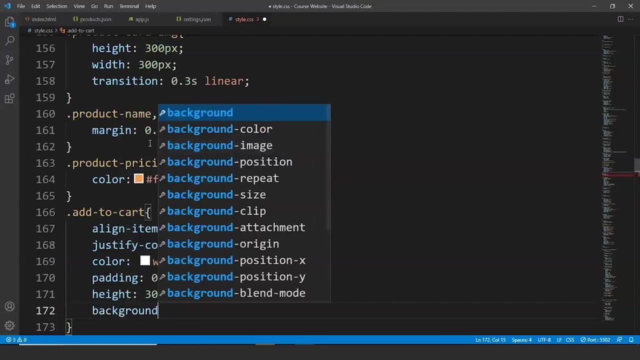 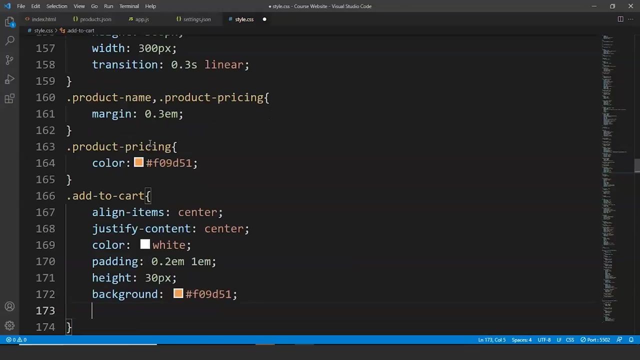 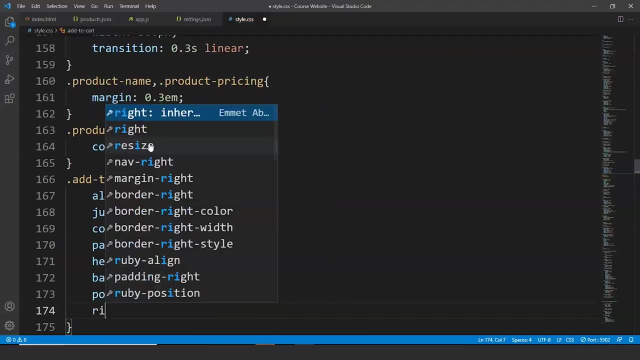 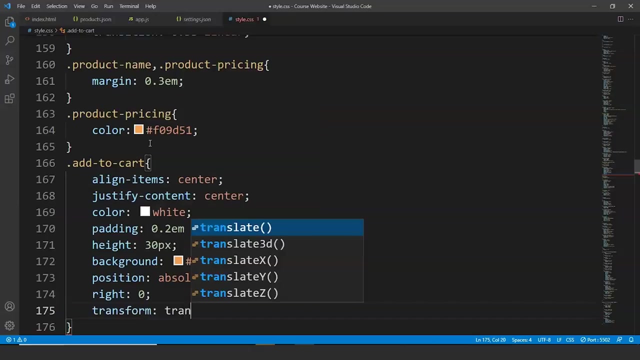 going to be 0.2 m and 1 m. fine height is going to be 30 pixels. background is going to be the same. F09D51 position is going to be absolute right is going to be 0. transform is going to be translate along the x-axis to hundred percent. 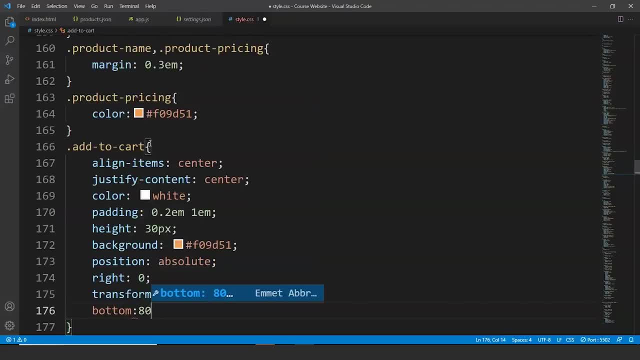 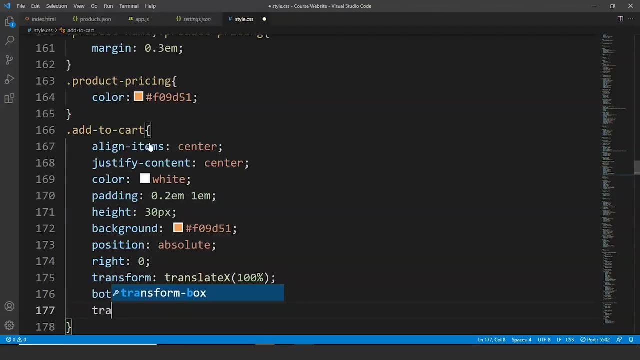 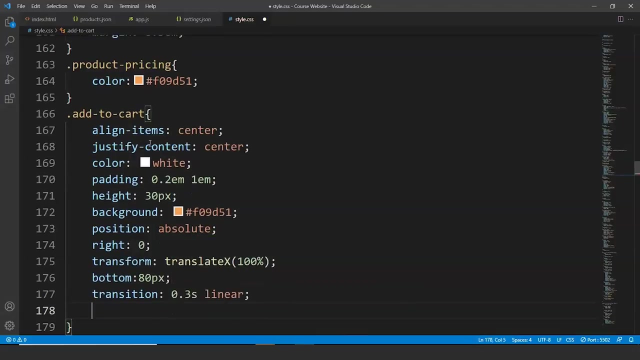 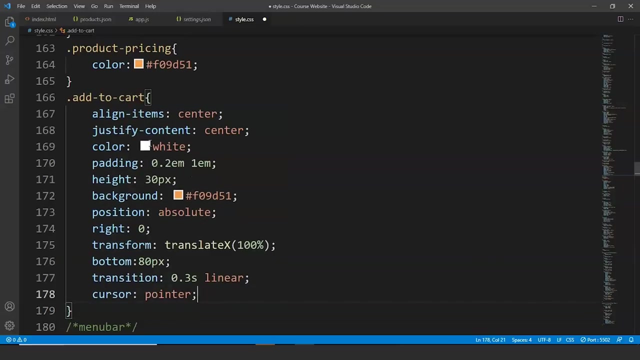 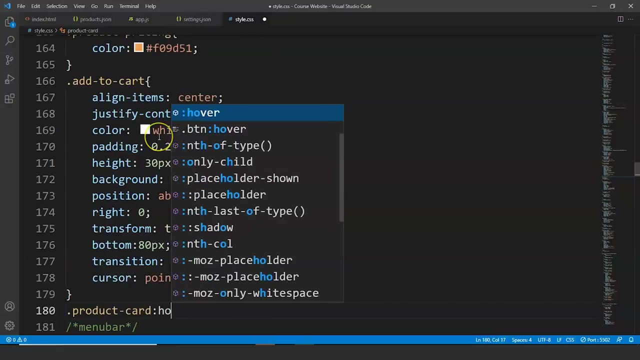 bottom is going to be 80 pixels. you have to put a comma here. bottom is going to be 80 pixels, transition is going to be 0.3 seconds again and linear cursor is going to be pointer. fine, then we have to write few more lines. so we will write here: product cart. we will. 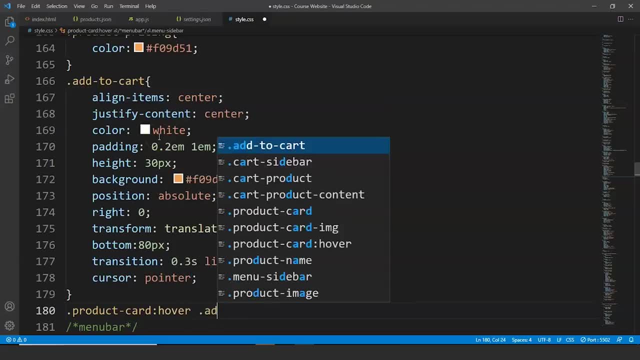 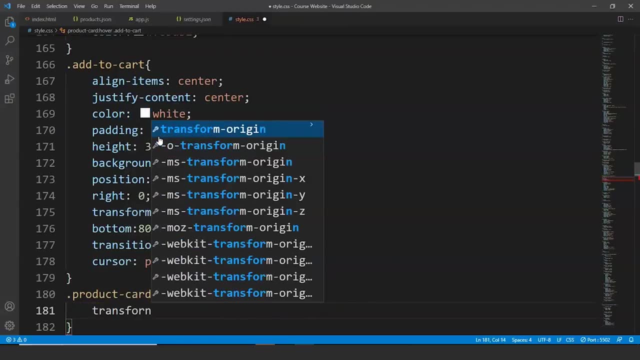 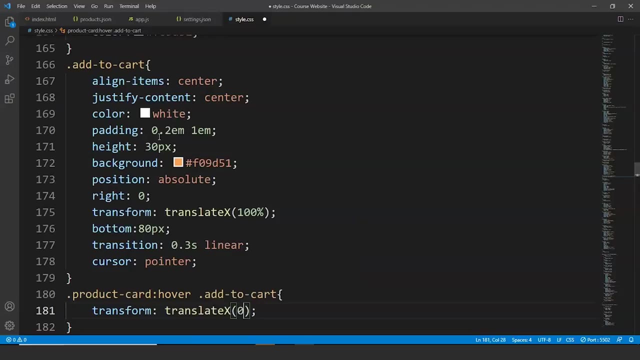 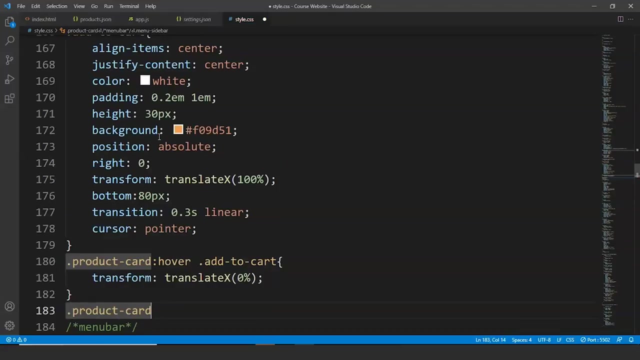 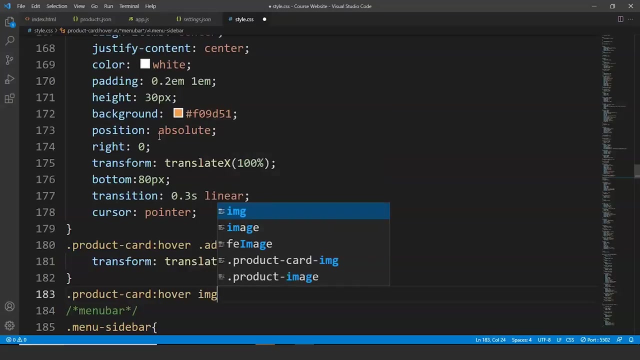 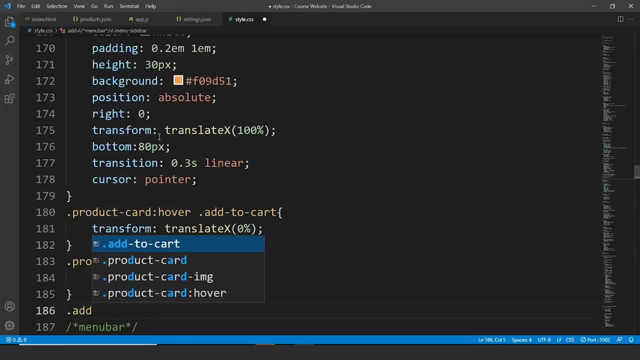 write here: hover, and we will add add to cart here. so we will write here: transform, translate x 0 percent. We will write here product card on hovering over the image. so we will write here: hover. img opacity will change to 0.7. let's try it. and finally, we will write here: dot, add to. 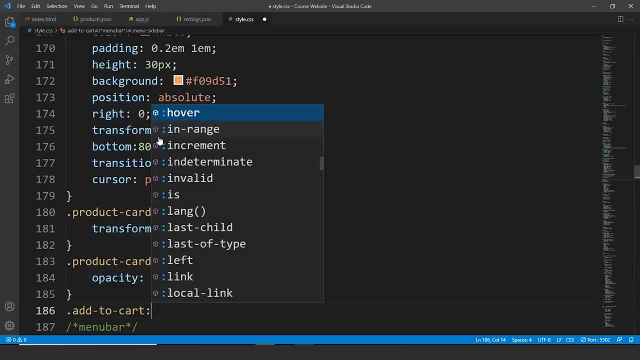 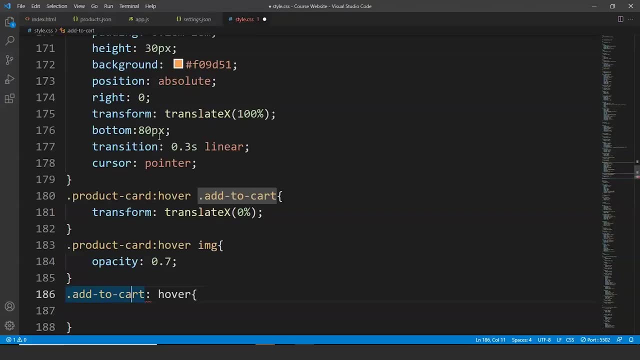 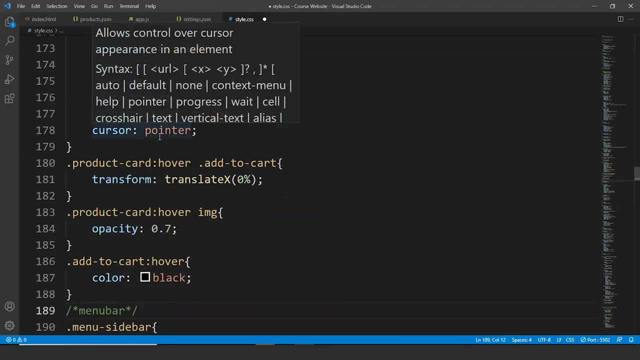 card over and here we will write color as black. fine, we are done with it. we have styled the products as well. we are now done with the website. save it, Move on to the browser and let's face the truth now. so you can see, it's not working. 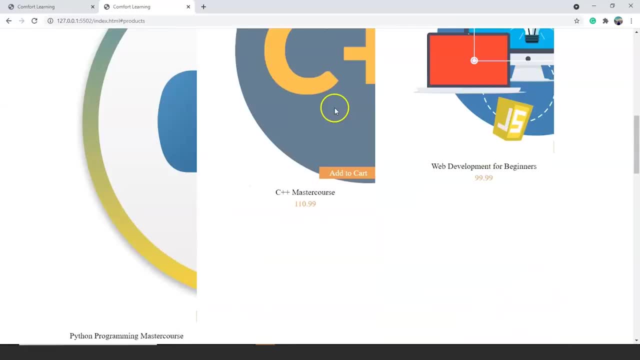 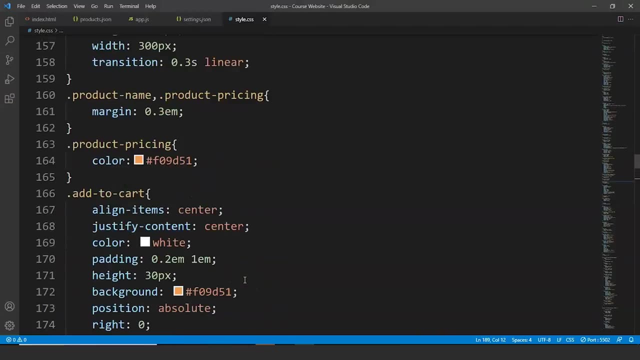 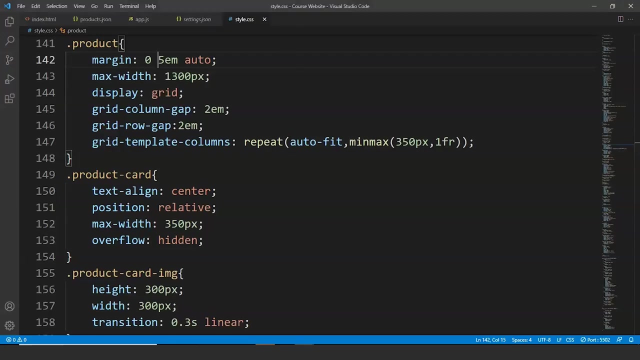 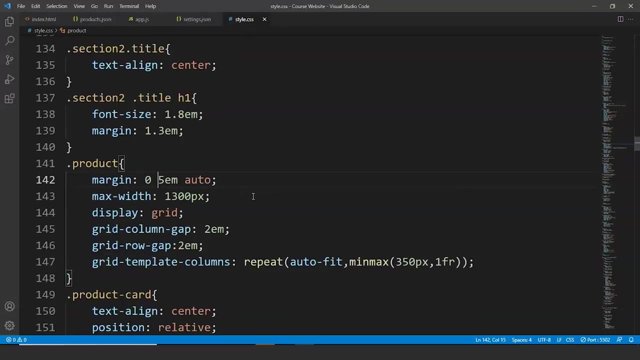 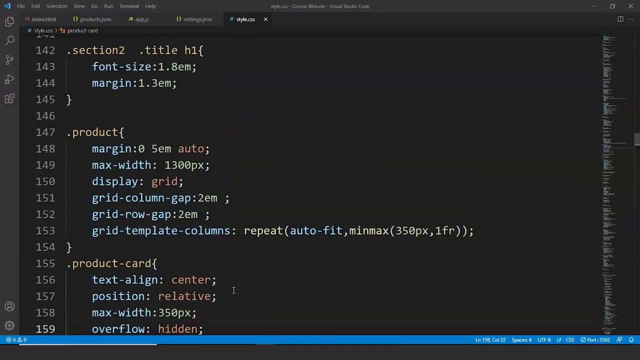 as of now, refresh the web page and the products looks really big. now what we have to do is we have to move over here and we have to see what's wrong over here. this was a mistake and it's done. let me see. Something is not right here. everything seems fine, but we have to search for the error. so 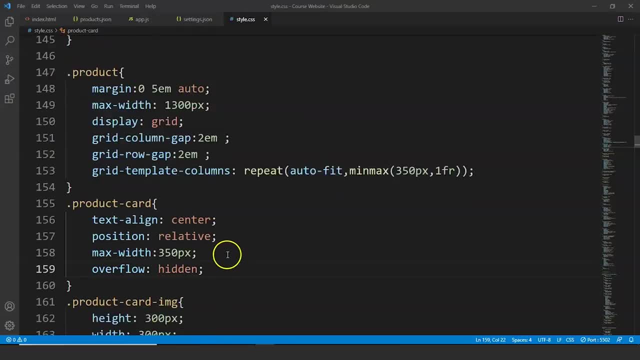 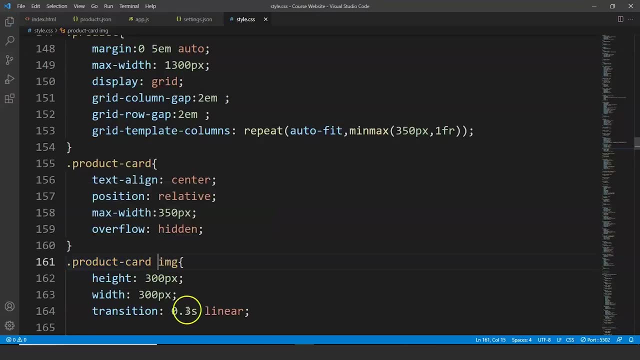 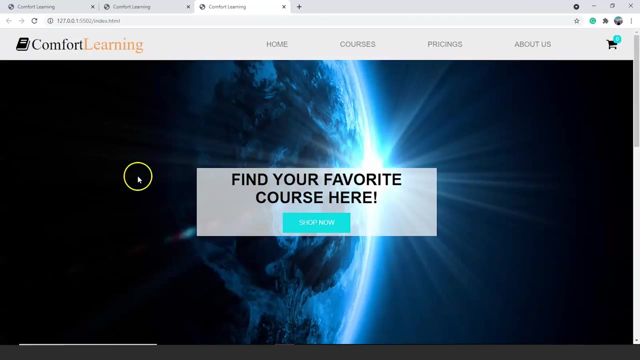 if we see here: max width is fine, the max width for product is fine, let's try to do this thing. we will write here this: save it now, and I know that this is the error we did so. such small errors sometimes cost us way more, So we will do this again. let's go to the browser and you can see our website is fine now try. 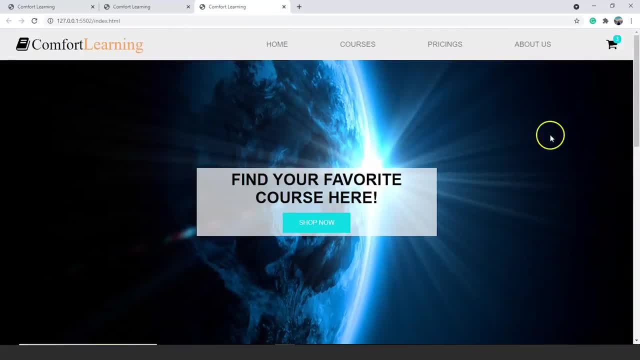 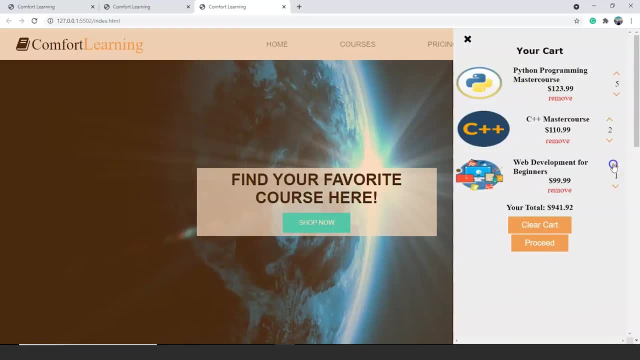 adding the products to the cart. you can see. the products are in the cart. we can increase the number of products. the total is increasing with that and it's working totally fine. click on the clear cart button and it's not working. click on the proceed button and it clears. 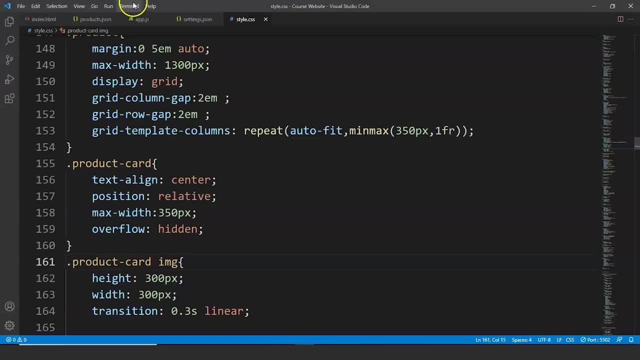 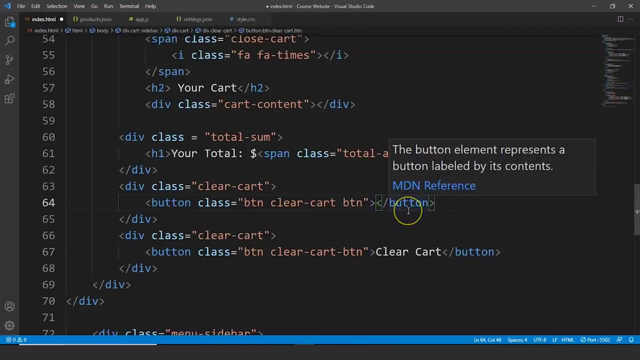 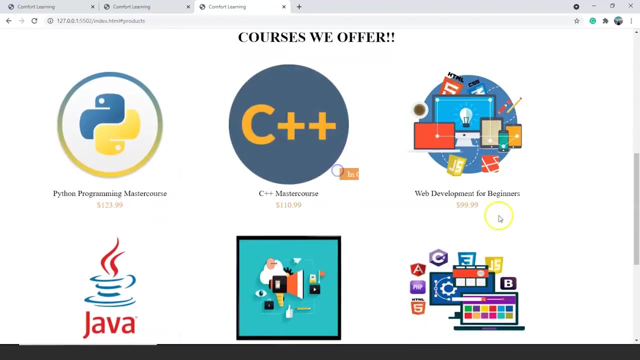 the cart. A simple solution for this. Go to the browser. Go to the browser. Go to the browser. the HTML file, write clear cart over here and proceed over here. save it. move to the browser. try adding products to the cart. go to the cart. increase the numbers.